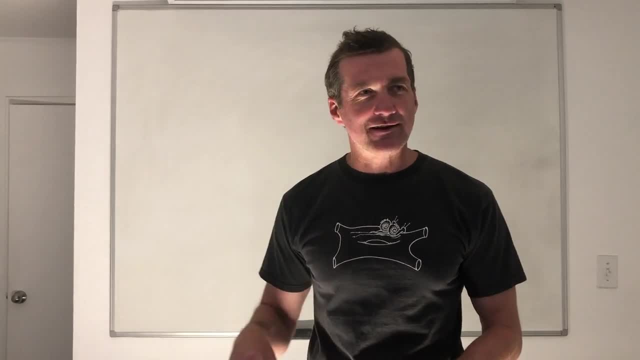 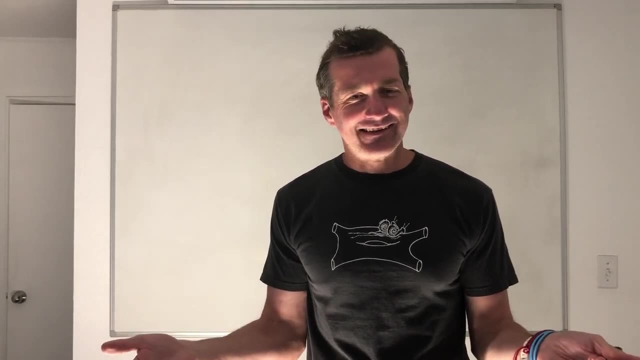 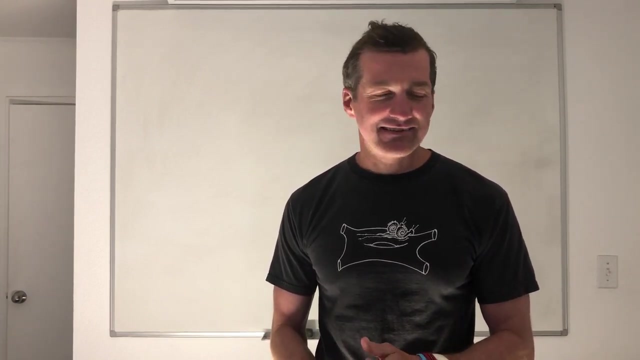 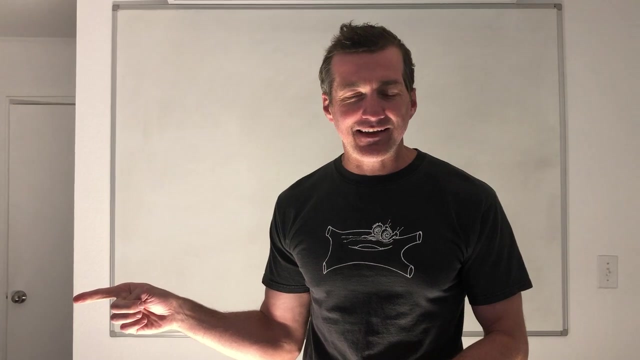 just, maybe I have it set so that if you sign on, you're automatically muted. but why are you all on mute, like right now? we're like socializing, are you serious? that's, that's, that's ridiculous. well, are you gonna keep looking over to the right Avery throughout my entire lecture? yeah, yeah. 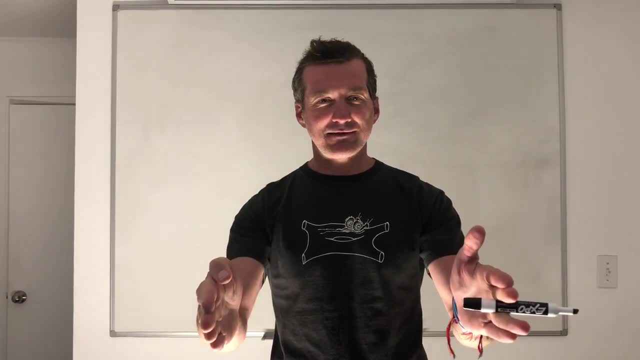 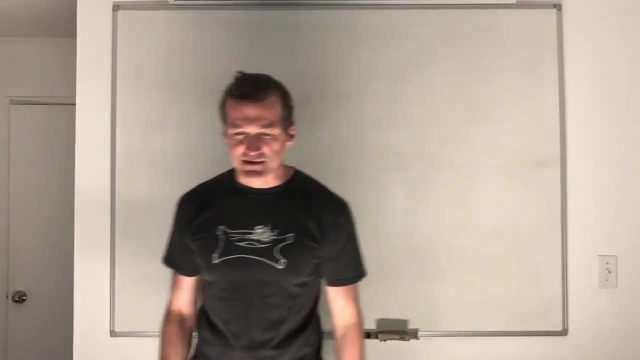 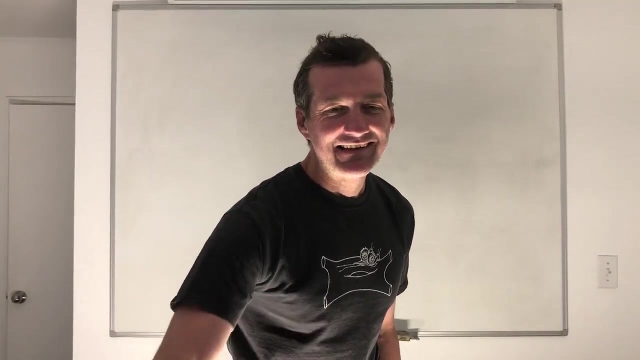 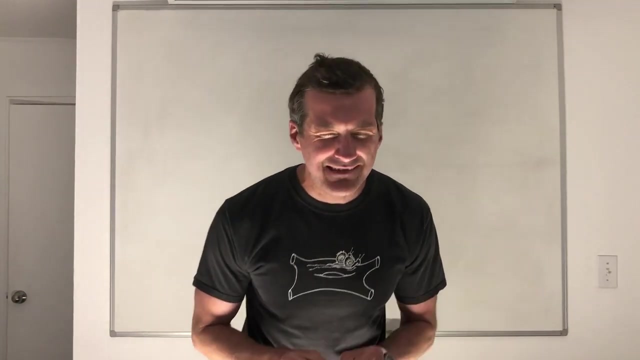 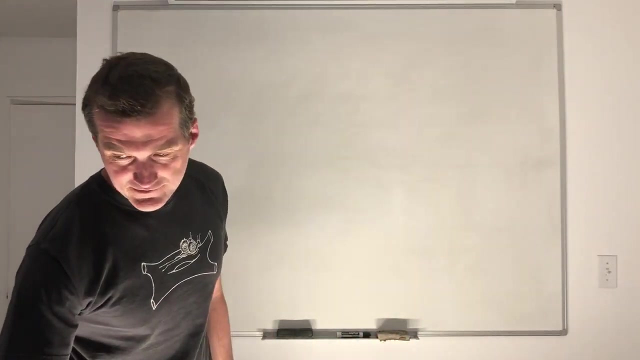 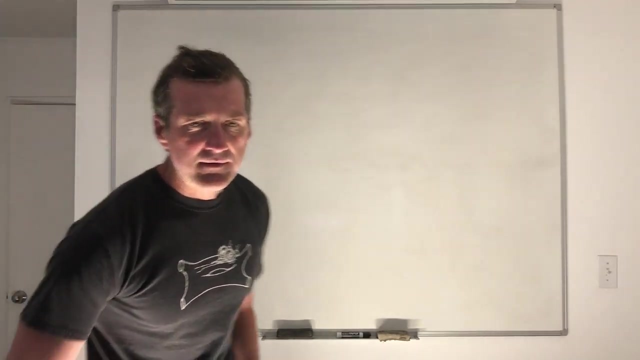 yeah, you need the Minecraft screen directly under the screen that's showing this, so that you can stare and just twitch your eyes. this is totally unacceptable. do I want you to do? I want you to do what? okay, yeah, anyway, I, I don't understand it at all, but that's okay. that's okay. so let me see how many. people on. well, this is going to be a lot of fun. I'm not going to be able to do a lot of stuff. I'm not going to be able to do a lot of stuff. I'm not going to be able to do a lot of stuff. 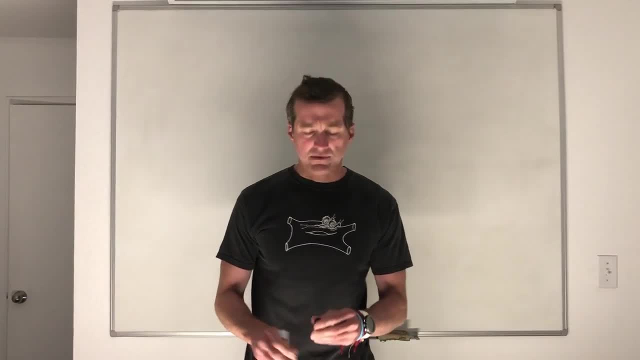 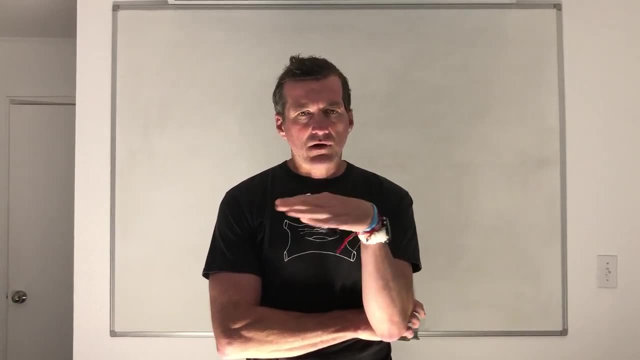 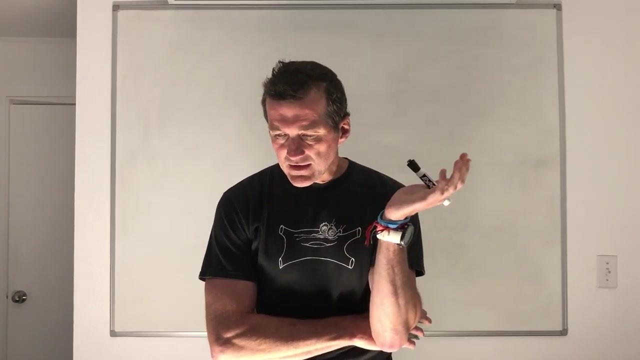 to be recorded so I can go ahead and get started and hopefully people that miss the lecture live can catch this on the recording. but I am gonna drop your lowest homework quiz grade. so I just wanted to let you know that, in case you you're looking at your grade hanging on one particularly bad homework quiz, that 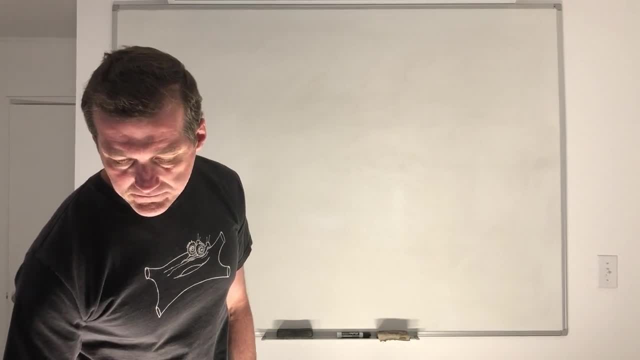 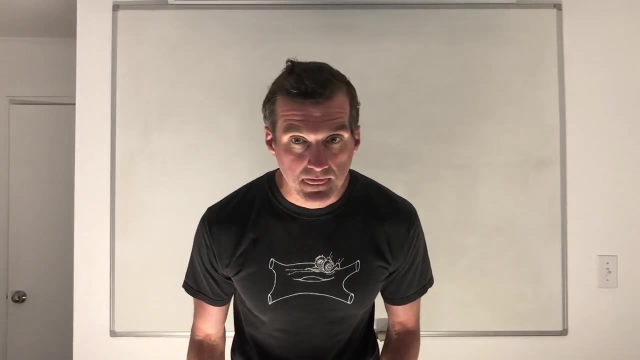 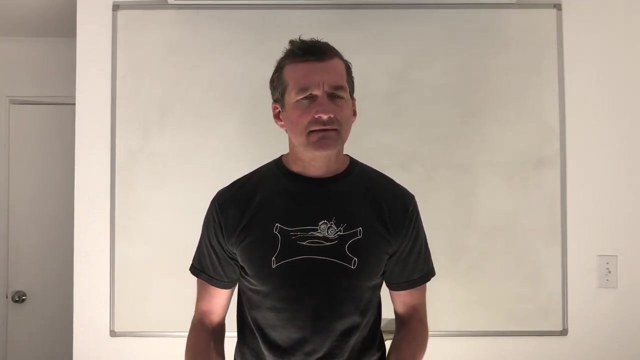 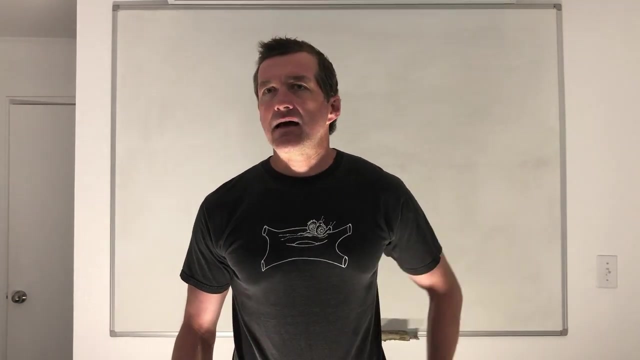 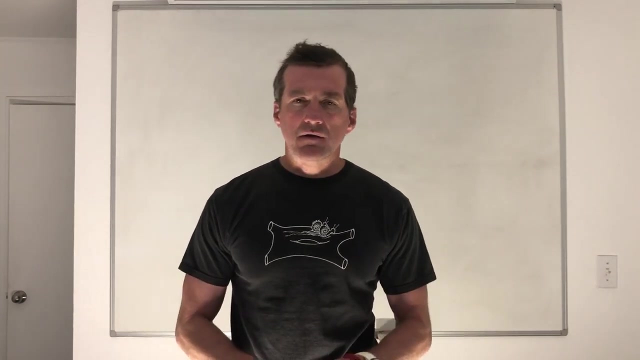 you, you took. so anyway, are there any questions that you guys have? before I get started say it again, did I say, wait, say it again? oh, I can also know the averages. so you know, posting grades when they're not when it, when they're not complete, is a little bit weird, right, because you've taken a. 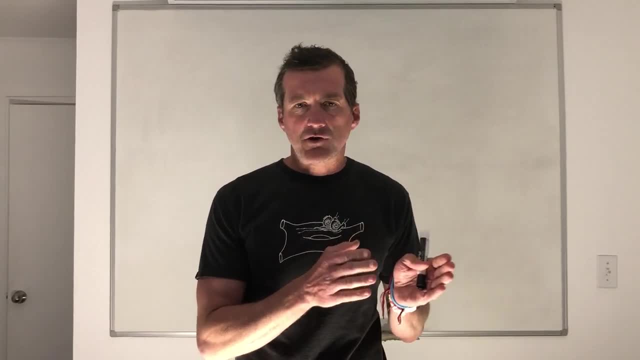 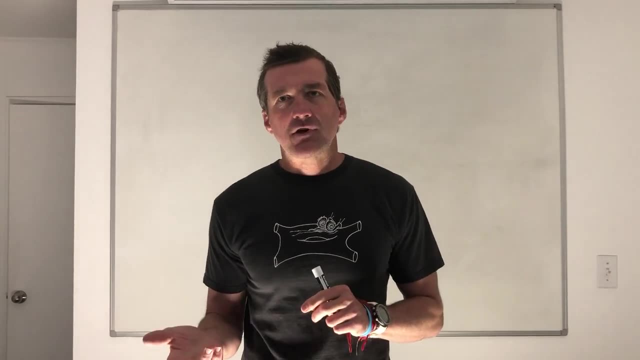 midterm, which you know. right now I'm not going to do my homework, so I'm going to represents a fair portion of your grade. and then you've taken some homework quizzes, so if I want to give you your grade in the class, should I give you the average of the homework quizzes counted? 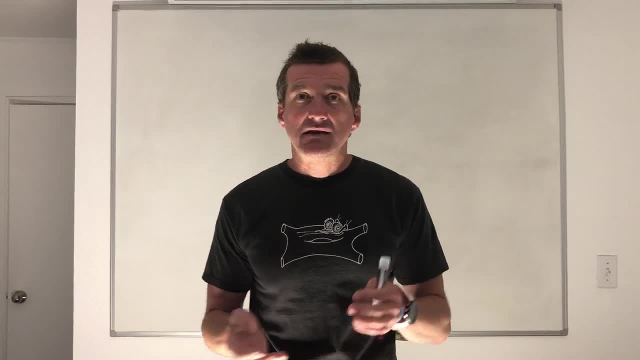 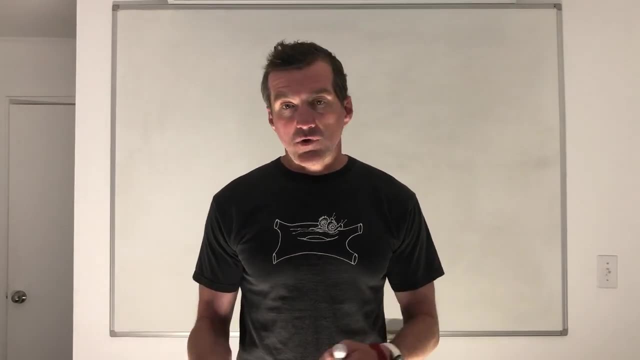 towards the overall percentage of homework quizzes are going to play in the class plus this test, but then the final's not there. so it's kind of weird. I mean I can just give you the grades you have on all your homework quizzes in your midterm, but in terms of putting that together to give you a 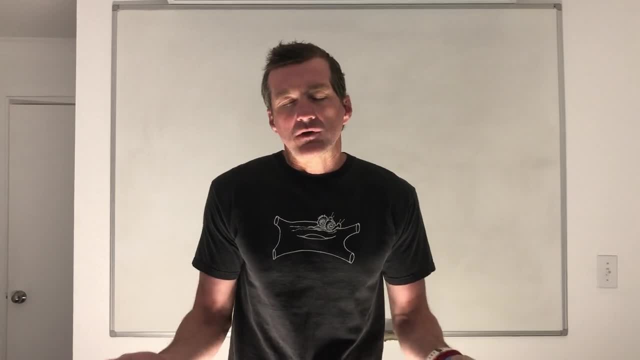 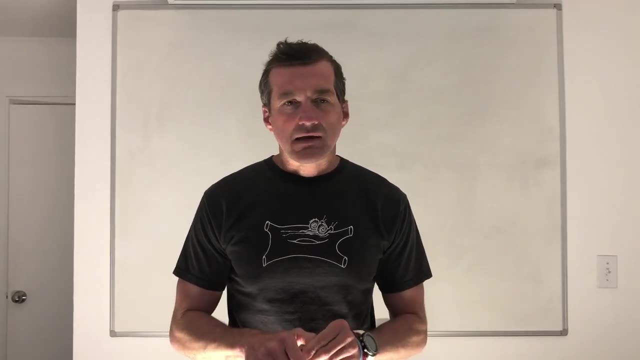 current standing grade. it's a kind of weird thing. I mean, people do it all the time anyway because we have to give midterm grades, but it's, it's kind of a weird exercise. so, like we do it in physics one, usually we take what they've got on their first two exams and we project out that they'll make. 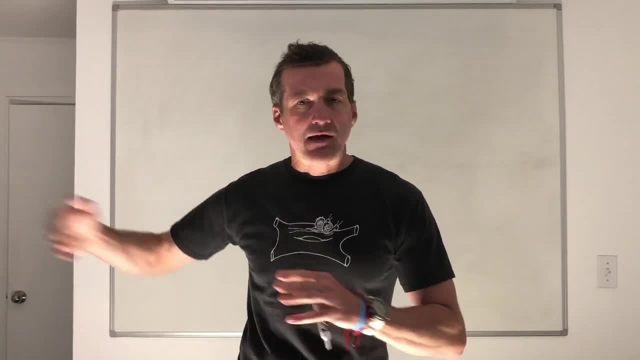 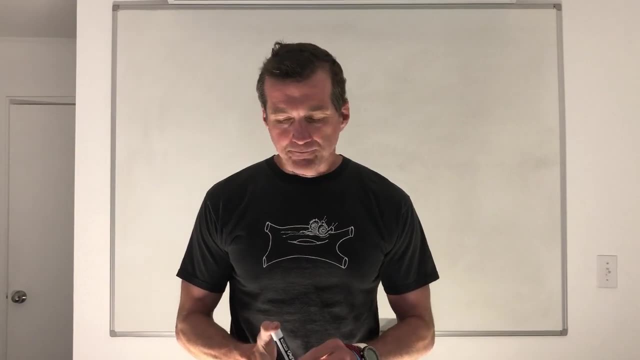 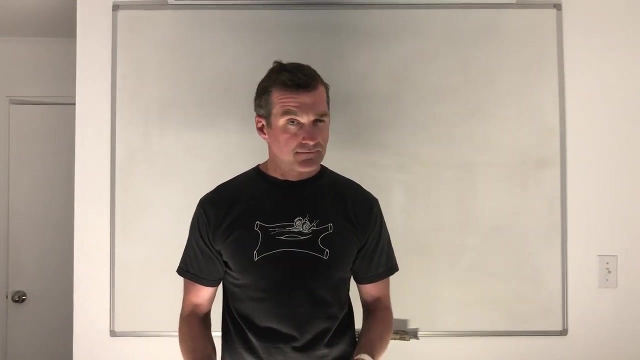 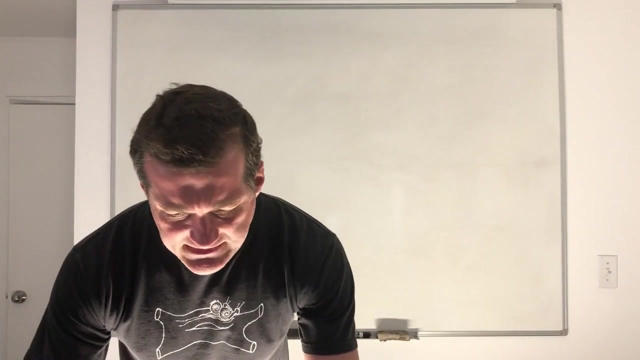 the same grades on their third and fourth exams. that way we can balance how much everything weighs together. does that make sense? yeah, okay, but I'll send something out to update you guys. other questions? no other questions? okay, all right, so let's, let's get started today. last time I'm pretty sure I ended. why it's really? 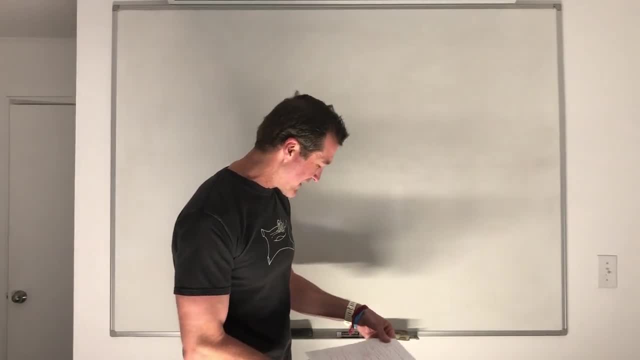 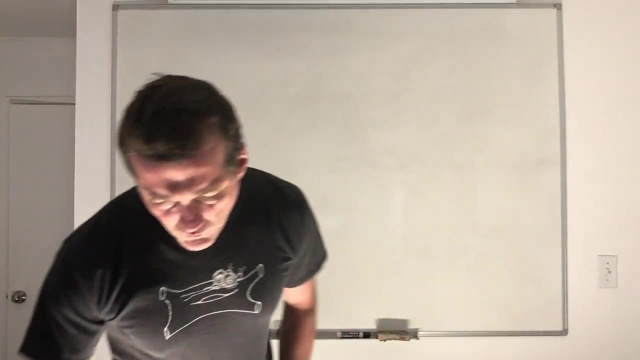 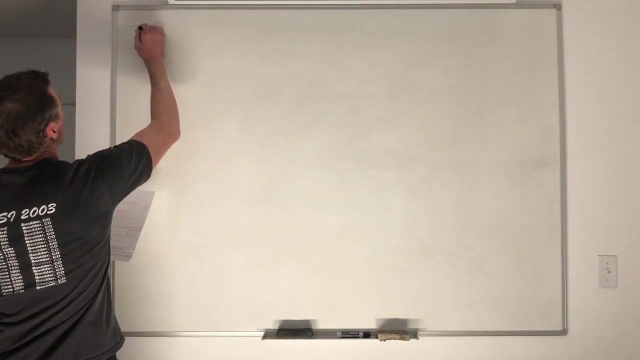 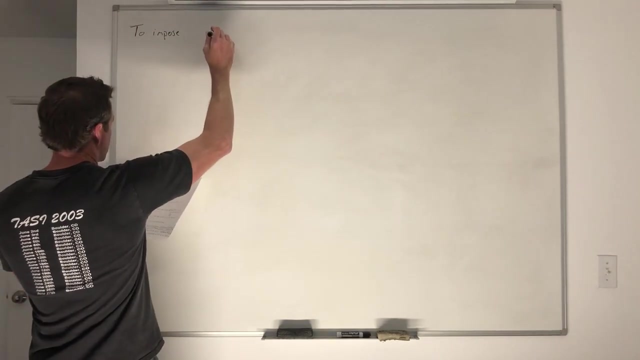 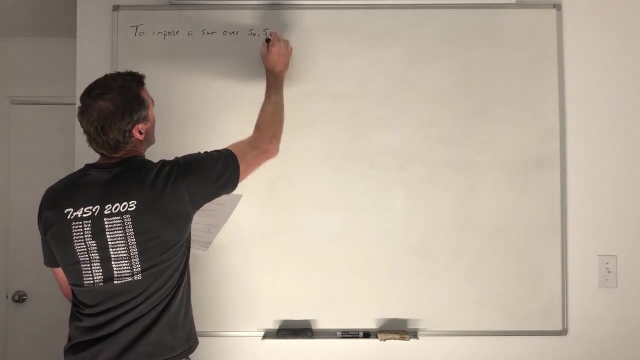 hard to read when my pages are backlit by this bright light. anyway, yeah, yeah, yeah. so last time we ended with this sort of rule, which is as follows: to impose a sum over the spin states a and b that are associated with the ends of a spinner sandwich. 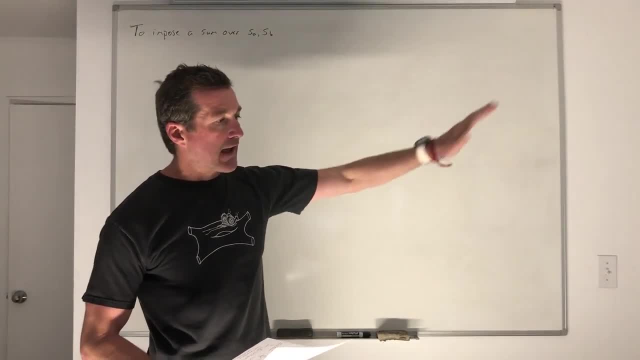 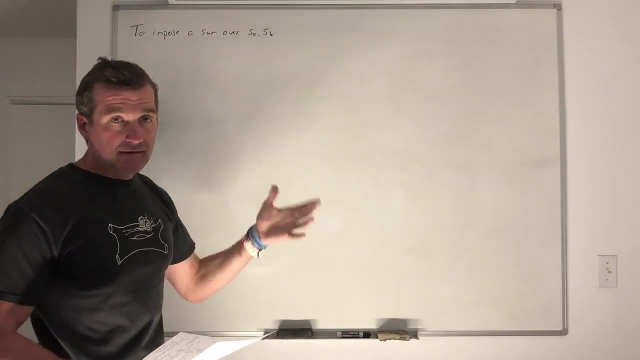 because remember, spinner sandwich, always you come in one outgoing or n going leg and then you leave on the other in going or outgoing leg, so you've always got to spins that area and that are sort of the boundaries of the spinner sandwich and you have to find something while you're setting up your 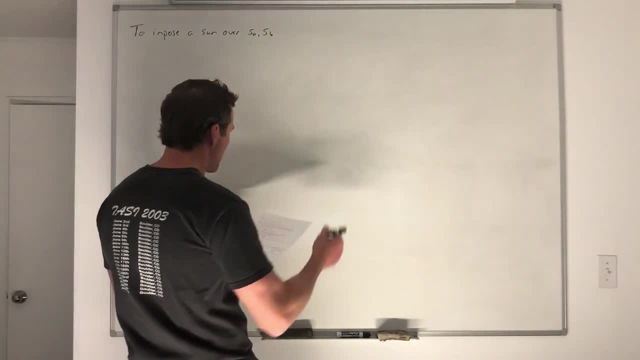 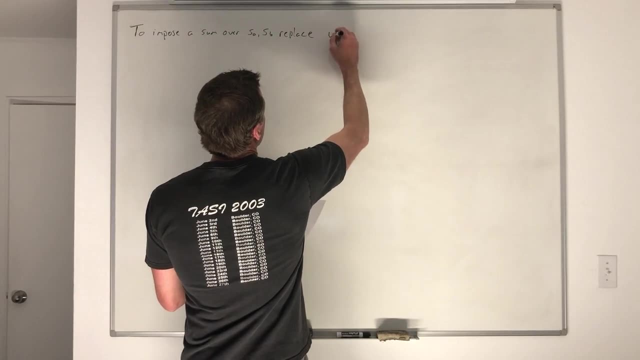 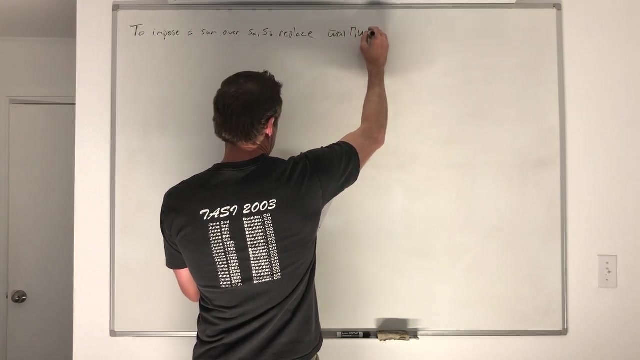 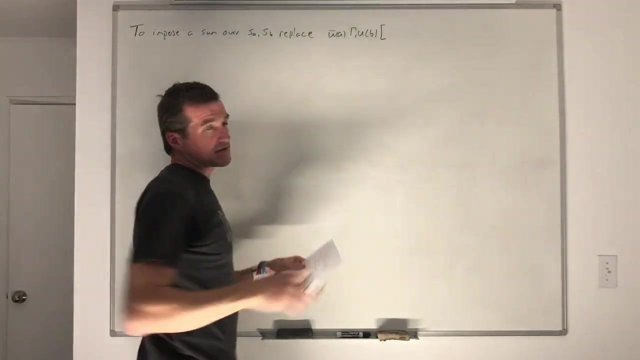 and those are the spins that you would want to sum over. then you replace the following: If you have a spinner sandwich of the form u bar a, gamma 1, u b and that's a spinner sandwich that goes into the transition magnitude m, 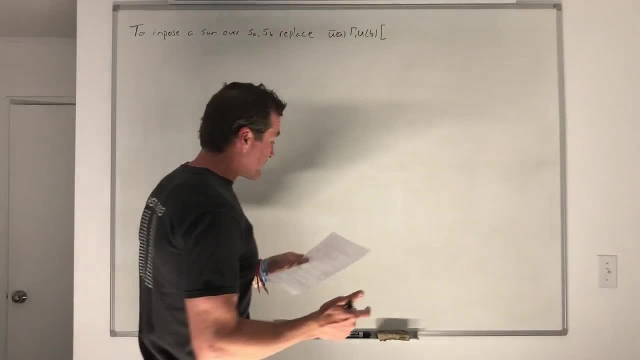 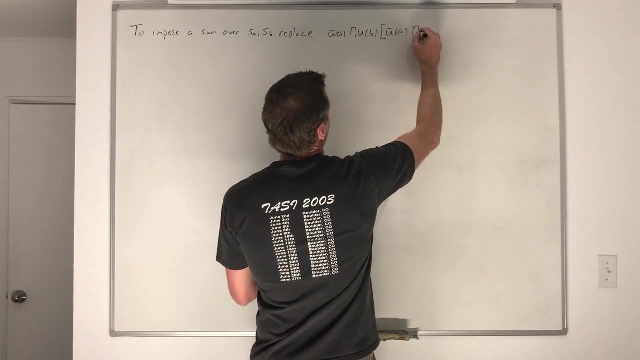 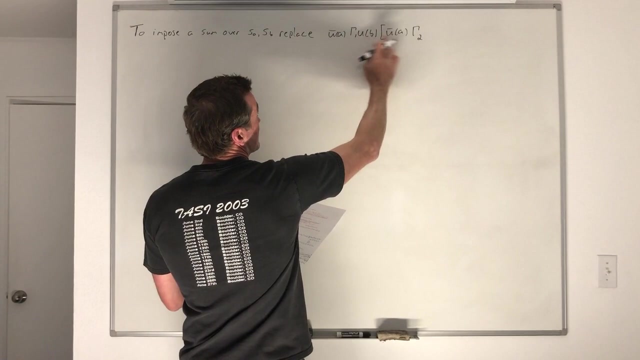 but remember, we're going to square m, so I'm going to go ahead and put another factor of this complex conjugated And again I'm going to put in a slightly different gamma or spinner matrix factor, just so that I can distinguish these two things. 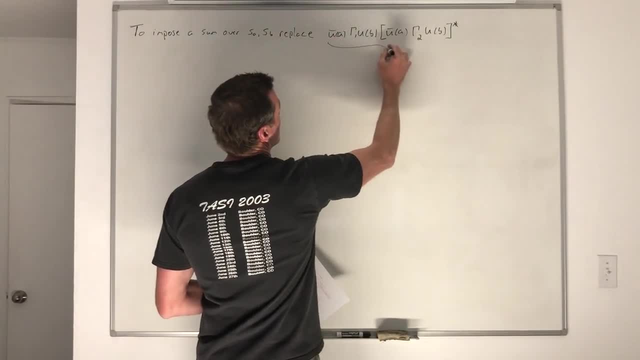 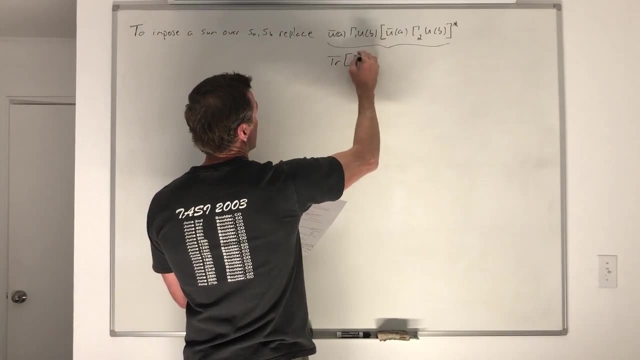 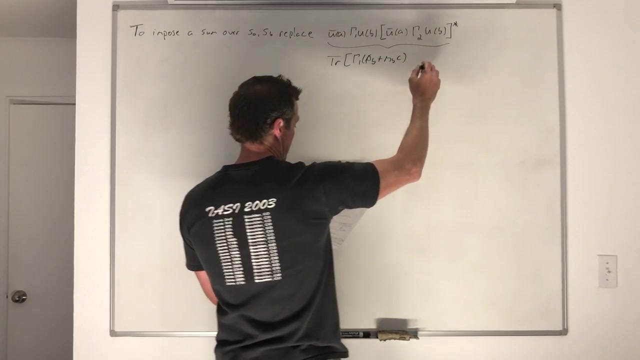 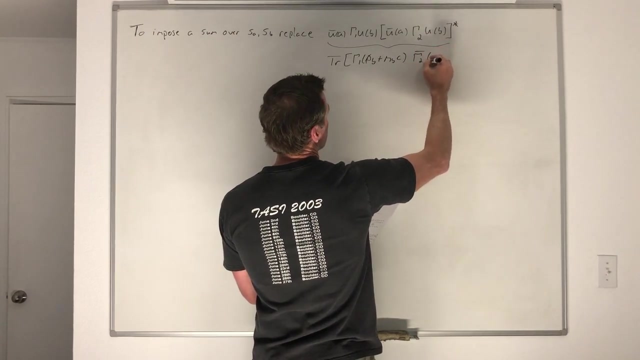 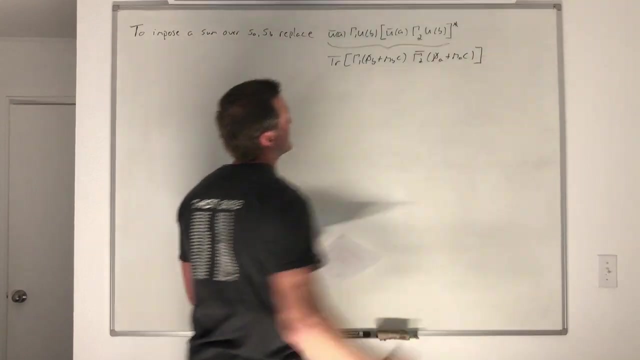 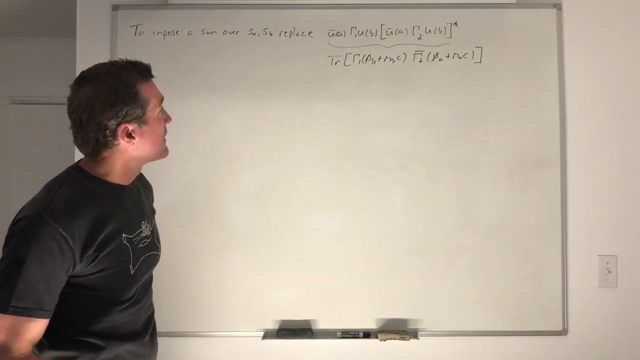 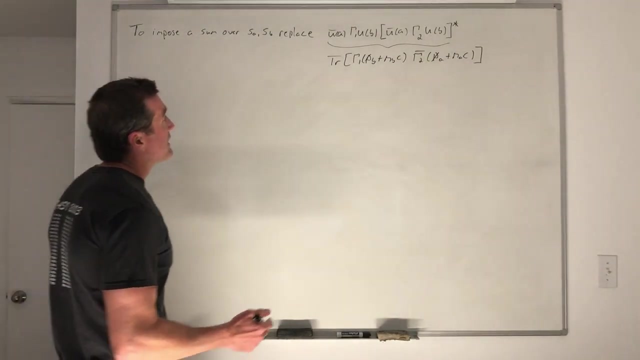 Okay, Then this gets replaced. It gets replaced by trace of gamma 1, pb slash plus mbc, gamma bar 2, yeah, not trace of p a plus m a c. Okay, Does that make sense Now? one additional thing that I should point out is: 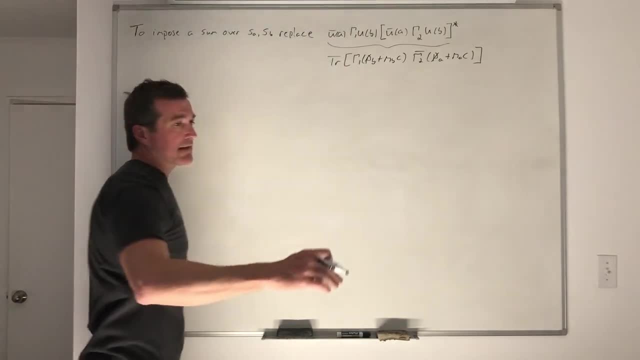 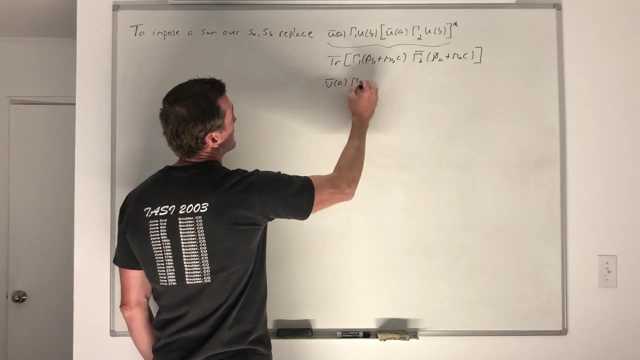 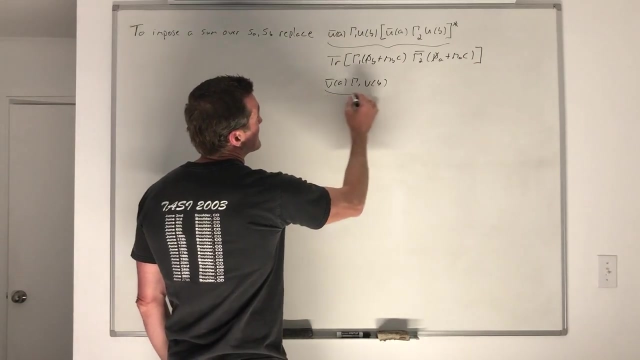 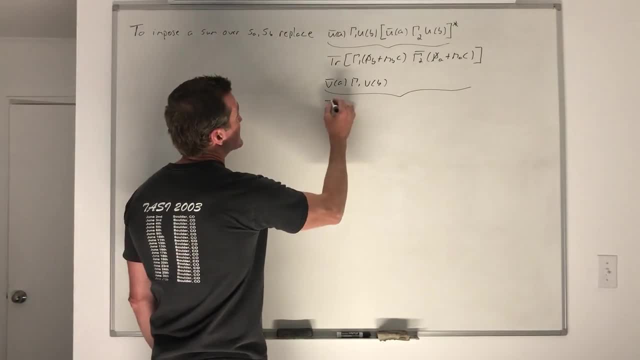 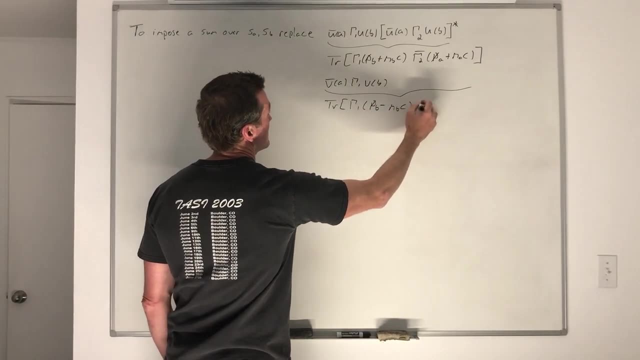 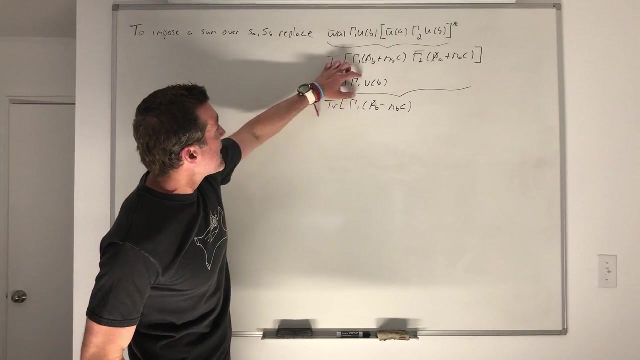 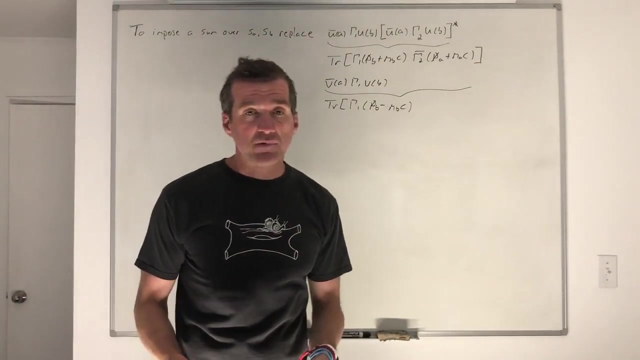 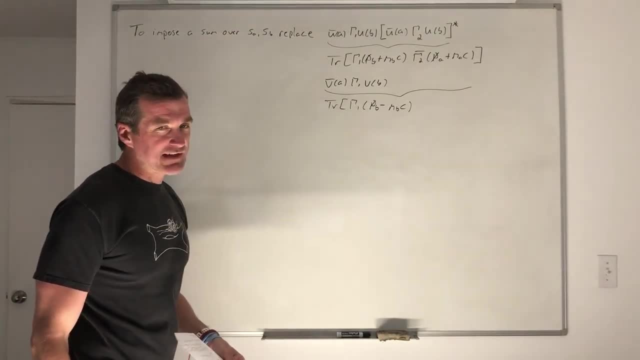 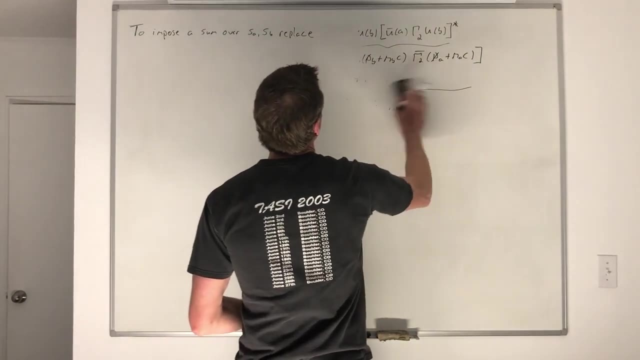 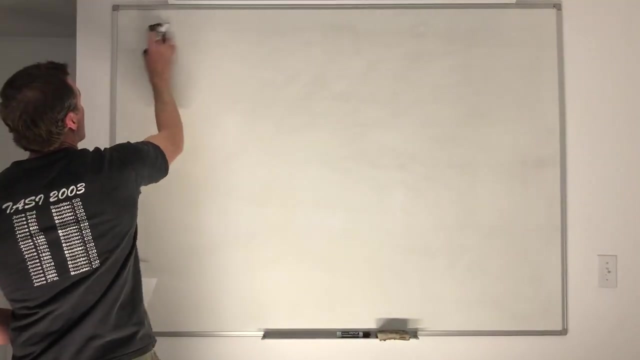 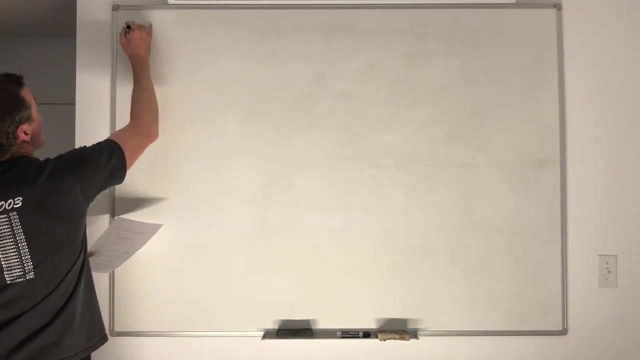 Okay, Okay, Okay, Okay. All right, We ready. It's about to get dirty, It's about to get so ugly. Okay, Here we go. Okay, So the process that I'm going to consider is: um and I. 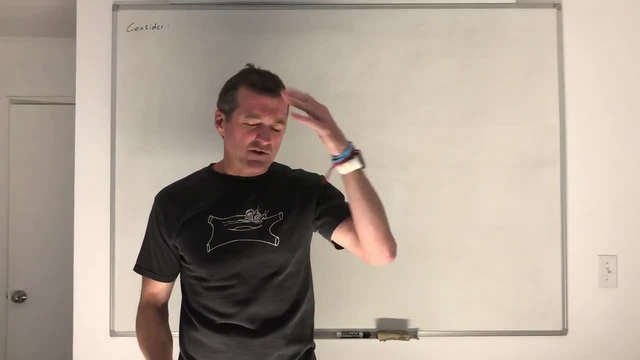 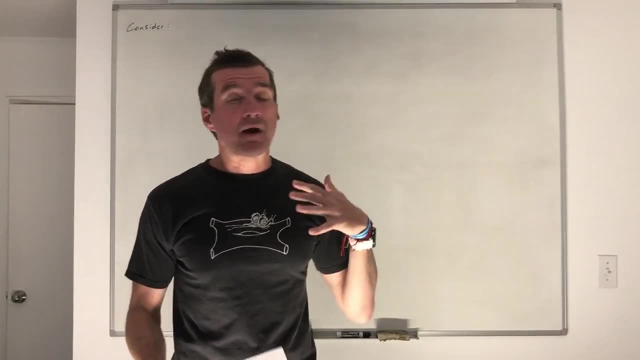 should say so today. what we're going to do is we're going to take this example that I'm about to give you. We're going to work through it again. I'm going to remind you. I'm going to basically go through exactly what I went through last time. I'm not going to go through the re-derivation of that. 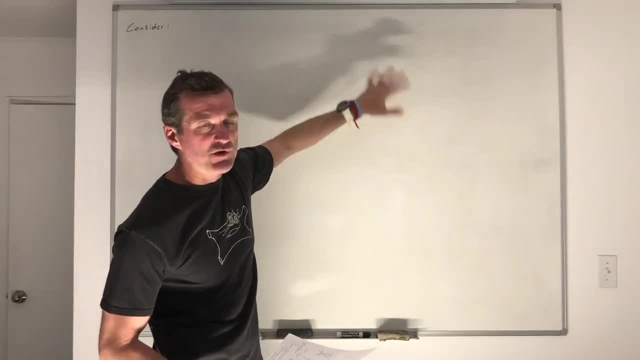 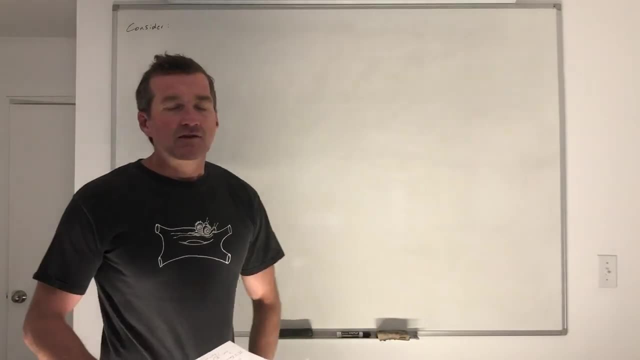 substitution. That's really special material for last time, because when you're working and doing calculations you just make that substitution. You don't go back and re-derive it every time. So I'm going to walk through the Feynman rules again, because that's what you use every time. 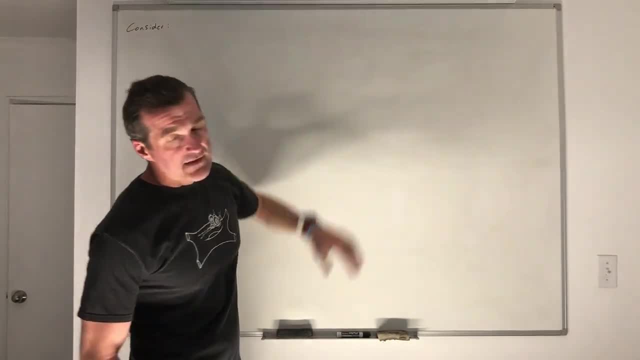 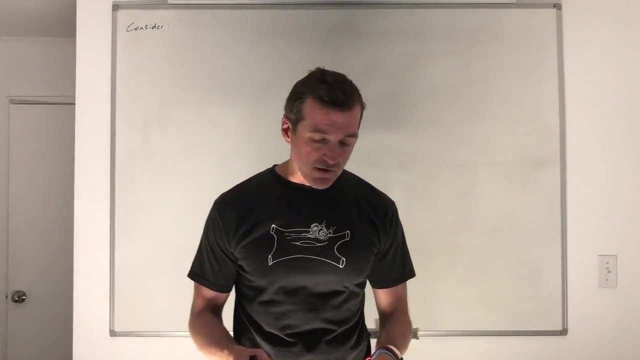 you're calculating amplitudes, We're going to make that substitution and then I'm going to finish up putting everything in terms of energy and momentum and getting rid of all of these spin matrices and so forth, And then what we're going to do is we're going to take some limits of it and we're going 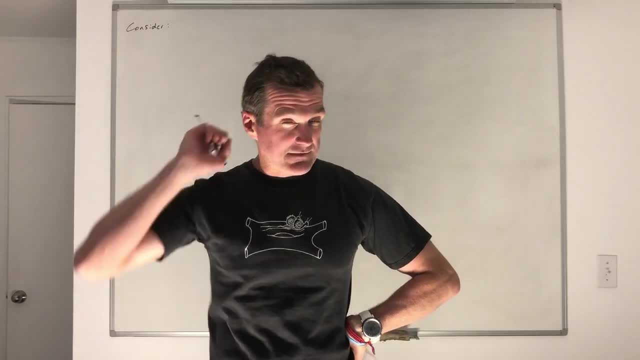 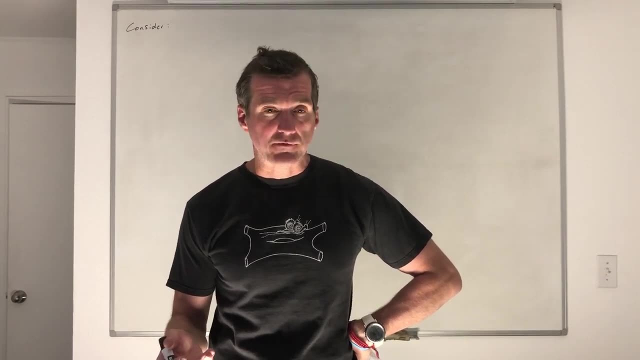 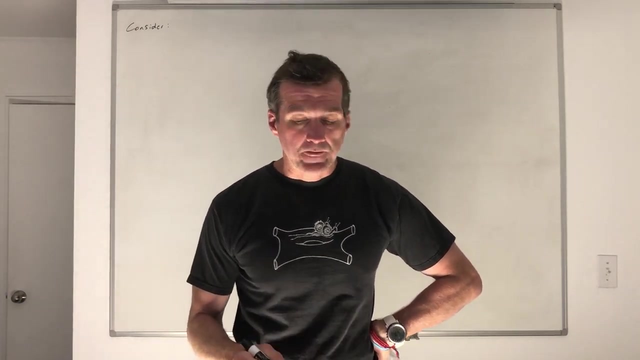 to eventually arrive at what should be at least familiar in name scattering equations. Okay, how many of you have ever heard of the Rutherford formula? Raise your hand. Okay, we're going to derive the Rutherford formula today. Okay, So and 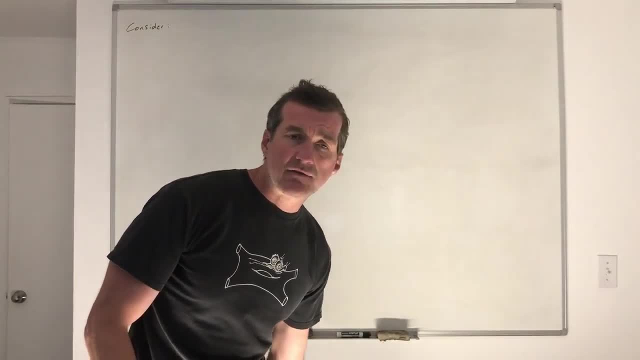 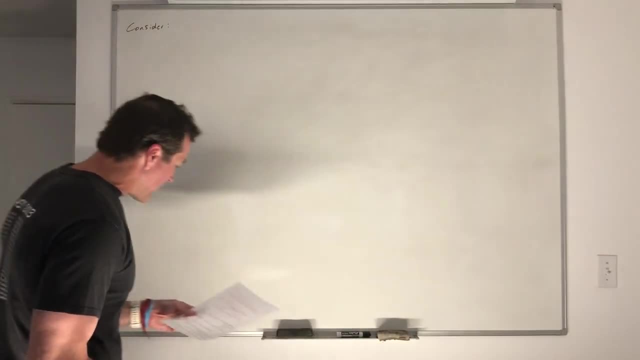 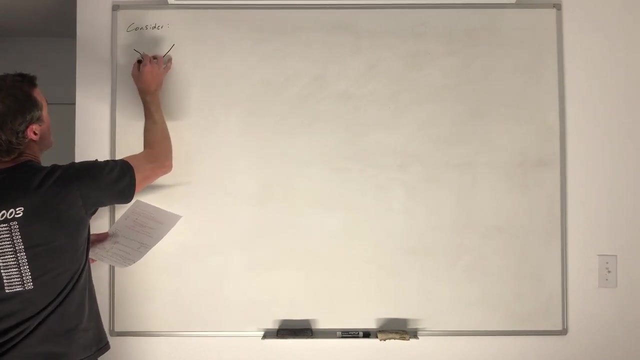 then next time we're basically going to take this story and we're going to translate it into QCD and do quantum chromodynamics on quarks. Okay, so here's the process we're going to consider today. So we're going to have an electron come in. 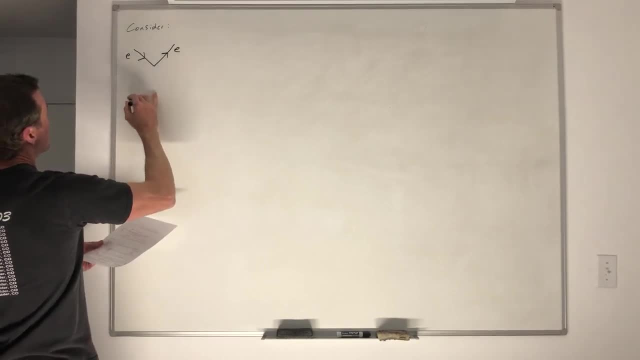 And we're going to have a muon go out. Hold on, I got to grab something. really quick Shoot. where are they? I got to find them. Hold on, Over there and here. Nice drawing here Over in the red rack. 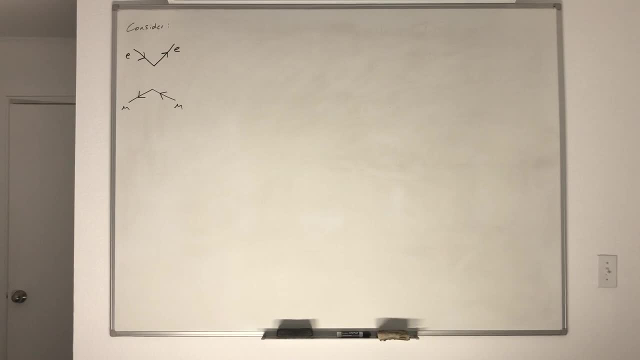 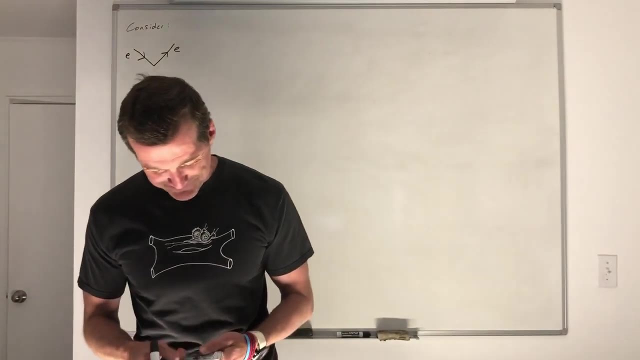 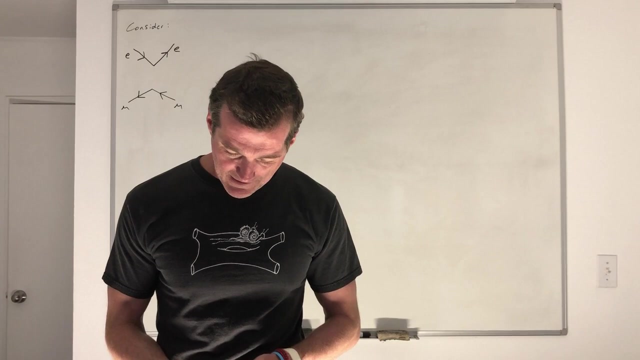 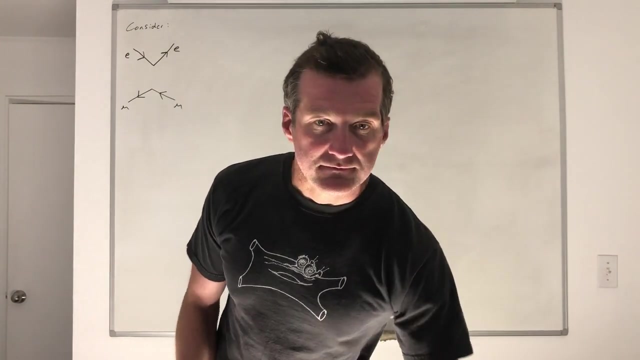 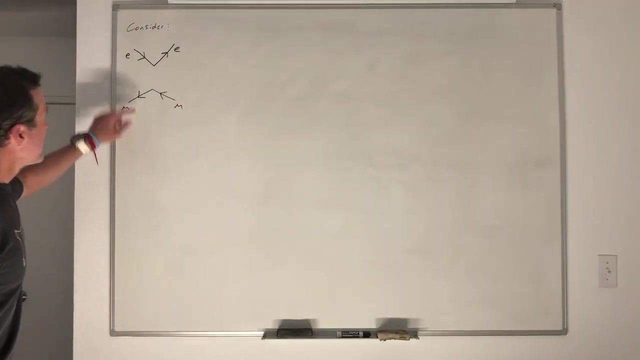 I found them. uh, I am picking off the top. Yeah, Okay, I'll pick up stuff. Okay, Gabriel, Gabriel here. Yeah, there's Gabriel. So, Gabriel, is this a collision between an electron and a muon? 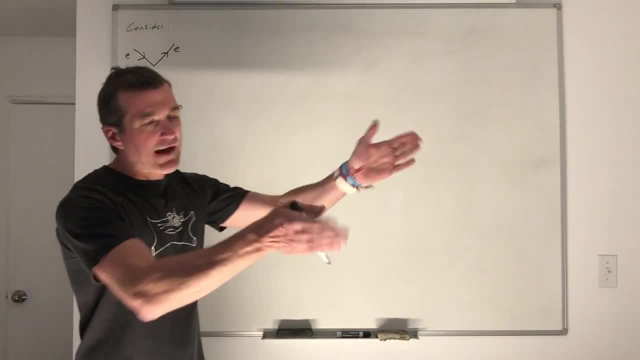 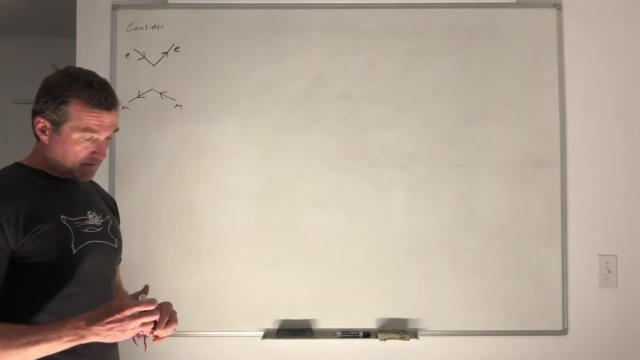 What do you mean by collision? Well, I mean- sorry, it's an interaction- An electron and a muon come in and an electron and a muon go out. Is that what this is? Not currently? Say it again: Not currently. 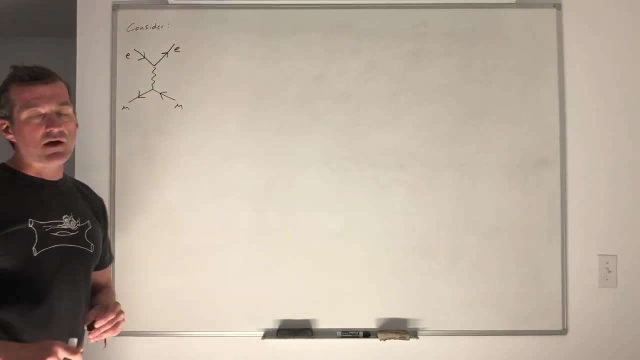 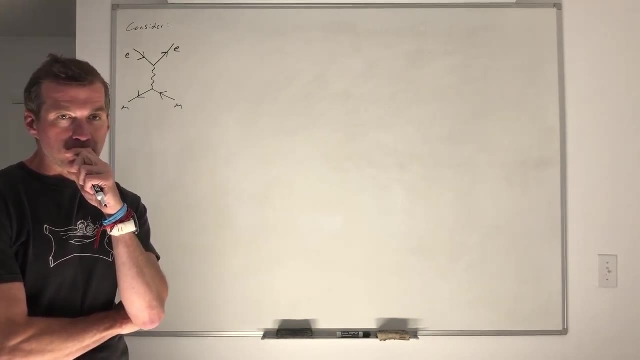 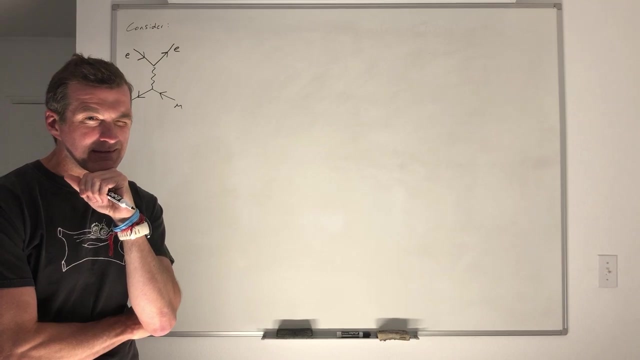 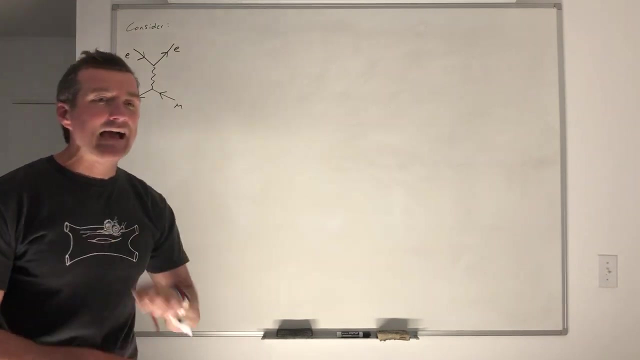 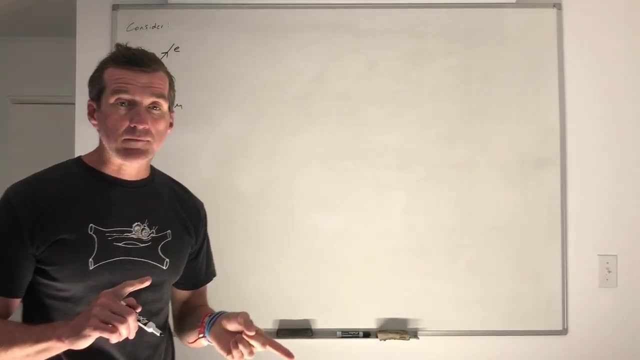 Well, okay, I'll finish with the exchange of photon. There we go, sure, No What, Anybody want to help him? Sarah, I think it looks like it's like an electron and then the antiparticle. Exactly, Remember, the direction of the arrows that you put on the lines tells you whether it's a particle or an antiparticle. 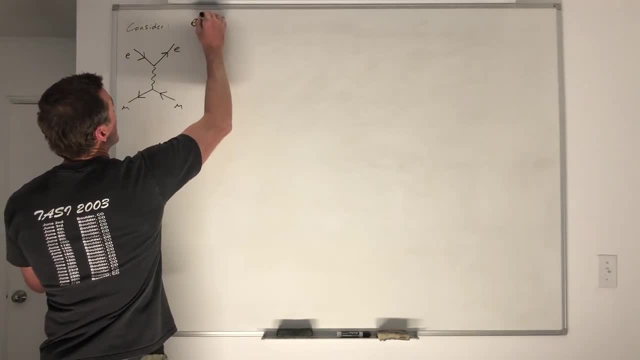 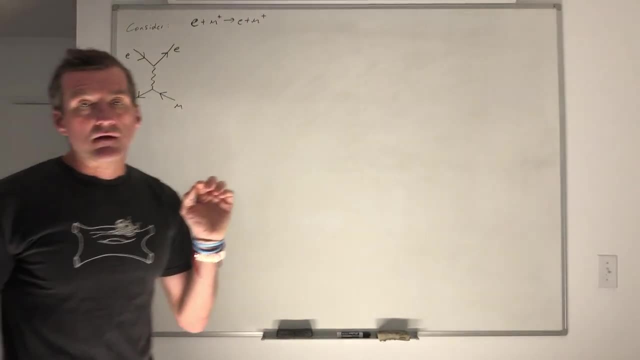 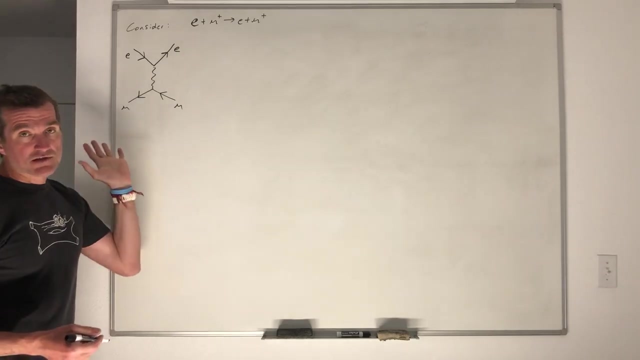 So technically this is an E, E Plus a mu plus, going to an E plus a mu plus. Okay, Normally a muon particle would have a negative charge, just like the electron, but this is the antimuon, so it's going to have a positive charge. 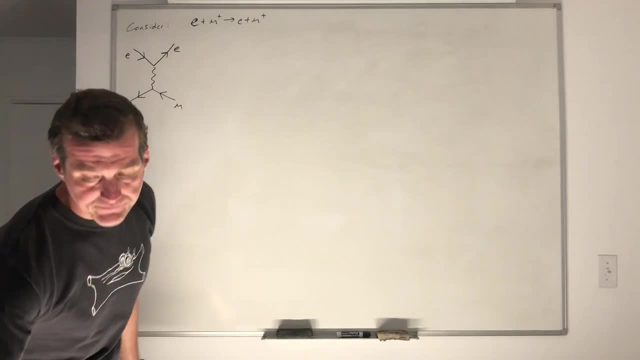 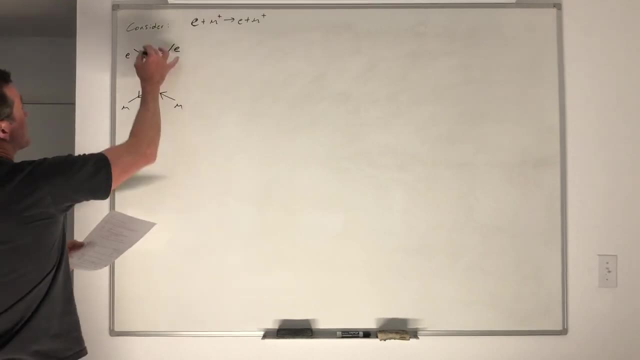 And we usually denote that by a plus. Okay, So let's go ahead and get our diagram suited up. So I'm going to pick momenta for all of them, Momenta for all of these, And I hope you all realize you're going to be able to follow everything I'm about to do, because I'm really repeating the steps that I taught you last time. 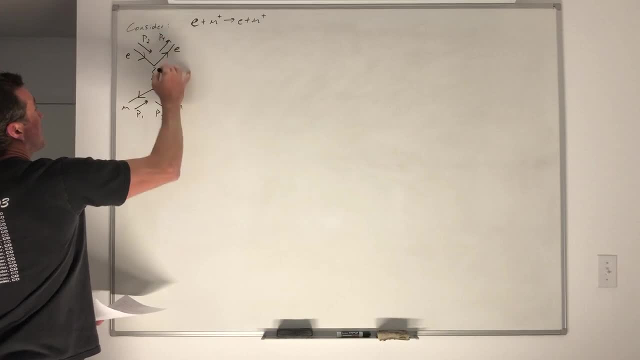 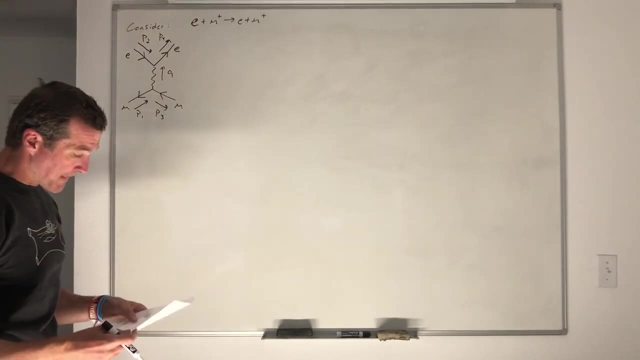 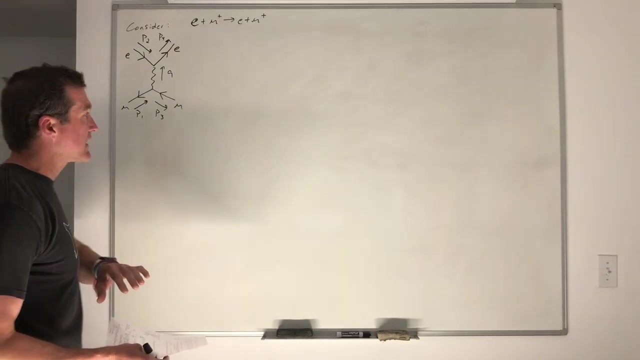 So p1, p3, p2, p4, and then we'll have the photon momentum going up with a value of q. Okay, And now let's follow the spinner sandwich construction rule. Okay, So if we want to build a spinner sandwich, you might, you know, harken back to the Feynman rules for QED that I gave you. 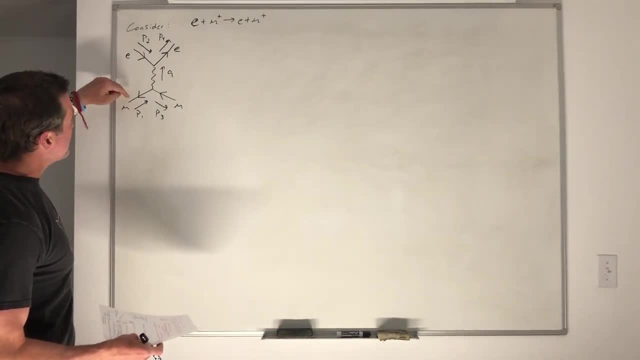 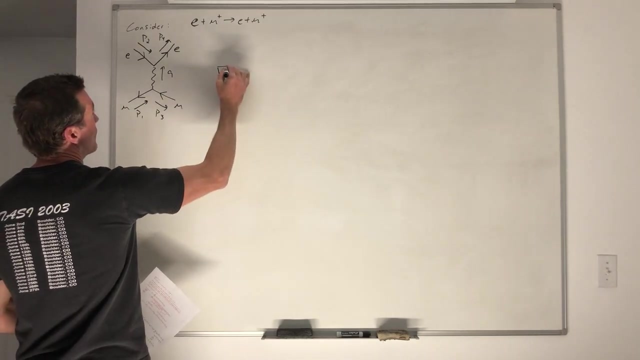 But if you're following antiparticles, you actually want to come from the ingoing one first. So we write down a factor for the incoming one, And the factor for antiparticles is v, So we have v. So we have v of 1, because that momentum for this incoming anti-muon is p1.. 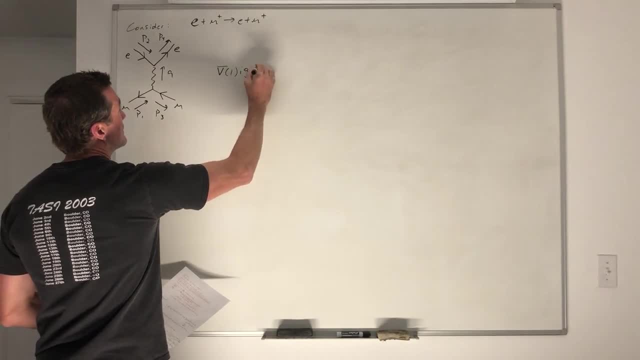 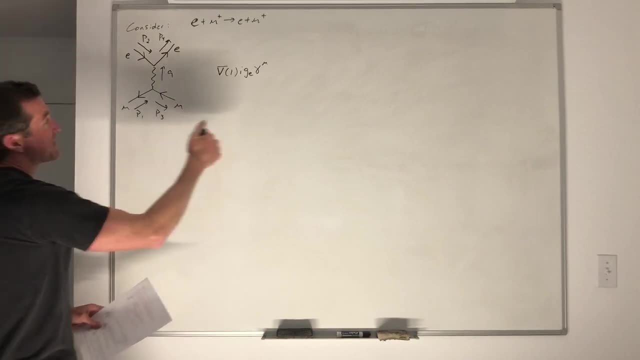 And then we hit a vertex, And then we go out on this anti-muon line which has momentum 3.. Okay, Now that might make a lot of sense, But remember, when you're now going to do a particle line, when you do a particle line, you actually start with the outgoing particle and then the vertex, and then the incoming particle. 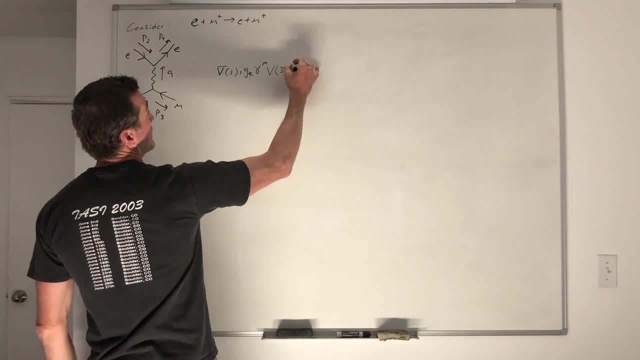 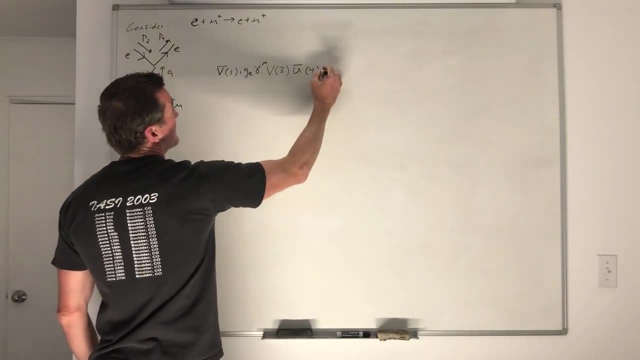 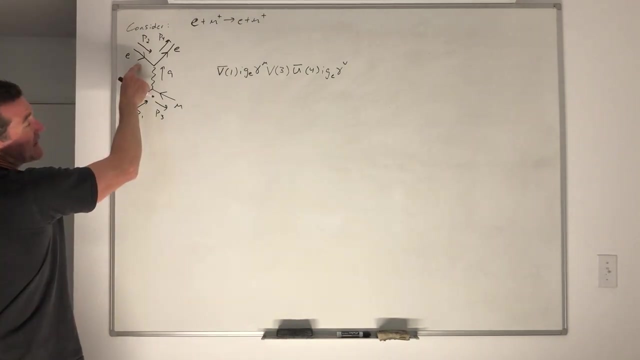 And it's the outgoing particle that gets the u-bar. Okay, So u-bar of 4 and then a vertex factor. Make sure we give it a new index And then we get a u-factor for the incoming particle, So we have a u2 factor. 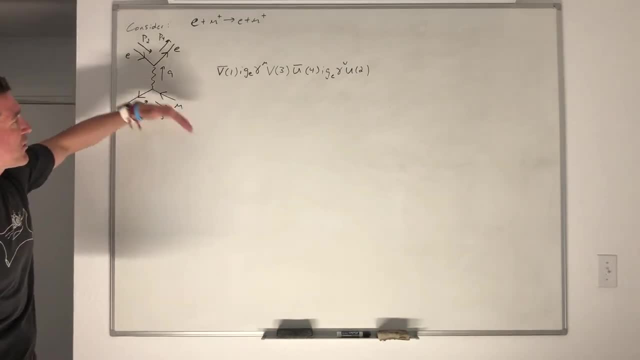 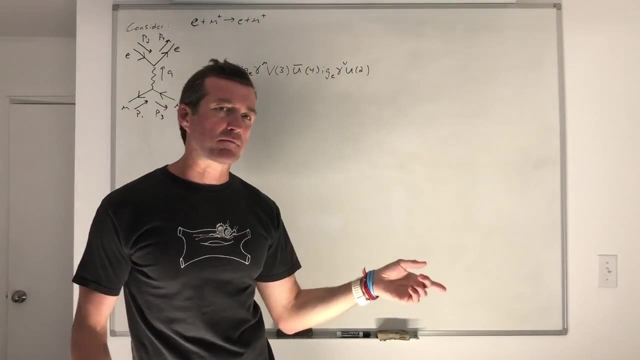 Okay, So you go with the flow if it's an antiparticle. You go against the flow if it's a particle, Which is kind of interesting, because usually we think of antiparticles as going backwards in time and particles going forward in time. 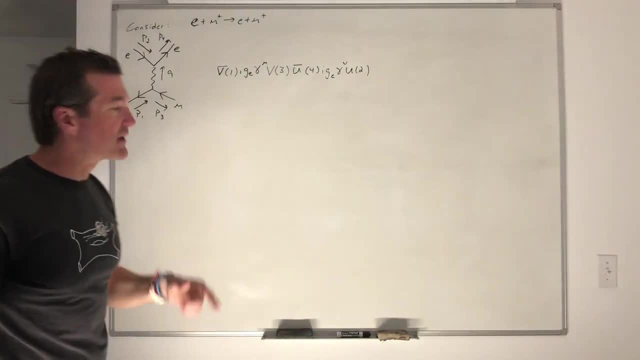 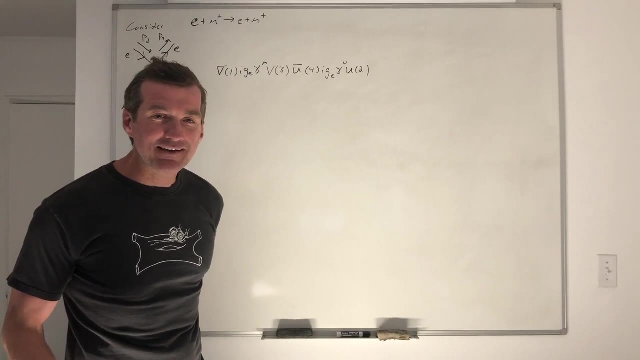 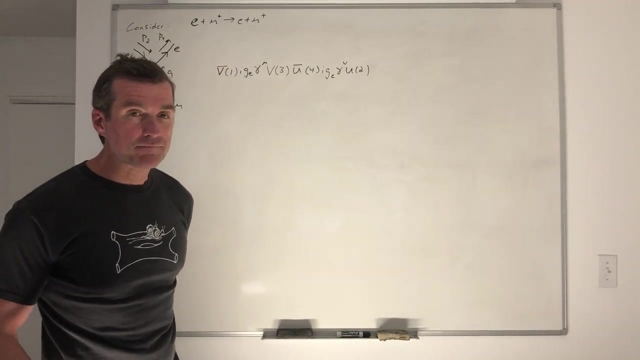 But this is the one-time retracing The making the spinner sandwich thing. you've got to reverse the trace if you're on a particle versus an antiparticle line, Got it You? okay, Avery, Yeah, So if you're doing a particle line, you go from the outgoing one first to the incoming. 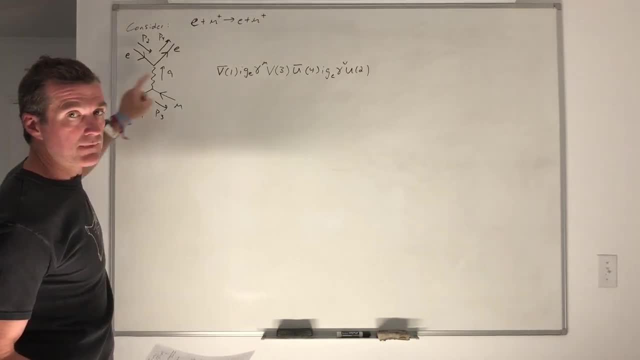 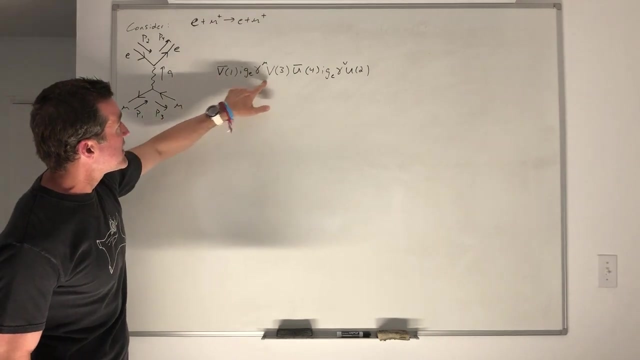 And then, if you do an antiparticle, you go from the leftmost all the way to the… Rightmost. Yeah, And all that that's really doing in this expression is whether the incoming or outgoing momentum is associated with the… Spinner factor or the conjugate spinner factor. 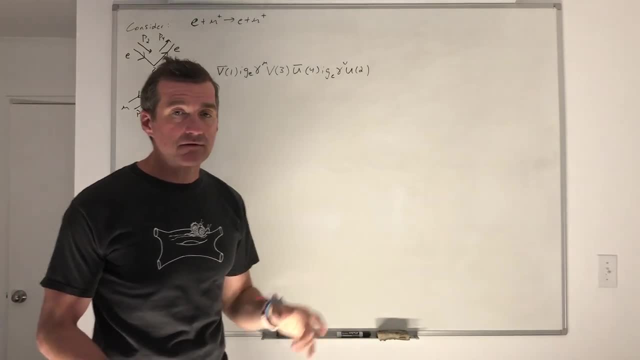 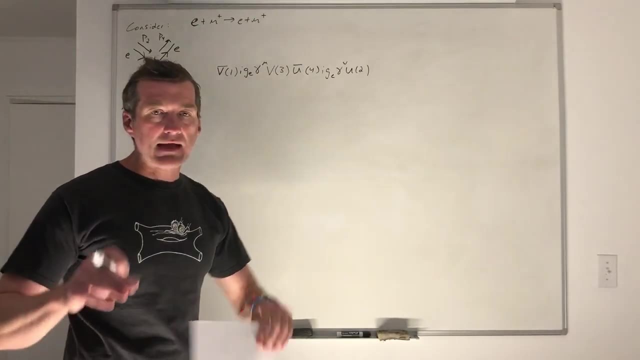 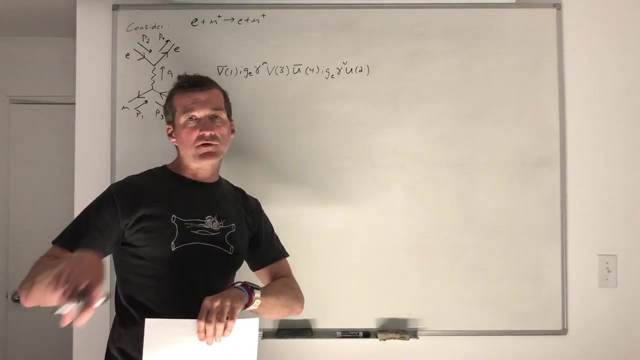 So it does make a difference which way you trace it. Okay, But again, if you go back to when I laid out the Feynman rules for QED, I drew that bubble And I had the outgoing particle, the outgoing antiparticle, the outgoing photon, the incoming particle, the incoming antiparticle and the incoming photon. 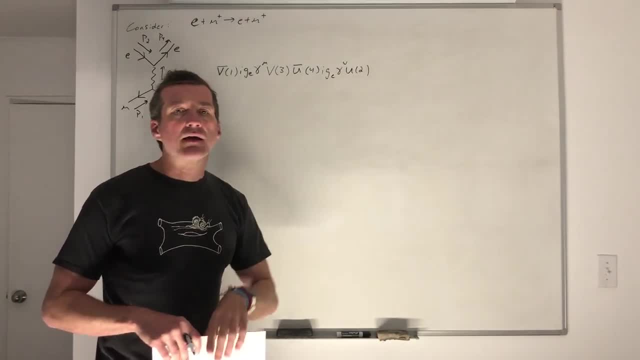 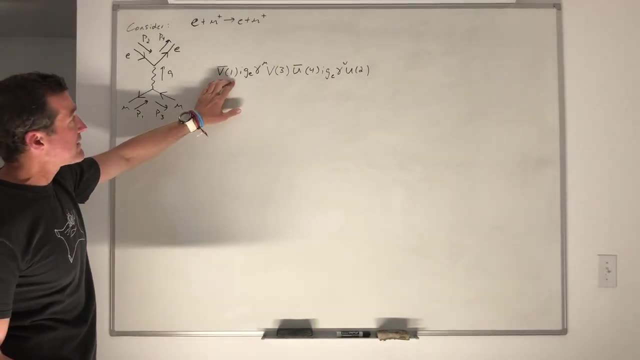 And I wrote the various u, u, bar, v, v bar. So if you just look at that bubble, that tells you what you have to write, Because you always have to start with the adjoint spinner and end with the spinner. 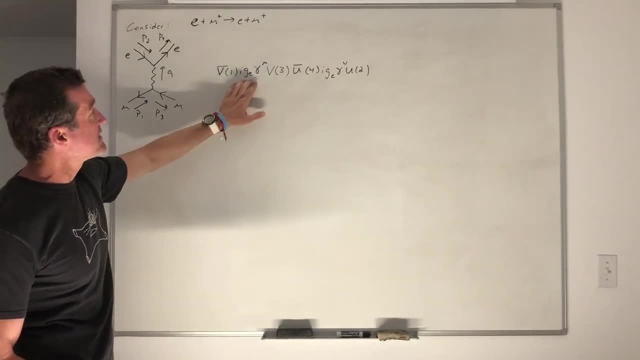 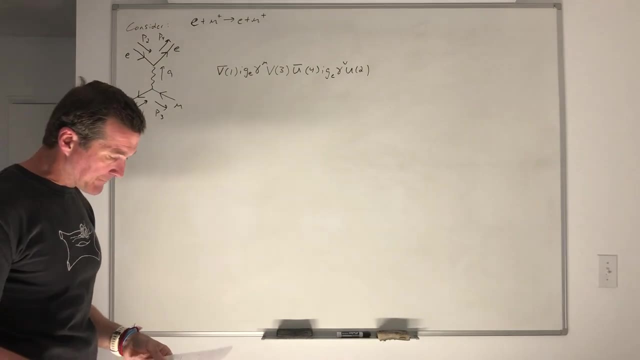 Okay, I mean, imagine this is a row, this is a column, this is a matrix, and that's what you need in order to make a number. So, regarding the squiggly… Which one do we do first? squiggly prime or squiggly star or squiggly not star? 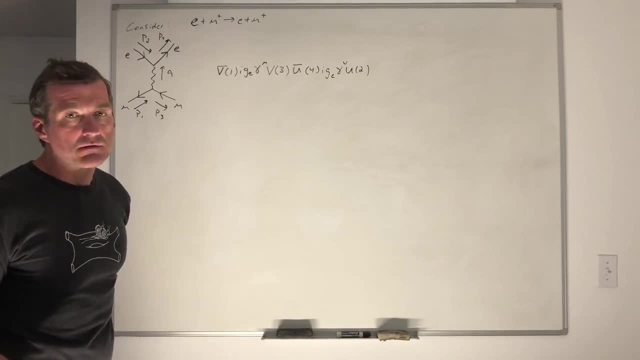 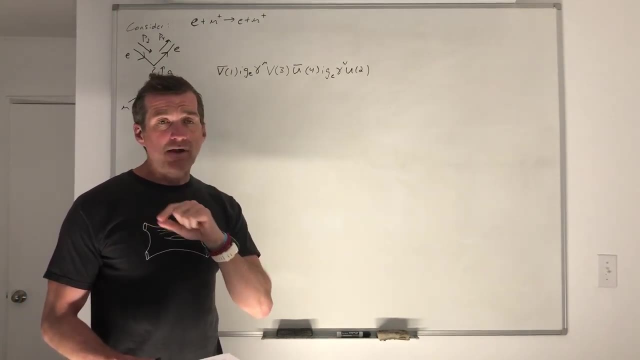 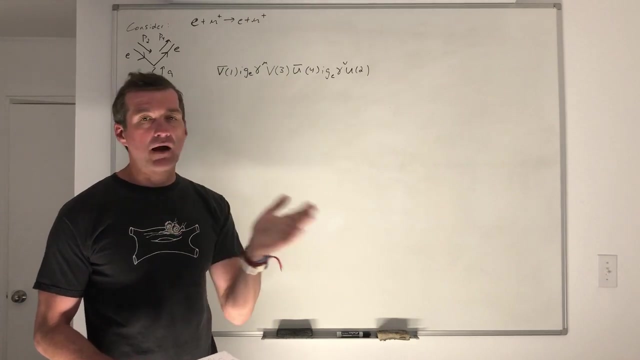 That one doesn't matter so much. That one doesn't matter. No, So the ordering of the squiggles… So the squiggles are the external photon lines And they're not spinners at all. So we're going to use index notation to talk about. you know how you combine and you know things. 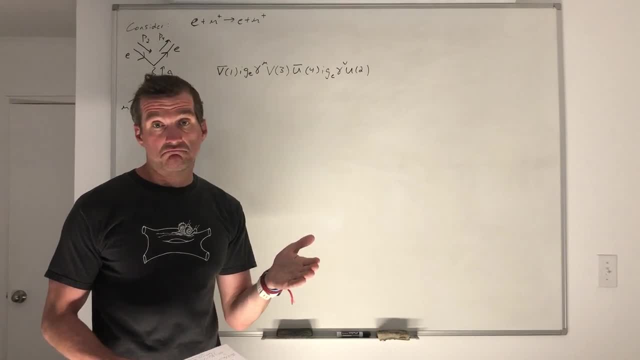 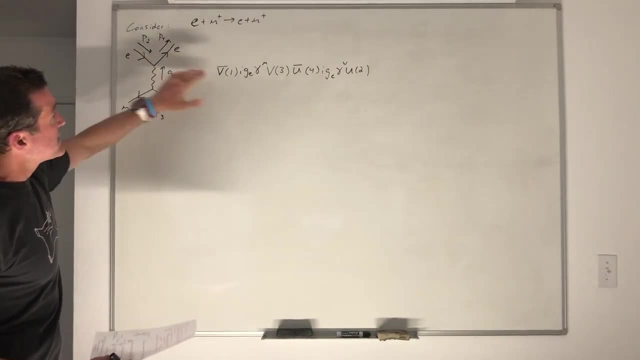 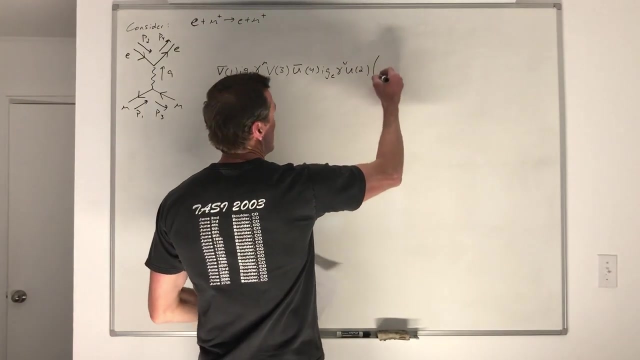 We only need to worry about getting the order correct. if we're doing spinners, Okay, Okay, Perfect, All right. So we've got our spinner sandwiches. We're going to have to write down a propagator for our internal photon. 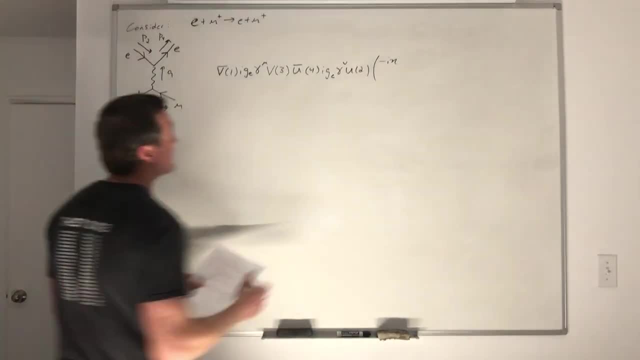 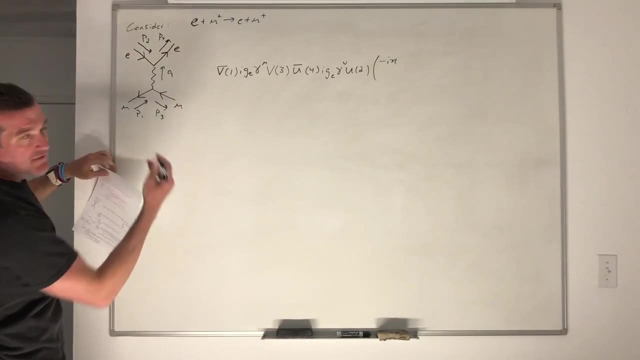 So we know that this gives us a factor of minus i times eta, And eta is the metric, And the two lower indices on the metric are associated with… And we might as well do this, And this is going to be helpful later on. 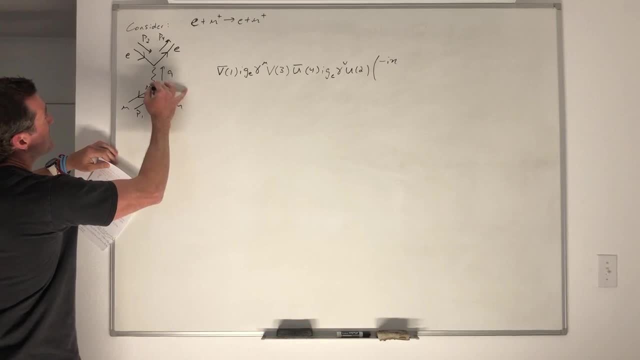 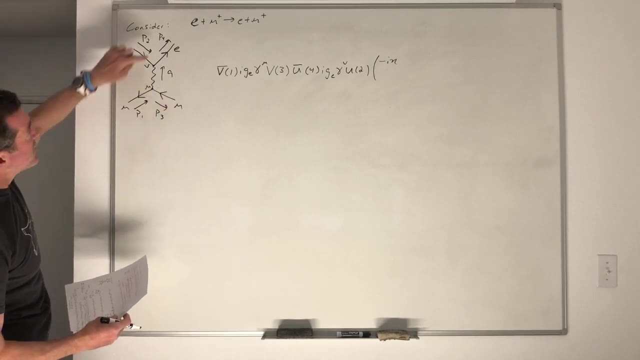 I might as well go ahead and label this the mu vertex and this the nu vertex, Because when I built this spinner sandwich, I used gamma mu. I built this when I used gamma nu, So the propagator that I'm putting in for the photon has a mu and nu index. 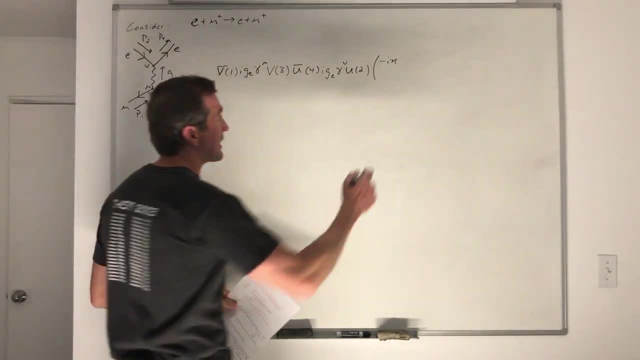 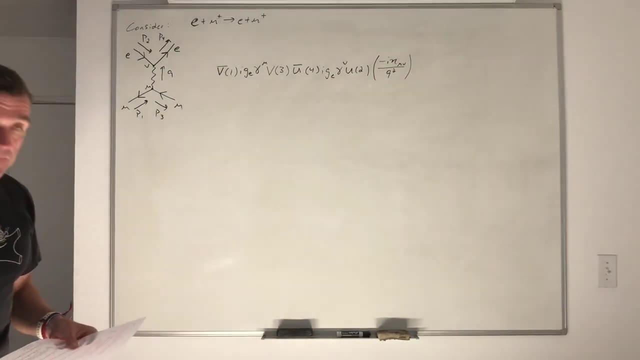 This is going to be more challenging and a more complicated example I'm going to work out later. So, mu nu over the momentum squared of the photon. Okay, And then the next steps are ones that we should be somewhat familiar with. We have to put in the delta functions which conserve momentum at the two vertices. 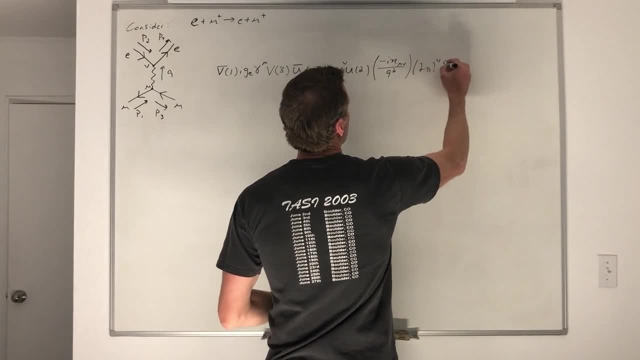 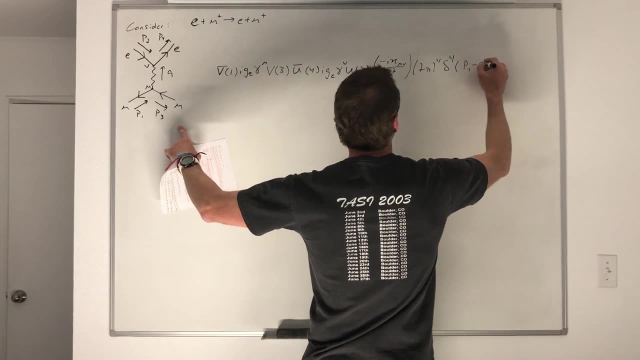 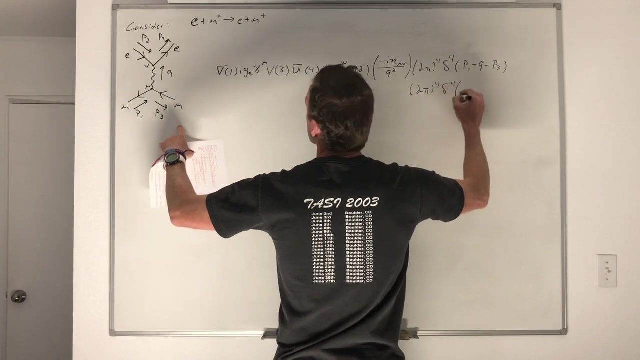 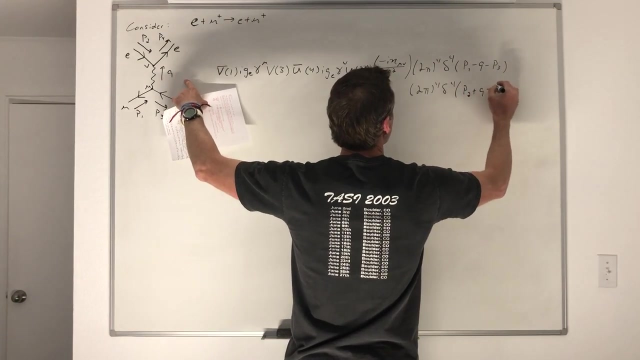 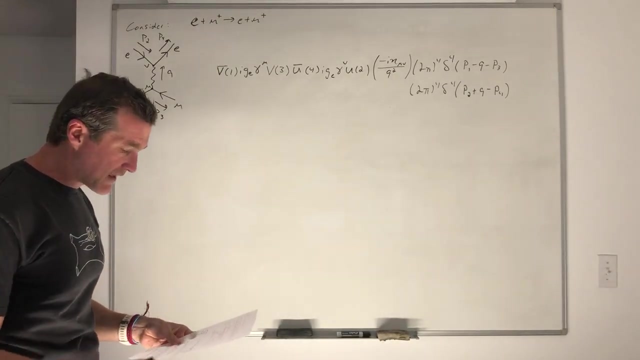 So we're going to have 2 pi to the 4, delta 4.. And then we can do p1 minus q minus p3. And then we're going to have p2 plus q minus p4.. Okay, So that's the momentum conservation delta functions. 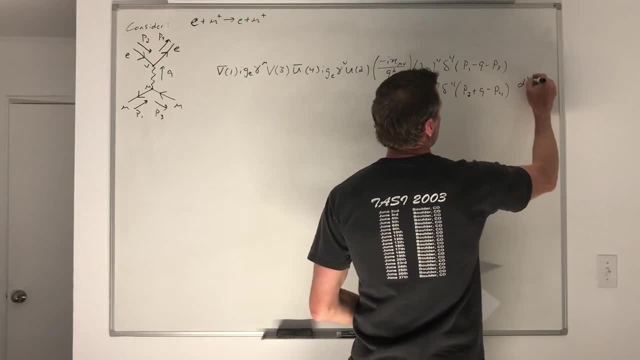 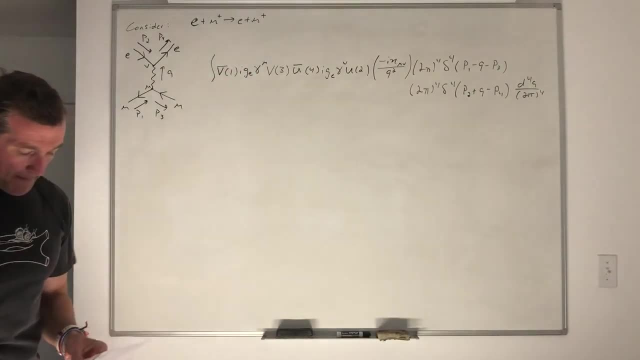 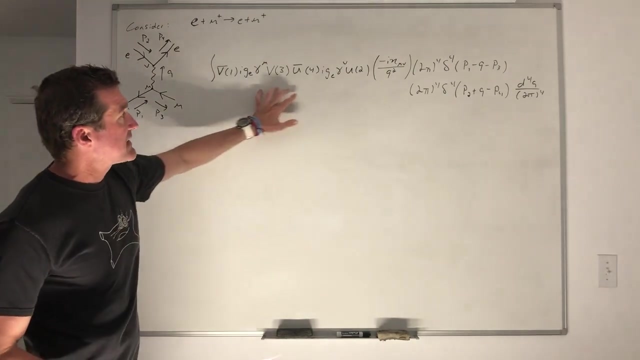 And then we have to integrate over the internal momentum d4q, over 2 pi to the 4. And then we have one integral sign. Okay, So again, the only new ingredient here are these spinner sandwiches and this different kind of propagator for the photon. 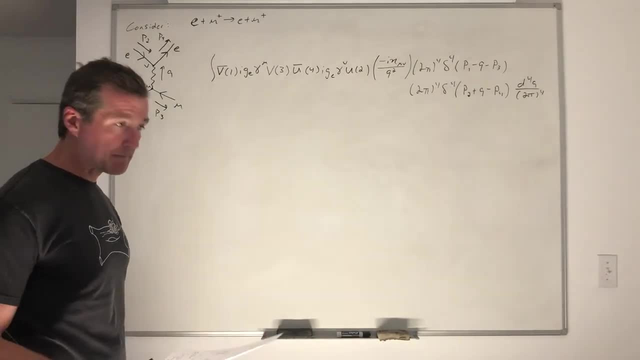 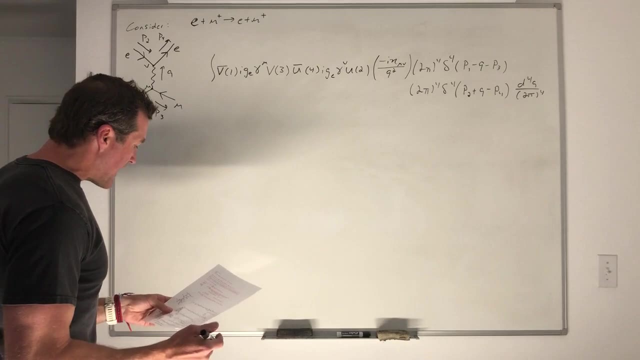 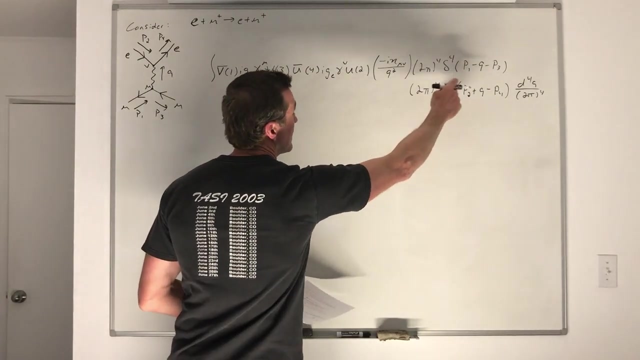 But otherwise we're still following the same sort of rules that we did with the ABC theory. Okay, So now let's clean this up a bit. Let's gather some factors And let's go ahead and do the. let's use the delta function to do the integral over q. 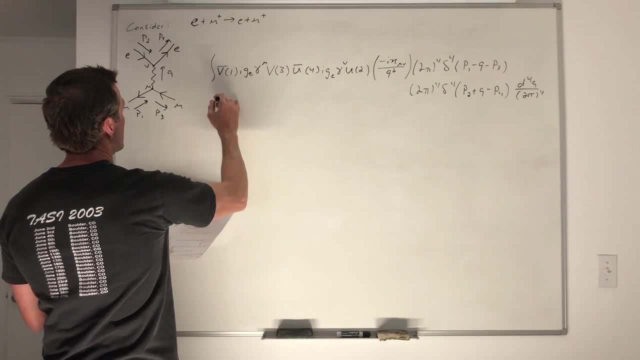 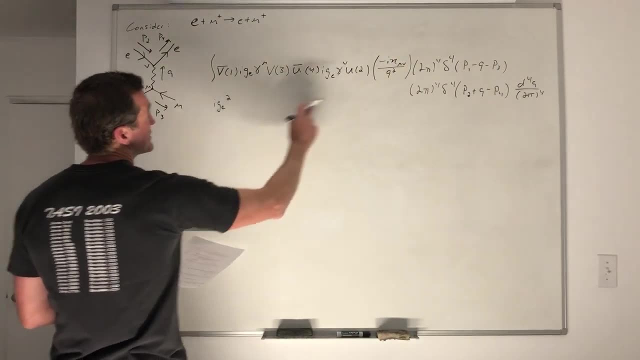 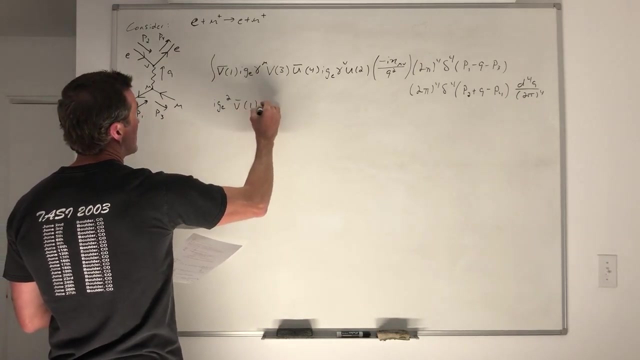 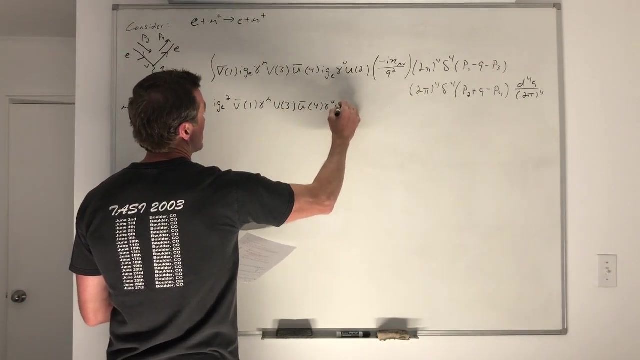 And what we're going to end up with is the following: i g e squared. I'm just going to say: i times i is minus, times that minus is plus. So this is that overall. i, right there, g e squared. And then we're going to have v bar 1, gamma mu, v3. u bar 4- gamma nu- u2.. 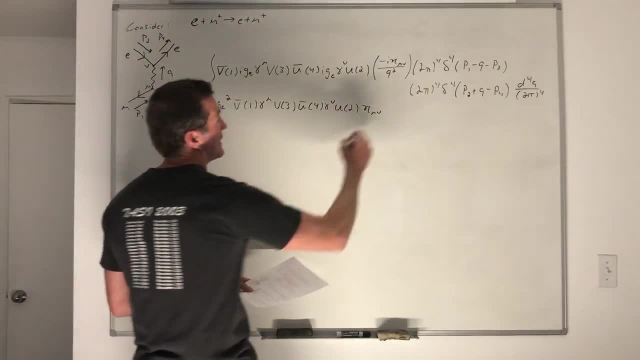 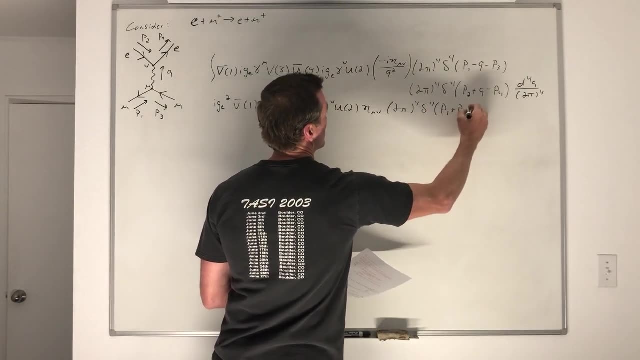 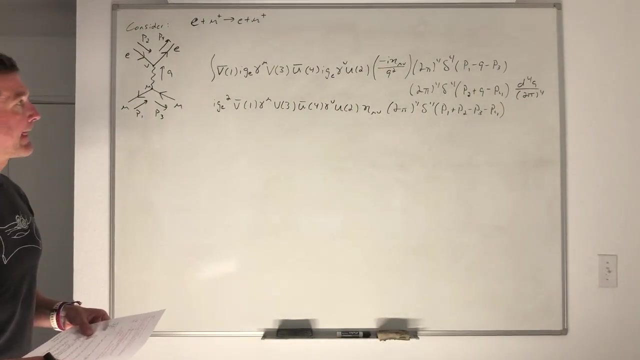 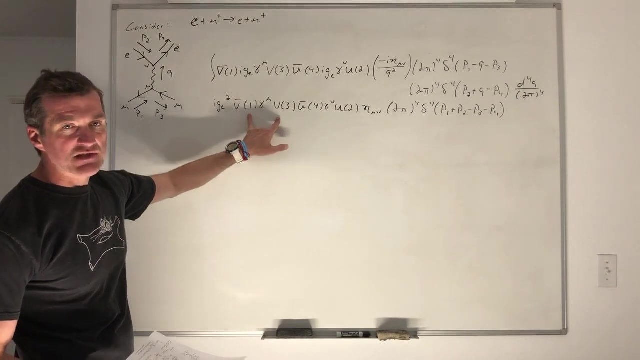 And then an eta nu And then an overall 2 pi to the 4th delta 4.. p1 plus p2 minus p3 minus p4.. Okay, And all I'm really doing is I'm pulling all the constants out front so that this is just a spinner sandwich that's made of non-trivial spinner things. 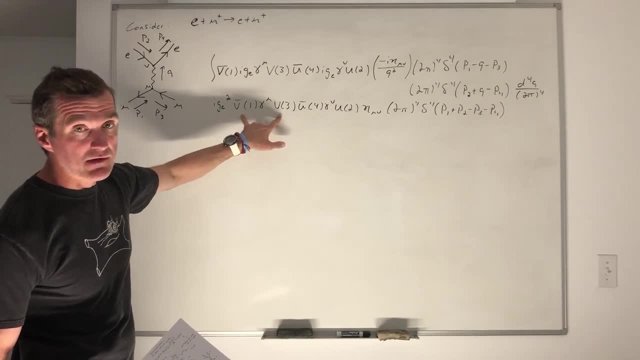 Like: this is a gamma matrix And these are spinners and androids spinners, And I don't want a bunch of constants sitting in there because I'm going to, you know, I'm going to replace these with things in a few minutes. 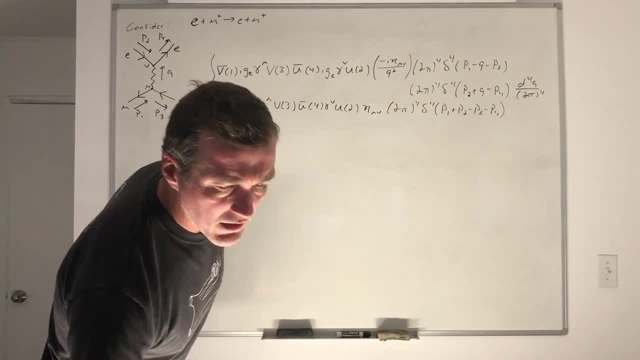 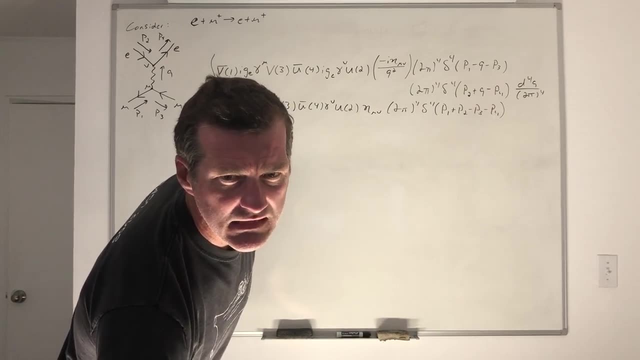 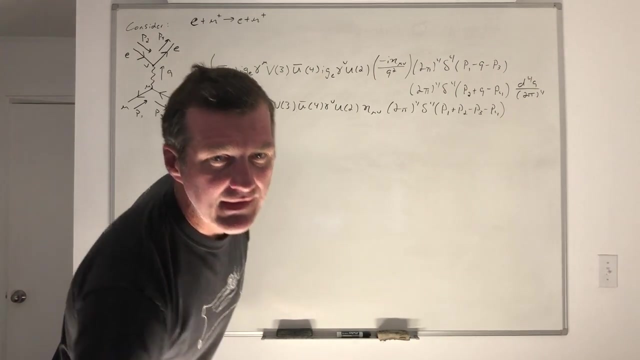 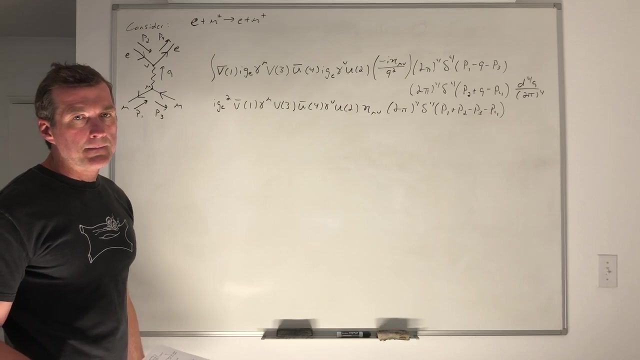 Okay, So let me grab a card. Andy, are you there? Is Andy there? I don't see Andy, Andrew. Yeah, Hey, Andrew. What do I have to do to this in order to get the expression for m? 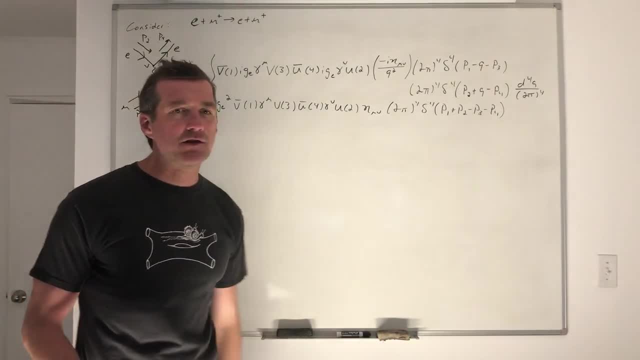 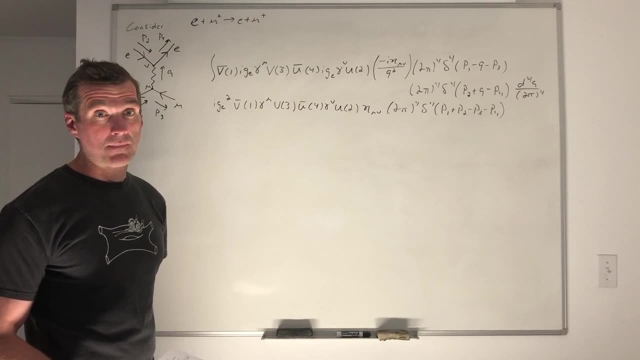 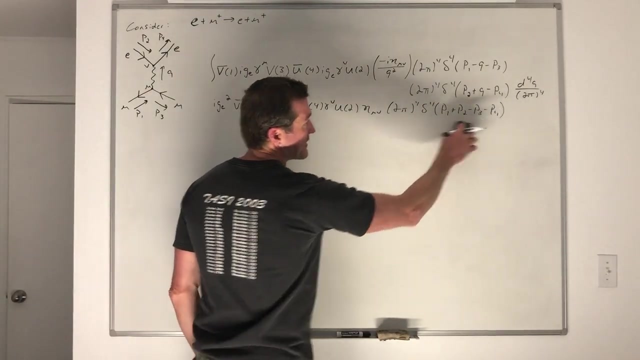 It's the final step, both in the ABC theory and in QED. What's the very last step? And then we just multiply by i And erase something. What do I erase? Oh, the 2 pi 4.. Yeah, because this thing is also going to appear in the golden rule. 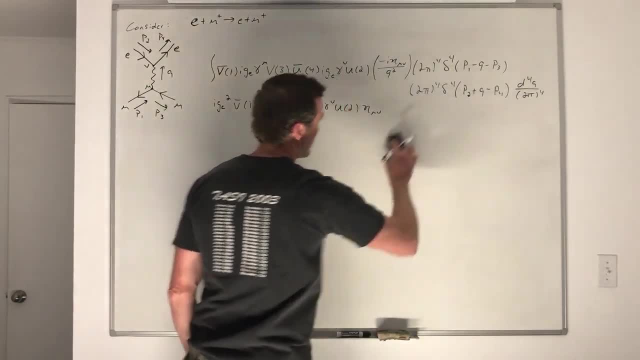 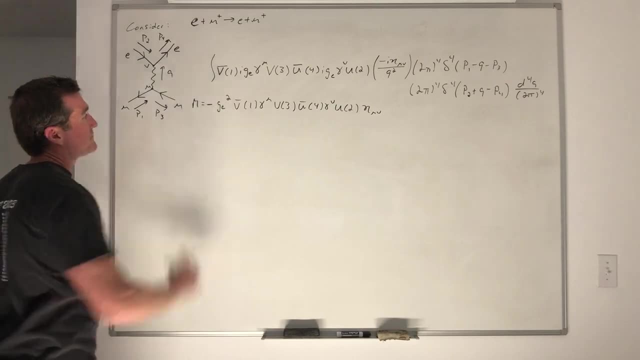 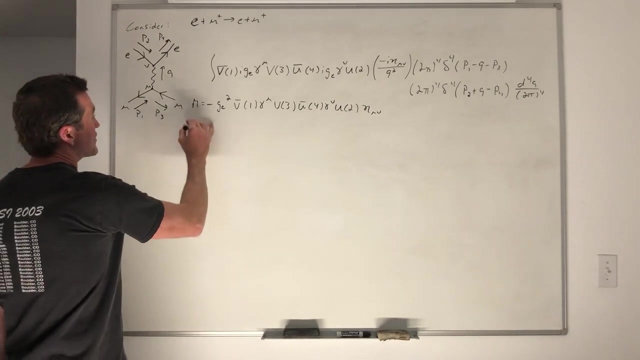 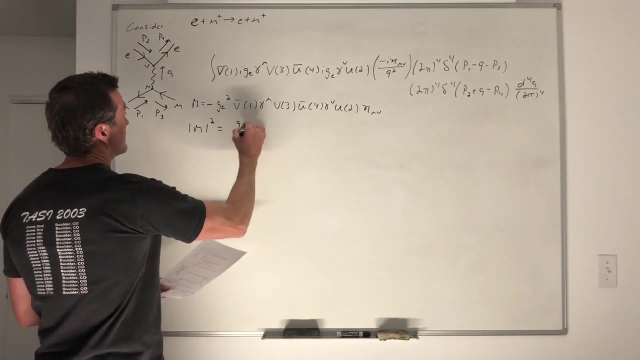 So we don't want it to appear in the amplitude expression as well. Okay, So there's my expression for m. Okay, All right. Now what we're going to do with m, of course, is square it. So let's go ahead and square this bad boy. 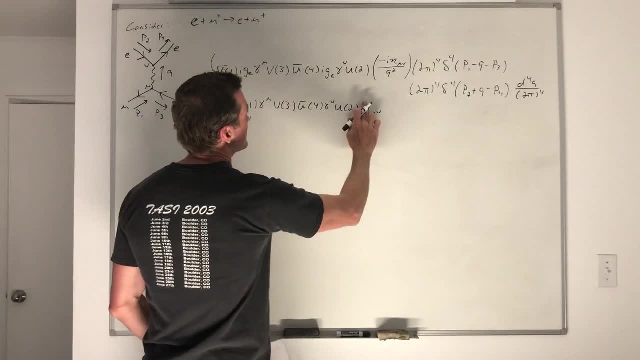 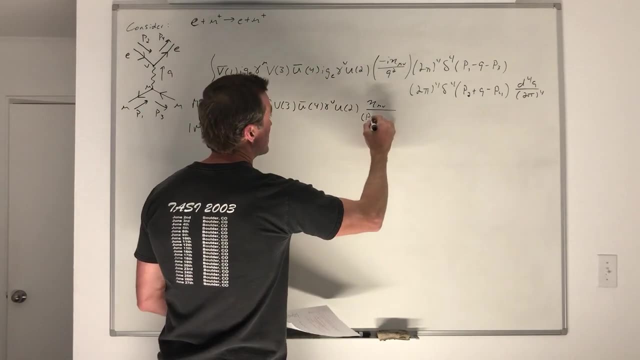 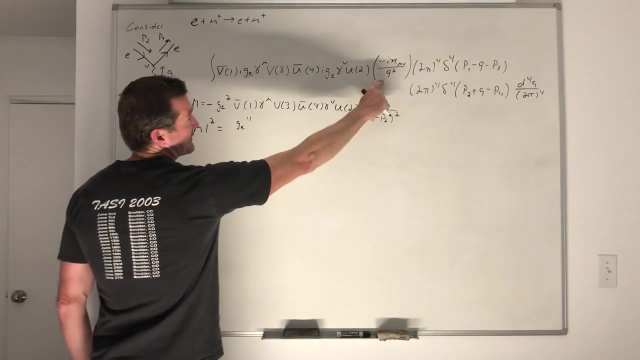 Oh, sorry, Sorry. This should have been a to mu nu over p 4 minus p 2. Square. Sorry about that. Okay, That's just the q squared. when you do the delta function, It replaces it with p 4 minus p 2.. 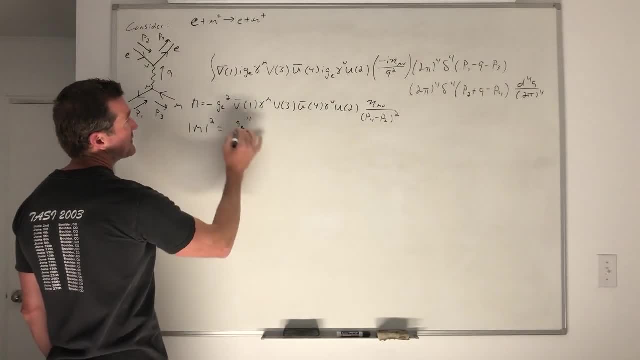 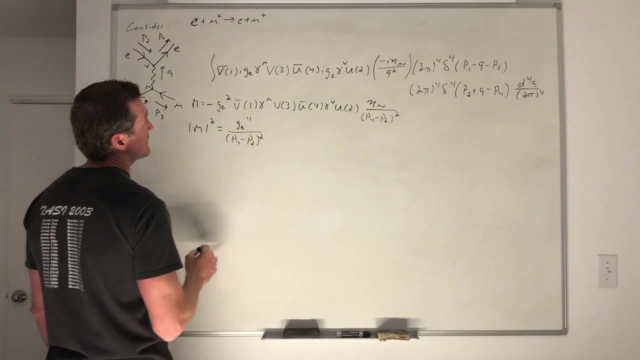 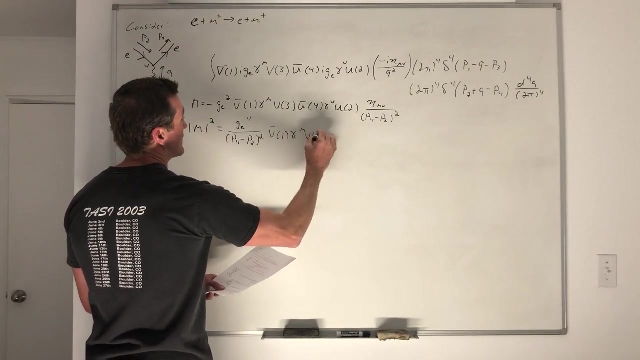 Okay, So when I square this expression, I'm going to have g e to the fourth. I'm going to pull that p 4 minus p 2 factor over here, And then we're going to have v 1, gamma, mu, v 3, u, bar. 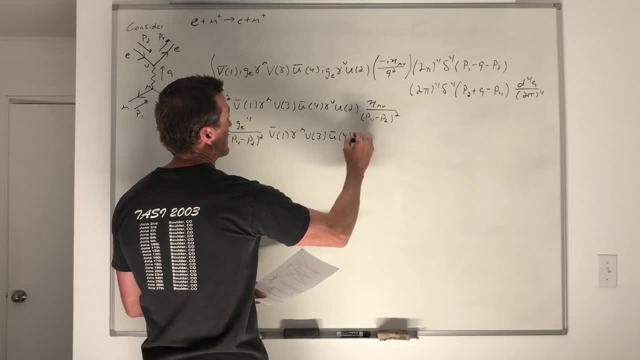 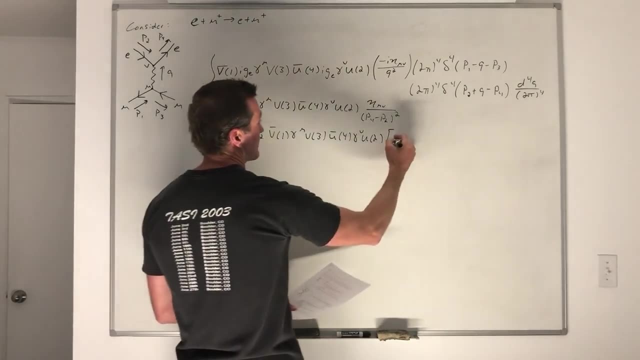 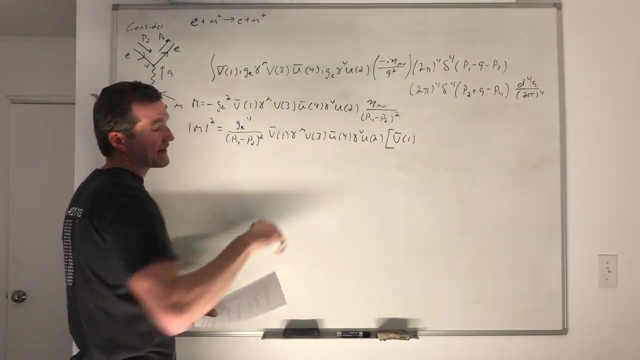 u bar 4, gamma nu u 2.. And then we repeat this. except when we repeat it, we want to make sure that we give the gamma matrices that appear in the second factor different indices, so that we don't accidentally sum over them. 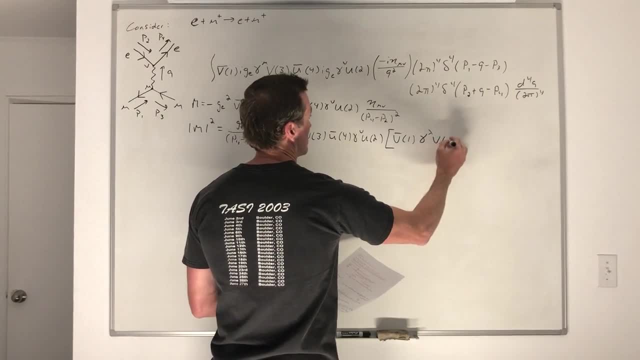 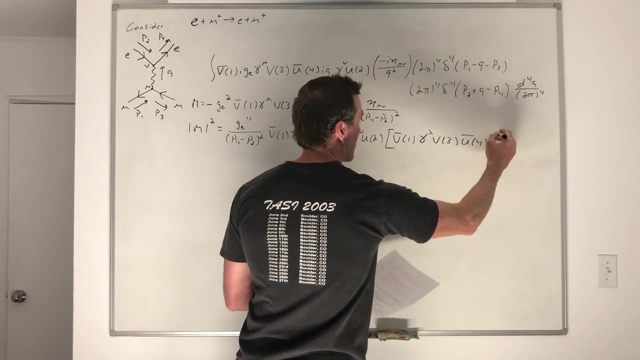 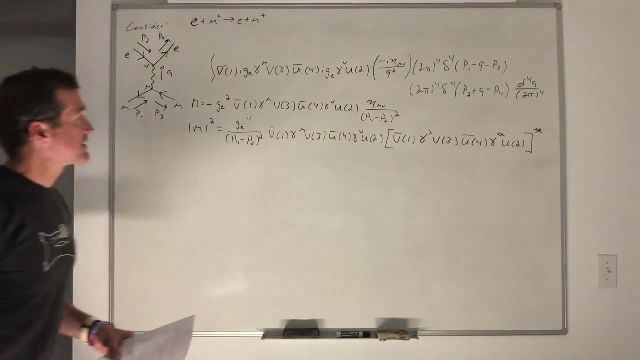 So I'll do a gamma lambda here, And I'll do a gamma alpha here, And then we want to complex conjugate everything in there. So all I'm doing is I'm taking this and I'm multiplying it by its complex conjugate. 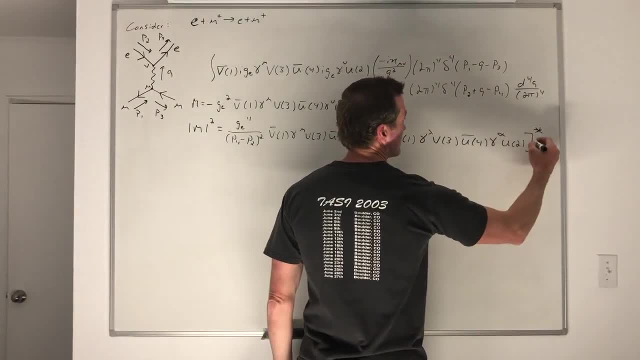 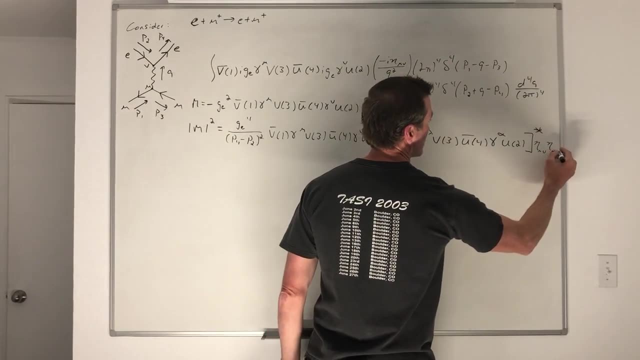 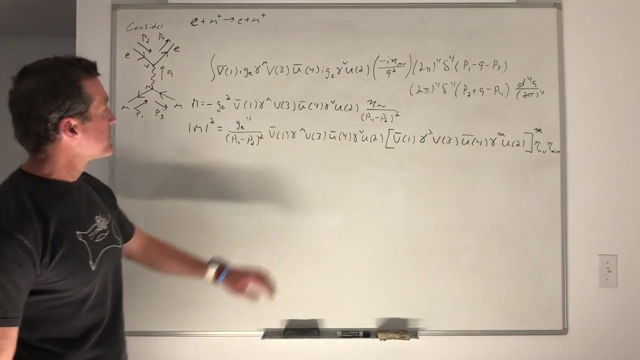 Okay, And then we also have a factor of eta mu- nu and a factor of lambda alpha, Sorry, Eta of lambda alpha, Eta sub lambda alpha. This is what I should be saying. Okay, Because if in this expression we're contracting the mu and the nu with a metric factor, we have to do the same thing in this. 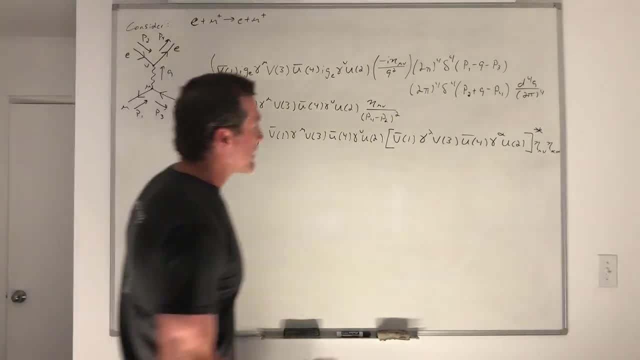 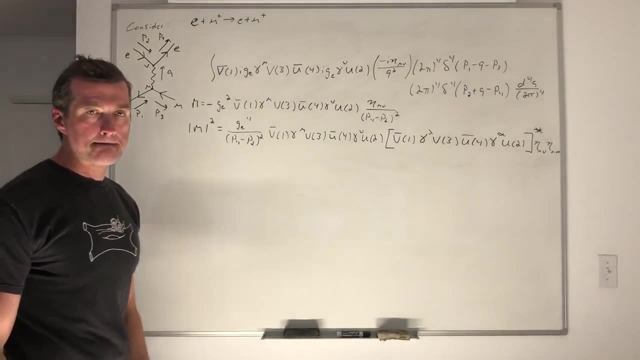 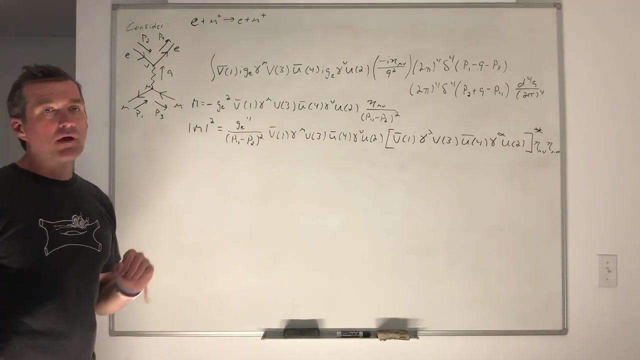 So we'll just get an eta lambda alpha in order to do that. Okay, We good, Excellent, Okay. Now is where I'm going to employ that rule for what to do if you want to sum over spins, Okay. So what we're going to do is we're going to go straight from this to this. 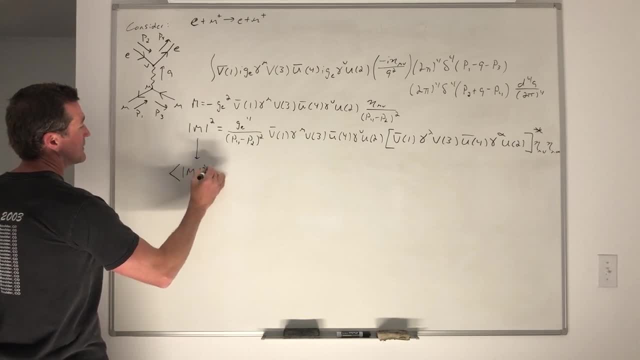 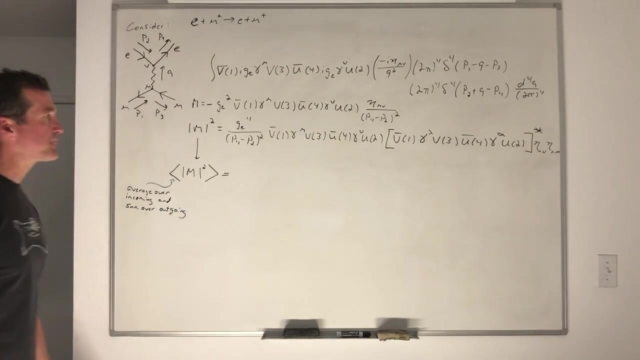 Where the bars mean average And sum over outgoing. Okay, So that's what my angle bars mean. So, first of all, if I'm averaging over the incoming spins, I have two particles and they each have two spin states that are available to them. 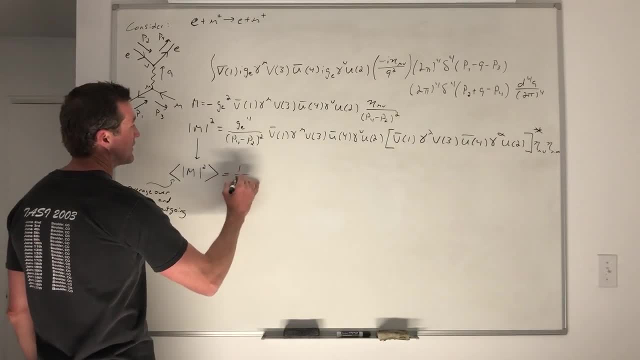 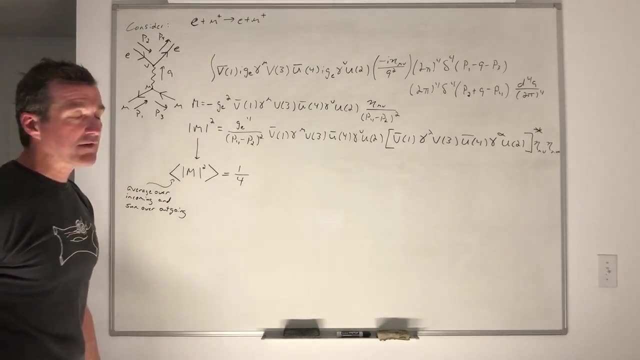 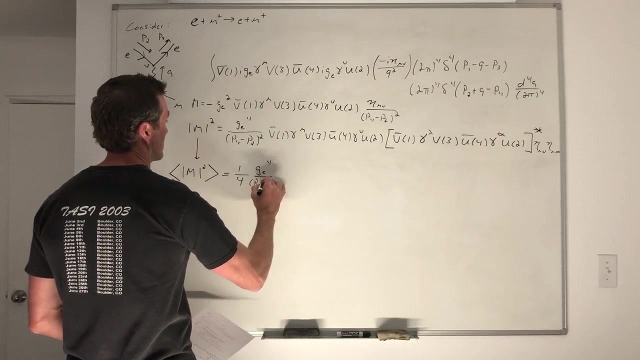 So that gives me an overall factor of one-fourth times the sum over the incoming spins. Okay, And then I have to do a sum over the outgoing spins, So that gives me an overall factor of one-fourth times the sum over the incoming spins. 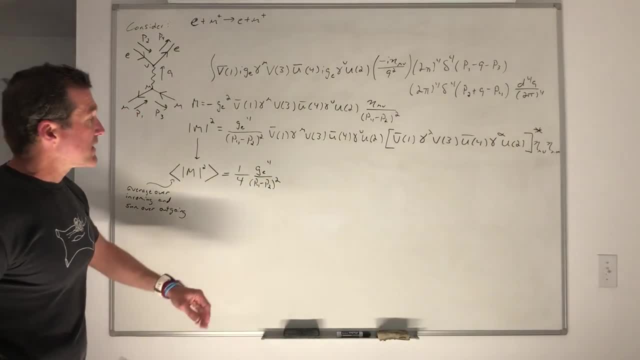 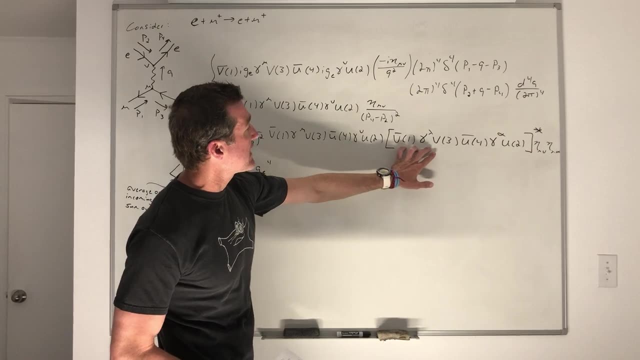 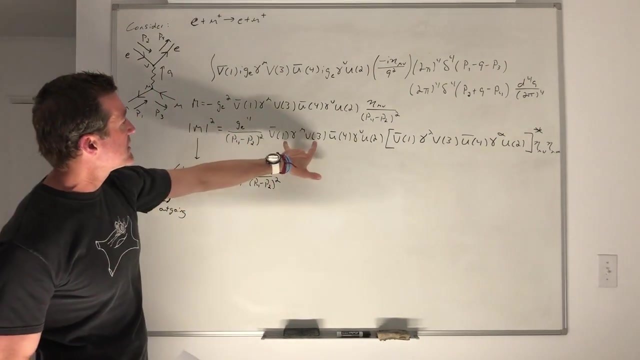 Okay, And now is where we use that little bit of magic, because we have v1 gamma mu, v3, v bar one, gamma lambda, v3, star times- a metric factor And we want to average, or we want to add up the spin states for one and three. 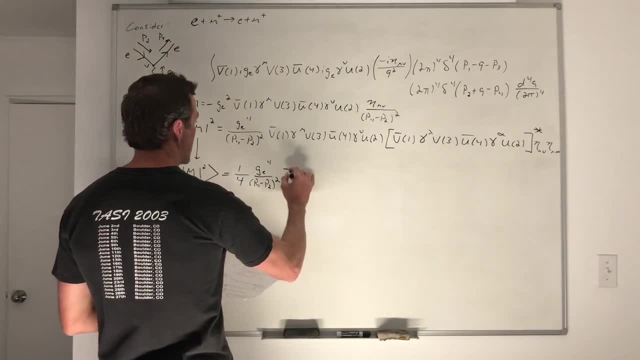 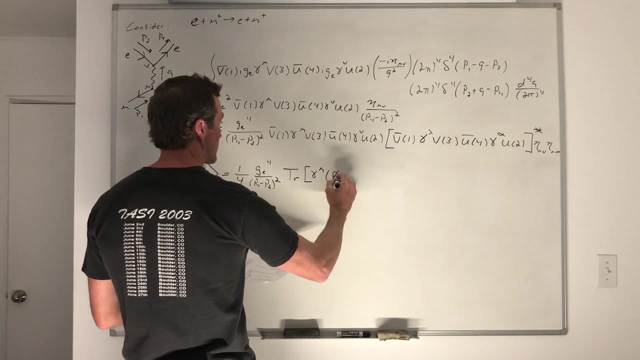 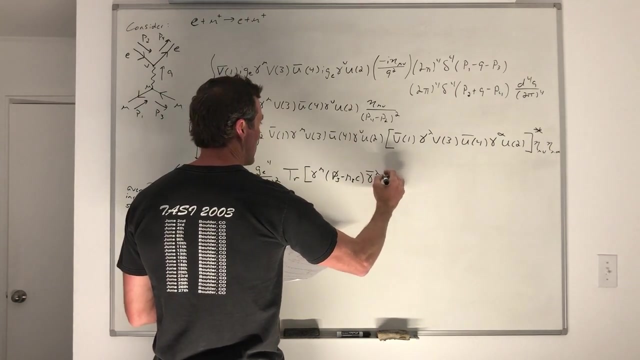 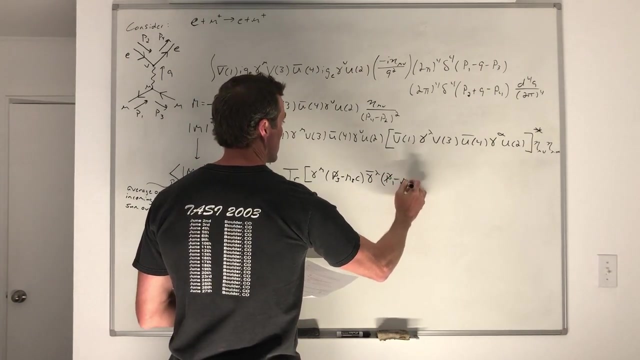 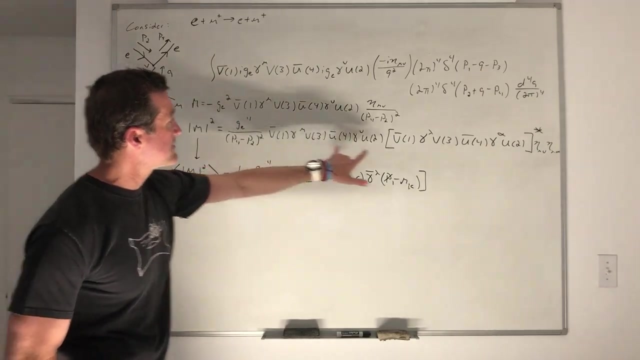 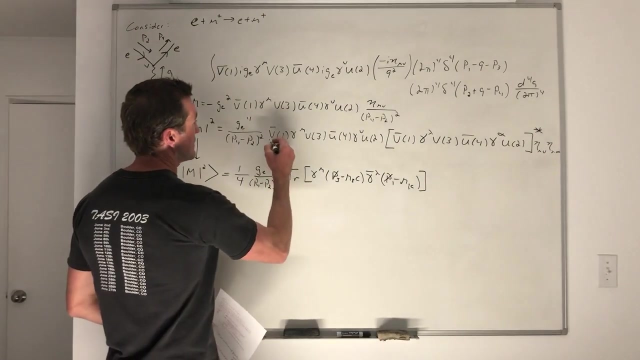 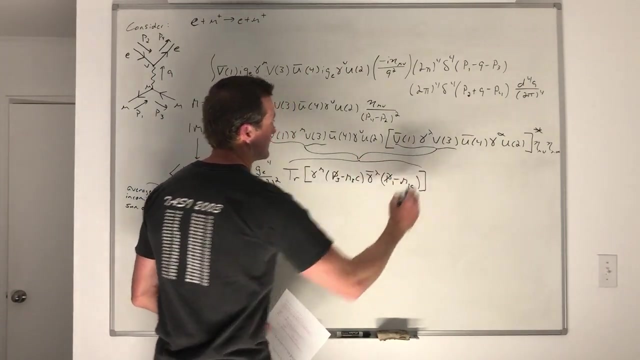 So when we do that, we have trace of gamma mu: p3 slash minus m3c. gamma lambda bar: p1 slash minus m1c. Okay, That's just substituting instead of this times this. If I want to do this times this and sum over the spins, then I get to replace it with this. 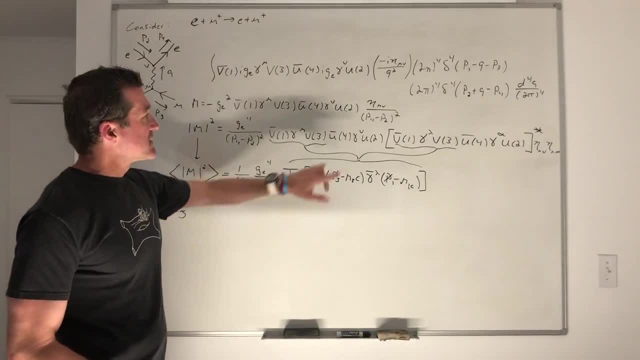 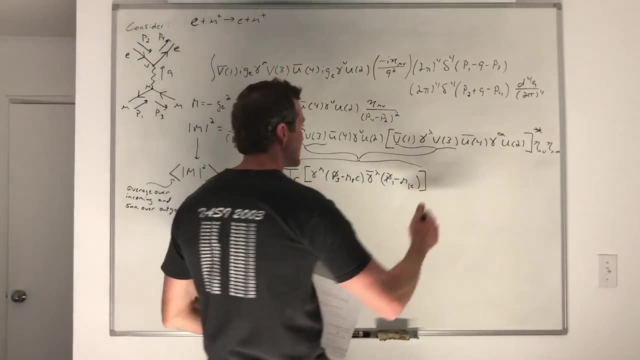 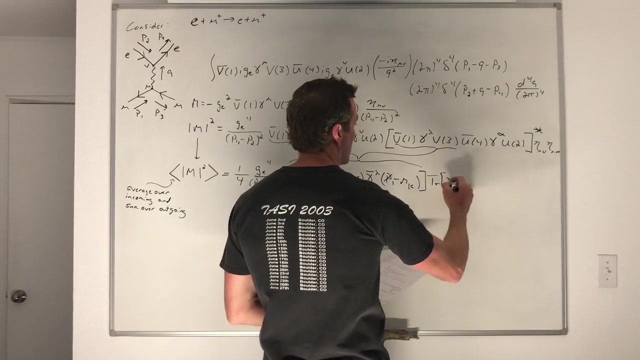 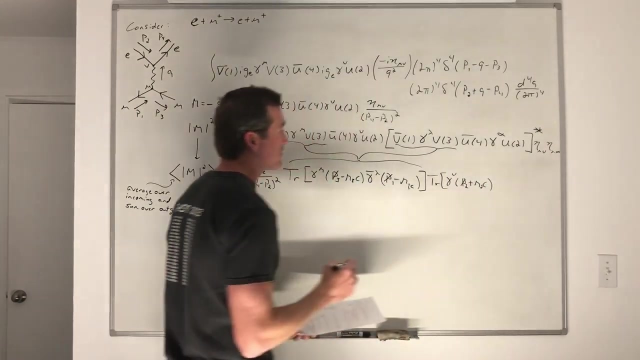 Okay, There you go. So then we can go ahead and write down what we need for the four and the two spinner sandwich, And so that's going to be another trace factor, And in this case it's going to be gamma mu, p2 slash plus m2c, because we're using particles instead of antiparticles. 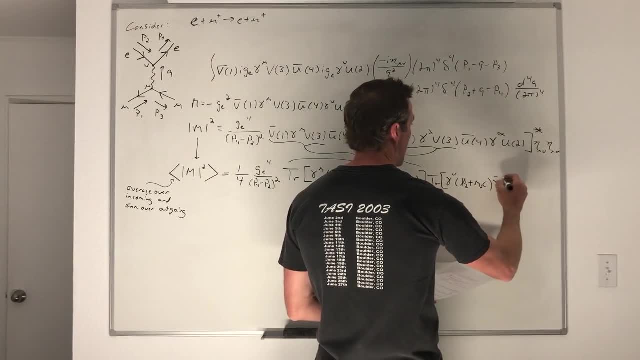 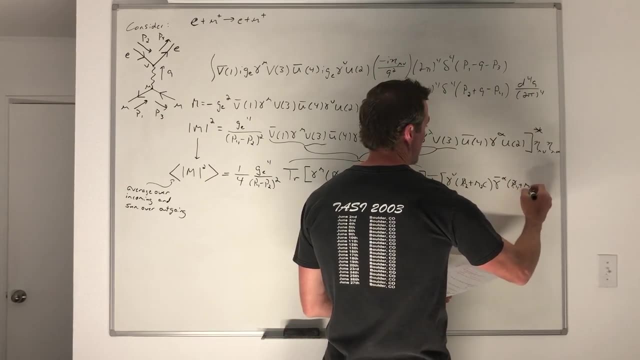 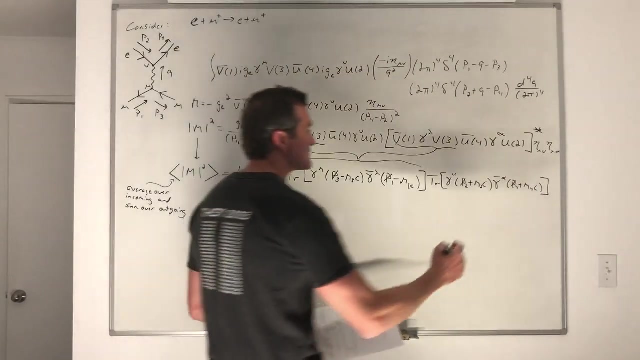 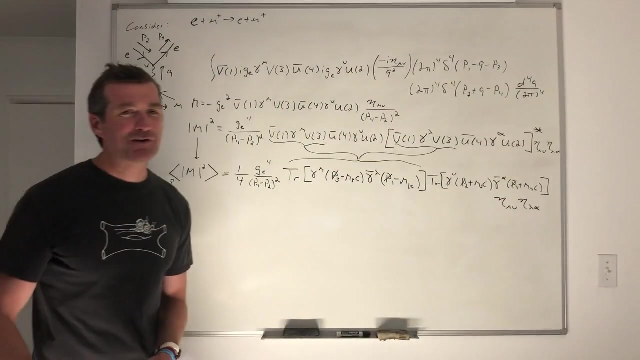 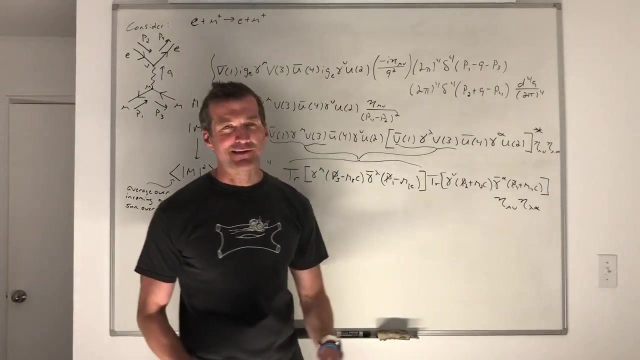 Gamma bar alpha, p4 slash plus m4c. Okay Times, of course, this eta mu nu, eta lambda alpha- And it's kind of funny that I used the word times, Isn't that funny? Like you, multiply by these two things. 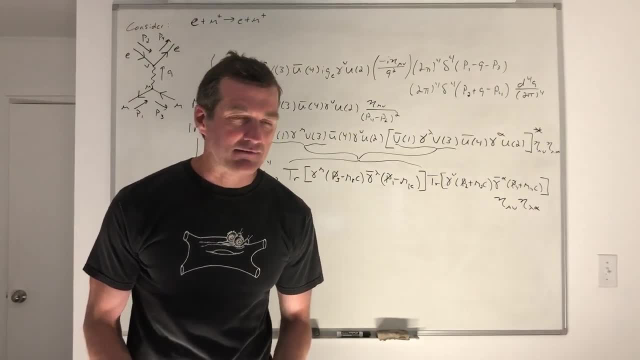 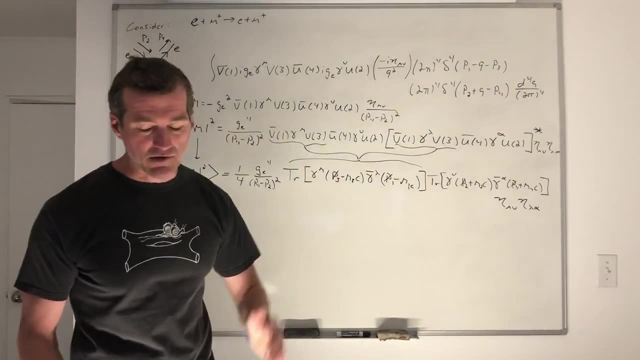 This is the biggest bunch of bullshit I've ever heard of These operators contract indices over here, So it's not just multiplying by a number. It's ridiculous that I would even say that You guys should laugh at me, But I'm very glad you're not. 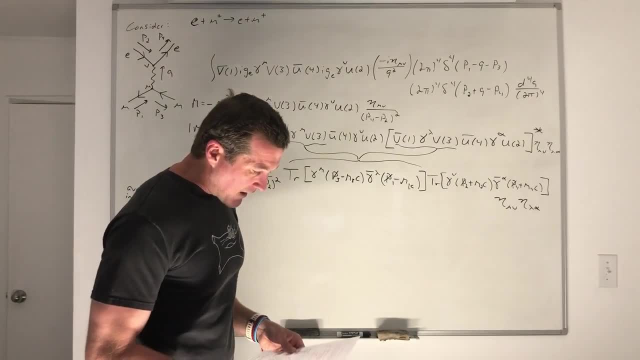 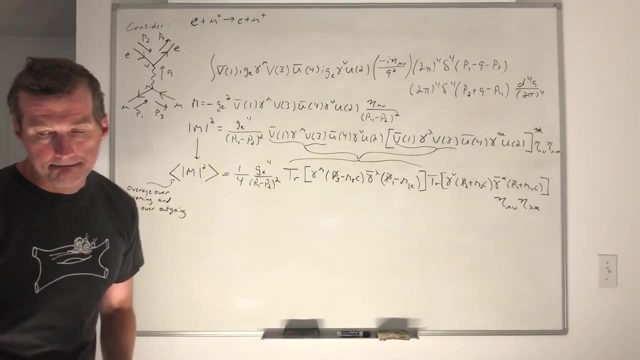 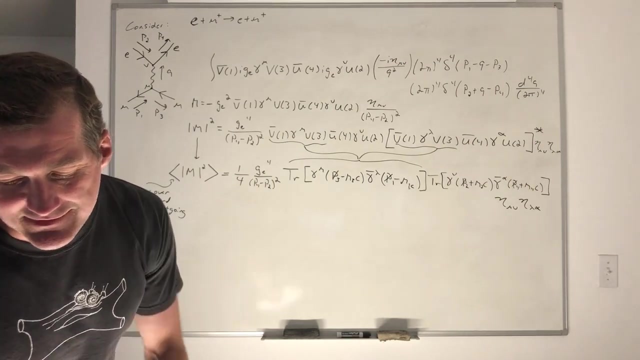 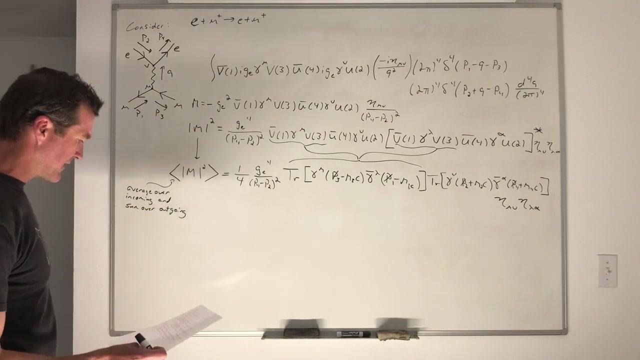 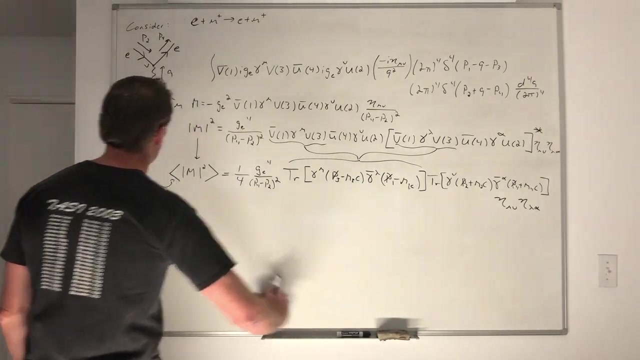 I really do appreciate it. Okay, So are there any questions about this expression? so far, None, Nice, Awesome. Okay, Now let me see how I can make some room. Okay, So let me just keep that front and center. 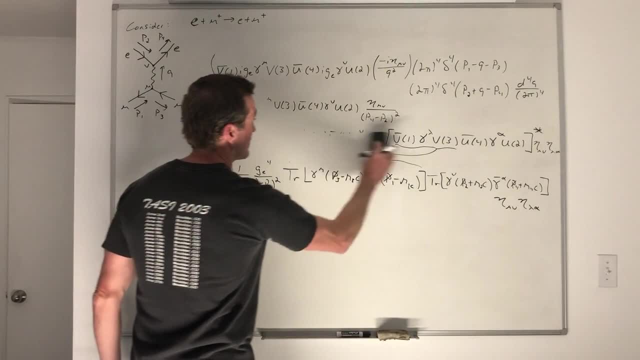 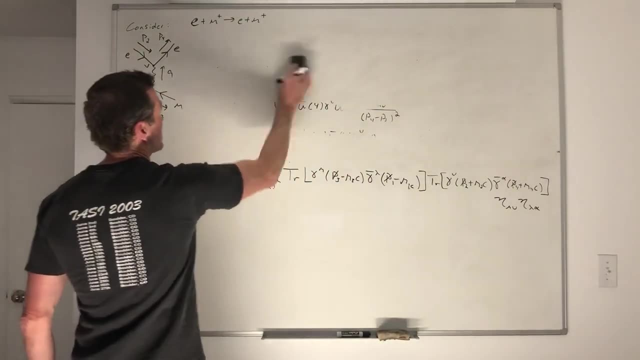 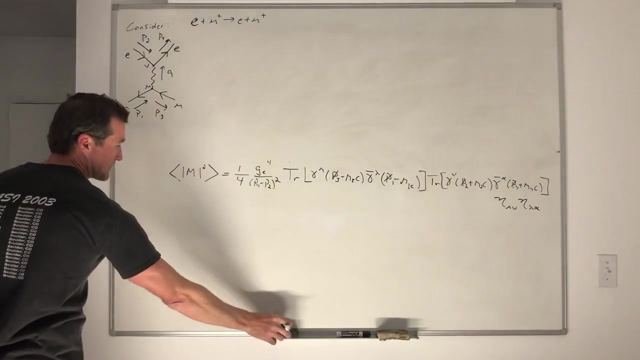 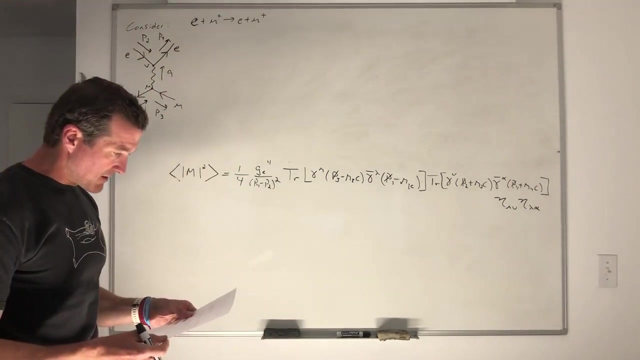 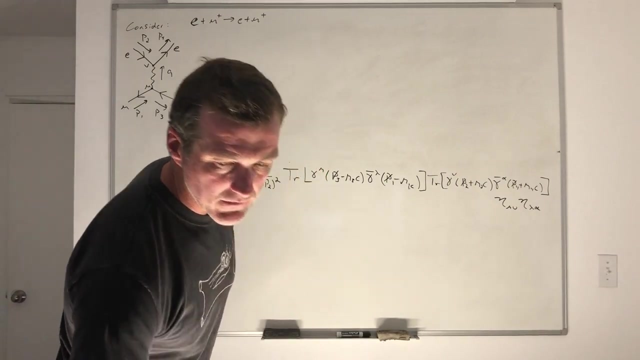 I'll get rid of all this. This could be pretty nice, It could be pretty sweet. Okay, All right Now. so, first of all, and let me pick a victim for this: Jalon. Hey, Jalon, You're up in my upper right-hand corner. 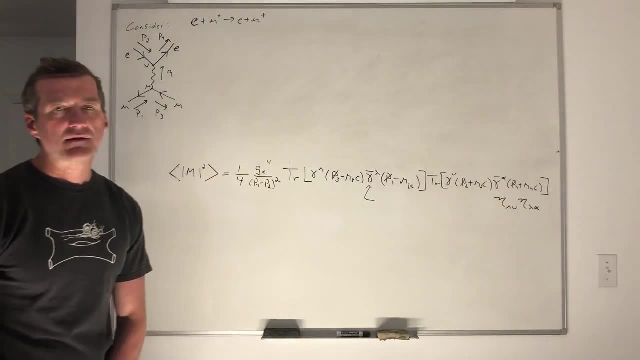 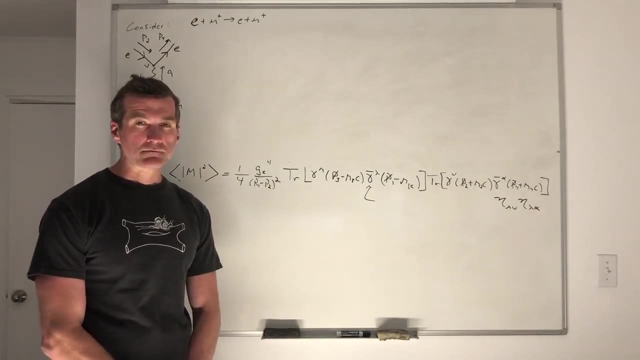 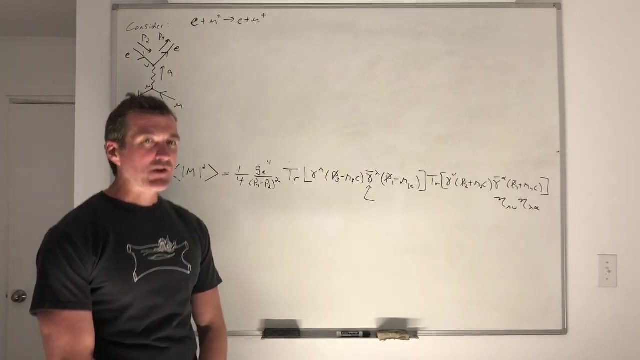 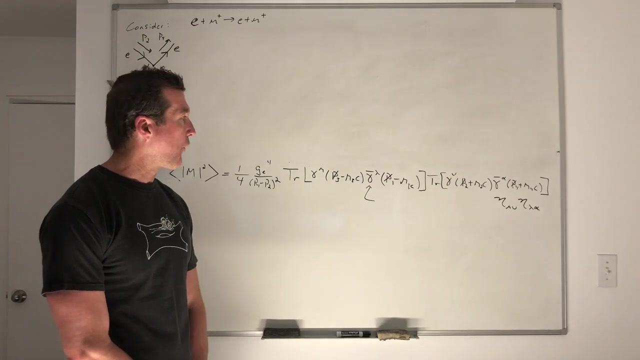 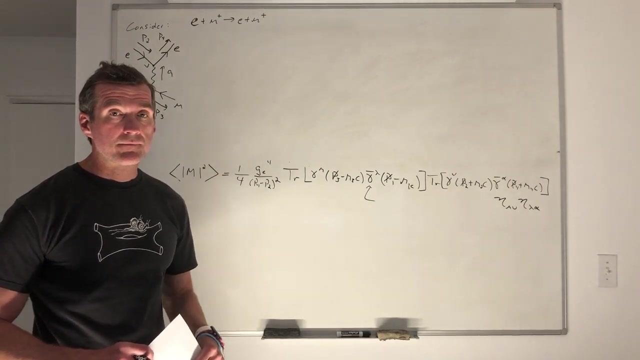 What does this gamma bar lambda look like? Like what does the bar mean? What do we do to make the bar? I have no idea. So look at the notes from the last lecture. Yeah, So you just stick the gamma mu in between two gamma zeros. 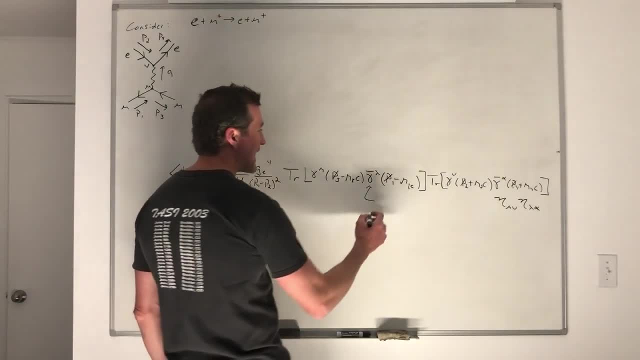 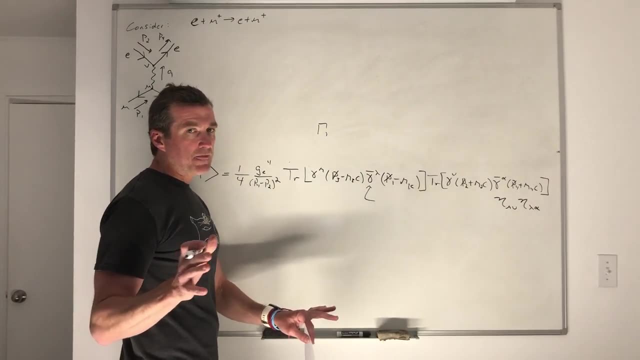 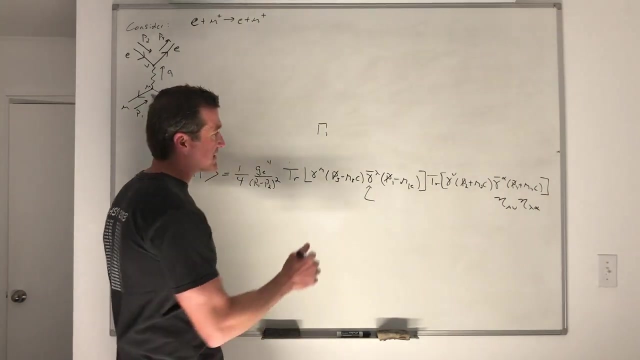 and then complex, conjugate the or dagger the gamma mu, Exactly. So I did it with an arbitrary spin matrix. Okay, Here our spin matrix is just gamma lambda. But you know, you could have situations where you have more complicated spin matrices. 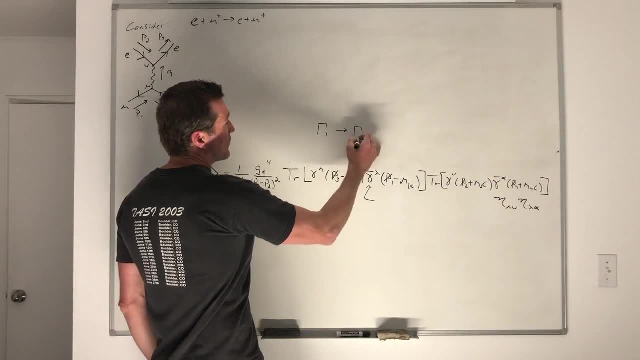 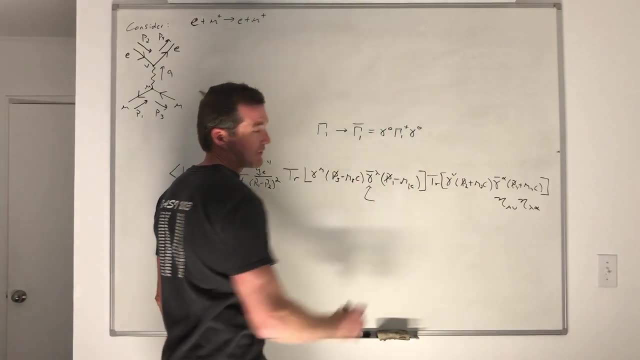 But at any rate, if I take gamma one and I want to make gamma bar one, then I do gamma zero. gamma one dagger gamma zero. So if I only have a spin matrix as gamma one. so in this case my gamma one is just gamma lambda. 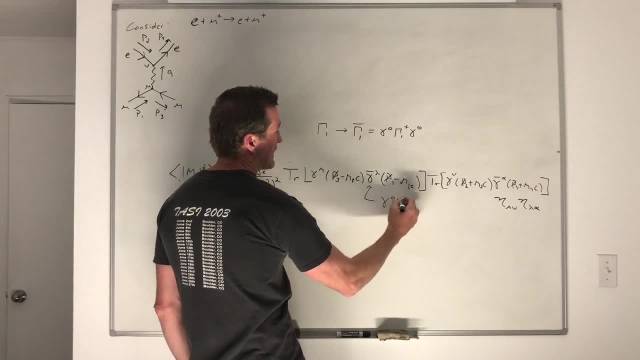 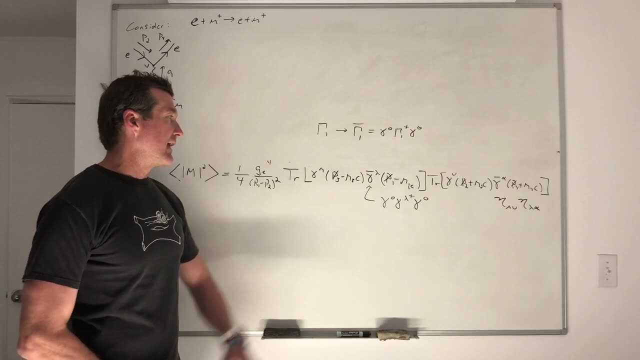 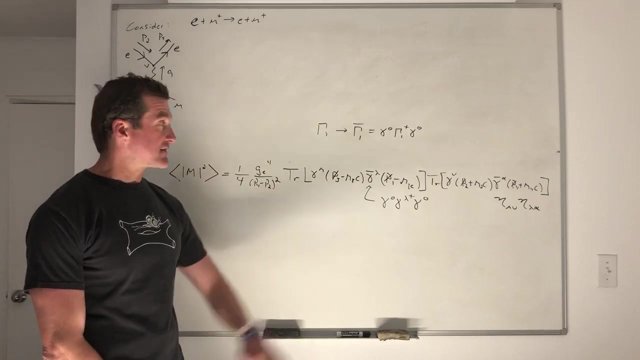 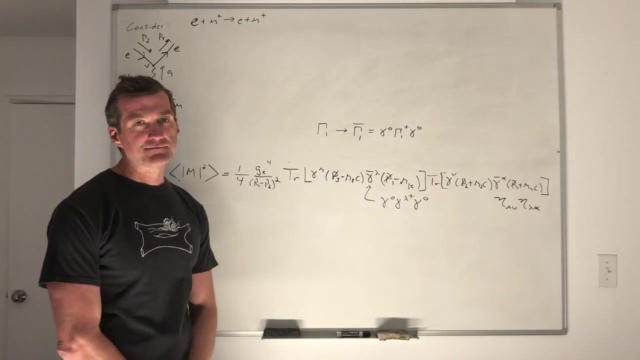 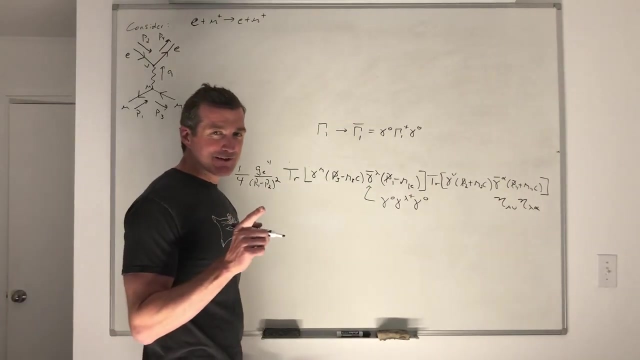 then gamma lambda bar is gamma zero. gamma lambda dagger: gamma zero. Okay, This is a special case. Why in the world do you think this is a special case? What in the world could be special about that? Well, it is highly non-trivial. 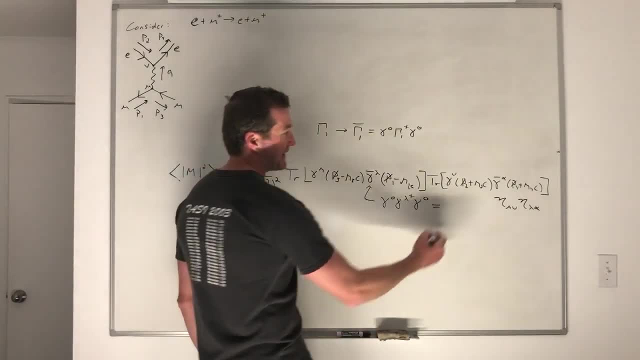 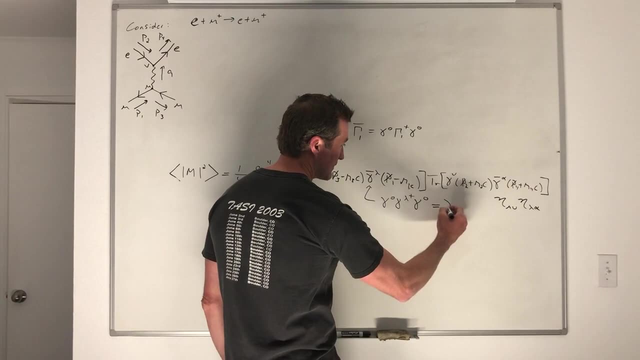 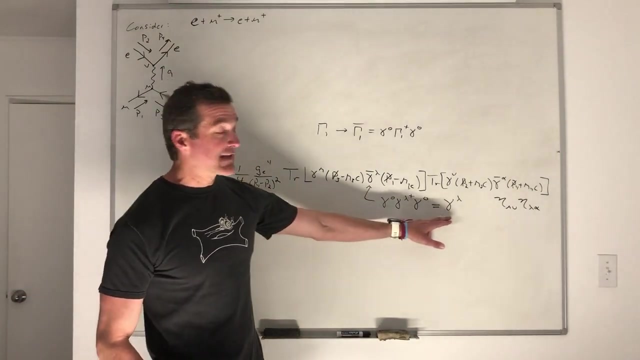 but this is equal to a very complex expression which I'll try and write small. I'm just kidding. This is actually just equal to gamma lambda. Okay, All right, And you don't have to take my word for it. You can verify this. 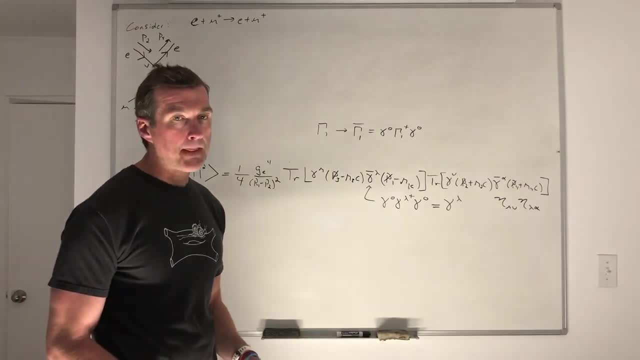 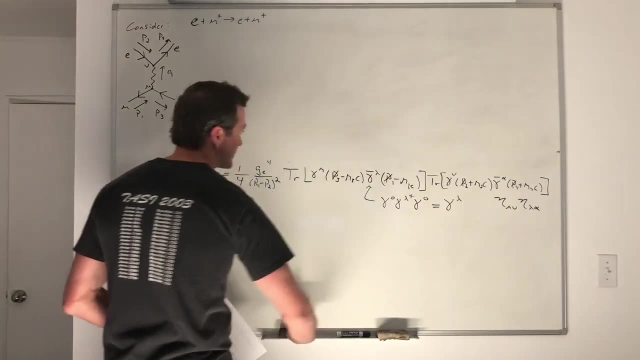 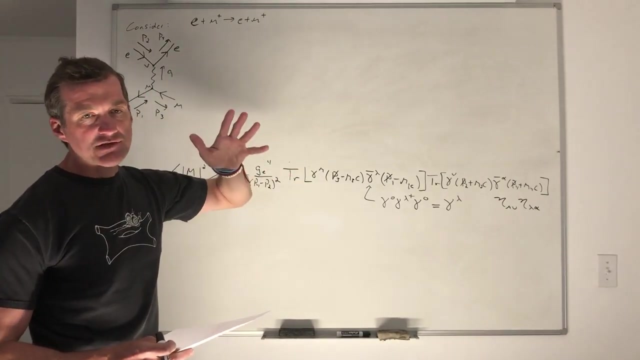 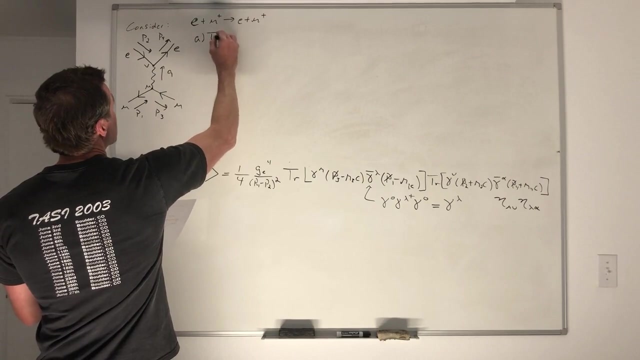 That's pretty straightforward, All right, Okay. So with that in mind, what I would like to do now is write down the trace identities over gamma matrices that we're going to make use of. So first of all, recall that, if I have the trace of four gamma matrices, 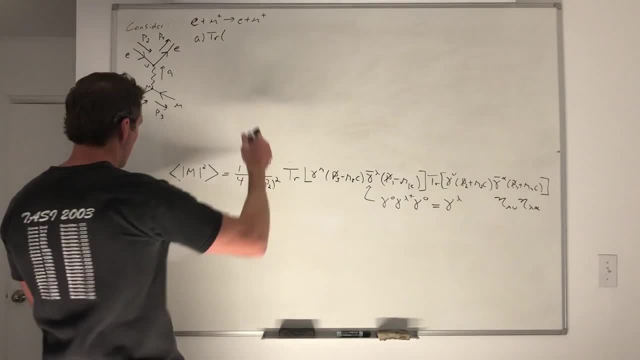 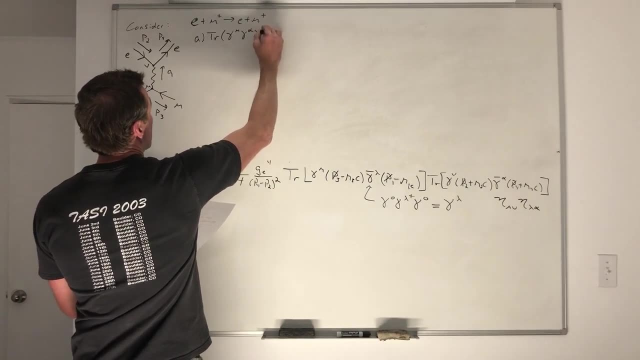 and I should be reminding you of this because you've done homework with these. In fact, you've proven them in your homework. If you have four gamma matrices, you can write down the trace identities over gamma, alpha, gamma lambda, gamma beta. 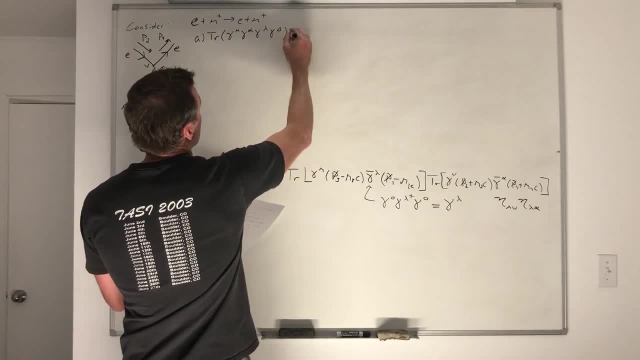 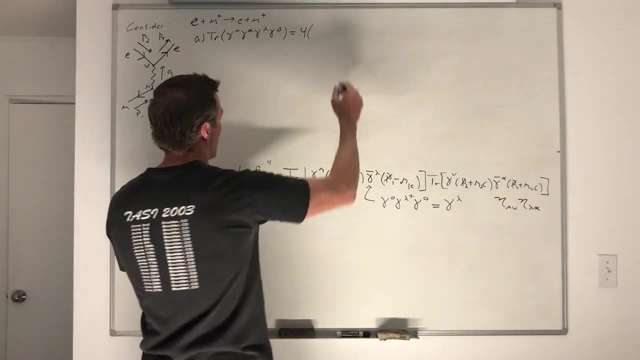 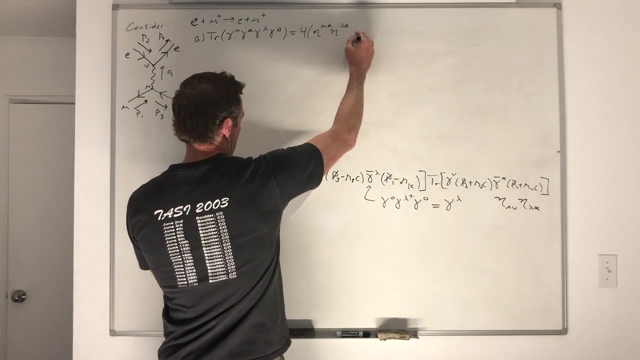 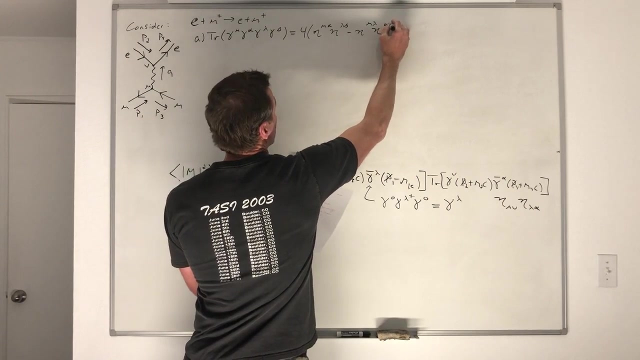 Then this comes out to be this sort of: it's a long expression, but it's four times a bunch of metric factors. So we have eta mu alpha, eta lambda beta minus eta mu lambda, eta alpha beta Plus eta mu beta. 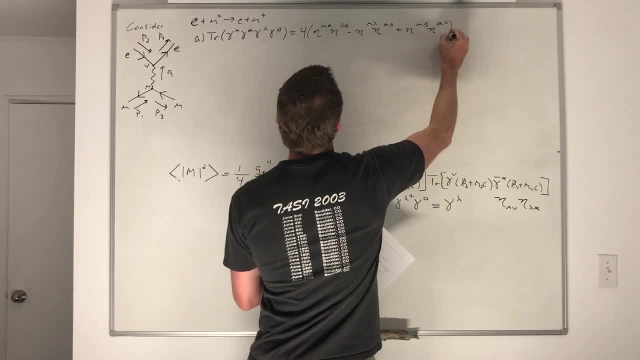 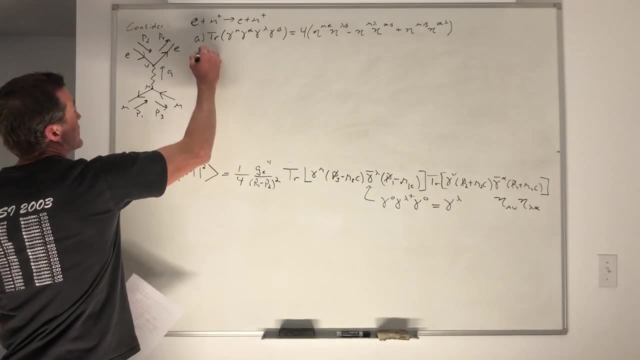 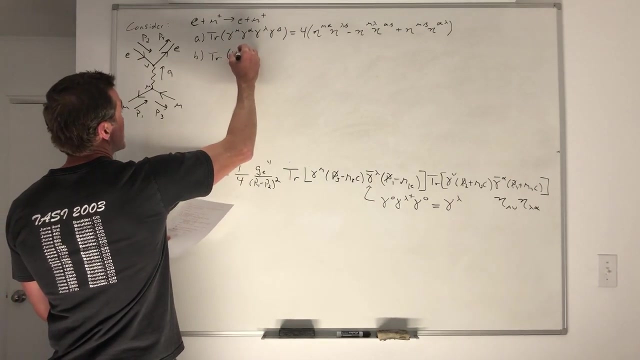 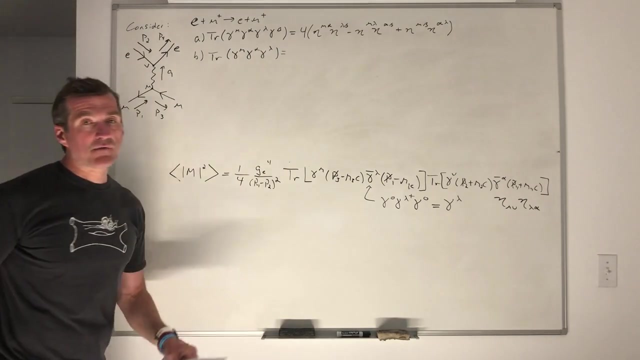 eta, alpha lambda. Okay, A second trace identity that we'll use- and this is a lot nicer- is the trace over an odd number of gamma matrices, but in particular we're talking about three. Anybody remember what the trace of an odd number of gamma matrices is? 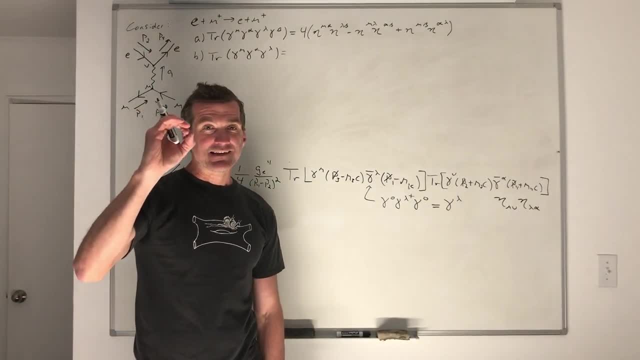 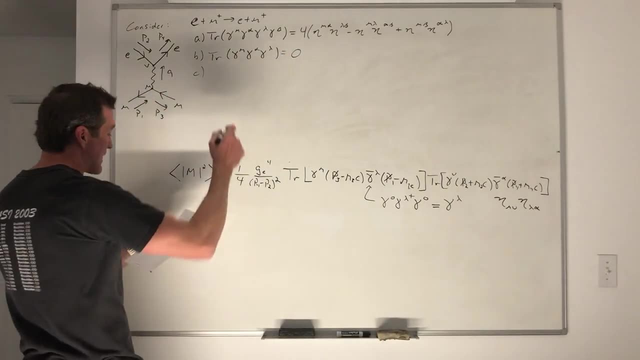 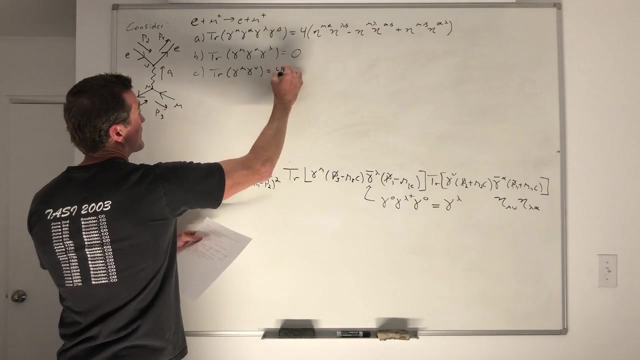 I see people holding up their hands. Zero, Yes, thank you, This is zero. And then, lastly, the trace of two gamma matrices is four times the inverse metric. Okay, And if I screw up and write a G instead of an eta. 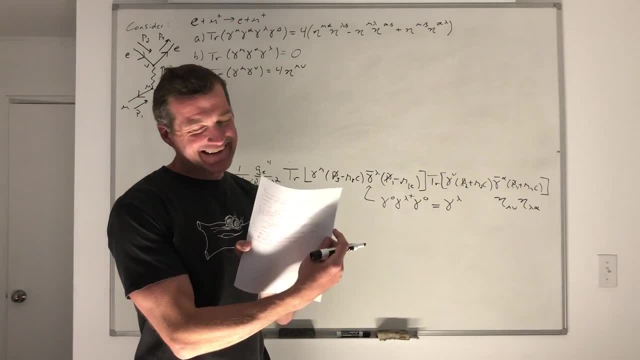 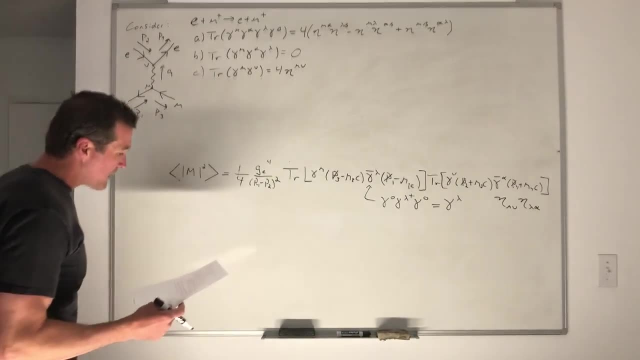 please somebody let me know, because it's G in all my notes And I'm doing my best to transition it to eta. Okay, Where eta is the metric of Minkowski space. Okay, So here we go, Here we go. 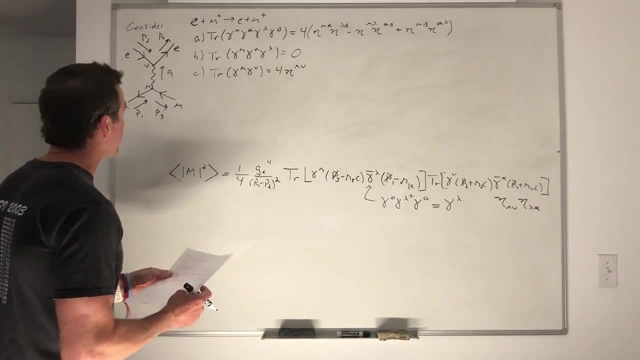 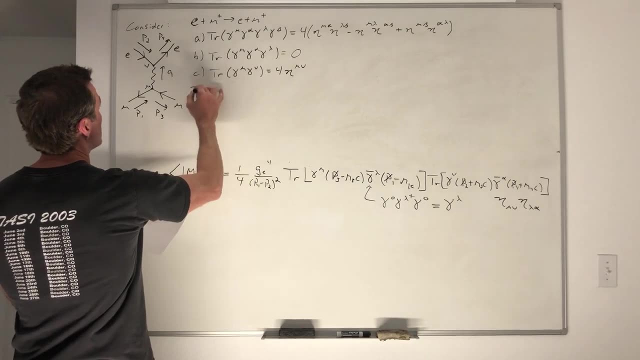 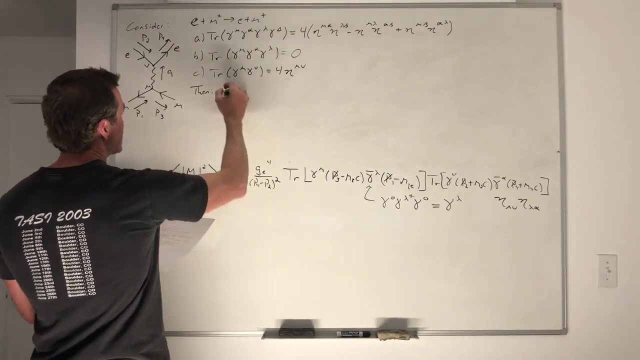 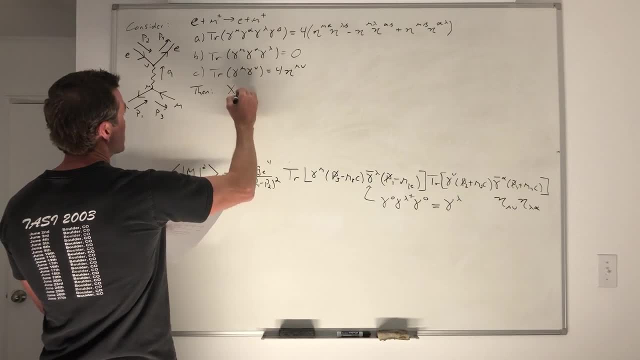 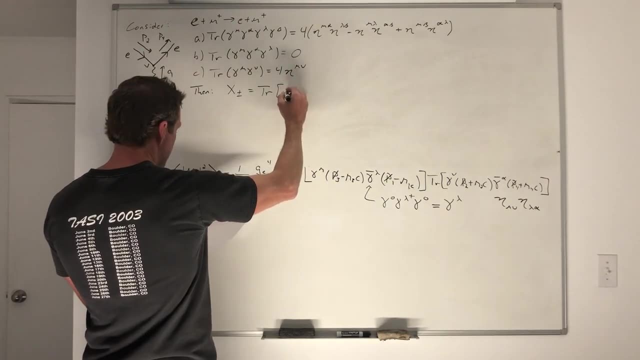 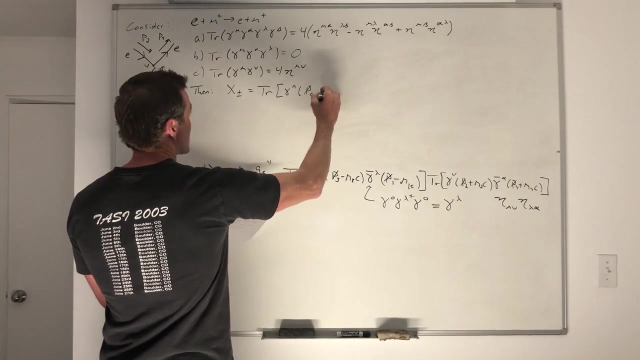 Actually, I'll do this. I'm going to define something called X plus or minus, And this is just going to be one of these trace factors. So we've got trace gamma mu P slash of A plus or minus, M, A, C, gamma mu lambda. 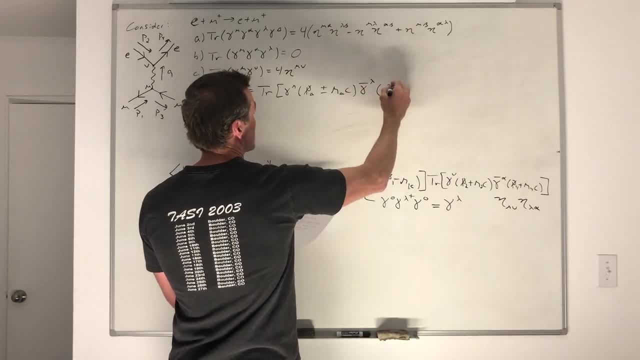 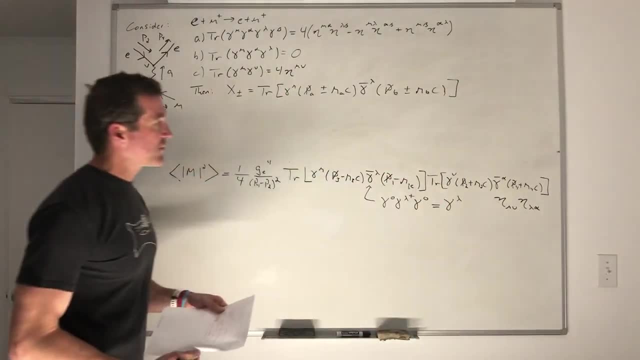 Sorry, Gamma mu lambda P slash B plus or minus M B C. So I'm just going to do this in general and once we get the answer, then we can just substitute it based on whether it's plus or minus down here. 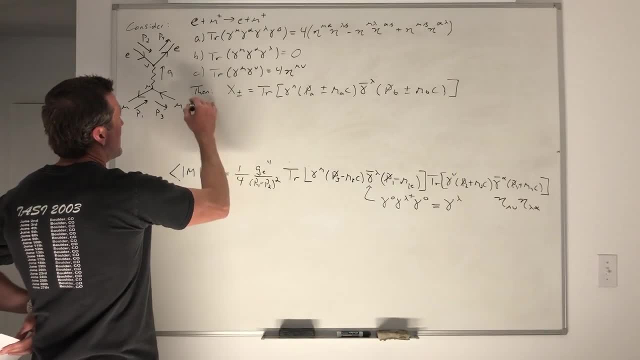 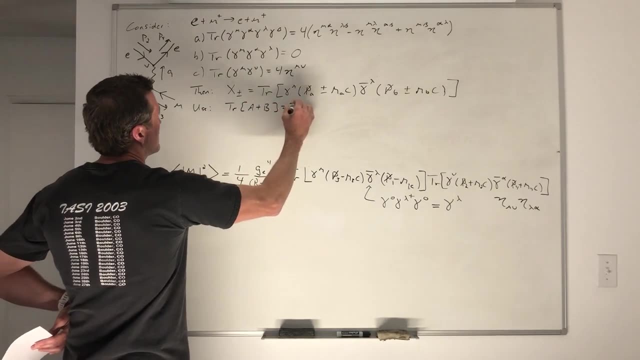 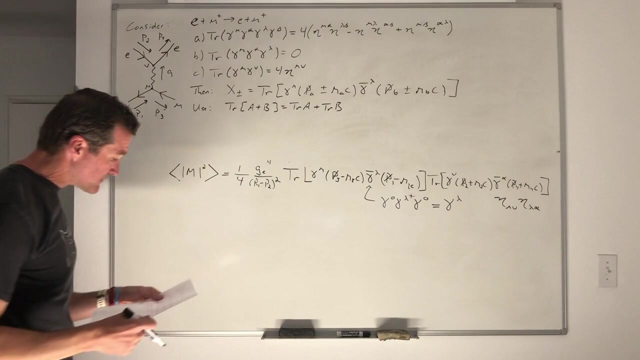 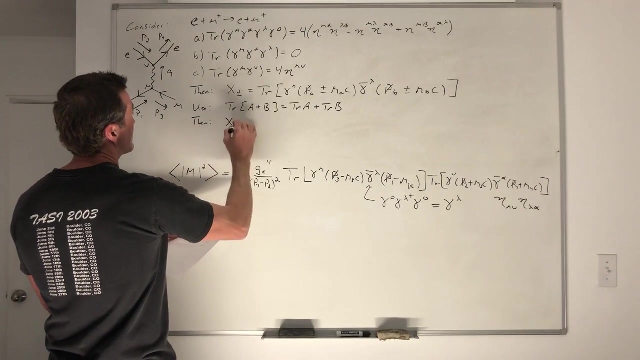 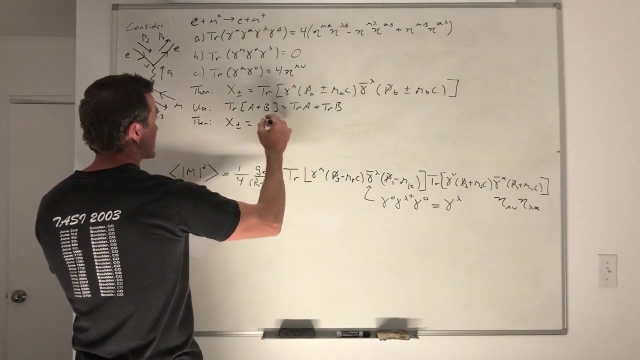 Okay, So first of all, let's use the following: Okay So the linearity of traces, And then what we're going to find is that if we multiply this out and then use this linearity, we're going to have the following set of traces: 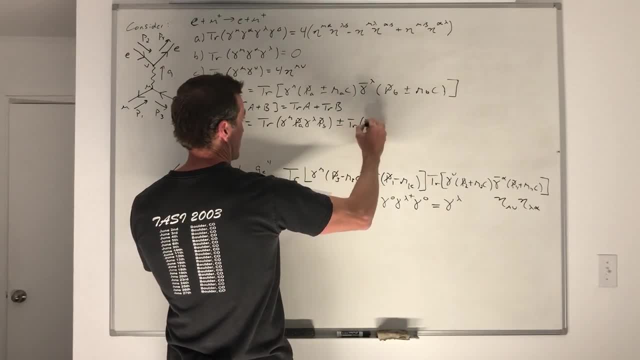 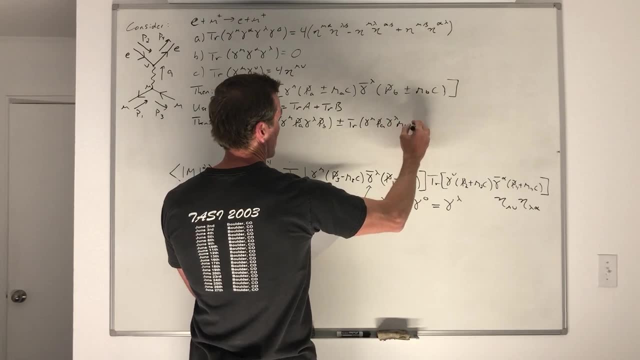 So again, I'm just going to do this. Let's put a value for this trace here, Okay? So if we calculate this thing, we're going to get the same thing. I'm going to take this all the way. 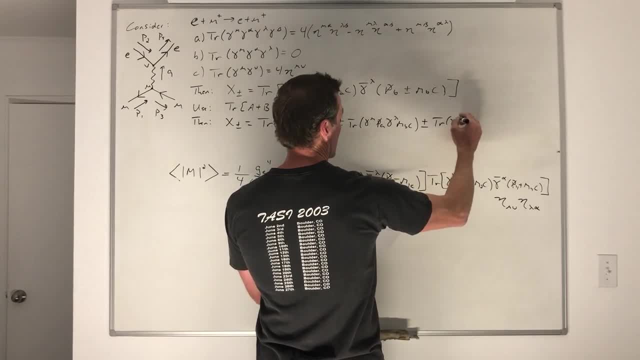 This is the same thing, but I'm going to multiply this by the value of this. So I just need to multiply this by the value of this. You're going to see where I get this from, But you can also do it this way. 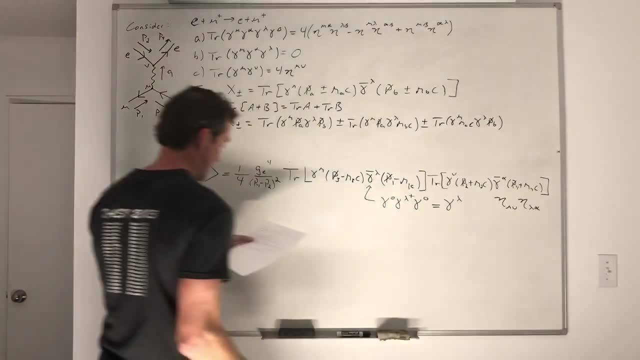 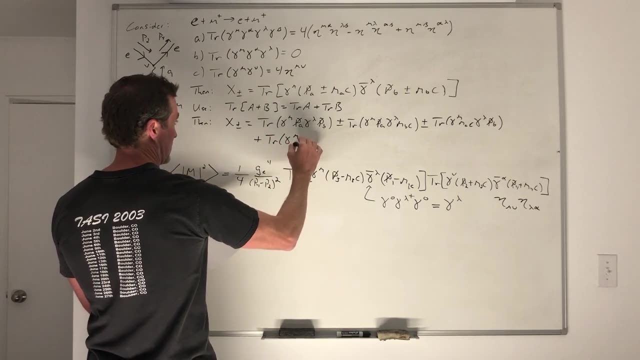 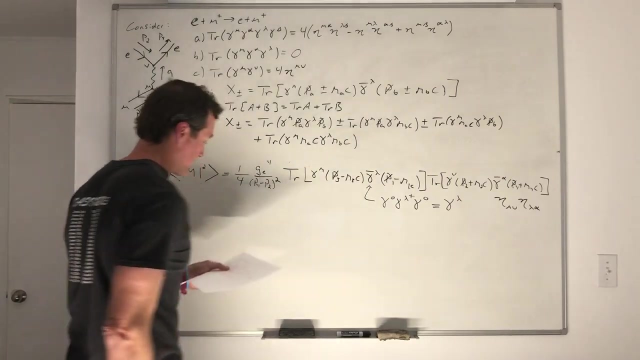 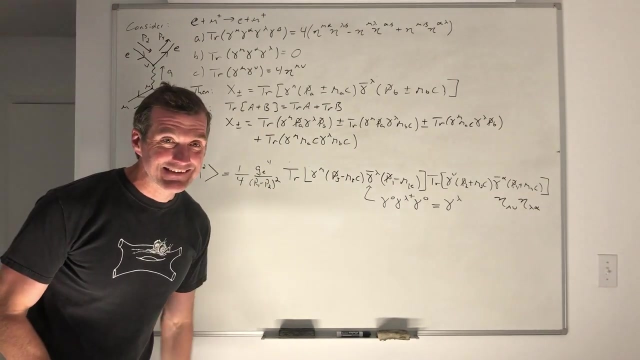 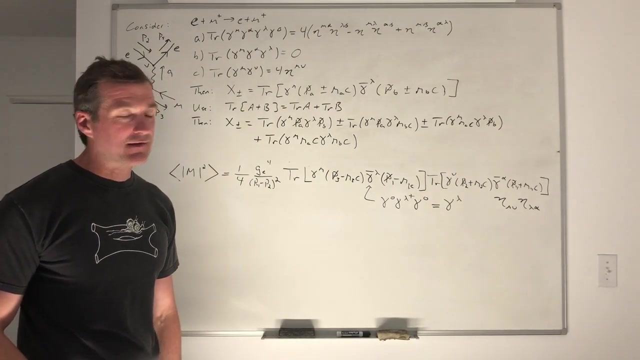 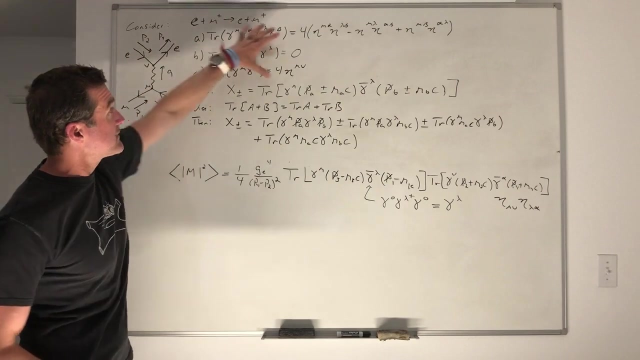 You know what I'm saying. You might say, okay, now you're ready, you ready, you ready. I hope you're ready, it's about to get good. okay, I wrote down these traces of nothing but gamma matrices. right, that's these you kind of remember working on from your homework. these are 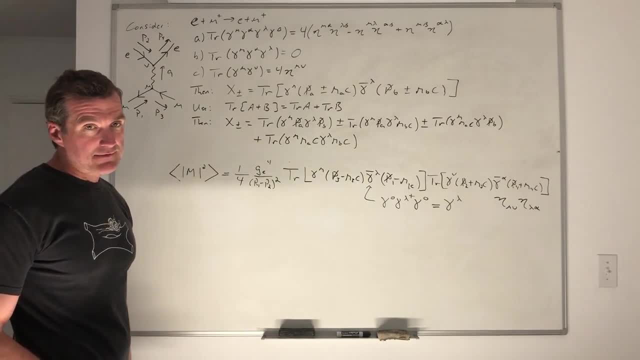 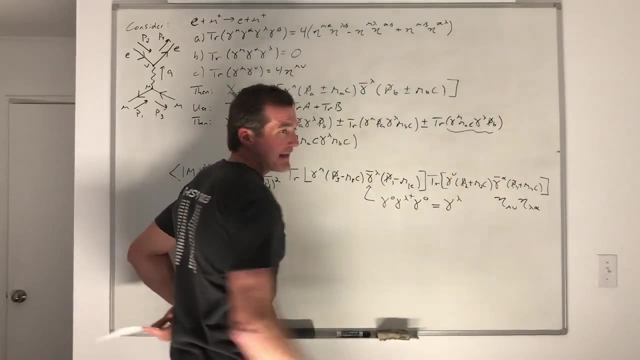 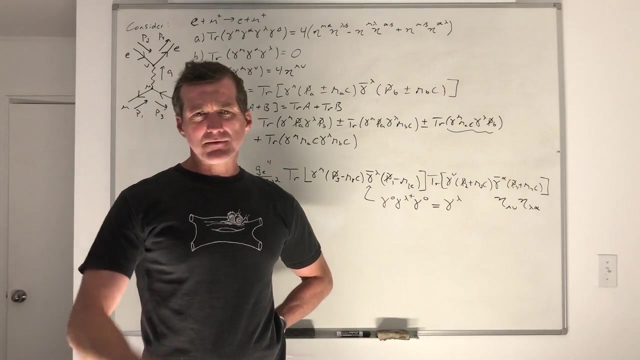 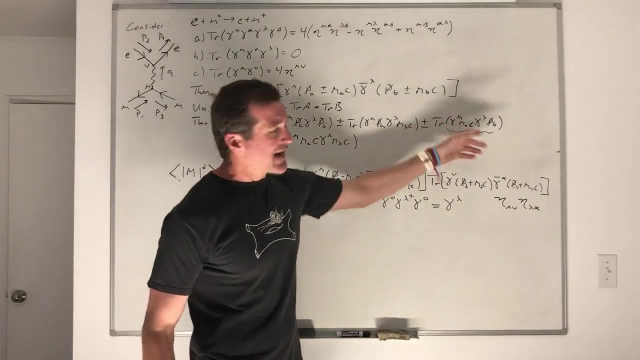 not traces of just gamma matrices yet, but let's take this one right here: ma times. C is that non-trivial and spin space? no, it's. it's completely turbulent spin space. M is a mass, C is the speed of light. that's a number. this tracing is tracing over the spin elements, so I can just pull out this Mac. 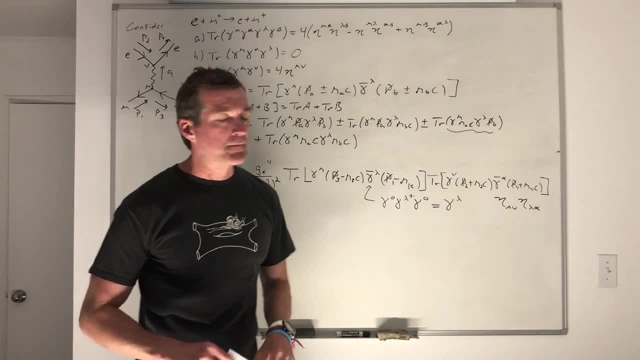 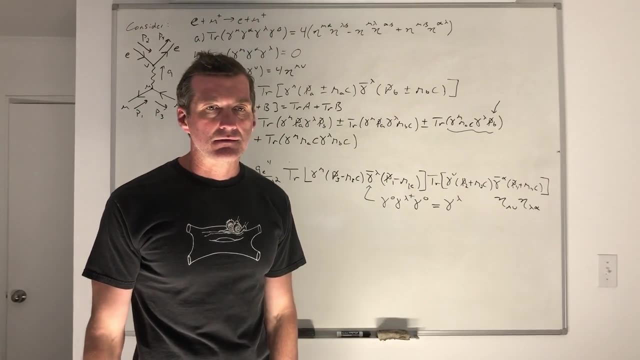 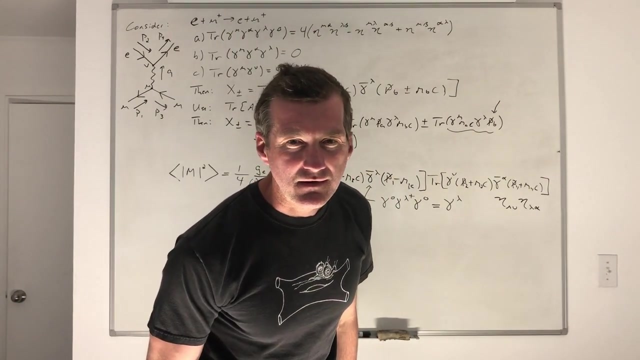 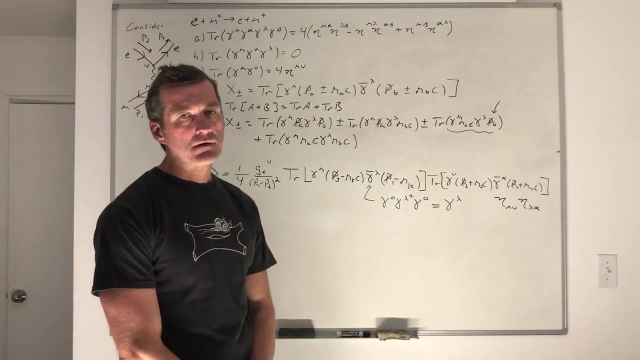 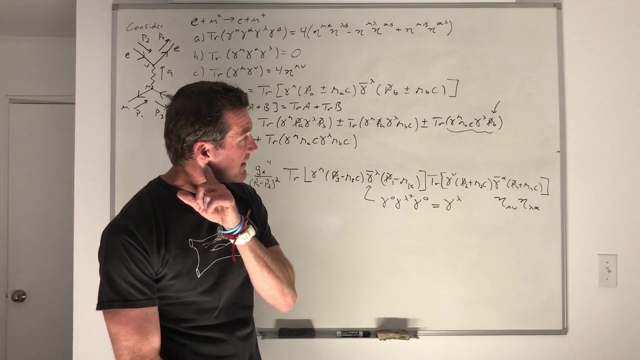 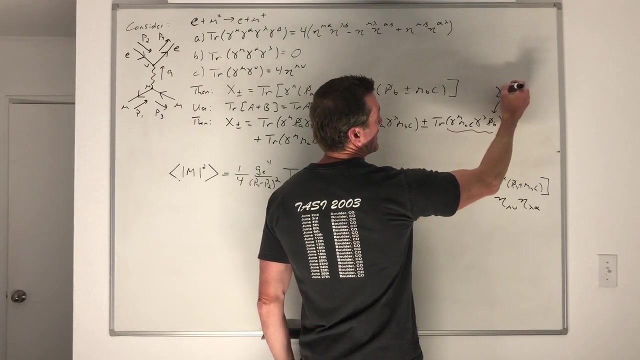 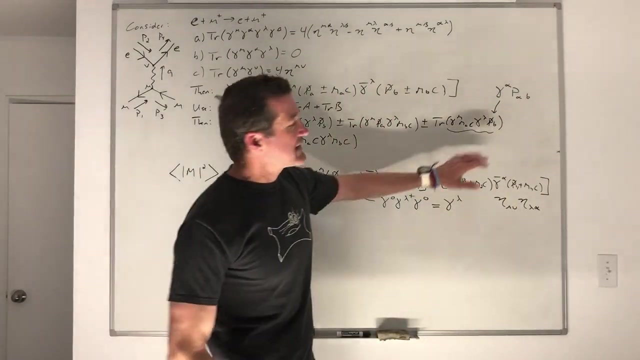 so that's gonna give me trace of gamma mu, gamma lambda. okay, well, what is P slash of B anyone? I'll pick a card in the E in here. you, yeah, you are in. what is P slash? so this was a notation I introduced last time. P slash is gamma alpha, P alpha of whatever particle you're dealing with. so this is. 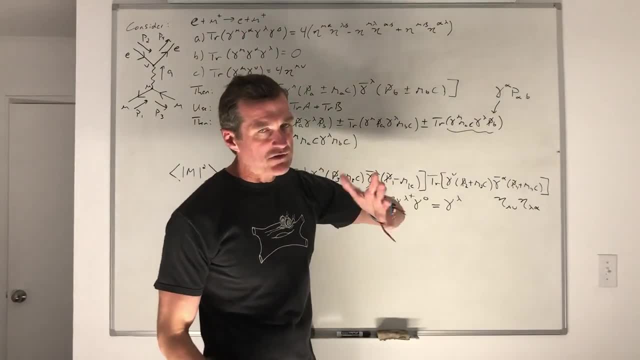 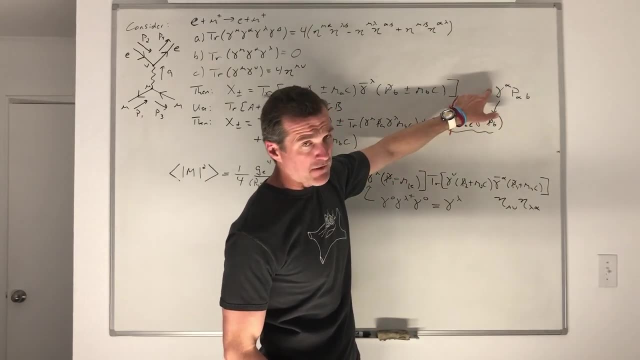 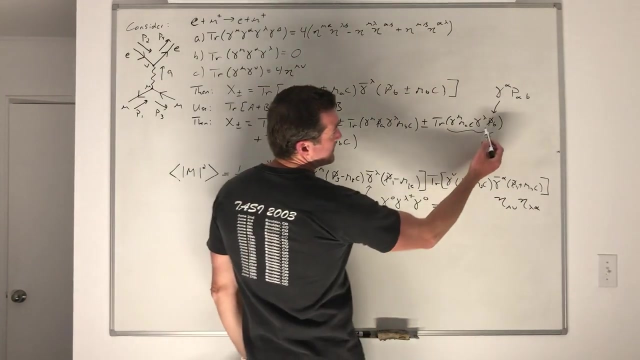 just a notation that's widely used. that's why I'm using it, otherwise I wouldn't even bother. so P slash is just that you're taking the for momentum and you're contracting it with a gamma matrix vector, and this is, of course, forming a space-time scalar. okay, so so I 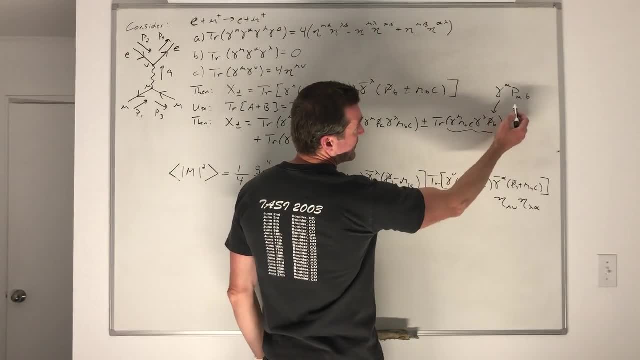 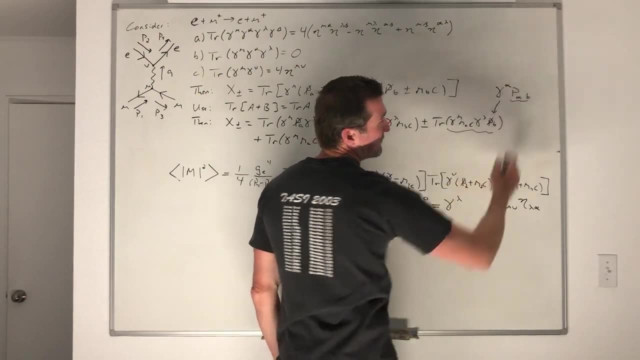 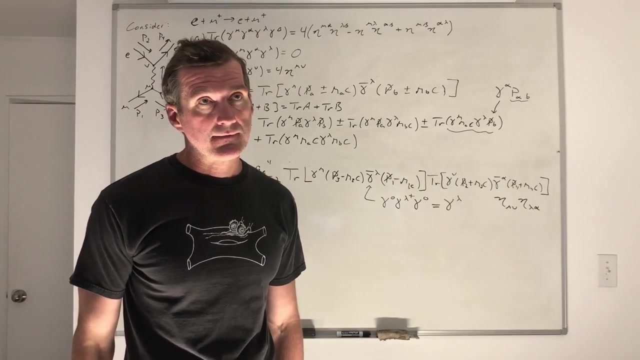 could replace this P slash with a gamma alpha. P alpha, but what and em this is a continuation of your question- is P alpha? that's the for momentum. is that trivial or non-trivial? in spin space, It's trivial, It's just a space-time-form momentum. 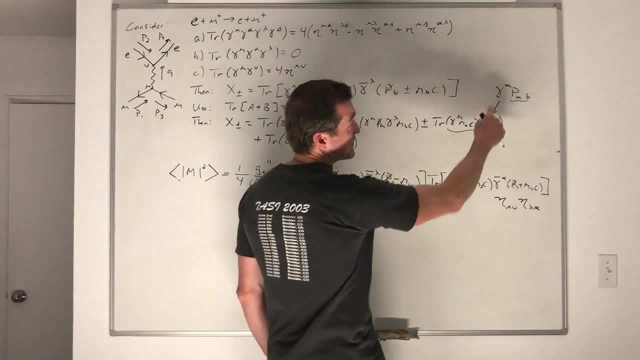 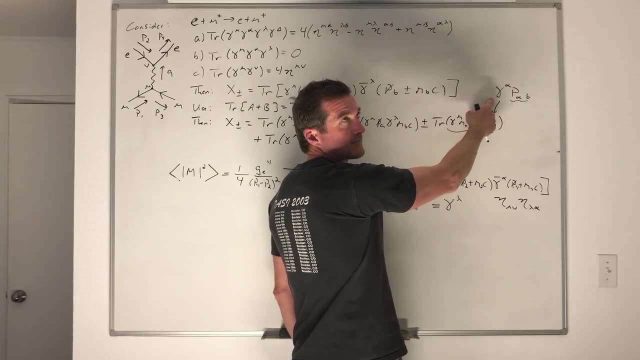 The fact that P slash is non-trivial in spin space is because it's got this gamma factor. The gamma's a matrix in spin space. You don't get less trivial than that. Okay. but what's important is just like we could pull M A times C. 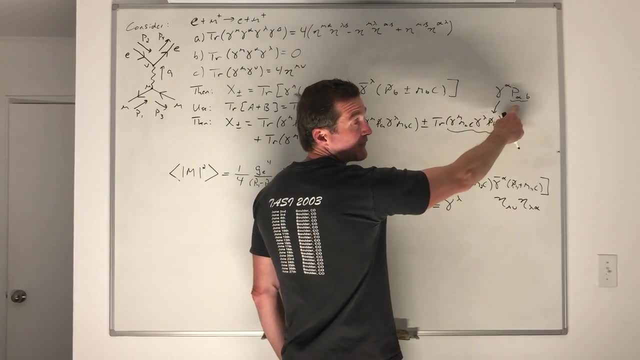 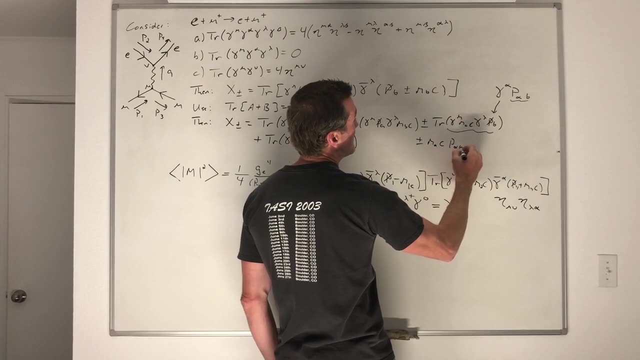 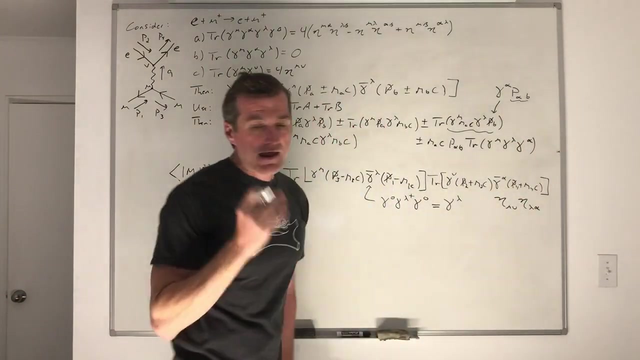 outside of the trace. we can also pull P alpha beta out of the trace, which means that this term is going to end up being M, A, C, P alpha B. trace of gamma mu, gamma lambda, gamma alpha and- oh my gosh. 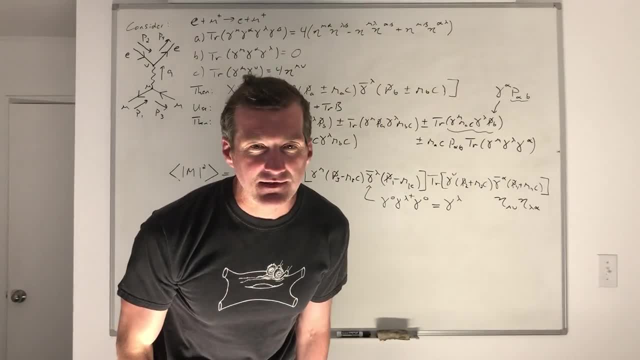 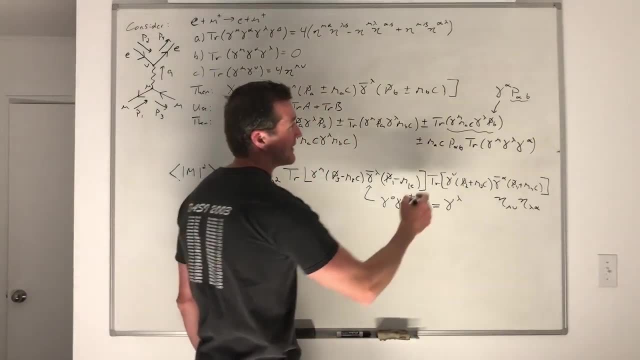 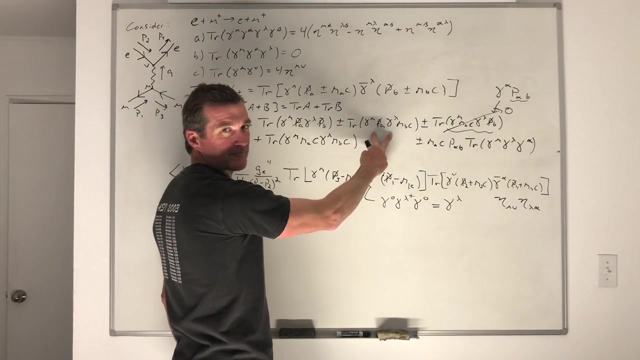 who's going to have to answer this one, Danny? Are you there, Danny? Danny Moore, Yeah, it's zero. Boom, This is zero. What about this one, Danny? That also is probably zero. Yeah, so this is something you want to get used to. 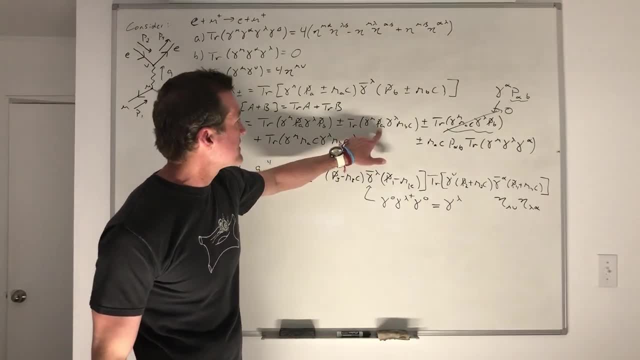 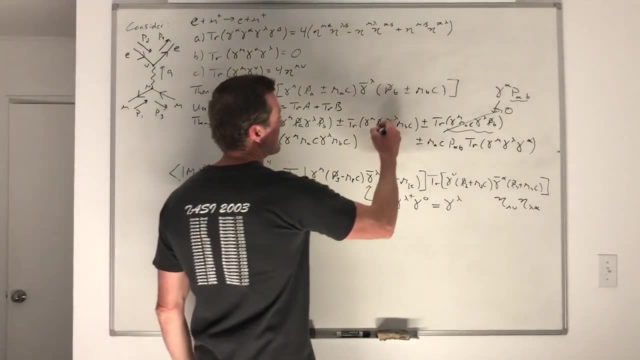 Every slash that appears is going to give you another gamma matrix. So you've got a gamma, a gamma, you've got another gamma from the slash, that's three gammas. all the other shit comes out. so this is going to give you zero as well. 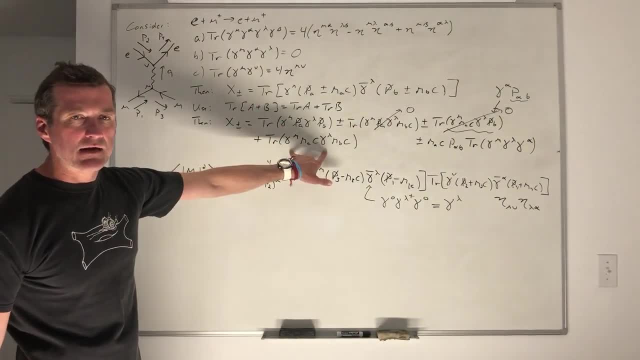 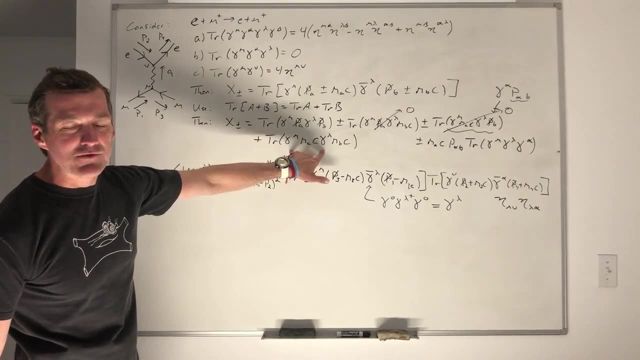 Okay, How many gamma matrices sit in here? And I'll give you here- I'm pointing at both of them- How many. Two, Two. You're all flashing peace signs at me. That's so cool. Peace, All right. 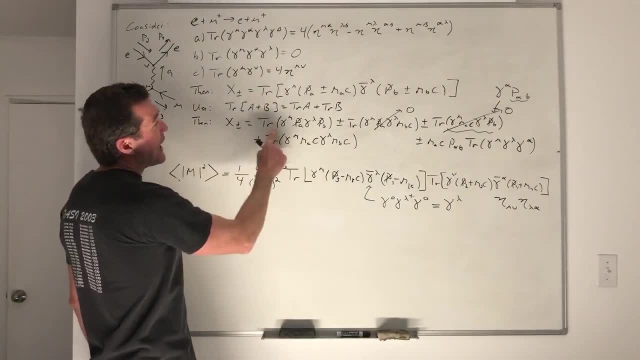 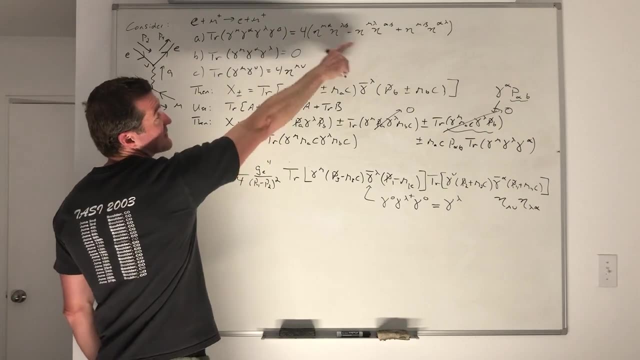 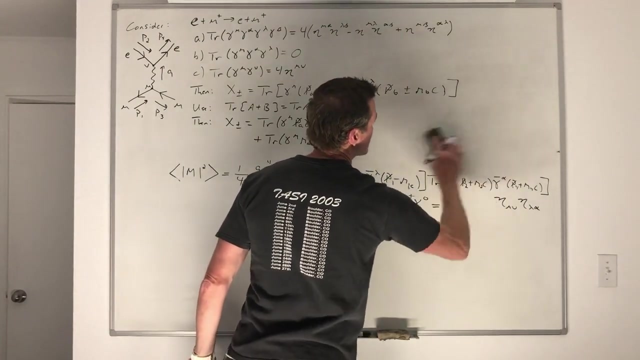 Yeah, so this is two. That's going to use this. How many gamma matrices are sitting in here? Four, So that's going to make use of this. Okay, So let me clean up this shit. that's zero. Who needs to keep in touch with that? 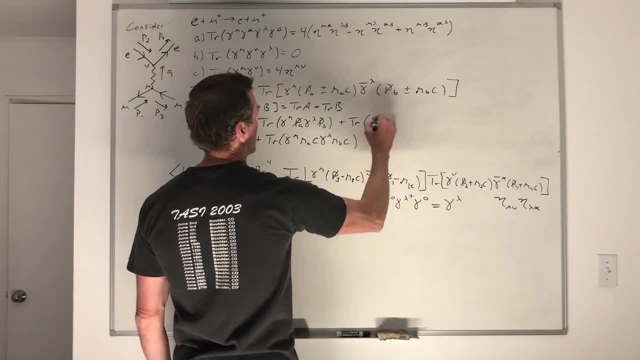 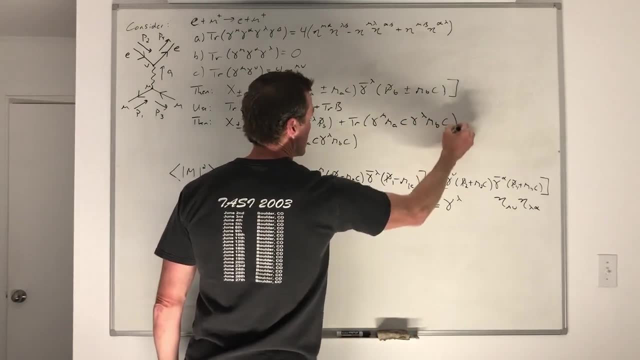 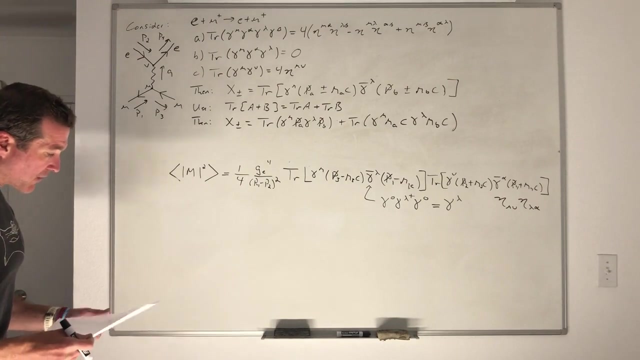 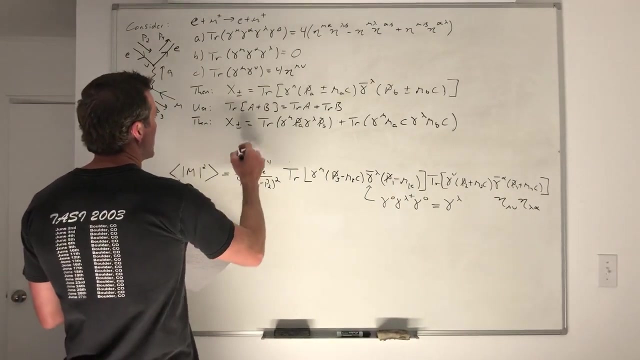 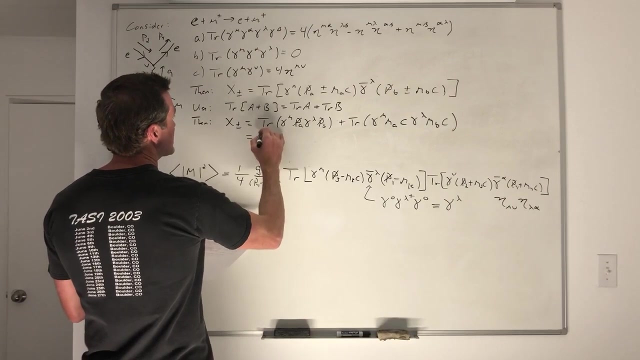 Let me bring this up. Here we go, Here we go. Let's see, Got a little bit of room, So let me clean this up. We're going to clean this up, So we're going to PAPB. Sorry, 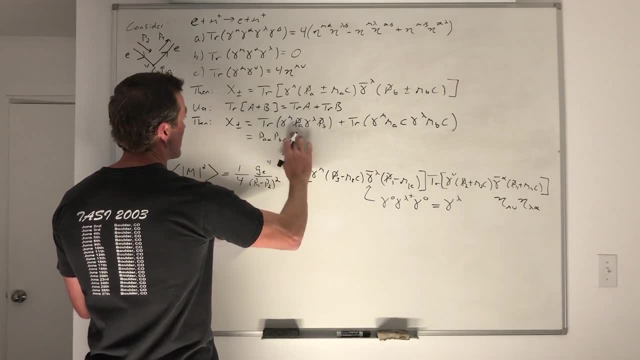 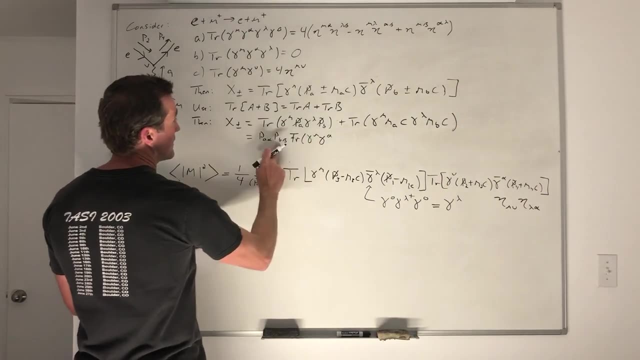 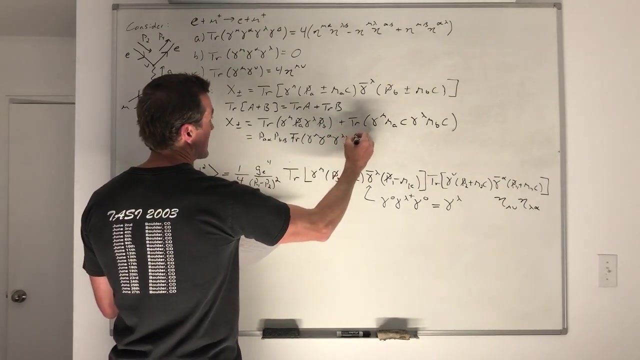 PA, alpha, PB, beta times, the trace of gamma mu, gamma alpha or gamma lambda, sorry. And then we have the PB, which has got the index beta, So we're going to have gamma beta. Okay, Notice, I'm getting the indices in the correct order. 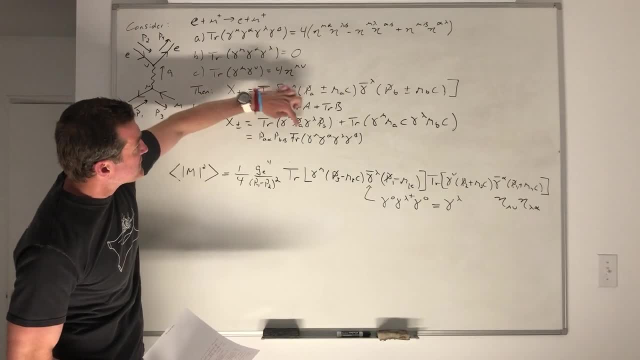 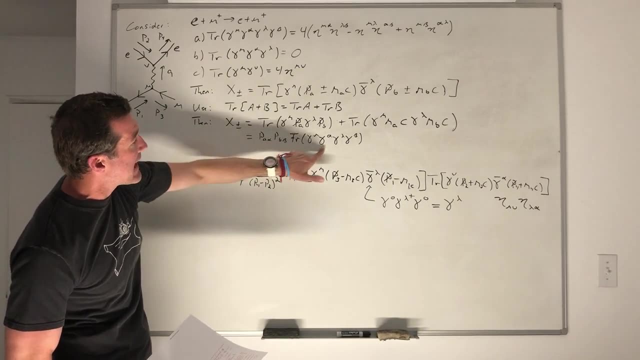 because it matters, Order really matters. So the gamma mu is the first gamma matrix. Then I had P slash of A, which I gave this an alpha subscript. So the gamma matrix here should have an alpha. And then I have gamma lambda. 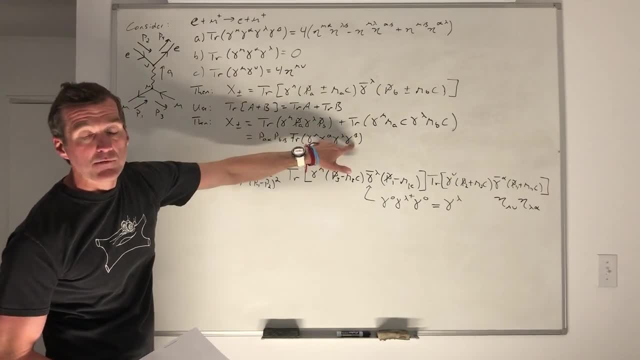 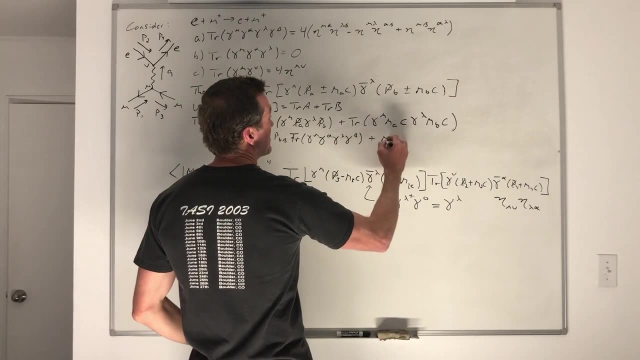 And then the PB. I gave an index beta, so I should give that gamma matrix an index beta. Okay, That's all I'm doing. I'm being really careful, All right, All right. And then over here we have plus M. 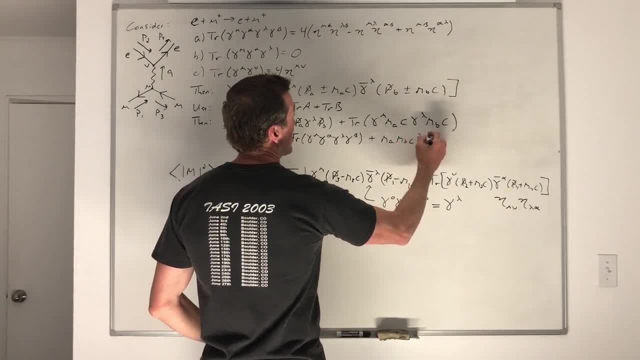 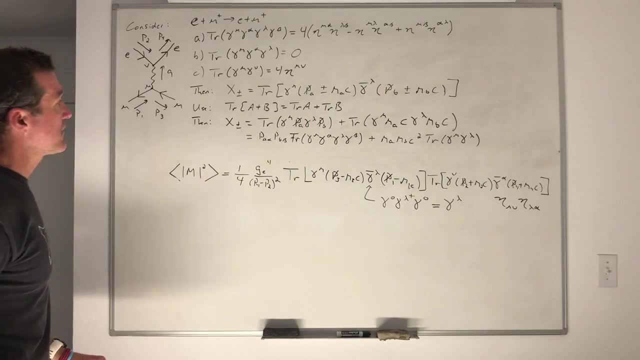 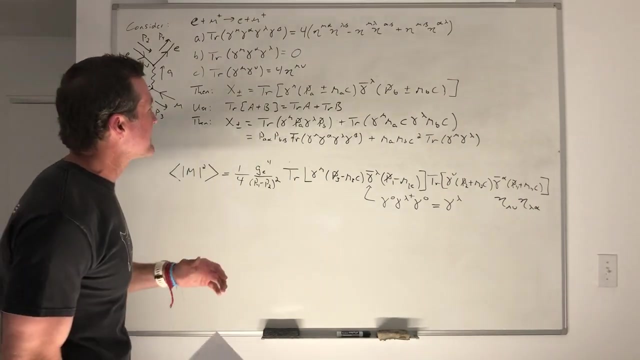 M, A, M, B, C, squared trace, gamma, mu, gamma lambda, Okay, And you might notice something really interesting. Well, it's not that interesting. I find it super interesting, but you don't find it that interesting. 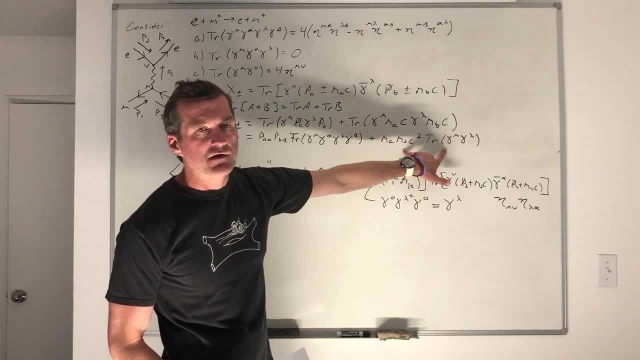 What's the total index space-time index structure of this term? It's a scalar, Oh no, no, it is. Oh no, it's a tensor. Sorry, it's a tensor, Yeah, and what rank is it? 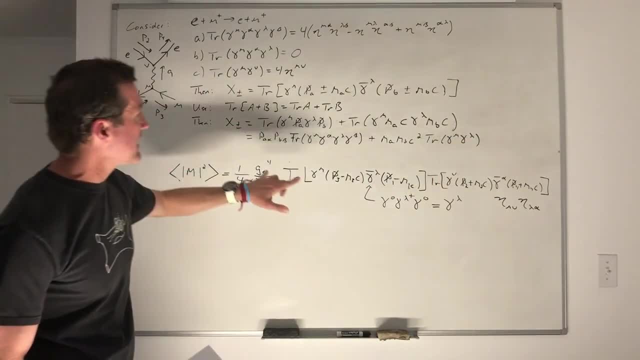 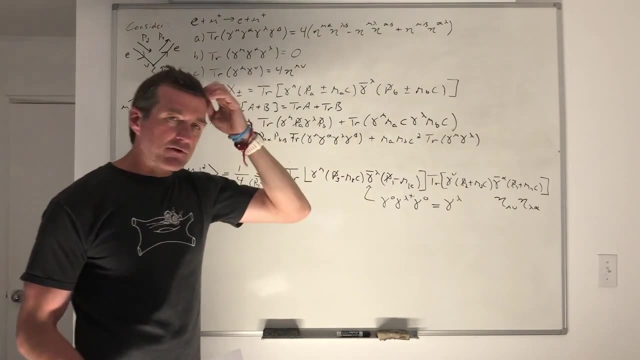 Rank two? Yeah, because it's a gamma mu nu and a mu lambda index. What about this one? That's also rank two in space-time? Yeah, if you're adding them together, they have to have the same tensor structure. But notice, the alphas get summed over, the betas get summed over. 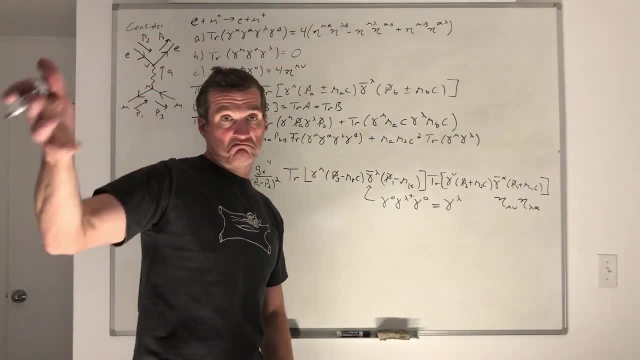 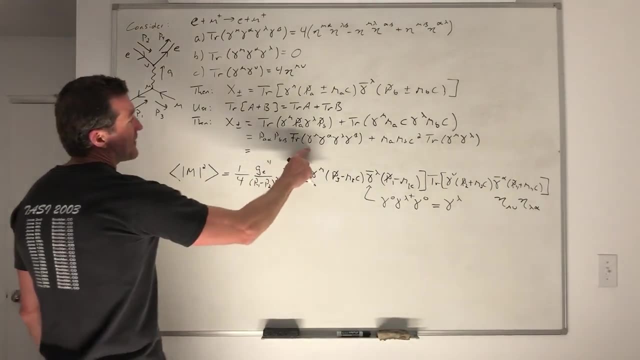 so this is just left with an overall upper mu lambda. Okay, I'm just pointing out the consistency of what I'm doing. Well, let's do it. So I'm going to replace this by that, and then I'm going to replace this by this. 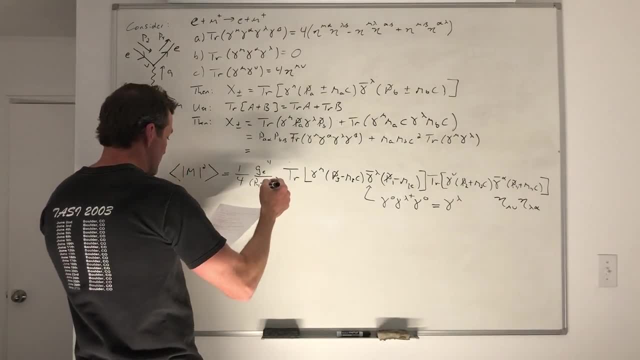 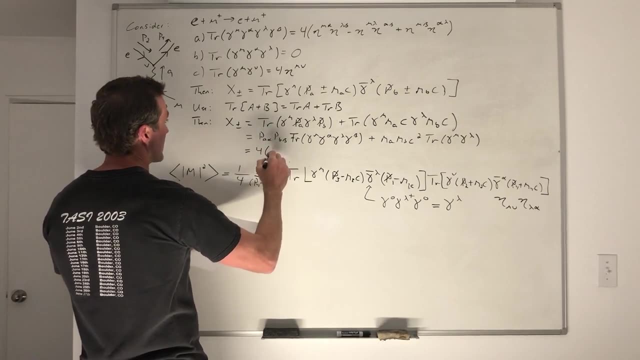 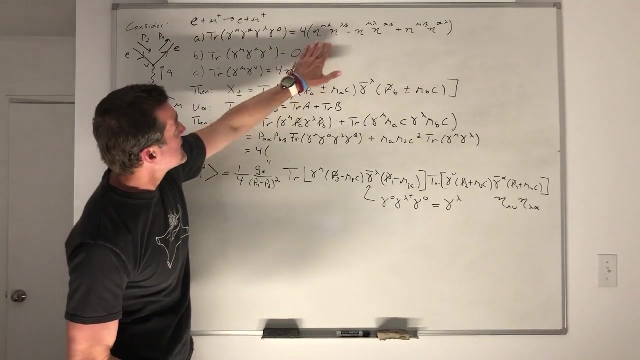 and that's going to leave us with the following: Okay, here we go. Now. I want you to notice what I'm going to do: Instead of writing down this eta and this eta, I'm just going to take this eta and this eta. 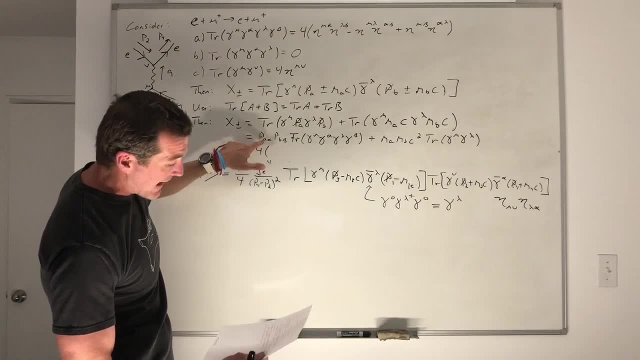 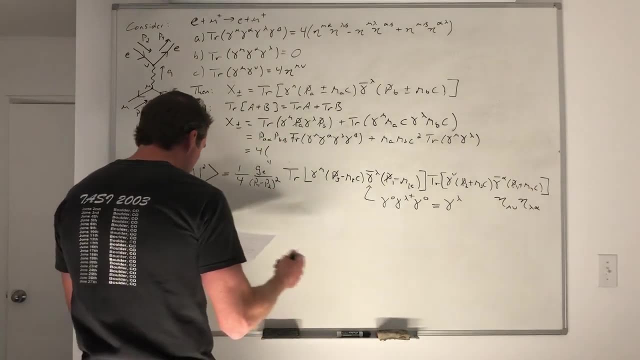 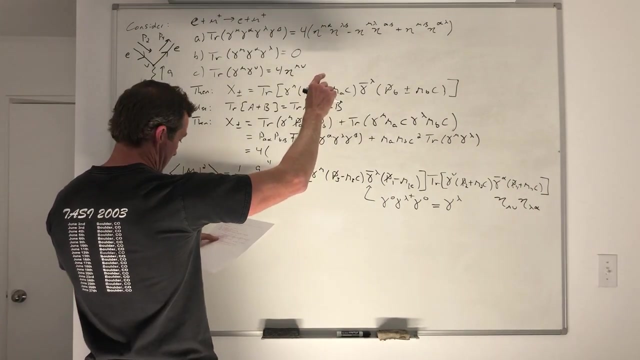 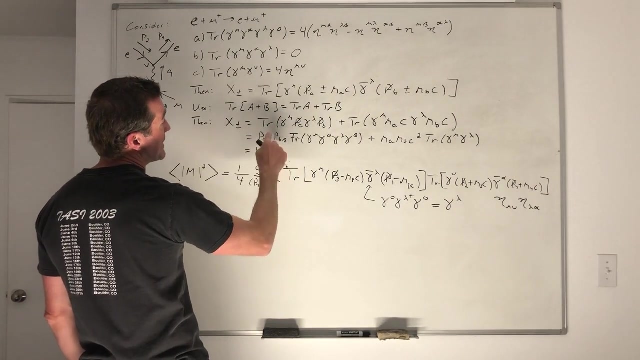 and I'm going to use it To contract the indices of these terms. Okay, So you'll understand what I'm doing in just a second. So, first of all, so the eta mu alpha grabs this alpha index and raises it and makes it a mu index. 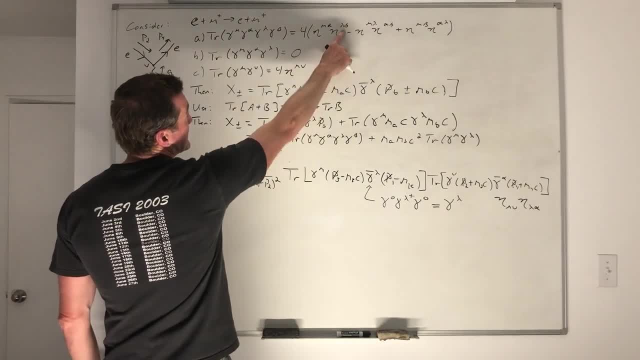 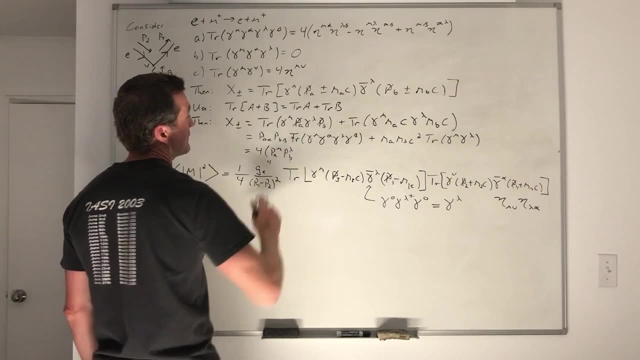 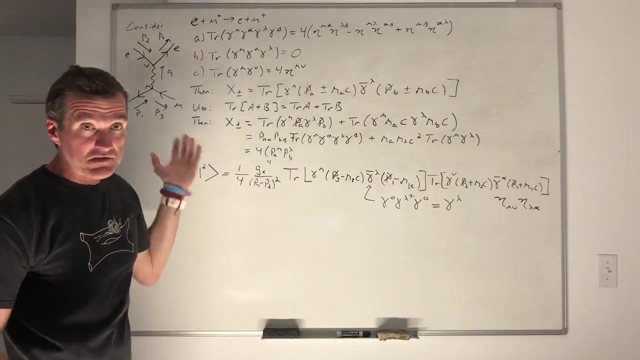 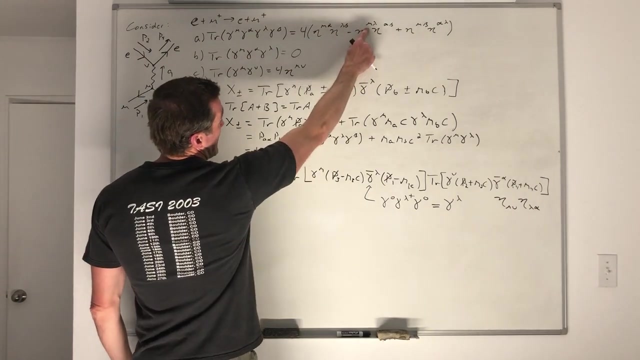 so this becomes P A mu, And then this guy, the beta here, grabs this beta and raises it and leaves a lambda. Okay, So that's how this first term contracts with the two momentum factors. Does that make sense? So now, if I take the second term, this grabs the oh wait. 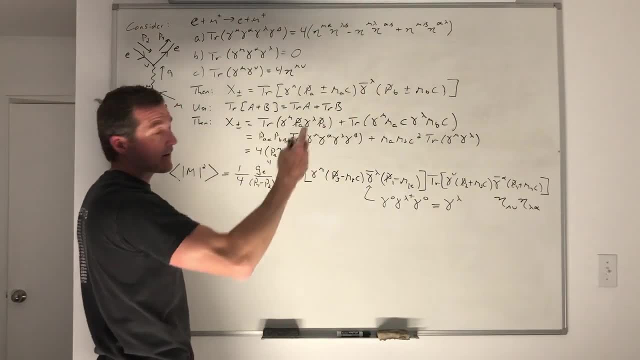 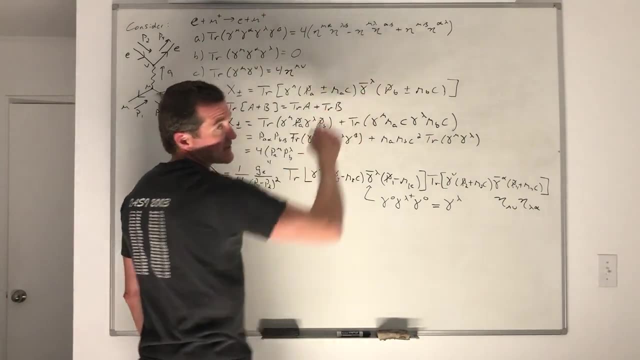 this one doesn't do anything, because this is eta mu lambda. There's no mu or lambda here. The second one, though, takes the alpha and the beta, raises one of them and turns them into the same thing, so they're summed over. 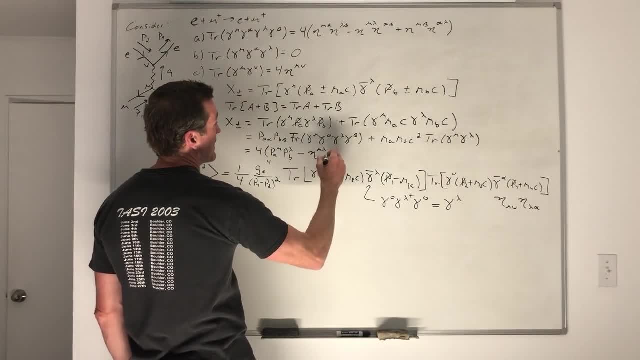 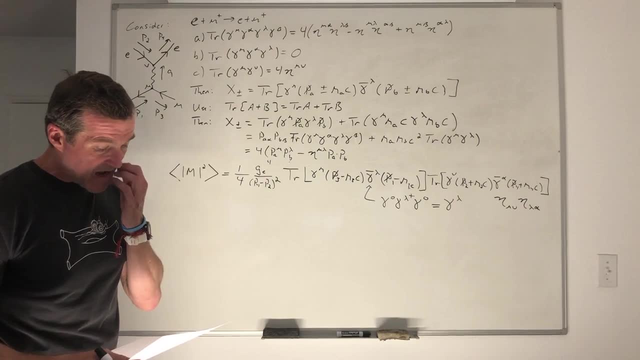 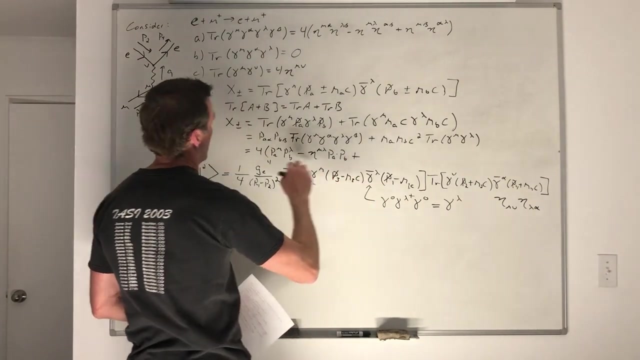 So this becomes: eta mu lambda times: P, A, P, B. Does that make sense? Okay? and then the last one is going to give us. we're going to grab the alpha, turn it into a lambda, Okay. So this is the alpha. 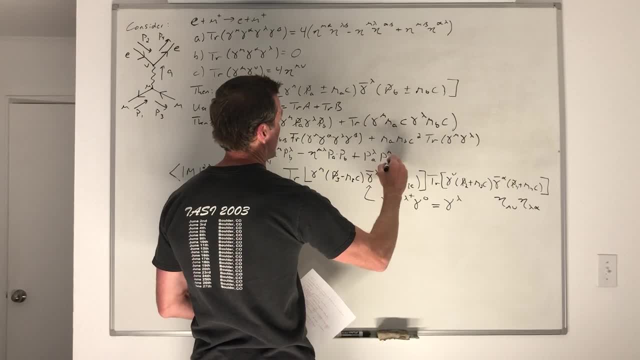 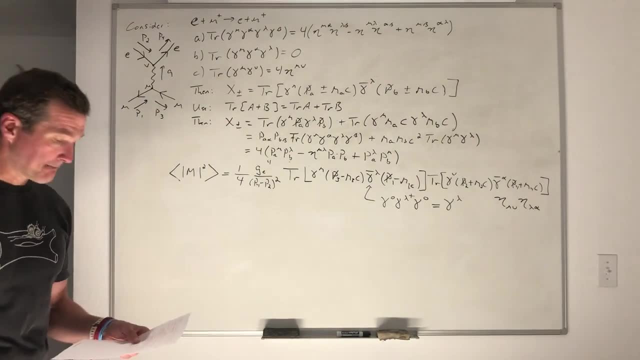 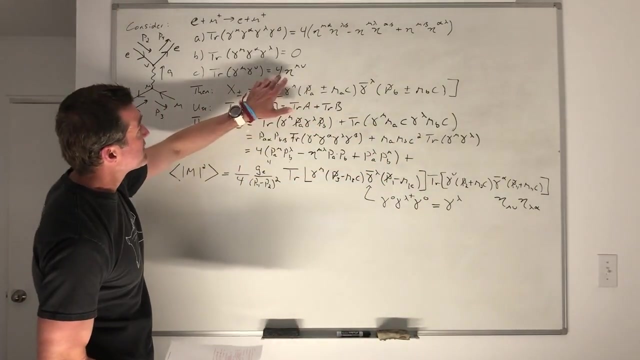 This is the mu, This is the beta, This is the mu And the b. turn it into a mu. Okay, not that bad. And then we're going to have for this guy, we're going to replace the trace for 4 times the matrix. 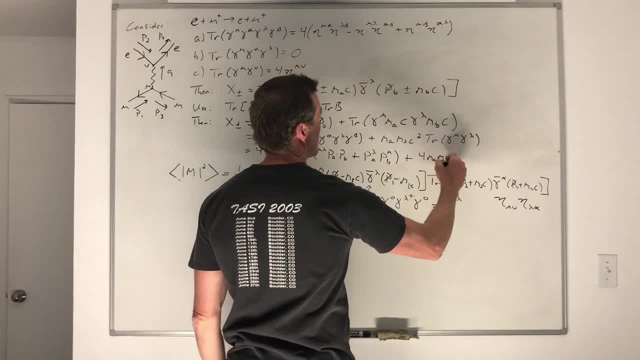 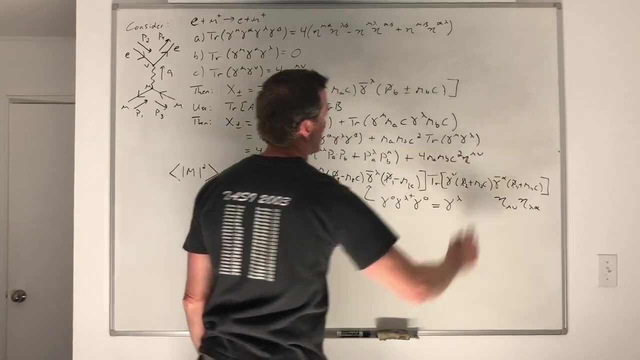 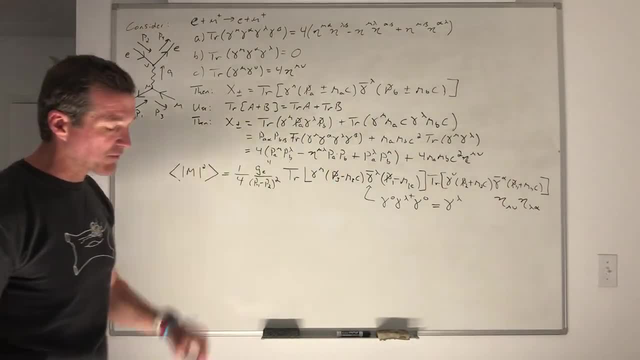 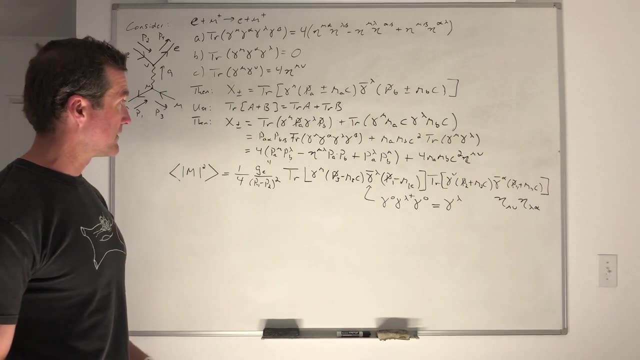 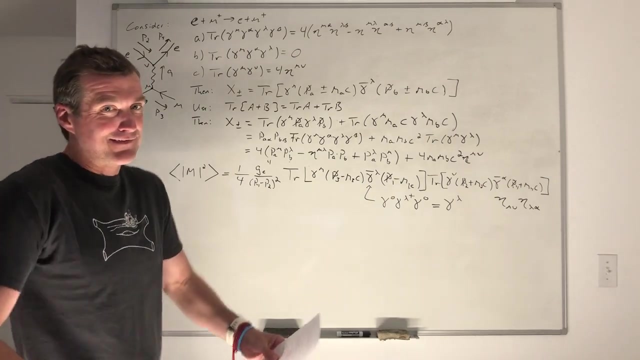 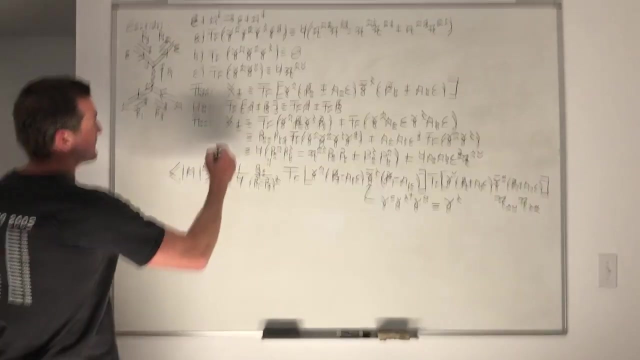 No problem, Thank you, Bye. Thank you really should be saying inverse metric, because the metric with two upper indices is an inverse metric. Okay, how are we doing? We're doing okay, Sort of Kind of: Eh, maybe, Maybe it's okay, I don't know, Possibly, okay, All right, all we want to do. so now we have this x plus or minus factor. 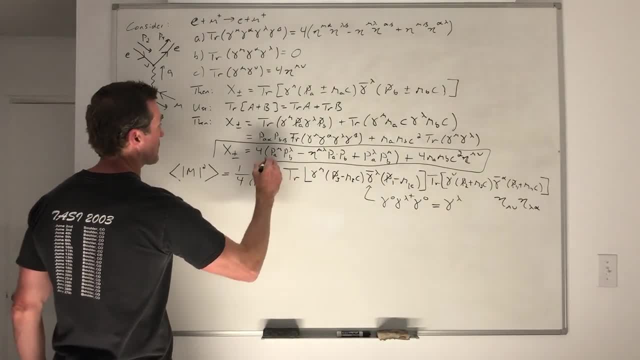 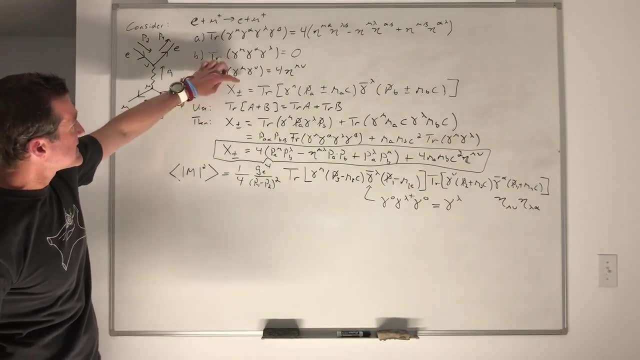 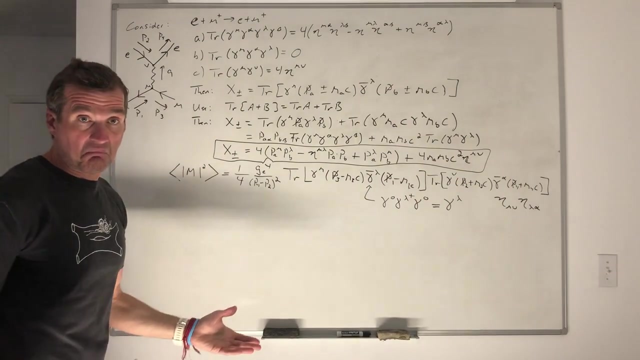 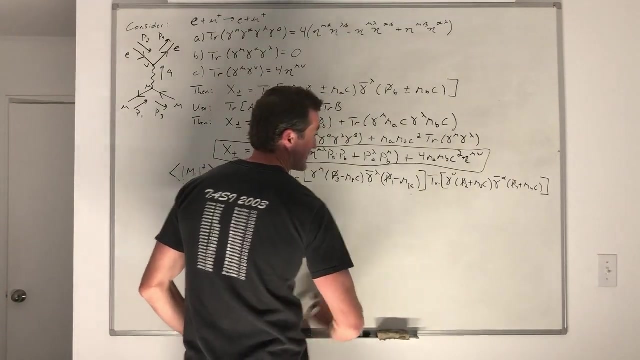 And remember what x plus or minus is. It's just what you're going to replace the trace of the product with, and we've got two of them here. Okay, So if we apply the trace, whoops, I didn't mean to erase those latitudes. 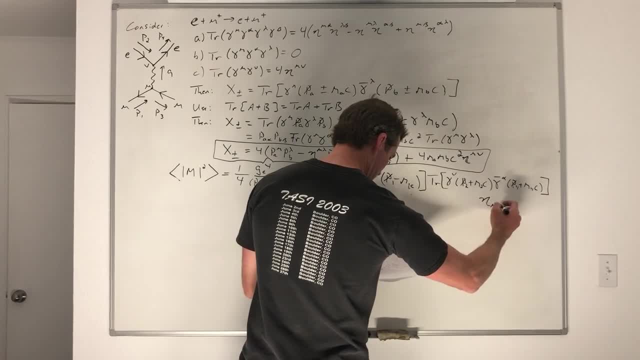 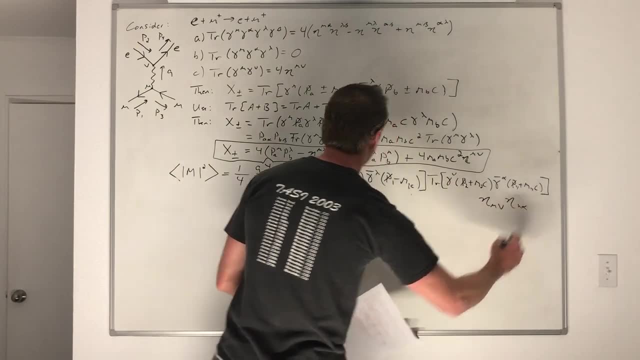 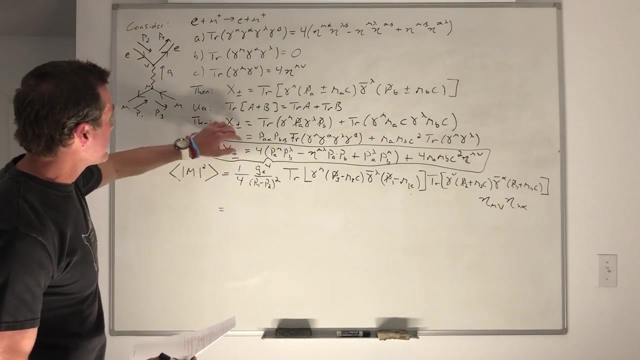 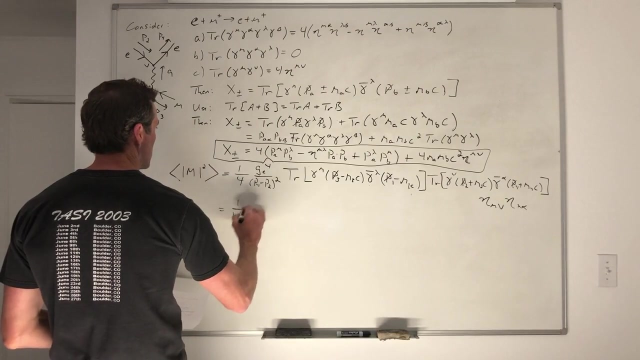 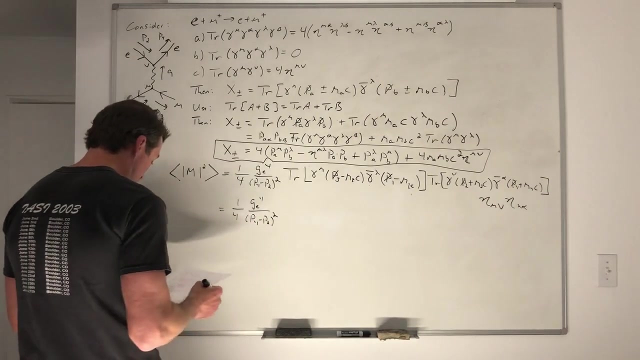 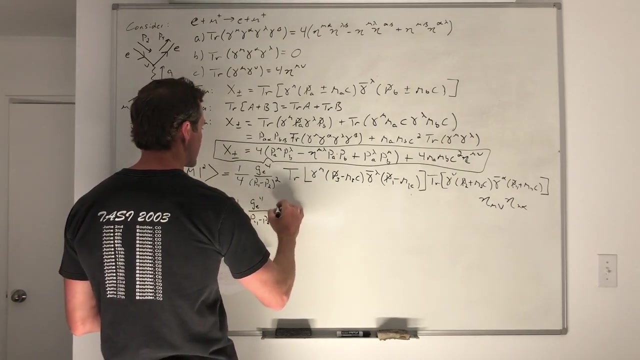 Um, Okay, So now I'm just going to plug x minus in for this one and x plus in for this one. So here we go. I can do this: Two factors of 4, so this is going to give me a factor of 16.. 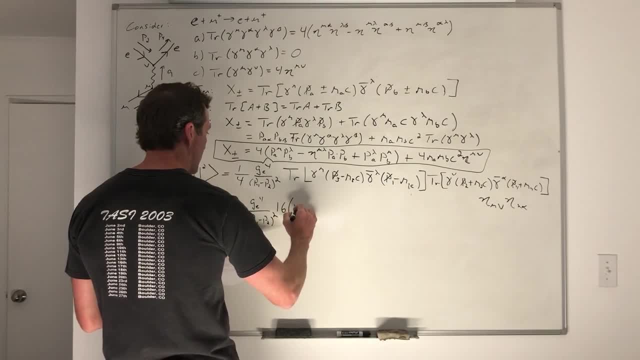 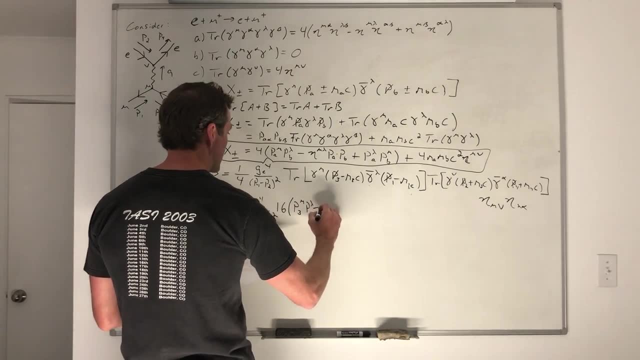 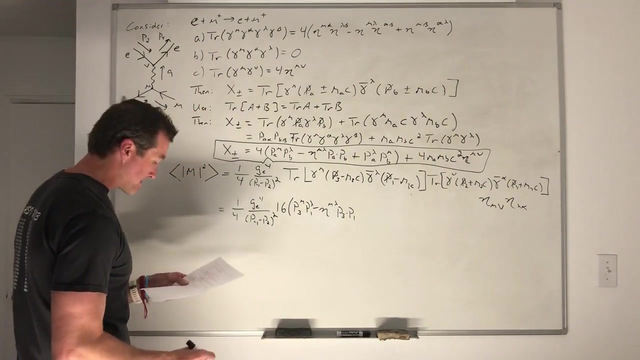 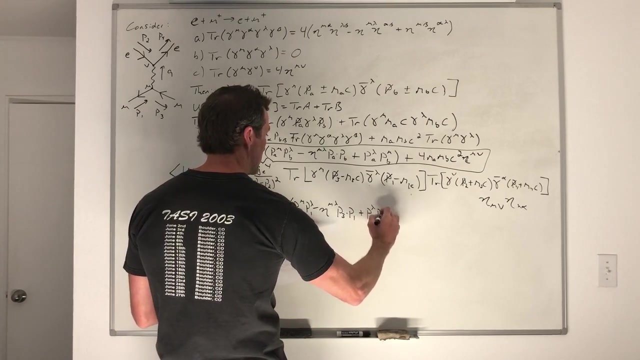 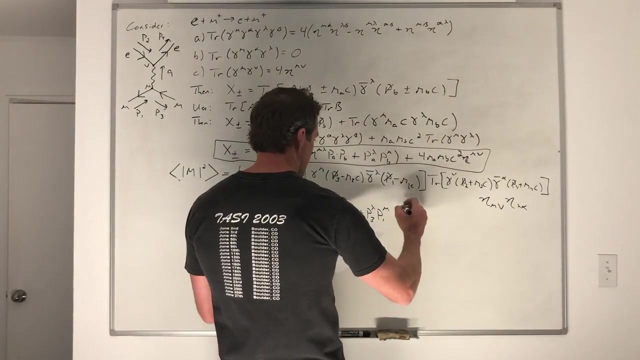 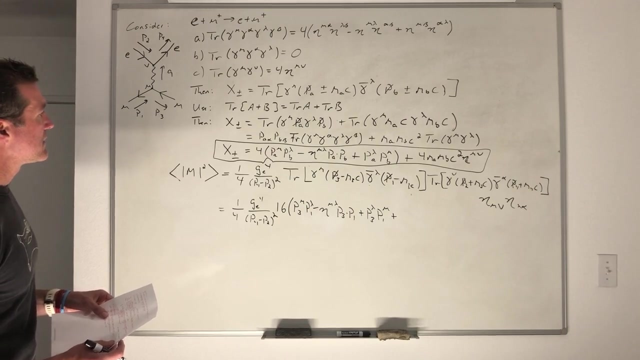 And then I'm going to have p3- mu, p1 lambda minus eta mu lambda, p3 dot, p1.. Okay, Plus p3 lambda p1.. Okay, Plus p3- lambda p1- mu plus mamb. So this is 1 and 3.. 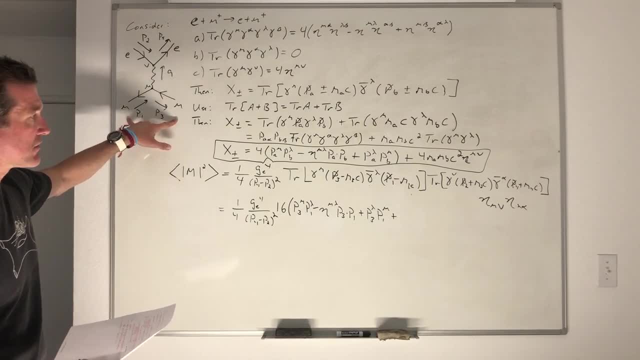 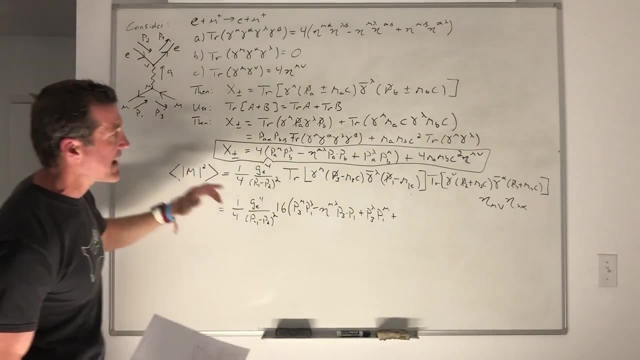 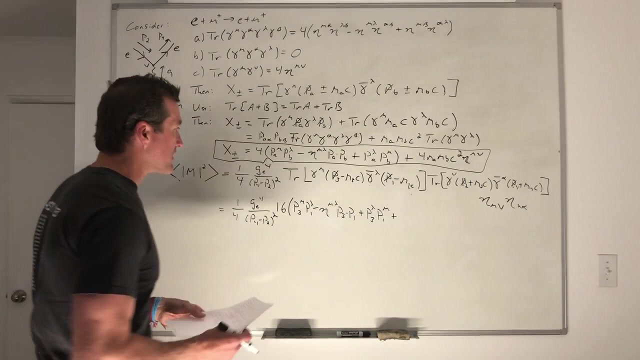 Oh, the mass that I should be working with is the mass of mu. Okay, Because these are the momentum 1 and 3.. That's following the mu line or the anti-mu line. They have the same mass. So the mass that I put in here is the mass of the mu line. 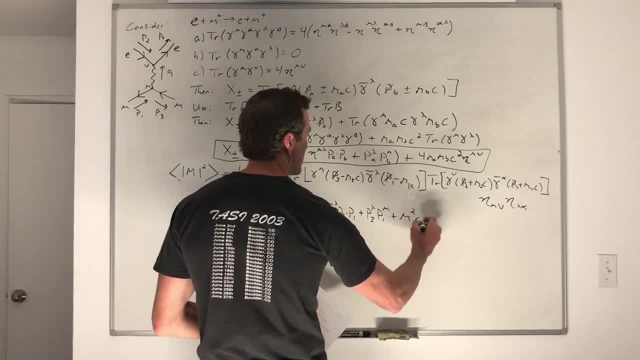 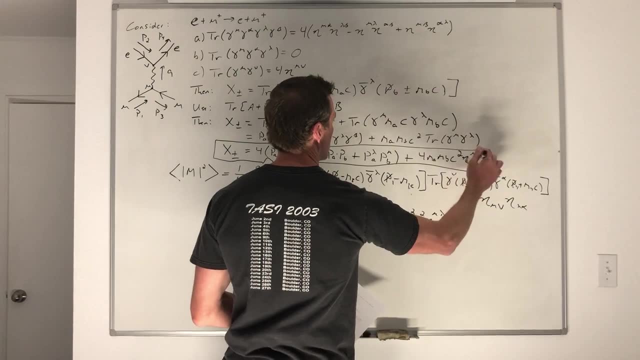 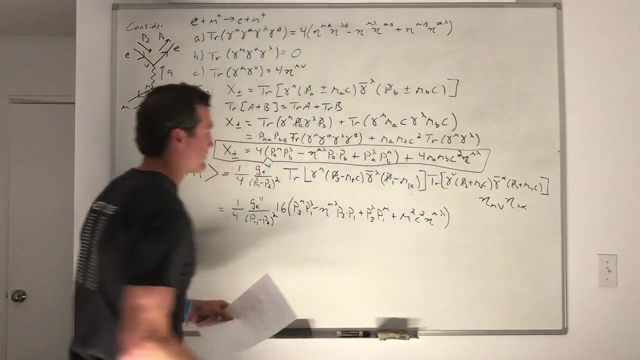 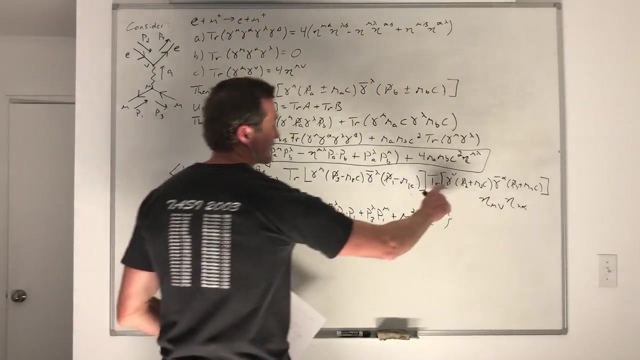 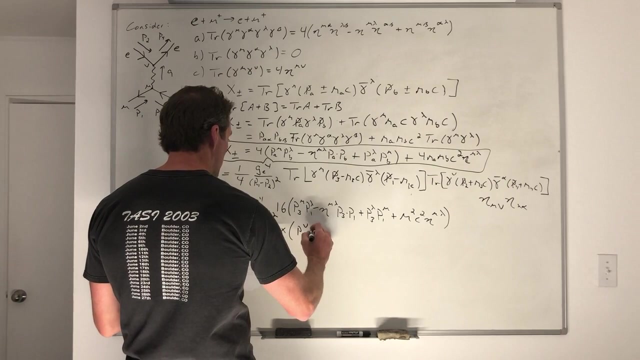 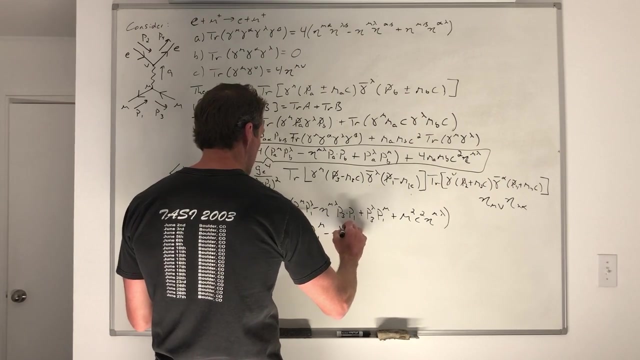 So we're going to have mu squared, c squared, eta mu lambda. This should be a lambda, Okay, So that's replacing the anti-particle terms, And then we also have a factor for these terms, And the factor for those terms is going to be p2, mu, p4, mu minus eta, mu, alpha, p2, dot, p4.. 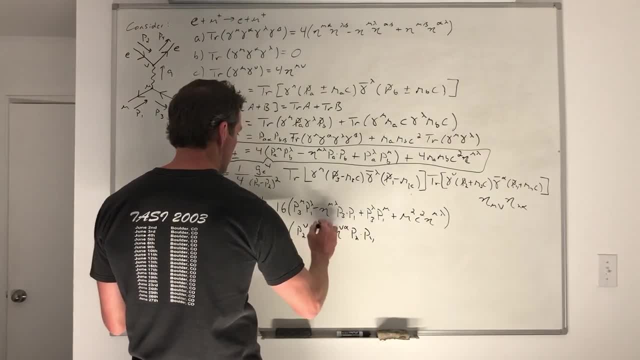 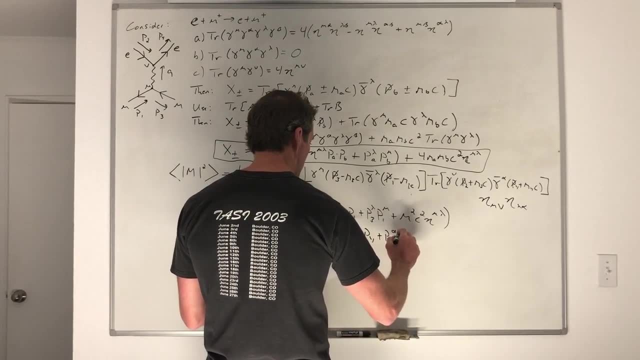 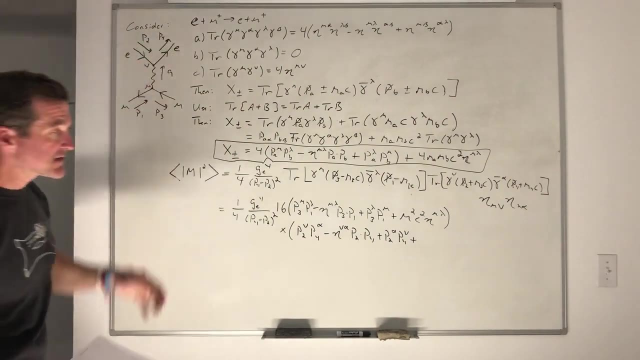 And that is totally wrong. This is an alpha, not a mu, Sorry about that- Plus p2, alpha, p4, mu plus. And now the 2, 4 line is associated with an electron, So we're going to use the electron mass. 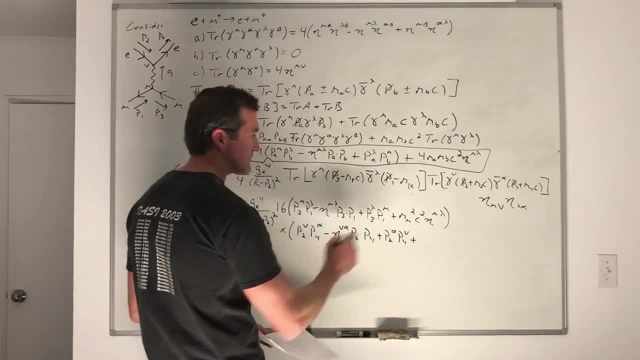 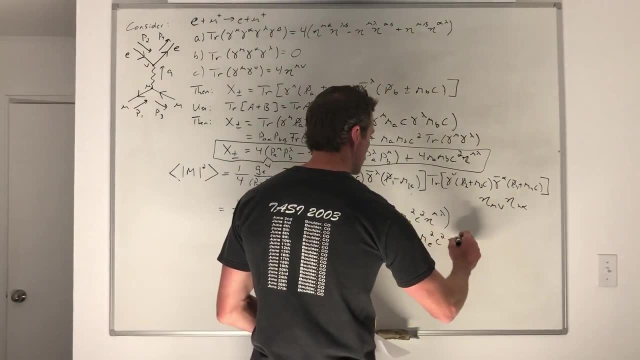 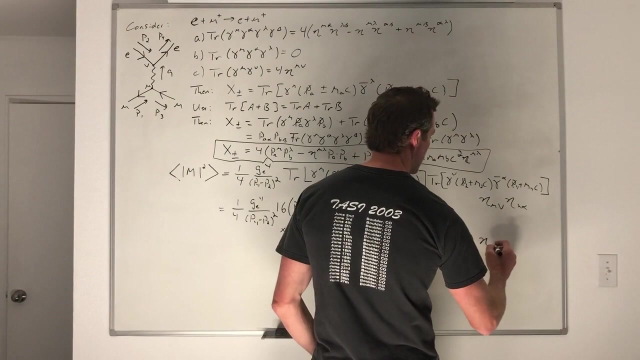 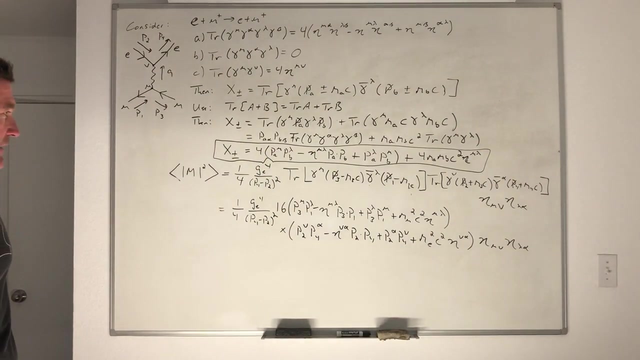 Sorry, This should not be mu squared, It should be the mass of mu squared. And then this is the mass of the electron squared: c squared, eta, mu, alpha. Okay, And then we've got our little outstanding metric factors. Looks pretty good, doesn't it? 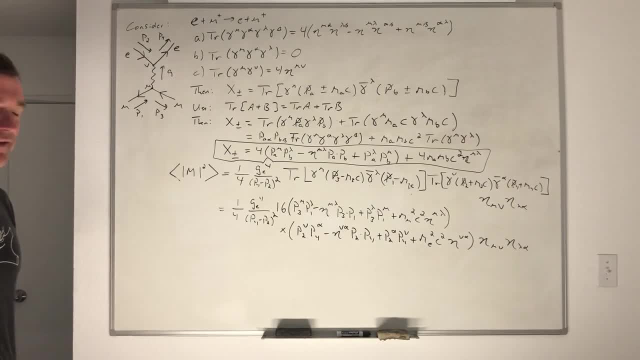 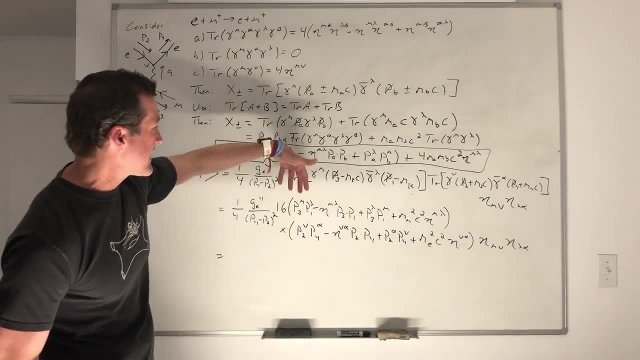 Doesn't it? No, it doesn't. It doesn't look that good. It's pretty damn ugly, to be honest with you. Okay, So now all I have to do is I have to take this 4-component thing and multiply it by this 4-component thing. 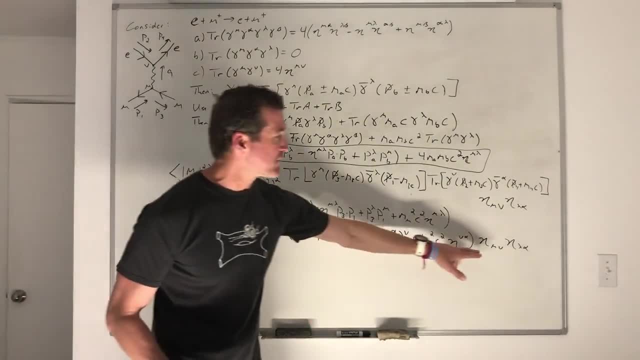 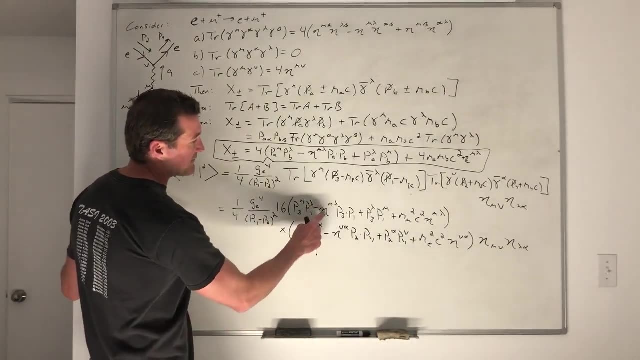 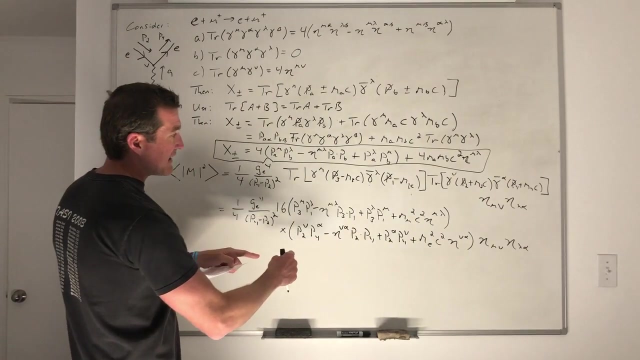 Then I have to sum over all of the indices applying these metrics, which you know, notice they'll do interesting things, Like this metric factor, this inverse metric factor, with this metric factor, is just going to give me delta, lambda, nu, which is going to take the lambda and the nu and make them the same everywhere. 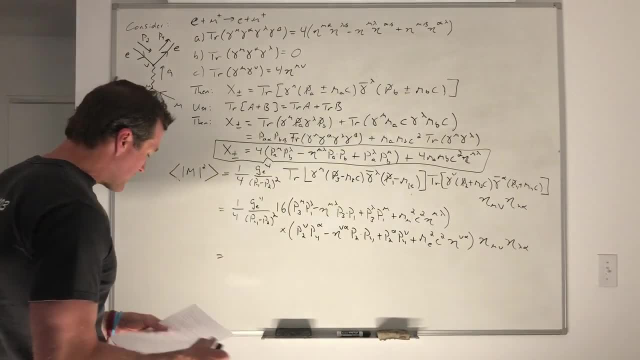 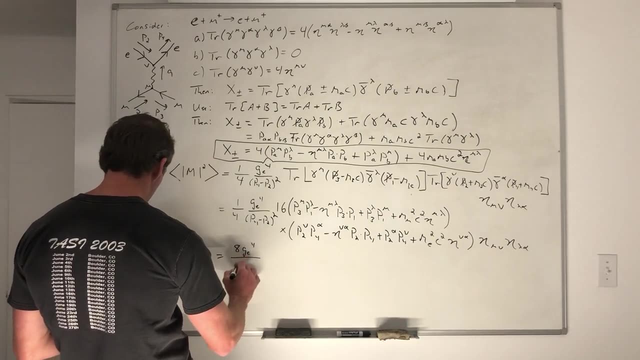 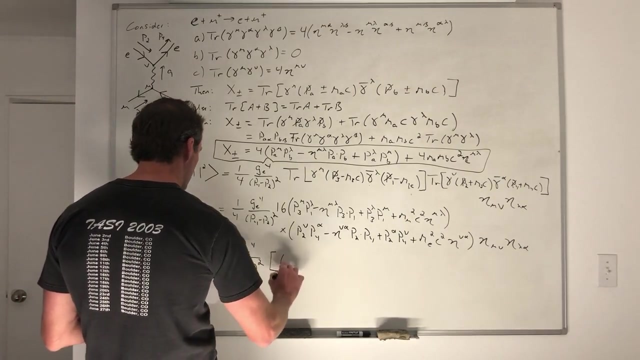 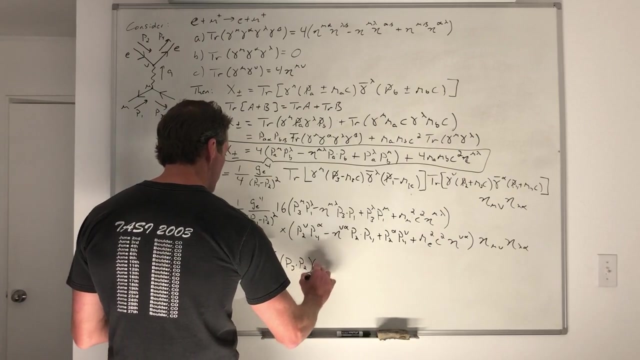 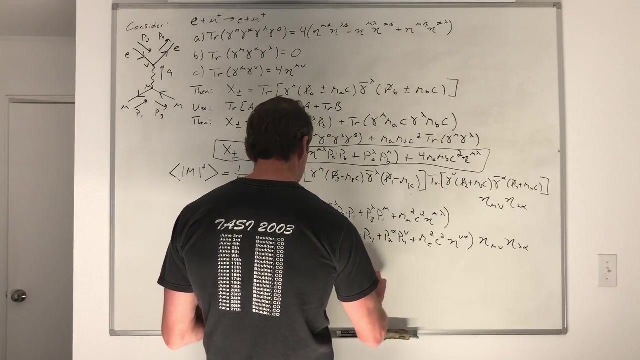 Okay. So there's a lot of massaging that you do here, But in the end you get an expression that looks like this: 8 Ge to the fourth, 8P to the fourth, over P4 minus P2. squared times: P3 dot P2, P1 dot P4 plus P3 dot P4, P2 dot P1. 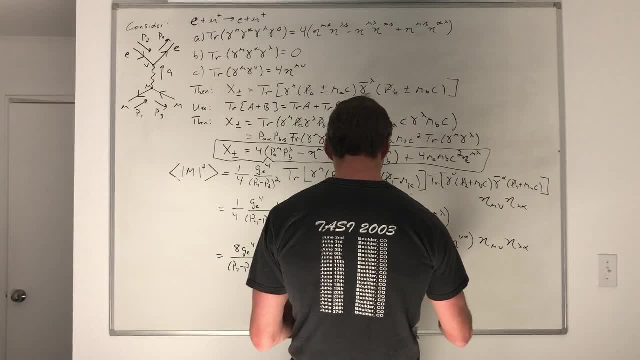 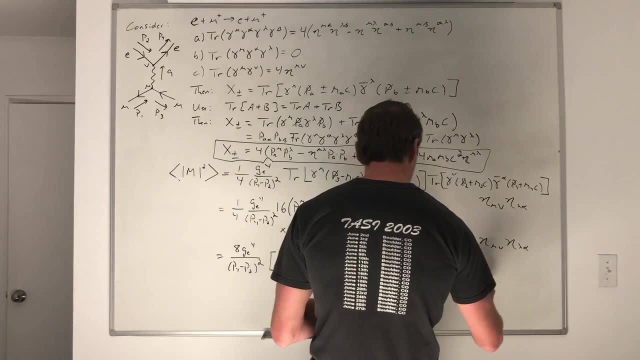 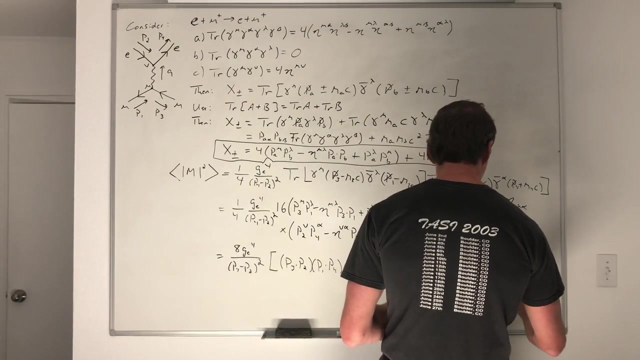 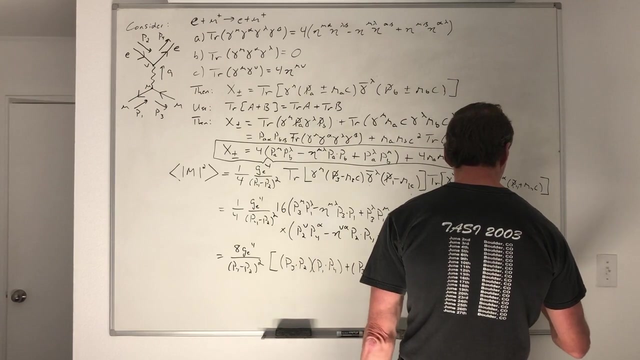 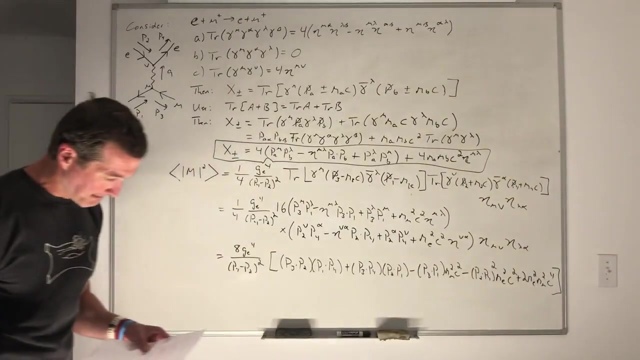 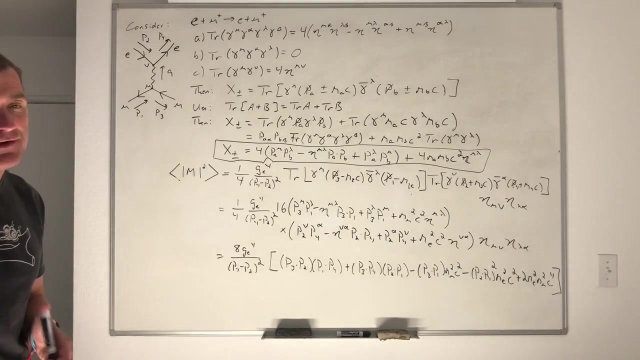 minus P2.. Okay, Minus P3. dot P1: mu squared C, squared minus P2. dot P4 squared me, squared C, squared plus 2me squared mu, squared C. to the fourth Now look, It's not pretty at all. However, it has lost some weight. 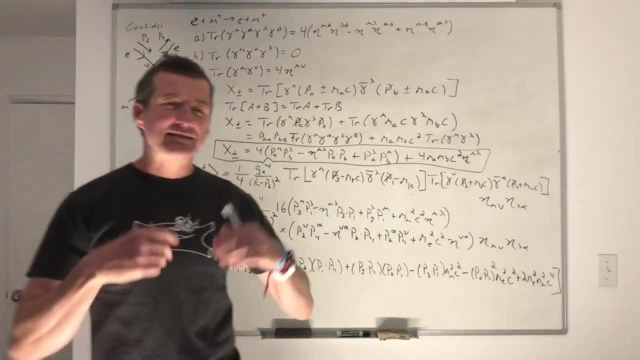 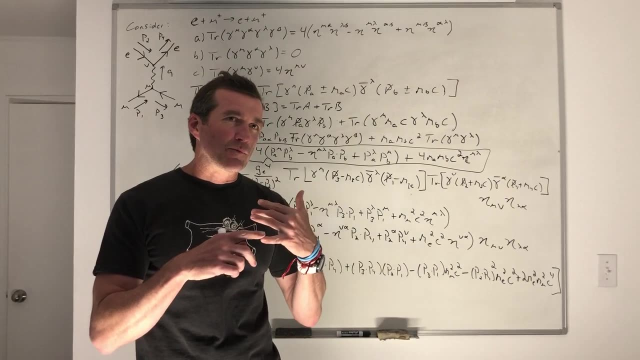 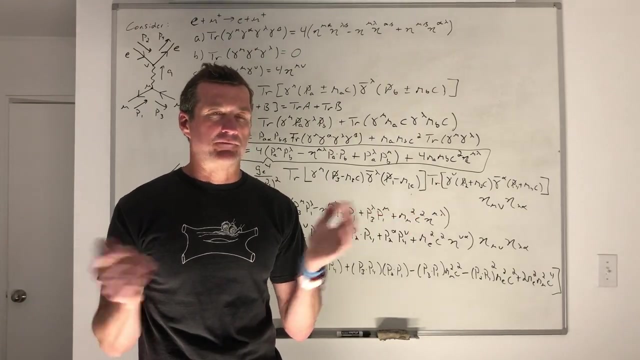 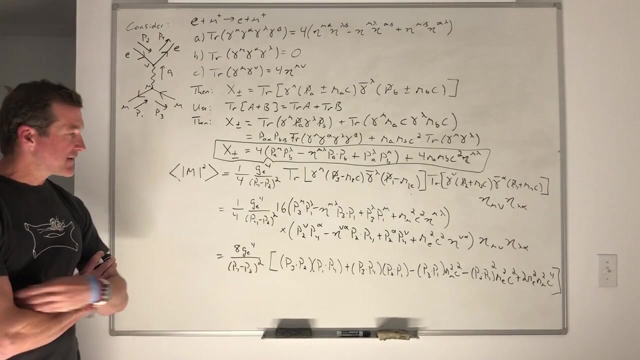 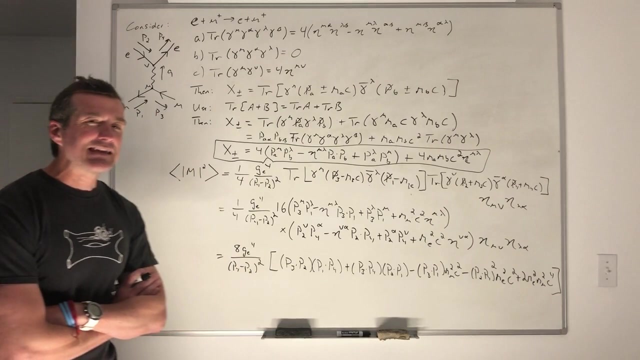 See, it went on the ketogenic diet, which is this diet where your intake is 100%, Space time, 10 seconds, Sink and no spinners. notice, there are no spinners in here anymore. this is an expression. say it again, you know. Atkins is a milder version of keto. keto is just. 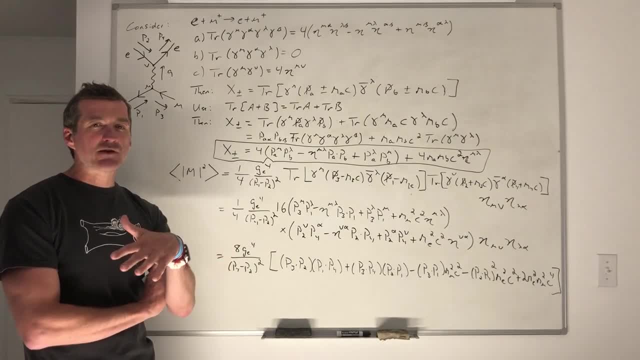 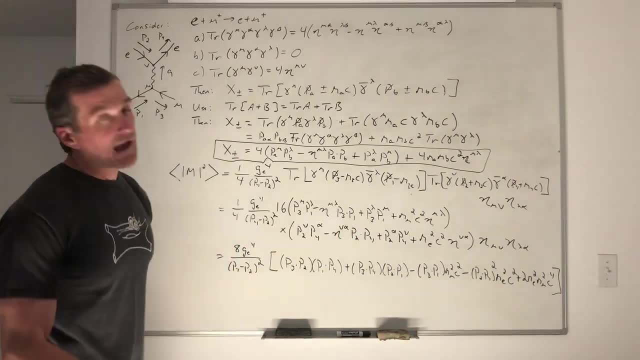 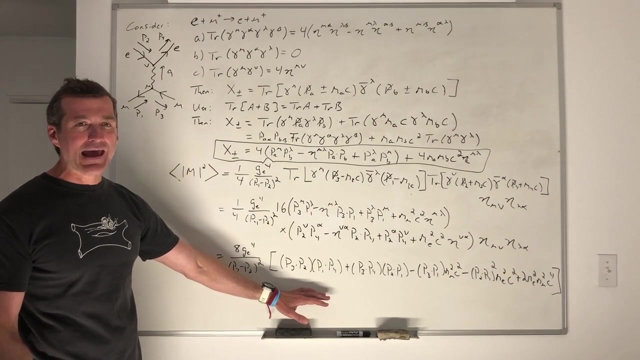 Atkins on steroids, which doesn't do any good because you lose all the water from your muscles and your muscles get small. so why are you taking steroids? because you're doing? I don't understand it, but anyway, I've tried it, trust me anyway. no, look at this. look, folks, we have peeled away. okay, we have completely peeled away. 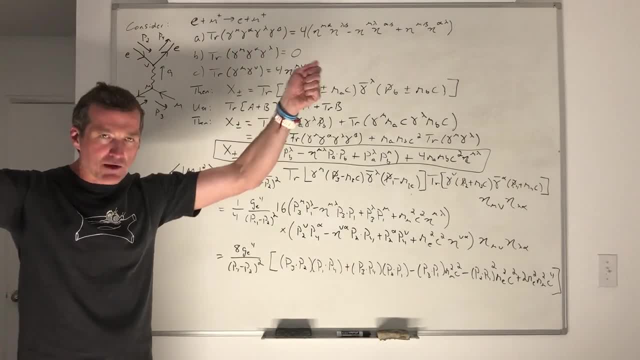 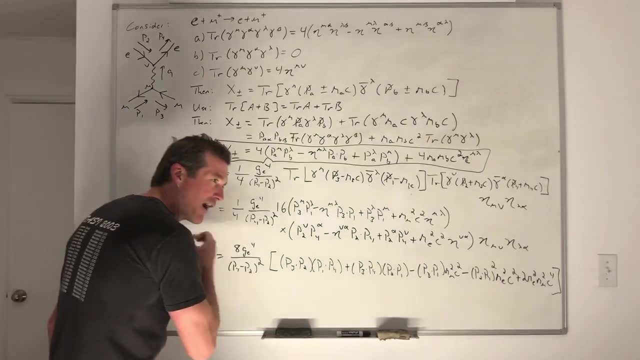 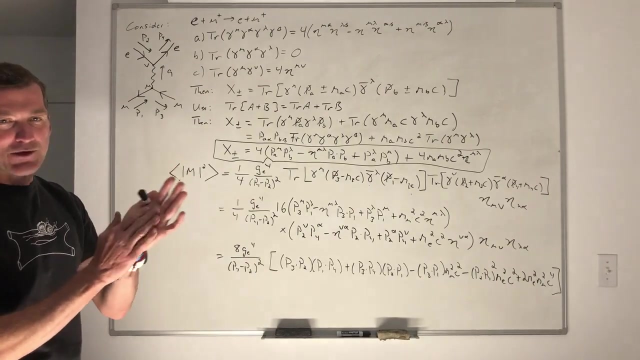 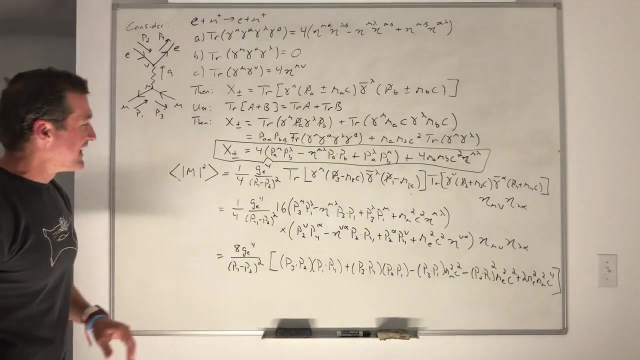 the presence of spinners. this should be a hallelujah moment, okay, cuz spinners suck. they're the worst thing in all of these calculations. and they are gone, thank you, thank you, it's all done in silence. it's kind of weird, but whatever, okay, all right. so any questions about- I mean, look, there's a, you know, multiplying. 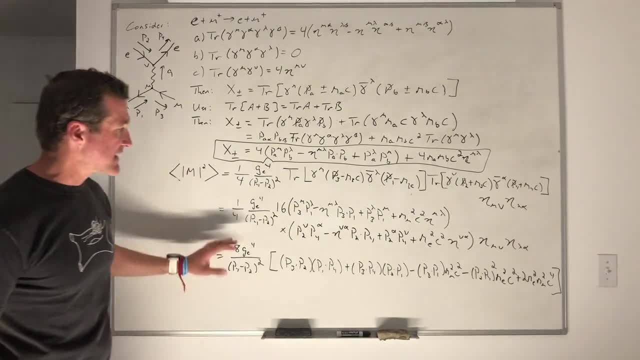 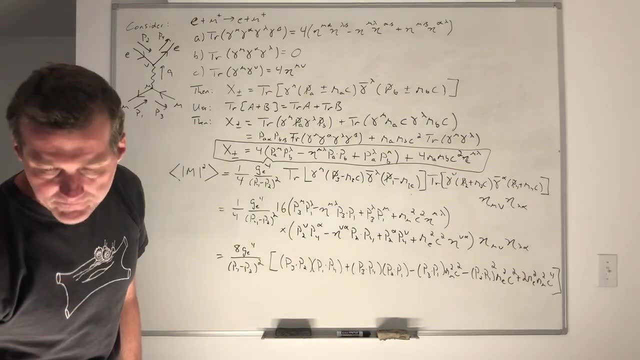 these two things together and then using all the metric factors to reduce things is. you know, it's simple, but I mean it's, it's, it's tedious, it's not hard but it's tedious. but this is our clean result at the end. and now what we want to do is we: 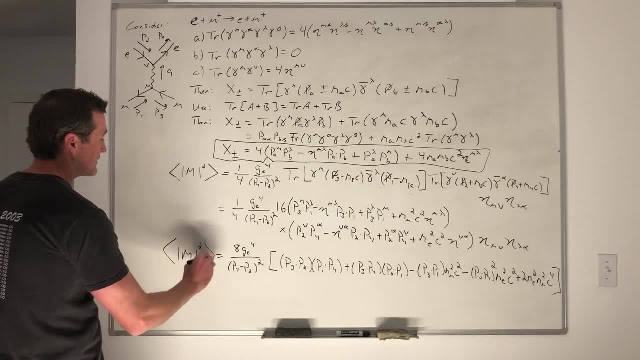 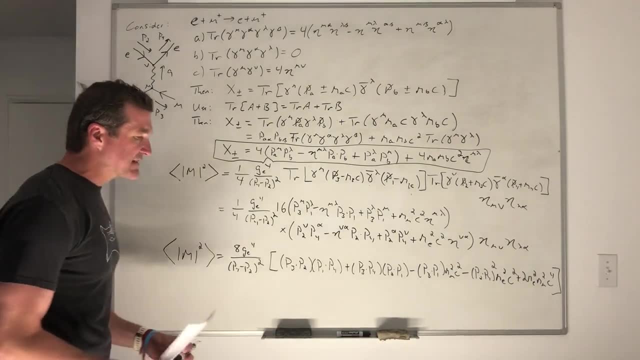 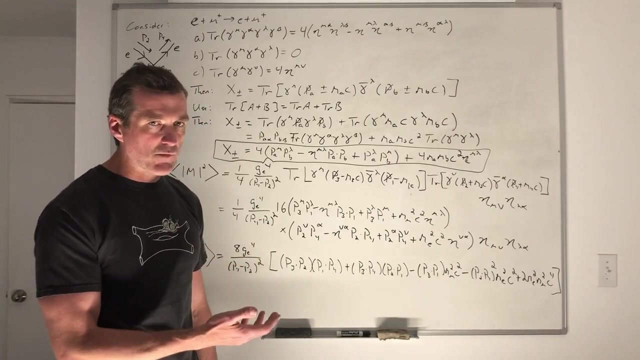 is. we want to take this and we want to go back to the golden rule with it. okay, Because I don't know if you remember, but the golden rule had all of these external factors which depended on the external momentum: p1, p2, p3, p4,. 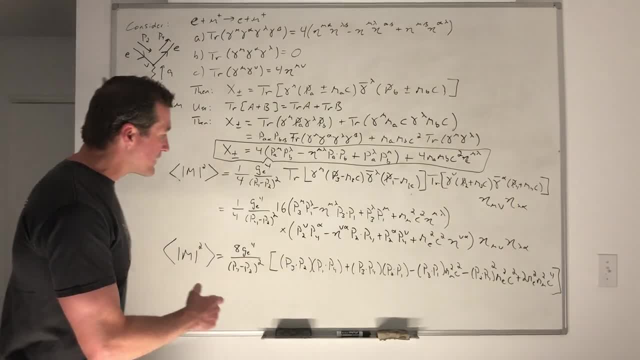 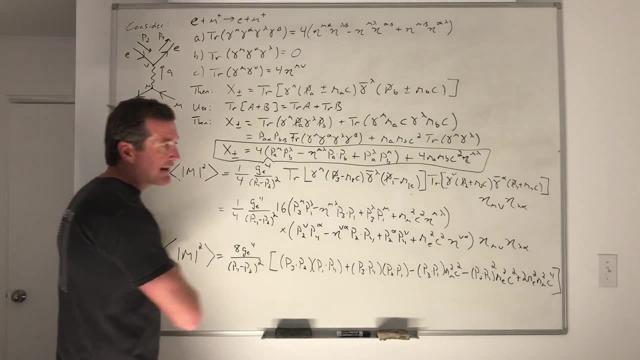 and then it just had this factor of m squared sitting there. Well, now we've transformed the factor of m squared by averaging it partly. We've transformed the factor of m squared into nothing but factors of the external momentum. okay, There's no more spinners to complicate things. 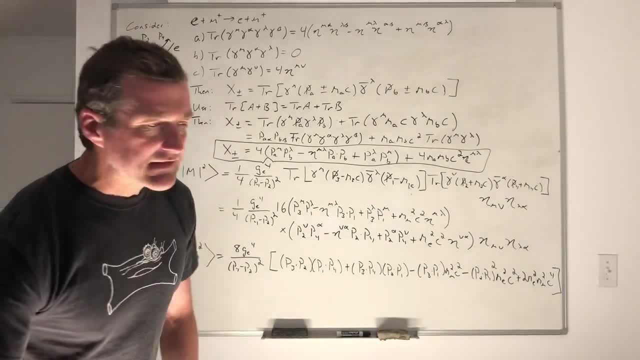 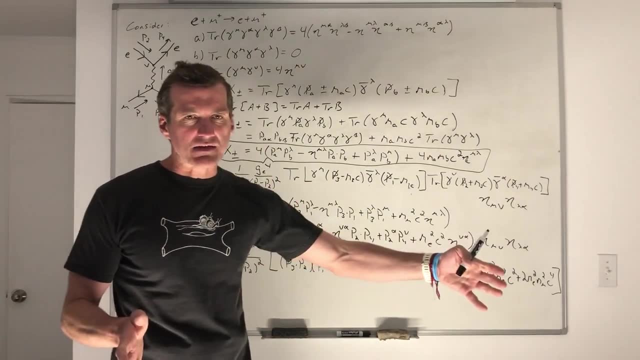 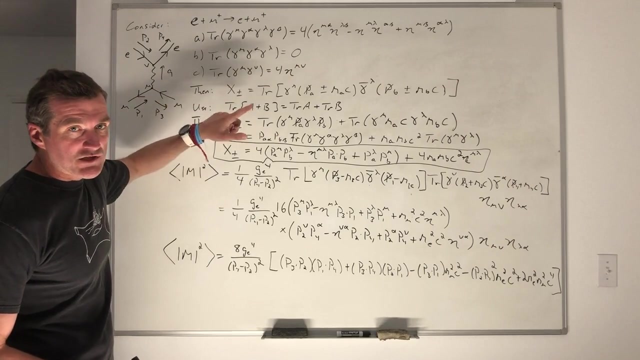 And again, look, it's not that we took the expression with spinners in it and we said, ooh, spinners, let's pull them out. and just look at the rest of it. That is not what we did. What we did was we constructed spinner sandwiches. 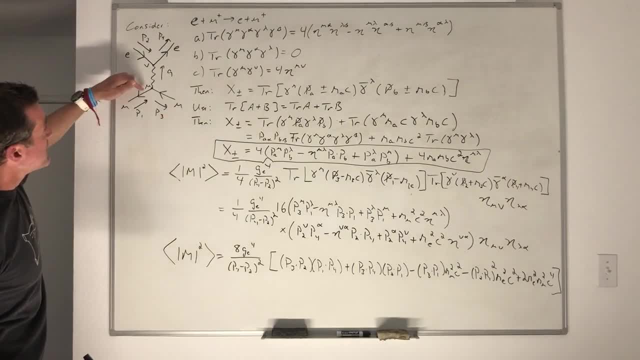 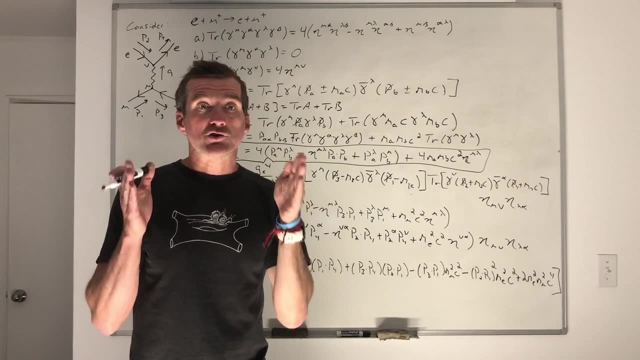 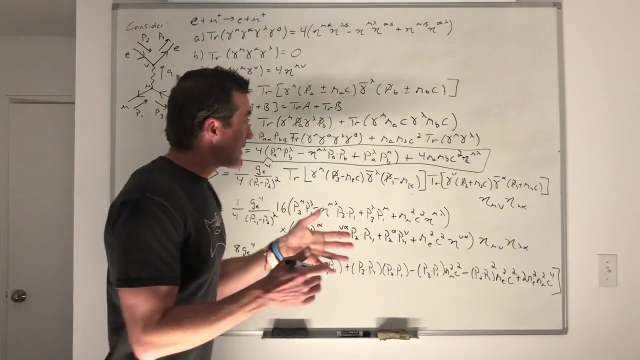 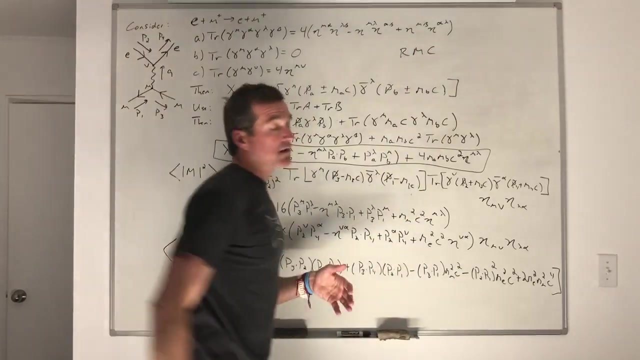 so that the spinners Spinner sandwich, v-bar, gamma matrix v, that thing itself we always knew was not trivial in spin. It was non-trivial in spin space because it's just a scalar in spin space. right, A spinner sandwich has got a row spinner, a matrix and a column spinner. 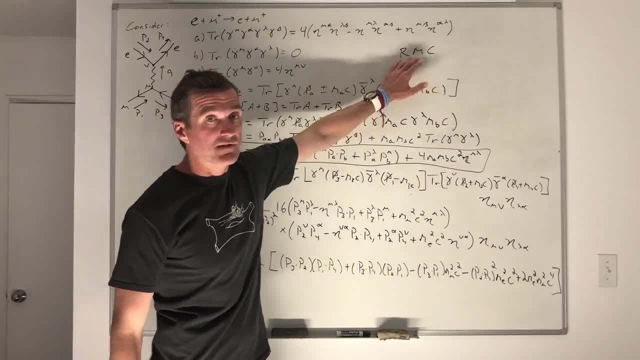 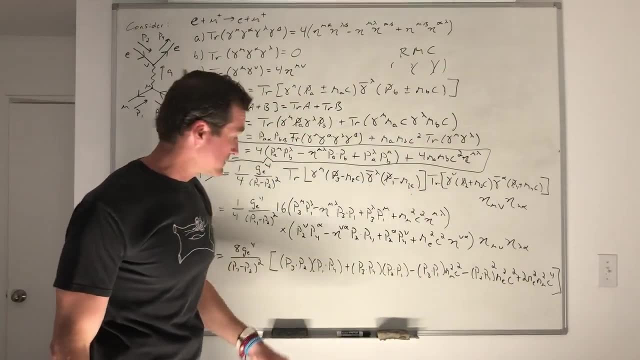 and those are their structures in spin space. okay, Well, if you take a row, you multiply it by a matrix and you multiply that By a column. that's always going to give you a scalar. okay, We're just actually doing all of that multiplication. 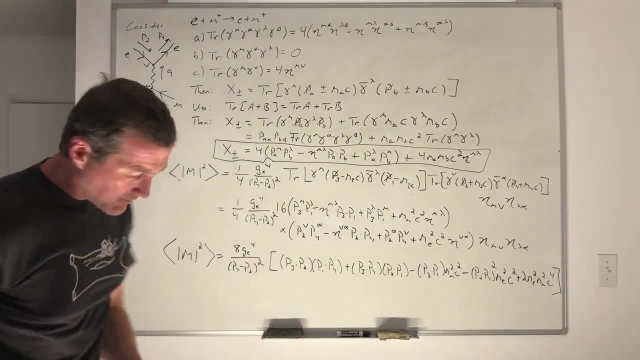 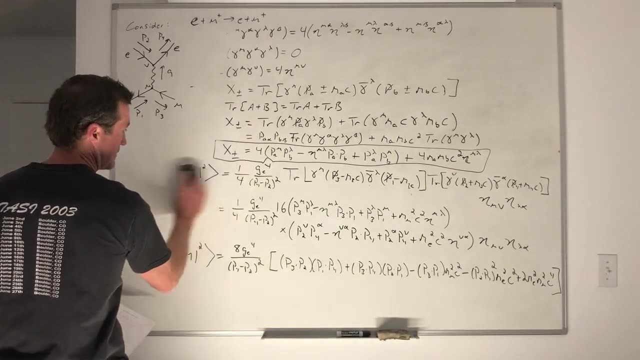 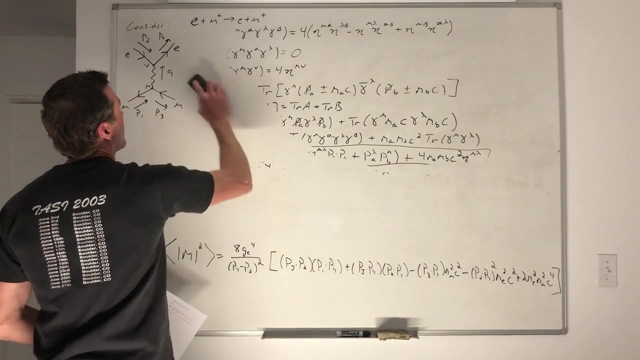 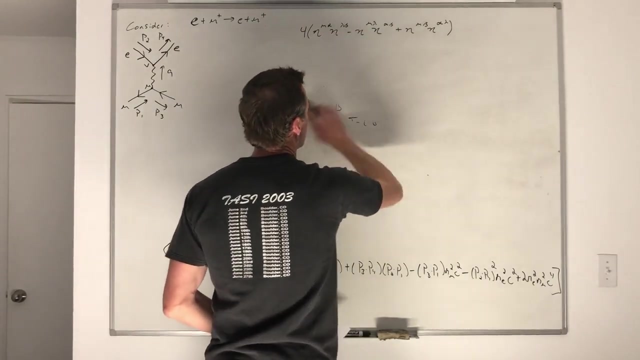 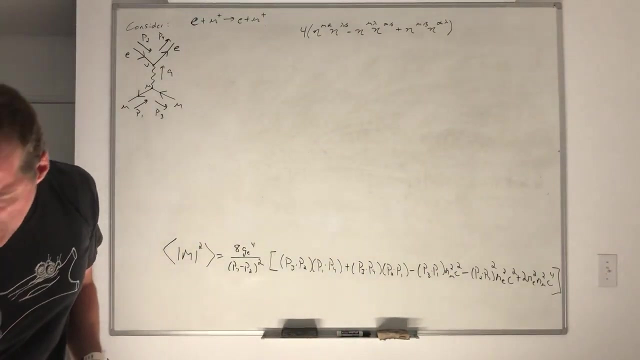 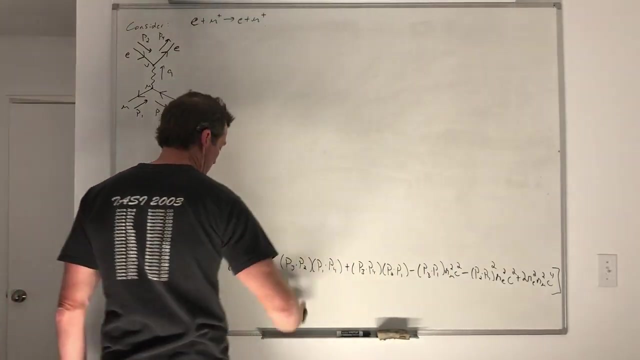 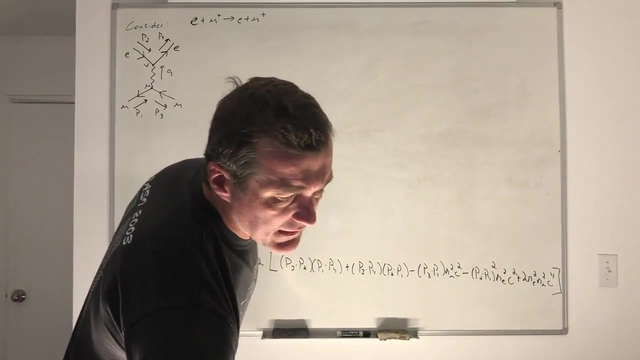 All right. So now let us go back to the golden rule. Oh yeah, I don't think that either. Okay, So for scattering events, what quantity does the golden rule actually calculate for us? avery, Avery, Avery, Avery. 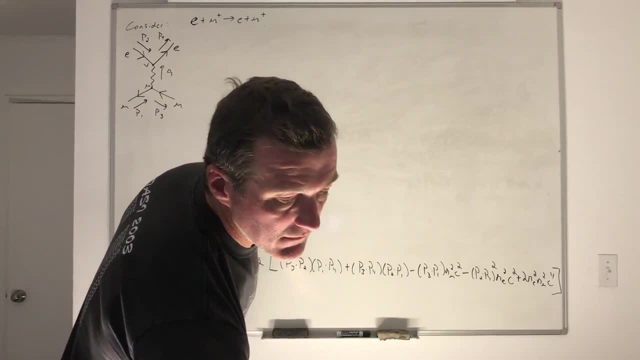 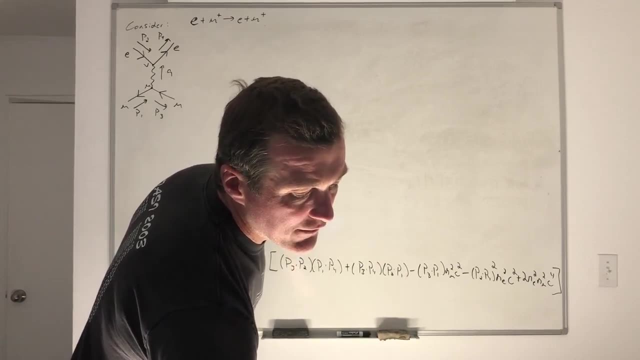 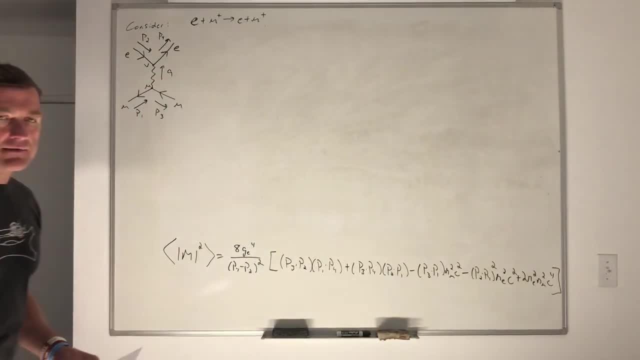 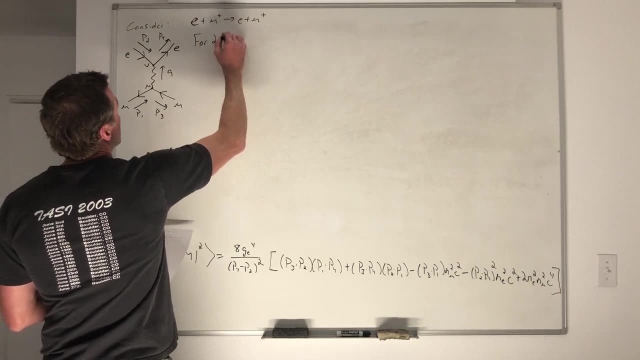 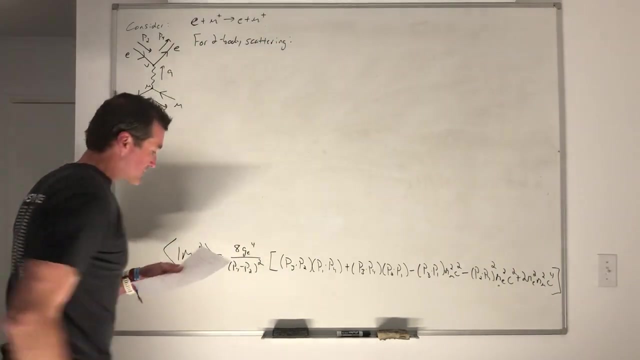 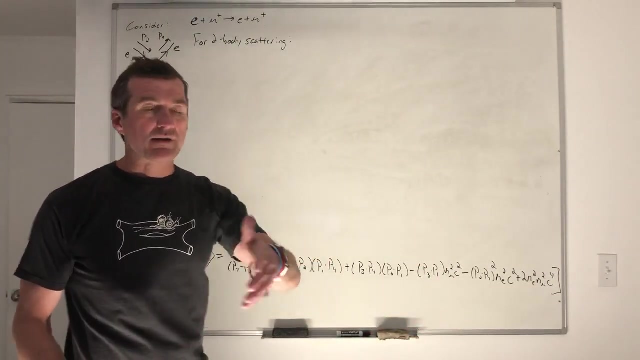 The cross-section, The cross-section or, in fact, the differential cross-section. Okay, So we have a two-body scattering event And we know that two-body scattering actually gives us a simplified form of Fermi's golden rule, which you worked out. 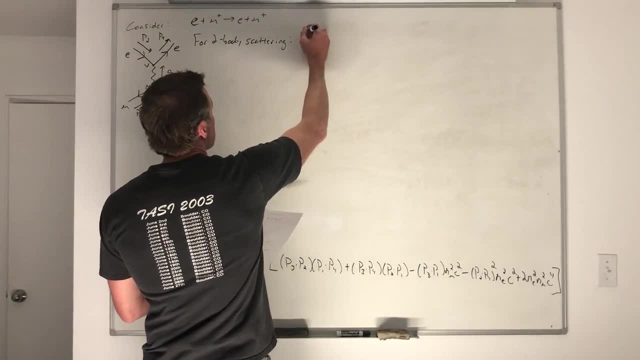 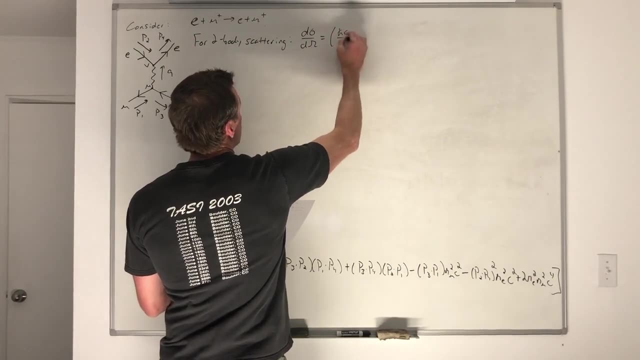 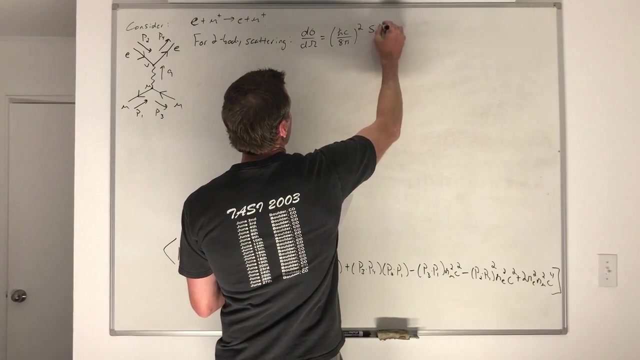 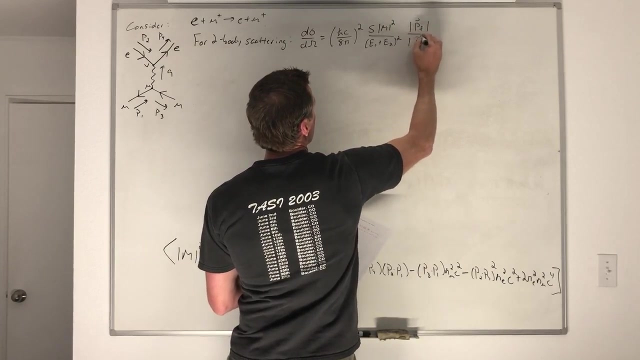 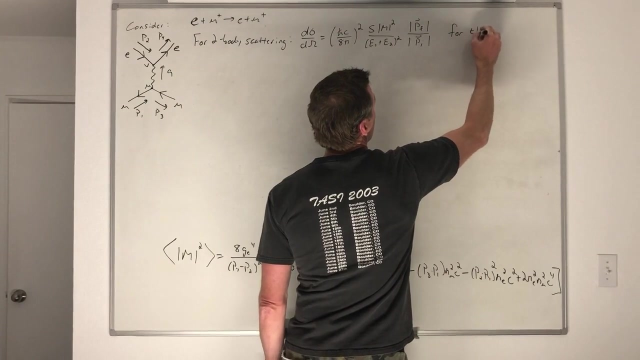 in your homework, but we have that. d Sigma, d, Omega is h bar C over 8 pi squared s, m squared over e 1 plus e 2 squared times, a factor of the magnitude of any of the outgoing momenta and any of the incoming momenta for the center. 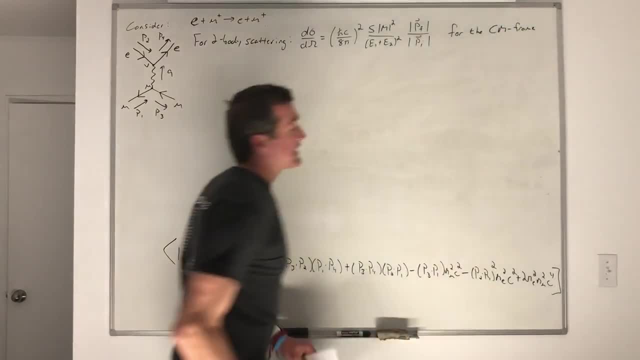 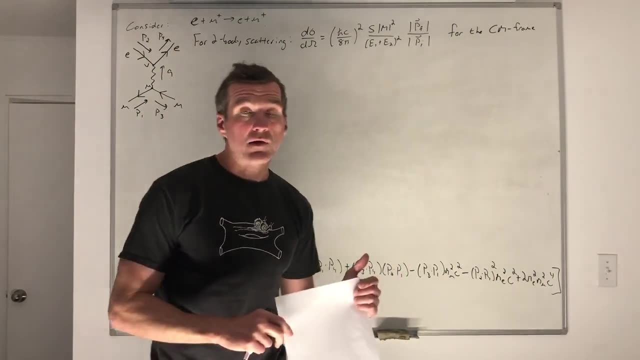 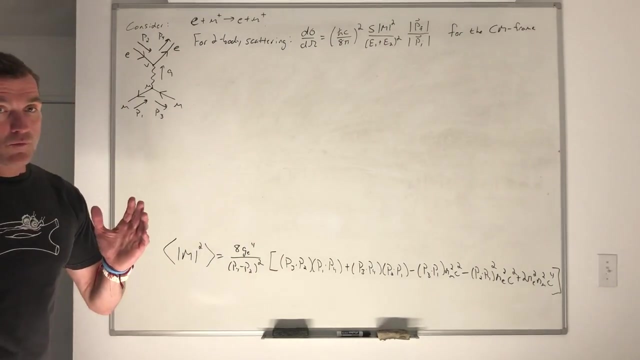 of mass frame. okay, so to get this expression, we have to take the center of mass frame, so that the total spatial momentum going in is the same as the total spatial momentum going out, which is 0. okay, now we can almost put this in its final form, because we've got an expression for the 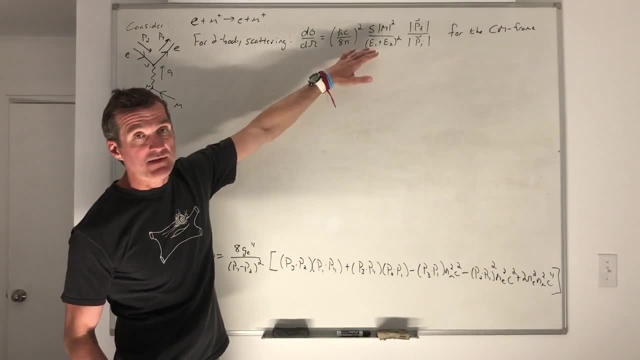 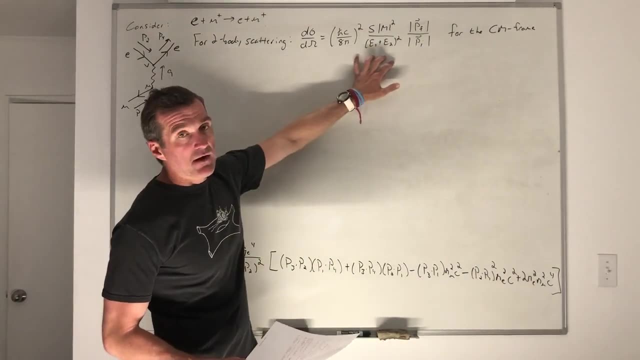 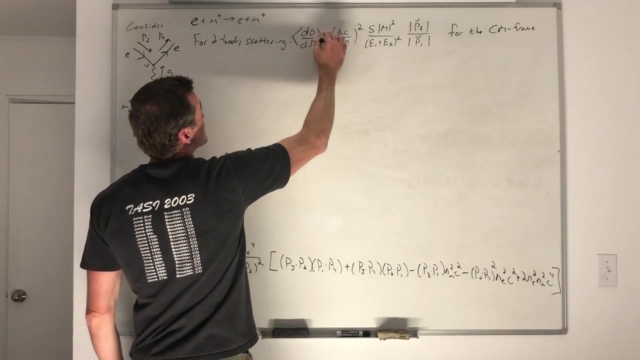 average of m squared and we're going to average over the incoming spins anyway and some of the outgoing spins. all right. if we did not want to do the average, this would have been our expression. but we can say: I don't care about the spin of the incoming particles or the spin of. 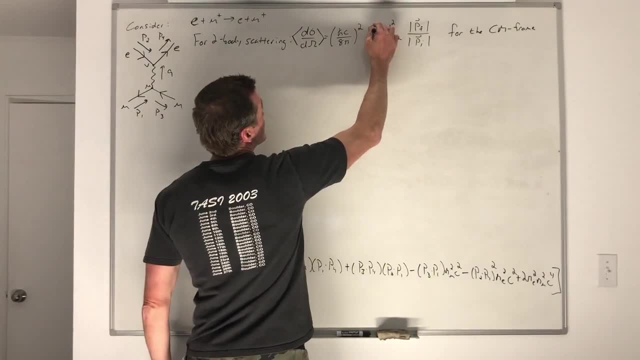 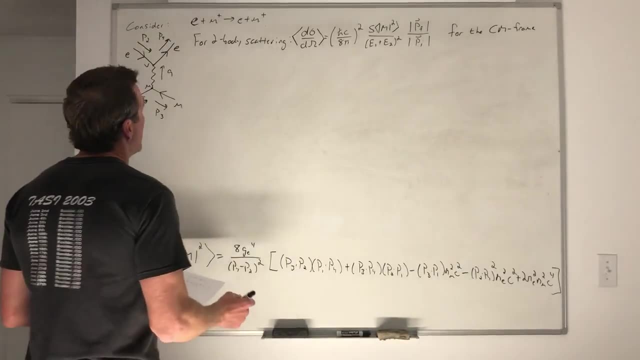 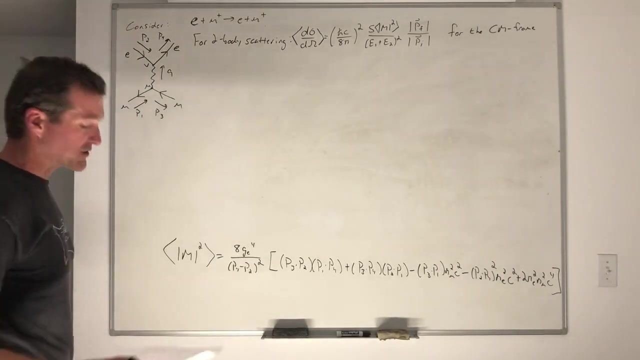 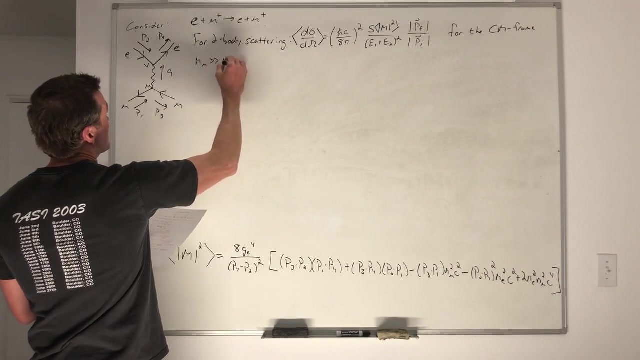 the outgoing particles. so to calculate the average I just use that guy. okay, now I'm going to, for this process, make some approximations in order to get to those formulas which I mentioned earlier. so first of all notice: a muon has a mass which is much, much less than the mass of the incoming particles. so that's the. 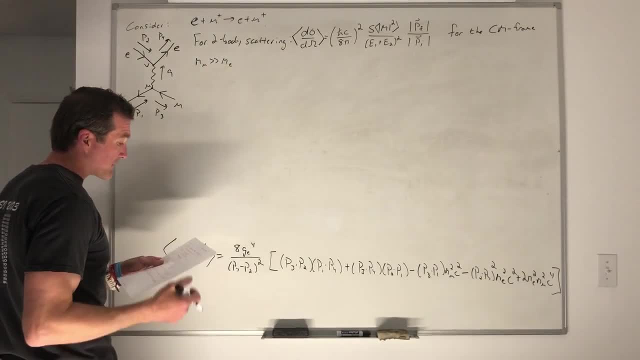 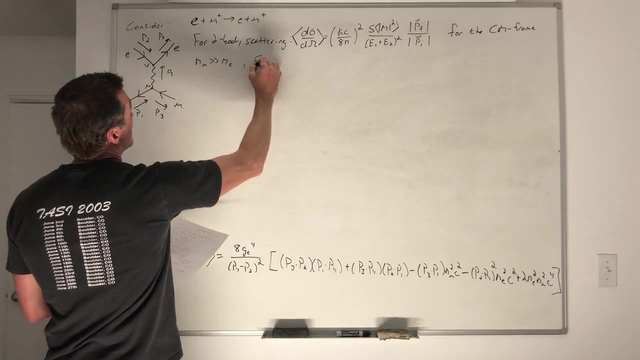 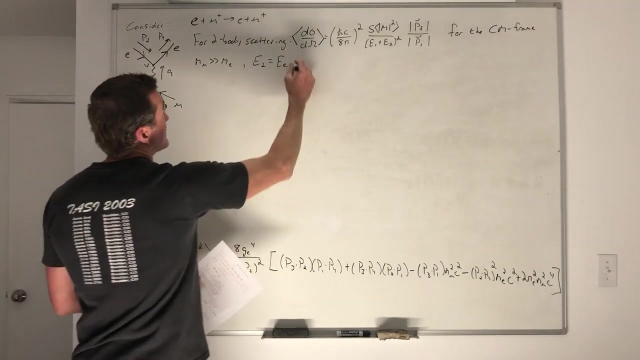 muon? okay, so I'm assuming that the mass of the muon is much, much larger than an electron? okay, and the energy of the e2 particle, which is the energy of the electron? okay, this is going to be much, much less than the mass of the muon times. 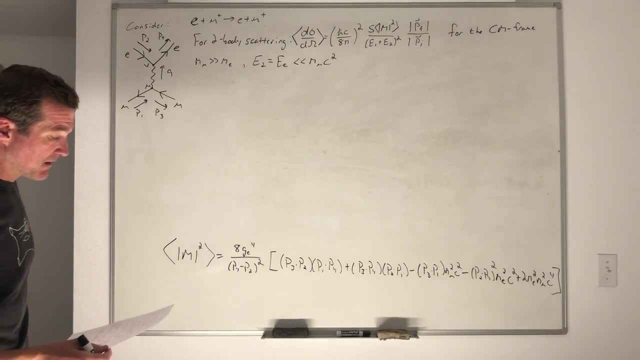 c squared, that's the rest energy of the muon. okay, so I'm assuming. what I'm guessing is that this electron's total energy, which is its rest mass energy plus its movement, movement related energy, the total energy of this electron is just going to be swamped by the rest energy of this muon. this muon is huge. okay, imagine this is. 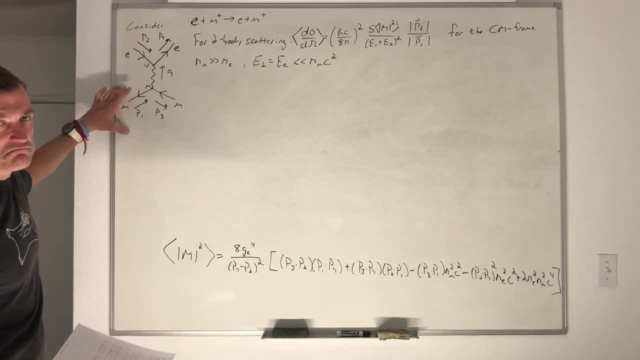 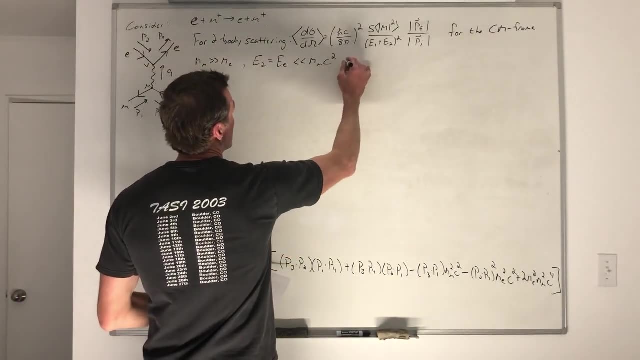 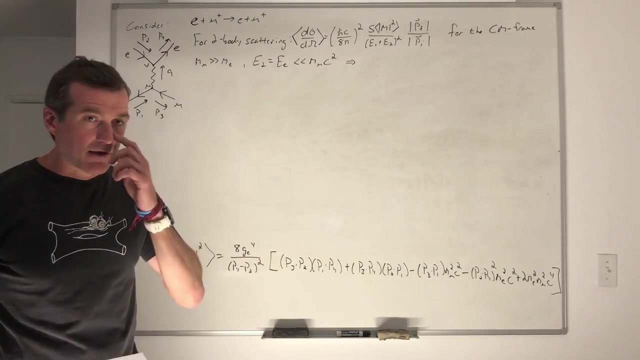 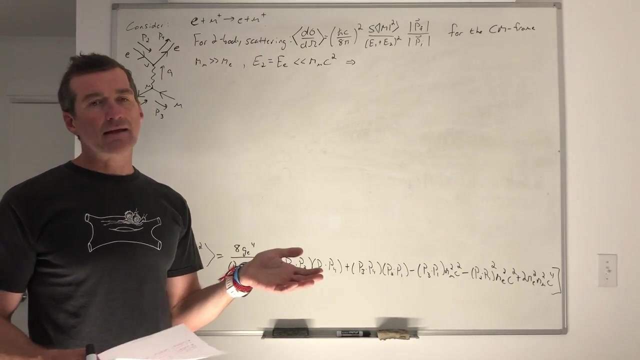 like a satellite and this is the earth. okay, now, this simplifies things because it's literally, it's like a satellite in the earth and some, you know, gravitational slingshot effect. how does the initial and final momentum of the earth or of the satellite relate in magnitude? 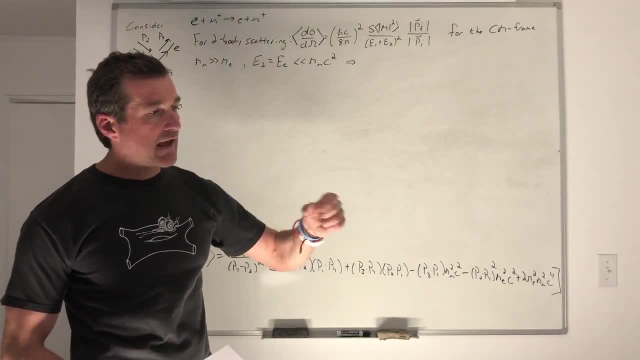 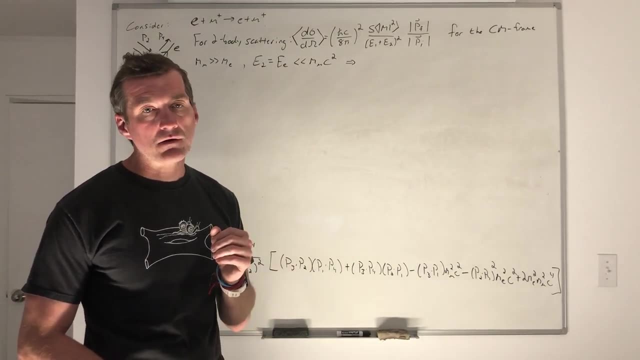 so if a satellite comes in with some momentum p initial and it leaves with some momentum p final, how are the magnitudes of those two related? if the earth is so big it doesn't move at all. don't make me draw a card, okay? so I'm assuming that the mass of the muon is much, much less than the mass of the 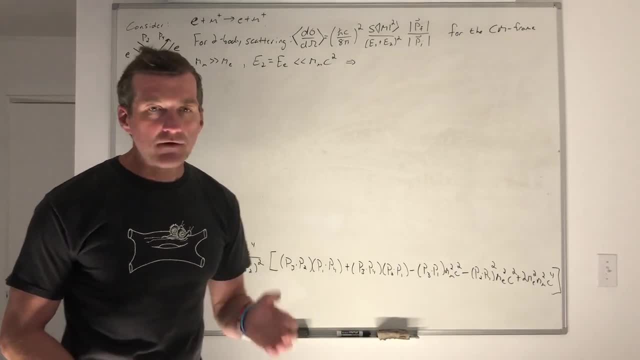 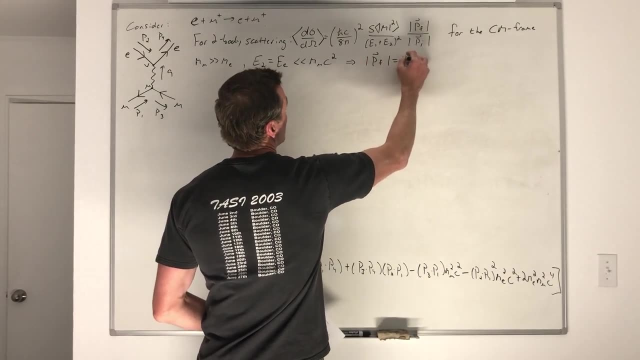 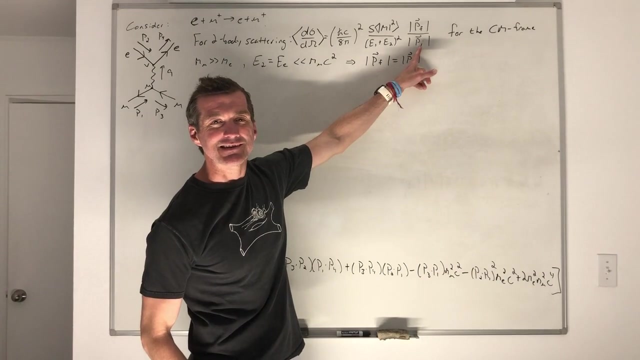 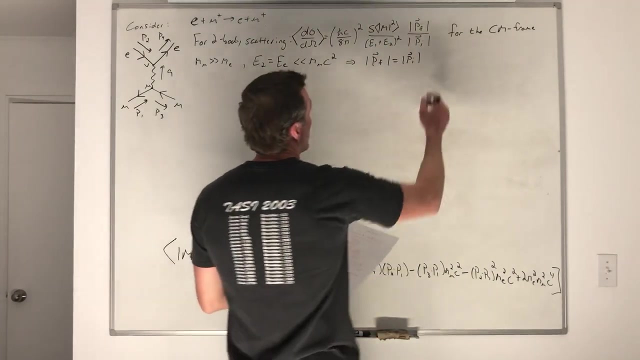 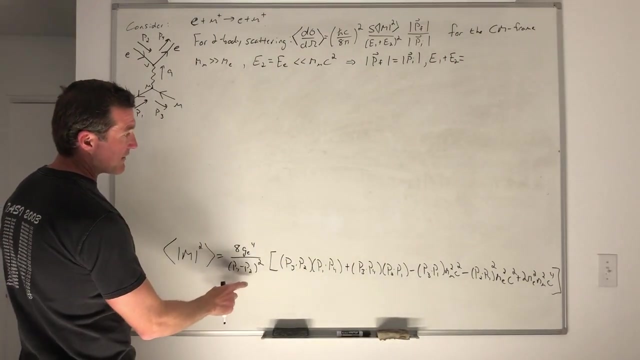 star, they're pretty much the same. yeah, so we can say that the magnitude of p final is the magnitude of p initial in this approximation, which of course makes this factor super easy. it's just a one, okay, more over e one plus e two which we've got to figure out for down here. okay, 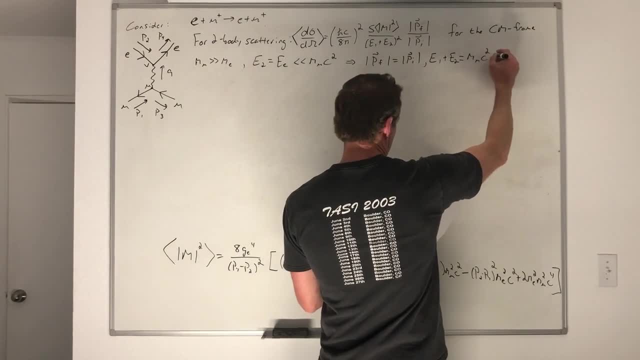 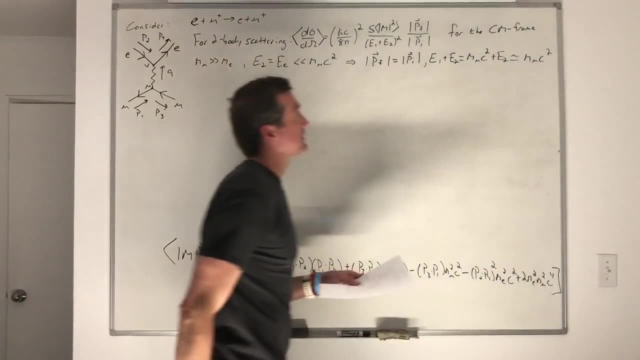 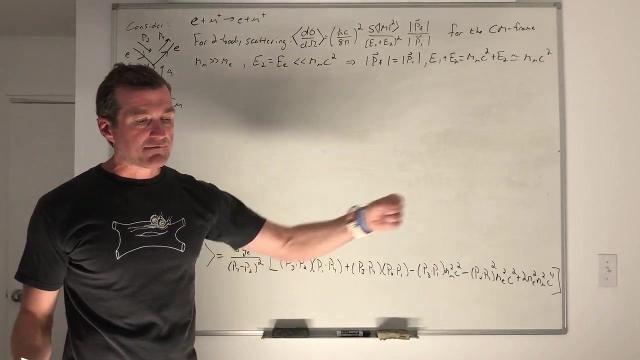 E1 plus E2 is basically mu c squared plus E2, which is going to roughly be mu times c squared. okay, Because if we have a huge mass particle and a very light particle coming in, where, approximately is the center of momentum frame, 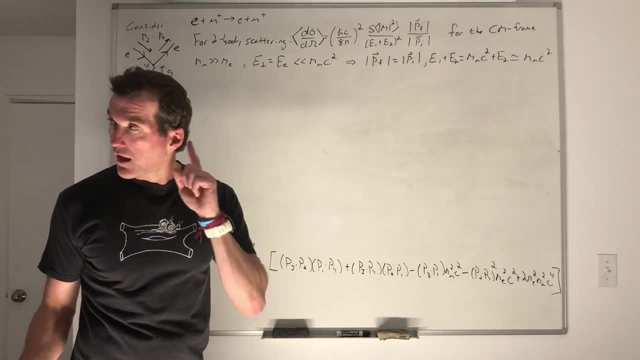 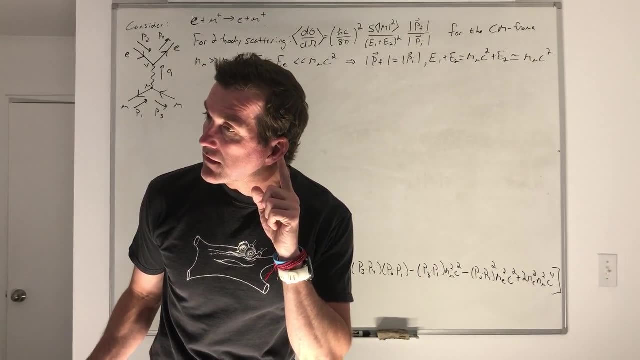 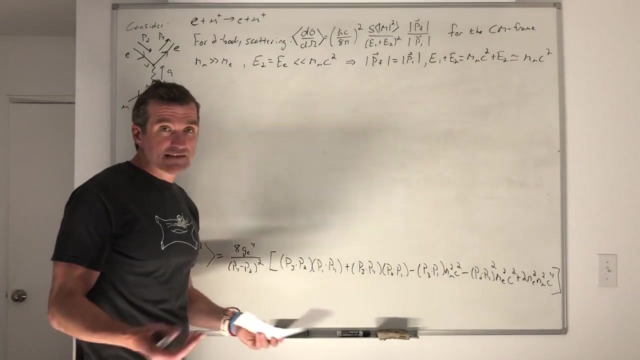 What's it? approximately equal to Big one. Say it again: The big one, the bigger one, It's the rest frame of the larger particle right, The rest frame of. I mean, you know, if you've got the Earth and you've got a little satellite. 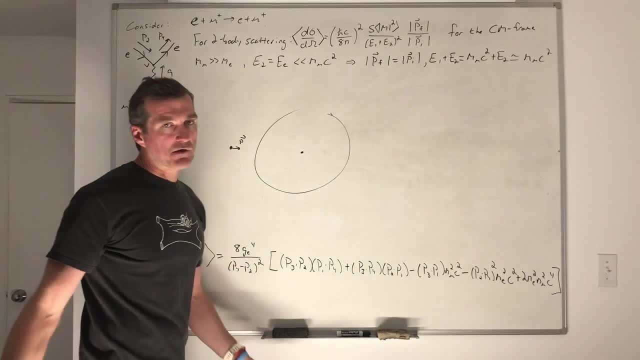 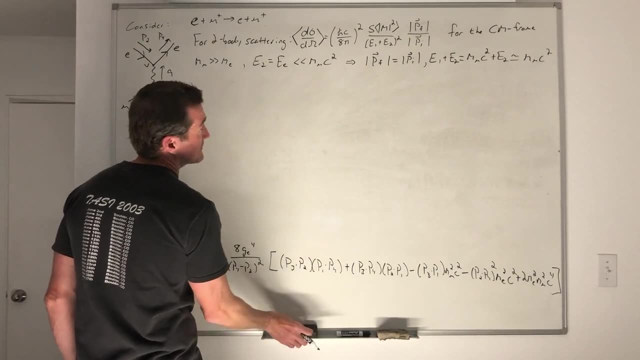 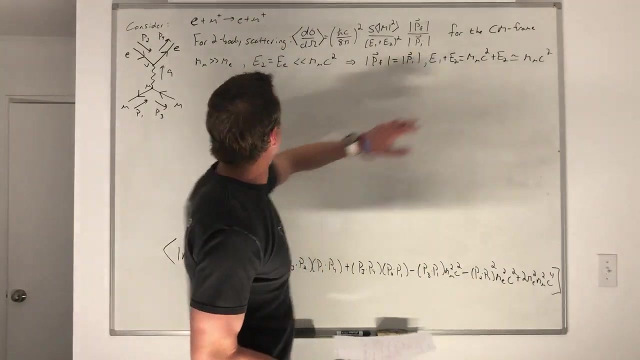 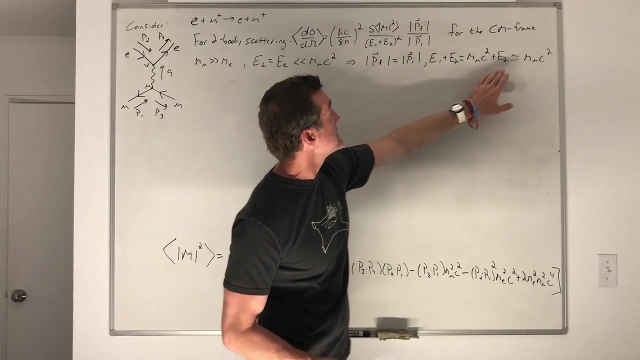 the center of momentum frame is roughly the rest frame of the larger particle. It's the rest frame of the Earth, okay, So. So the energy for particle one is just the rest mass energy of the muon and then the electron will be moving. but, like I said, E2 is much less than mu c squared. 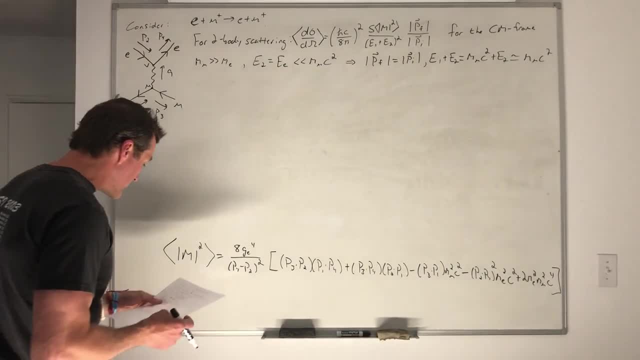 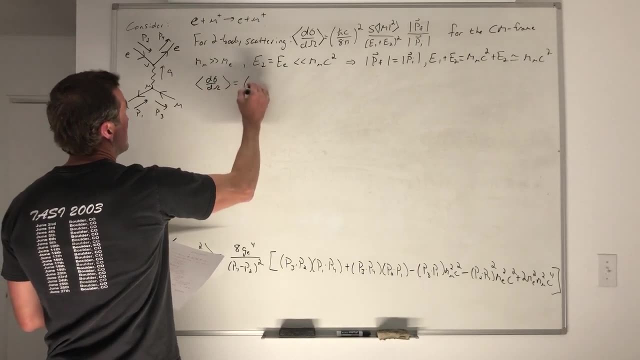 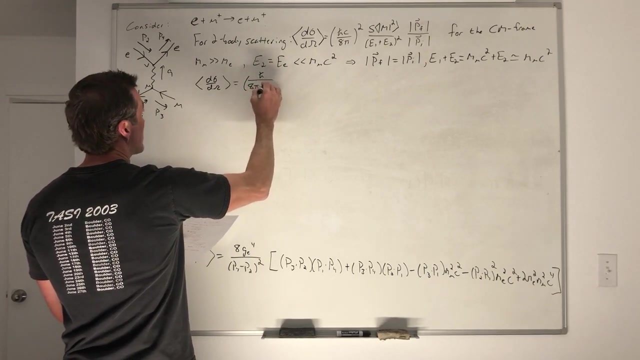 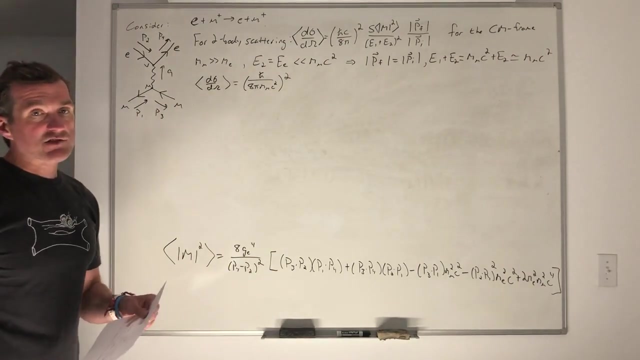 so we'll just approximate that sum by mu c squared. okay, So we have that d sigma, d omega averaged is given by h bar over 8 pi m mu c squared quantity. squared s in this case is just 1, because you can't interchange the outgoing and the incoming particles. 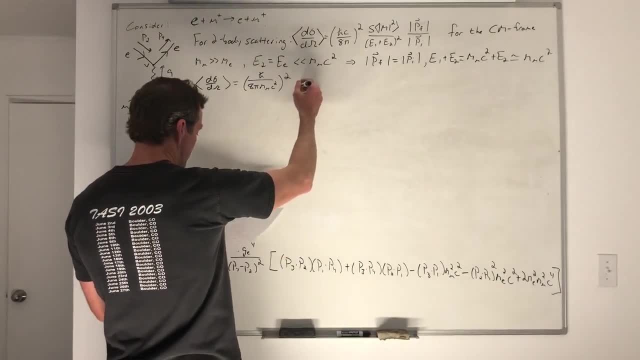 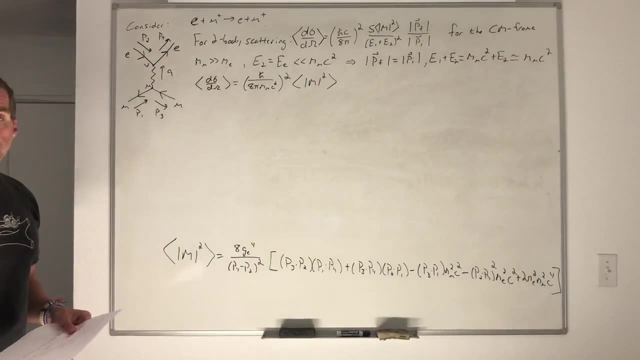 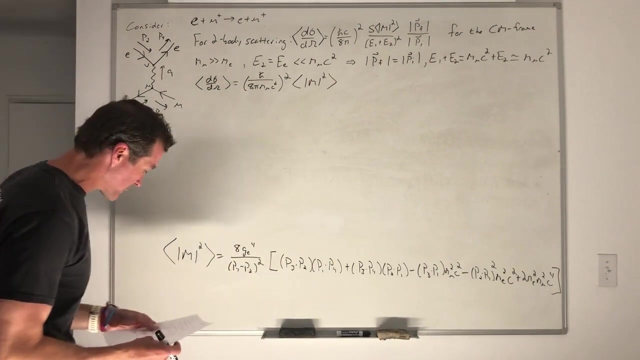 because they're distinct particles, so the symmetry factor is just 1, times m squared averaged. Okay, This is looking a little clean, but we still have to put in this, Alright. So, in order to figure out what this is going to look like, 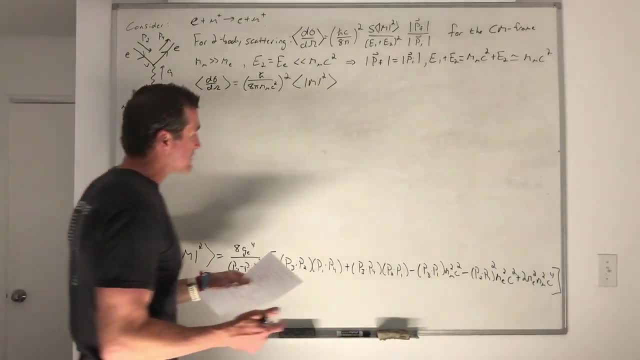 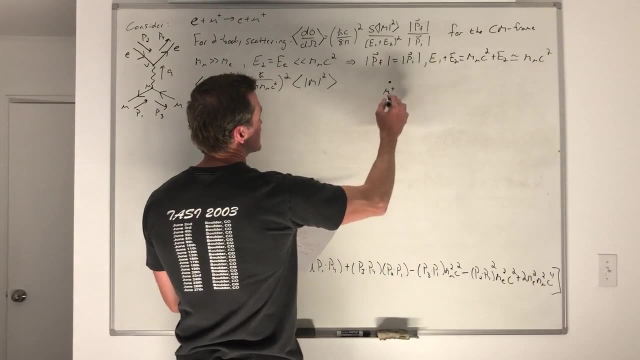 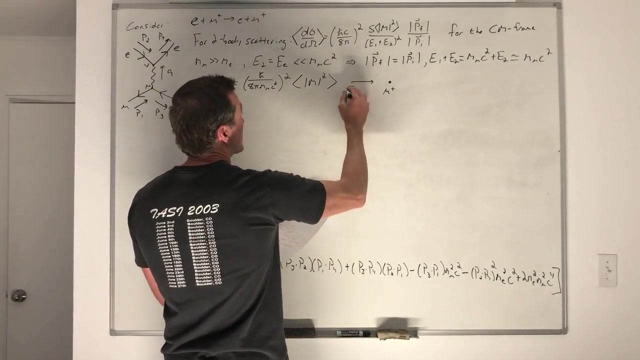 let me go through and make some assignments of quantities. So we're going to start with a little picture here. So we've got the mu plus, which is sitting at rest, and we've got the electron coming in with an energy and I'm just going to call its energy E. 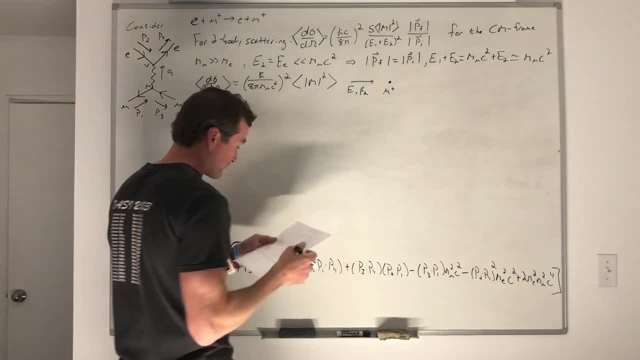 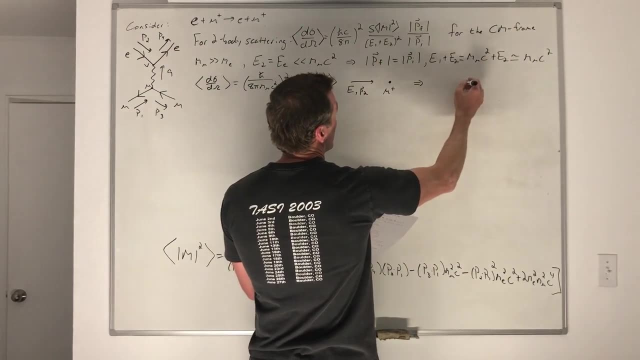 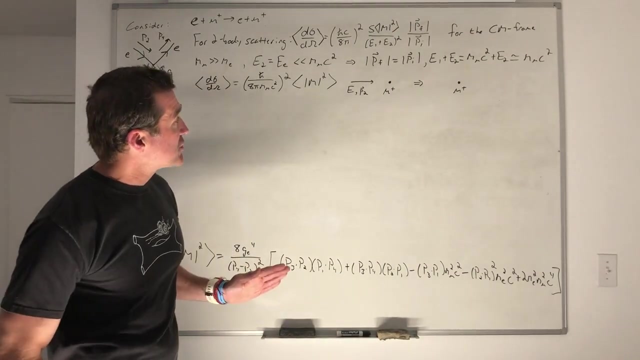 and a spatial momentum, p2, and then afterwards the muon will, or the anti-muon will, still be at rest, but the electron will move away at some deflection point, at some deflection angle, and that deflection angle is what we're really after. 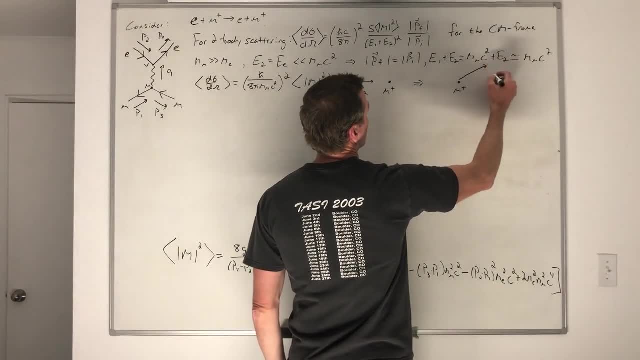 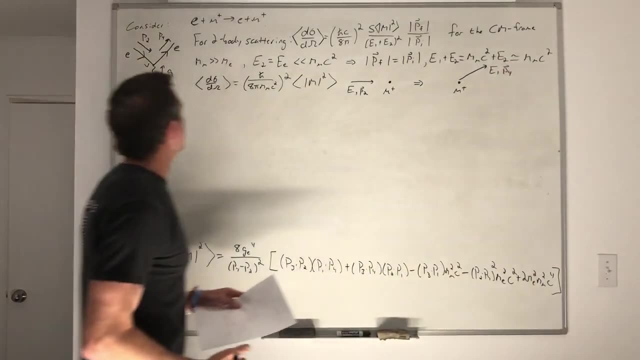 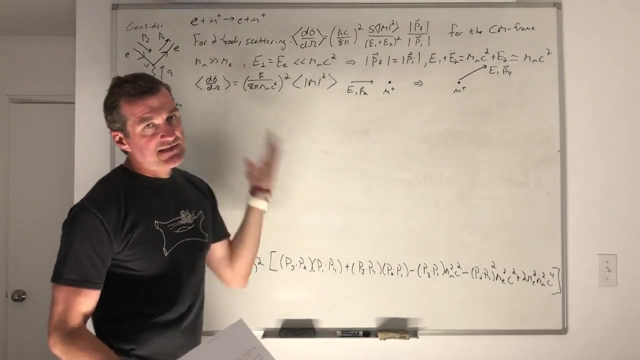 So the electron can be deflected with some energy E and some final momentum p4.. Okay, The electron has momentum p2 coming in and p4 going out. Alright, All I'm saying is that its energy doesn't change. the magnitude of its momentum doesn't change. 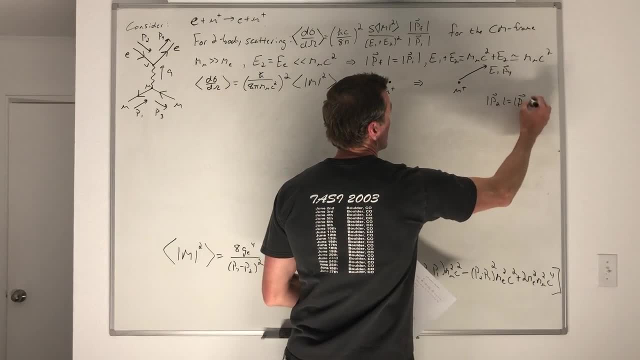 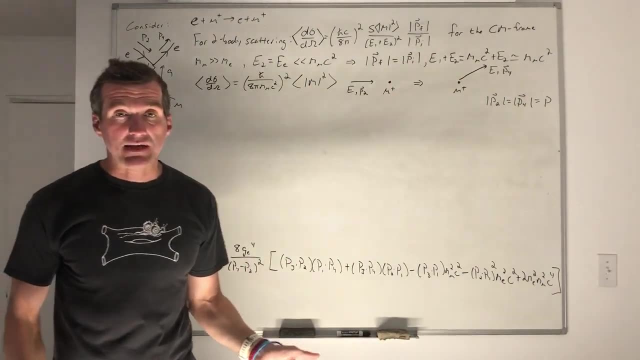 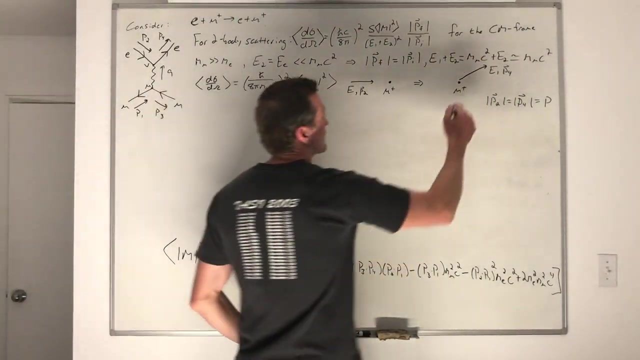 it's just that it's moving. Okay. However, there can be a change in the direction that it's moving, and if you just imagine that, you know that's the interesting result of these collisions. Okay, So I'll put in an angle theta there. 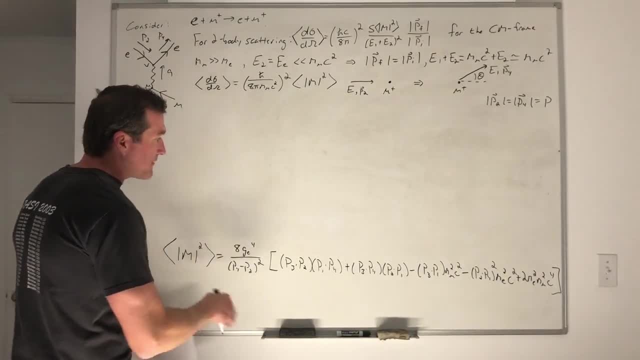 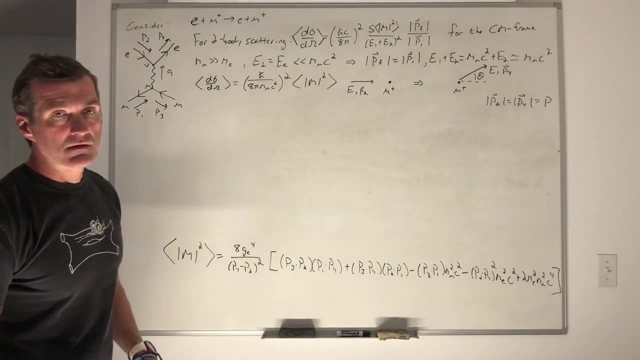 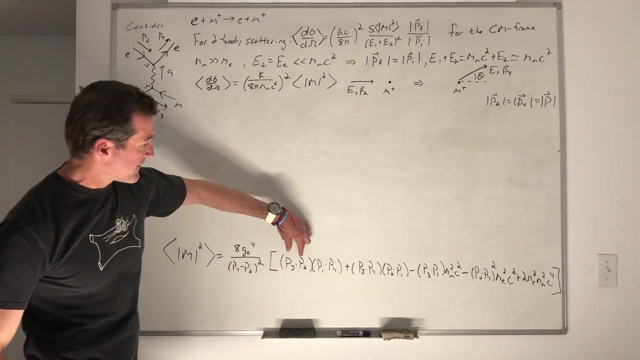 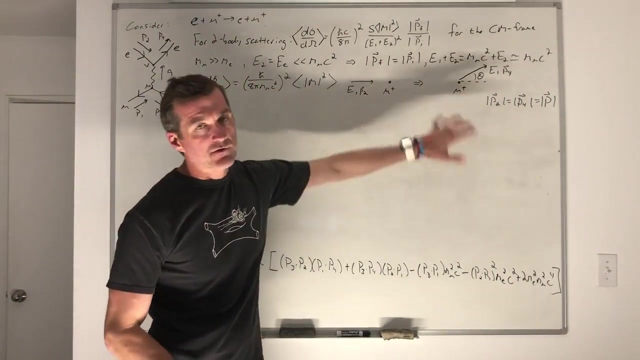 Alright. So now this thing is using what kind of vectors? Is that a 3-vector? It's a 4-vector. So what I need to do is I need to figure out what are the 4-vectors for all of these. 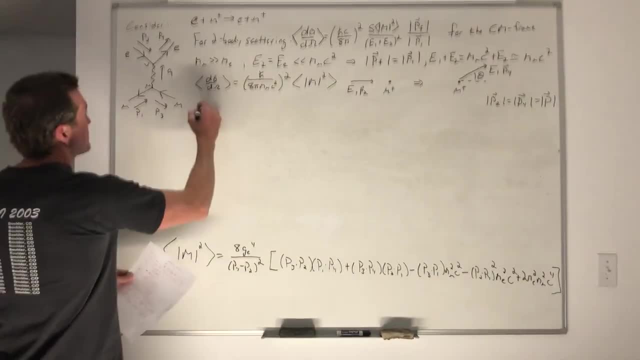 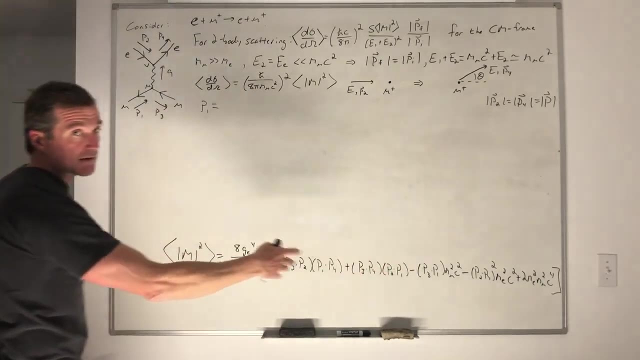 Okay, Well, that's pretty straightforward. So p1 is the 4-vector, So I've got to do p1, p2, p3, p4, and then plug them all in here. That's all I've got to do. 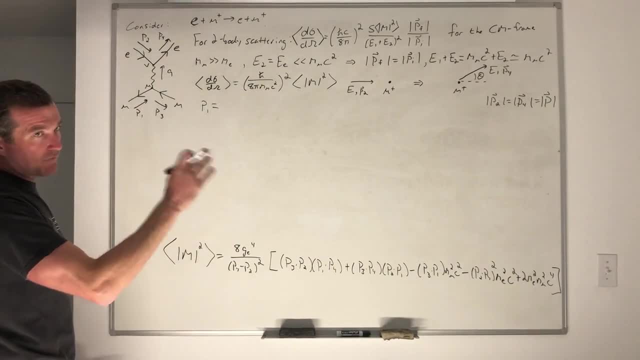 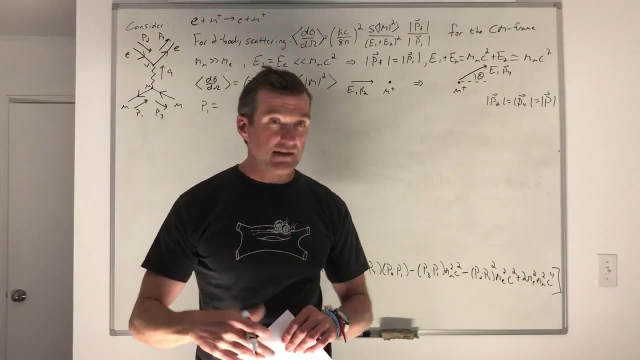 So I've got to write down those 4-vectors, Those 4-vectors, That's not 16-vectors. 4 times 4 is 16, but I'm talking about 4, 4-component vectors. Okay, So if you count the total number of components, 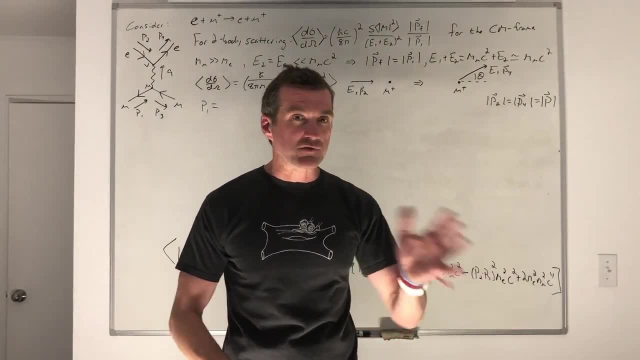 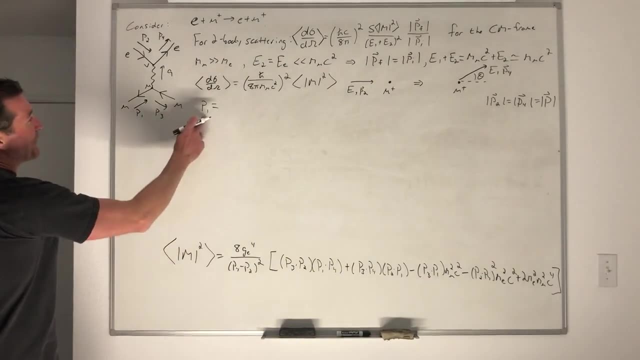 then you're going to multiply 4 by 4.. But we're not talking about total number of components. we're talking about the number of 4-vectors. So it's 4.. Got it Good, Awesome. What does the 4-vector for p1 look like? 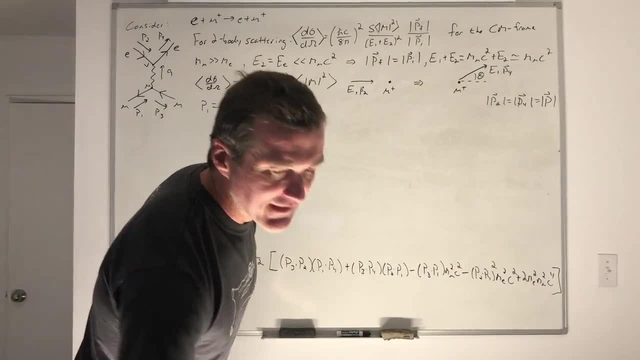 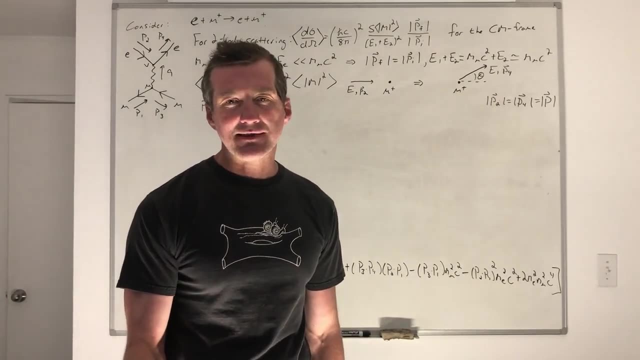 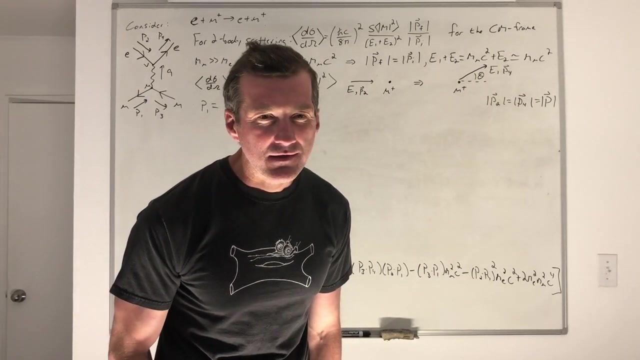 Let me draw a damn card. Oh man, See, Sam is not with us because Sam went back to the Midwest where he says his family's eating dinner at this time. So he watches the video. Ryan Is Ryan short on. 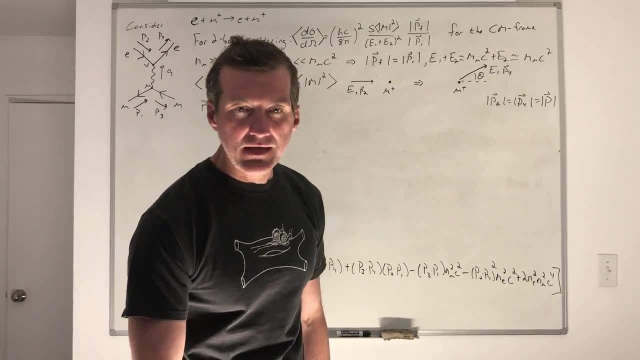 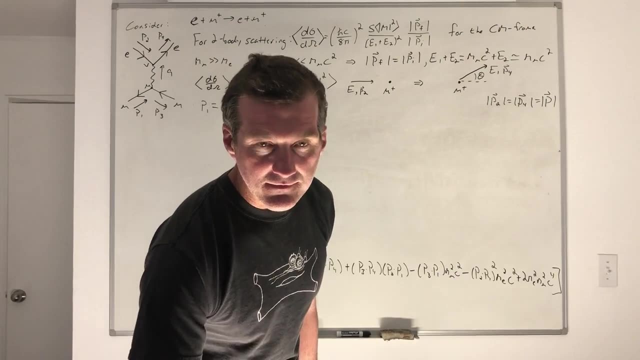 No, I don't see Ryan short. Nico, Are you on? He's not. No, I'm here, Oh you are. Wait, Yeah, no, here. Oh, there you are. You're up in the top left. 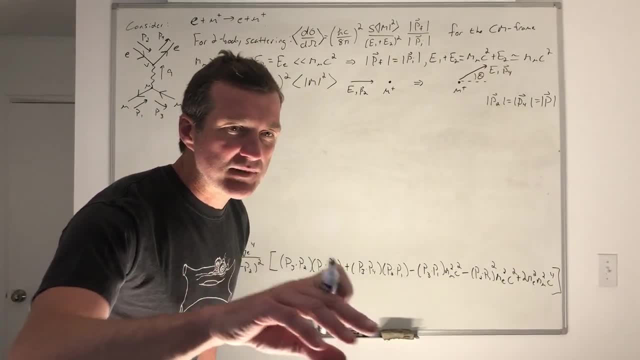 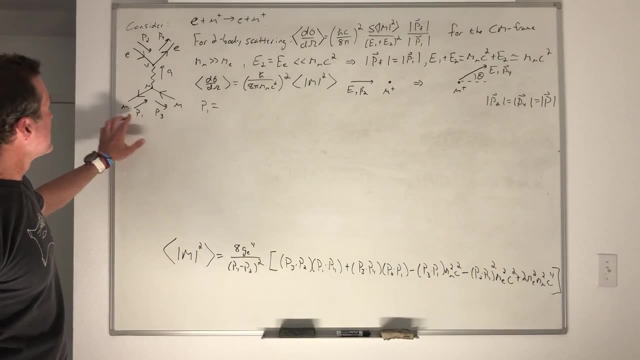 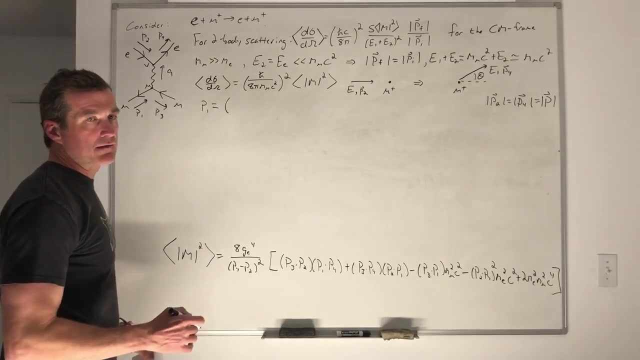 where the light coming in your window is so bright that it obscures your name, which appears on the bottom left. It's okay, Rest in peace. What is the 4-momentum for the p1 particle? So 4-momentum is always energy over C. 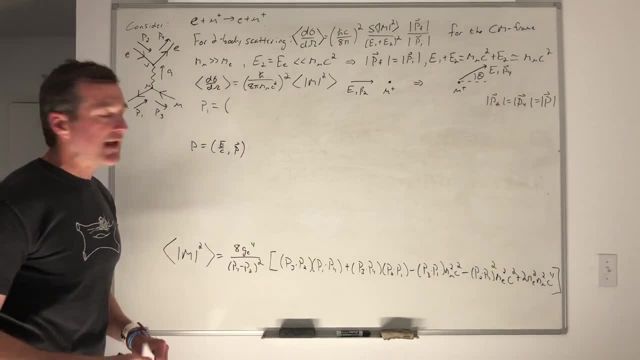 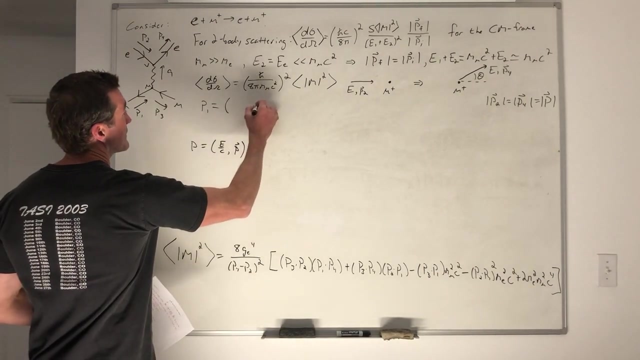 in the timeline direction and the spatial momentum, And this is the relativistic energy and the relativistic spatial momentum. Well, we said that it's not moving. Yes, So no spatial momentum. Exactly, So, it's just its rest energy. Yeah, so this is mu C. 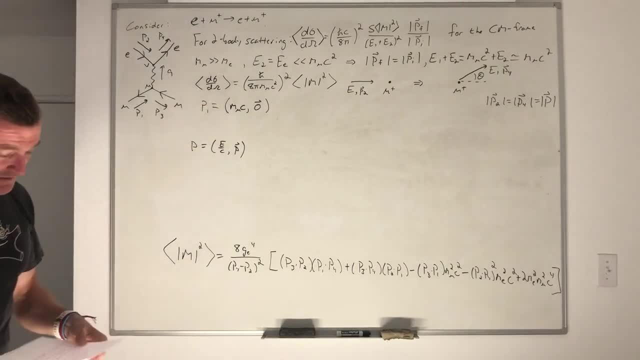 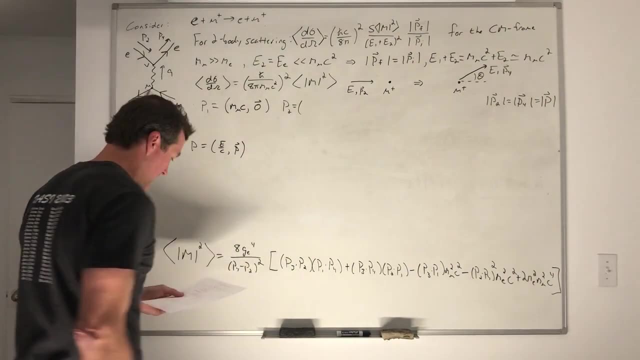 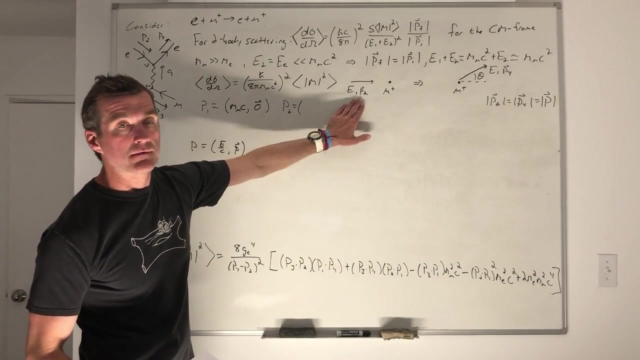 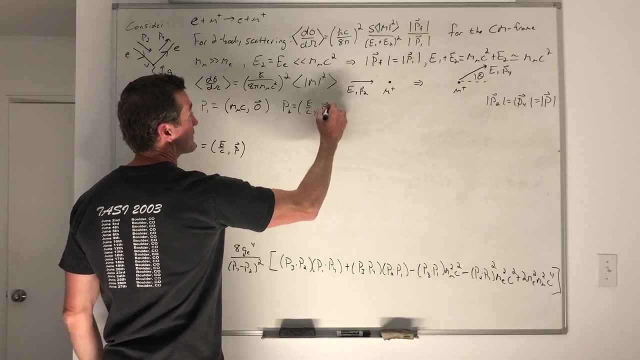 because the rest energy is mc squared. You divide by C, you get mu C. It's not that bad right? Okay, what about p2?? Is E over C? No, no, no, you're totally right, It's exactly that combination of things. 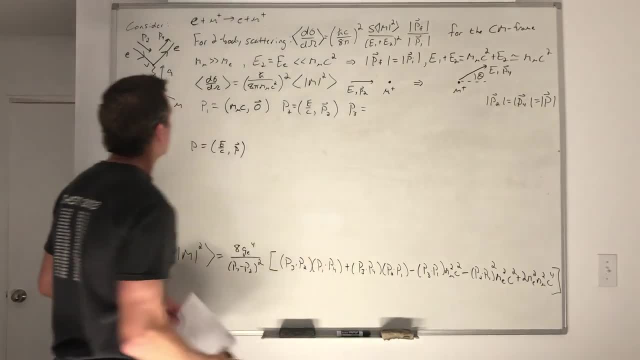 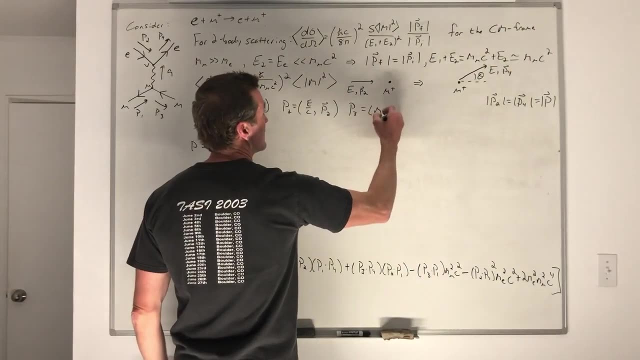 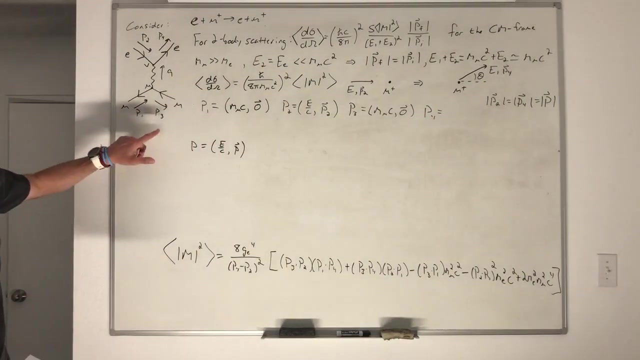 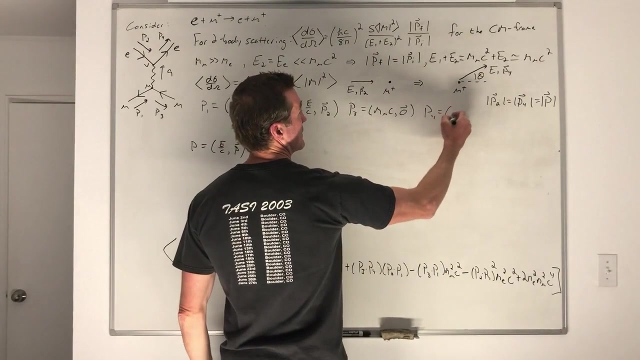 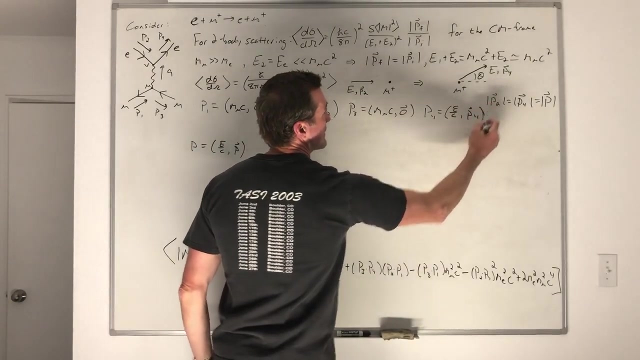 What about p3?? p3 is the p3 is the same as p1? Yes, This is not that bad. Finally, p4. Should be the same as p2, but p4 instead of p2? Yeah, Notice, you might think that these should have. 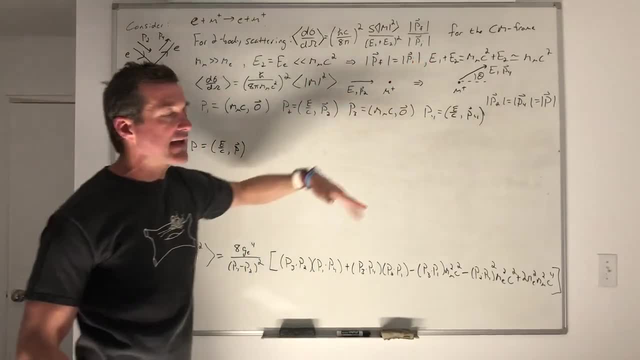 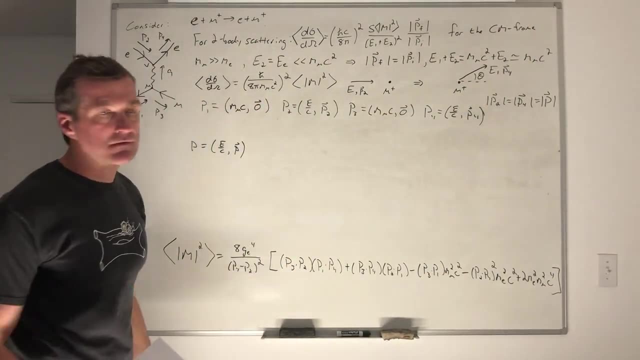 the same 4-momentum, but they could be moving in different directions and that's caught up in the spatial momentum. So we give this a label p2,, we give that a label p4.. They have the same energies, Okay. 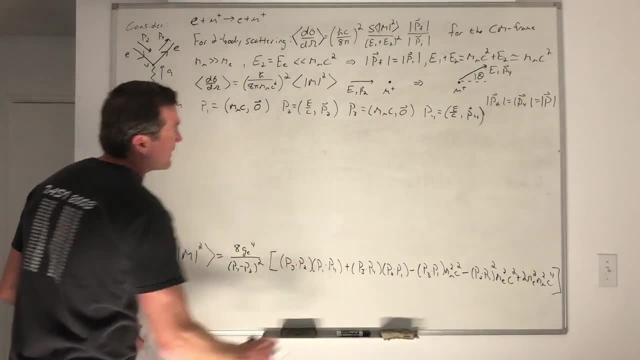 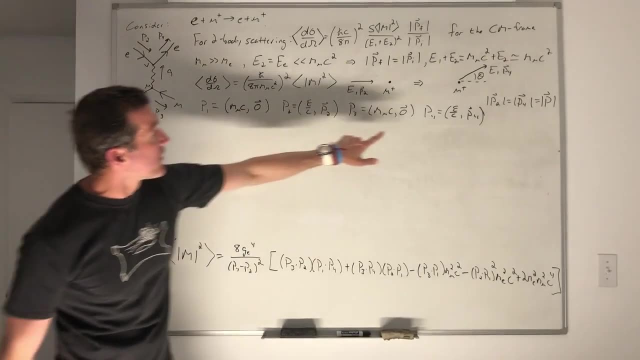 Good job, All right. So all we have to do, Folks, this is simple: We take p1 and we dot it with p4.. That gives us this factor. We take p3 and we dot it with p2.. That gives us this factor. 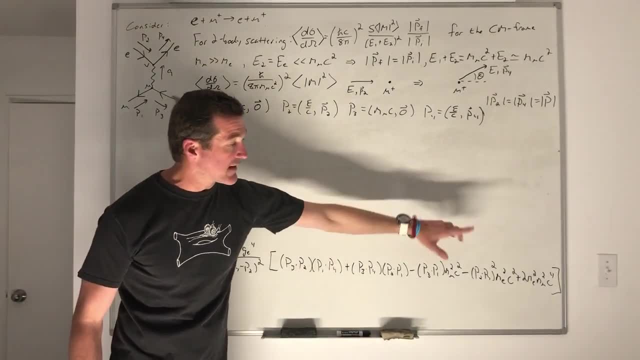 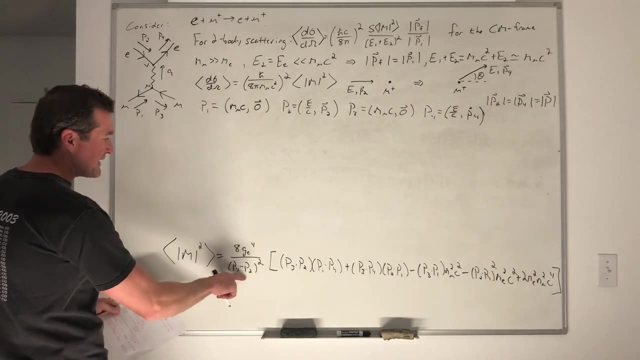 Then we take p3,, dot it with p4, p1, dot it with p2, et cetera, et cetera. We blow this thing out. So here we go. Oh wait a minute, There's this p4 minus p2- crap. 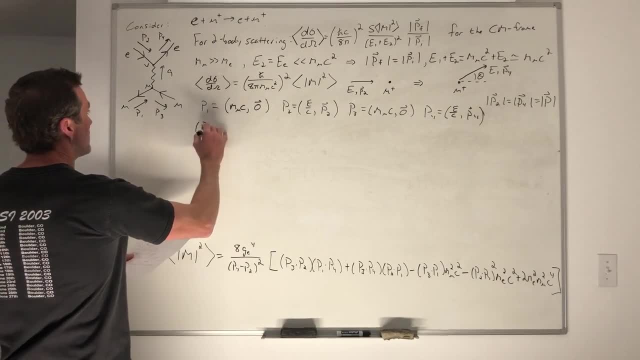 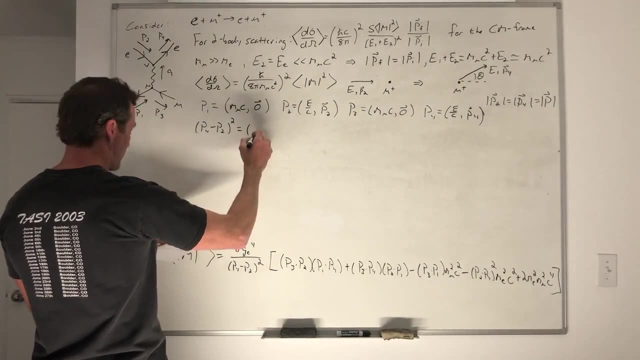 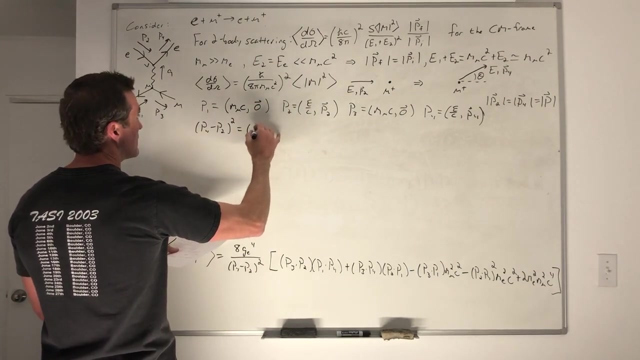 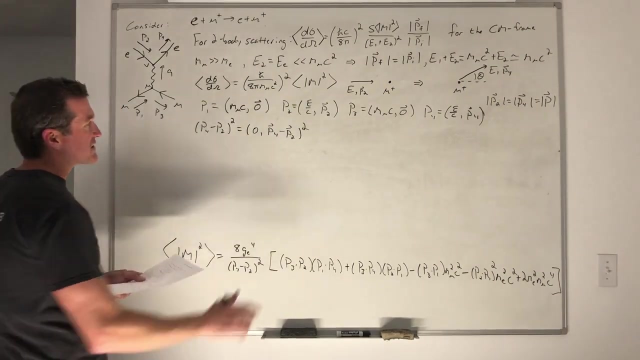 So let's do that first. So p4 minus p2, squared is Well p4 minus p2.. So 4 minus 2.. If the erc's cancel, So that just becomes the square of a 4-vector, that looks like that. 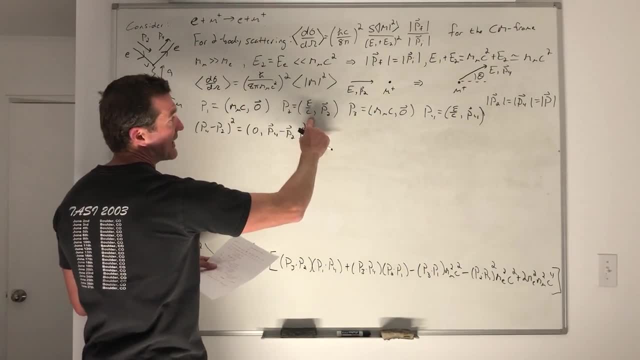 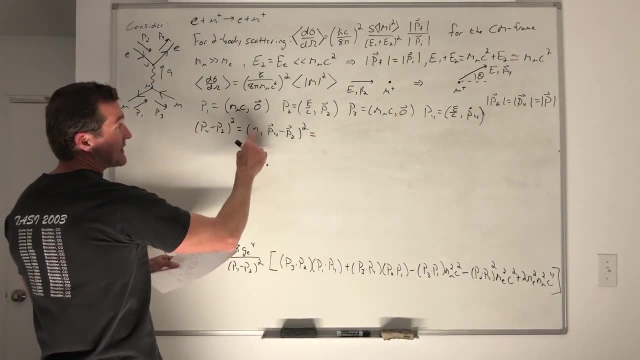 I'm literally taking this and subtracting this from it. So the time-like components cancel The space-like components. just become p4 minus p2.. Okay, If you square this, you get this squared, which is of course 0,. 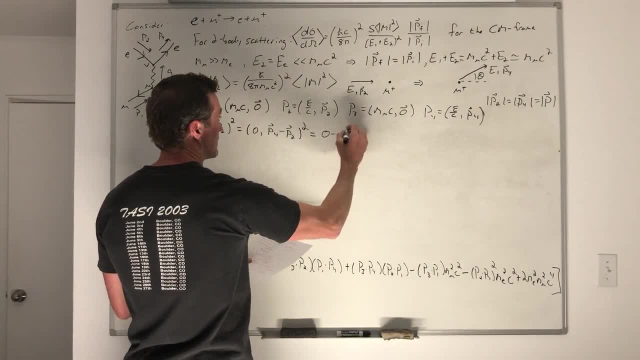 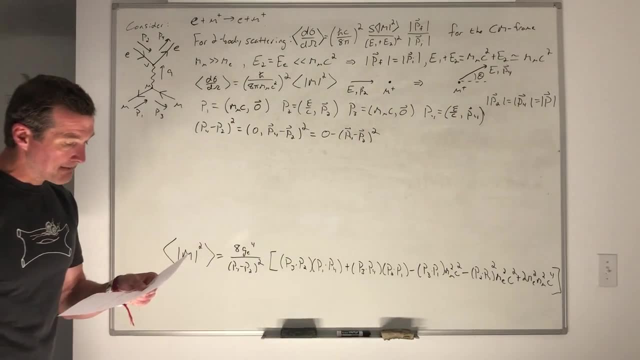 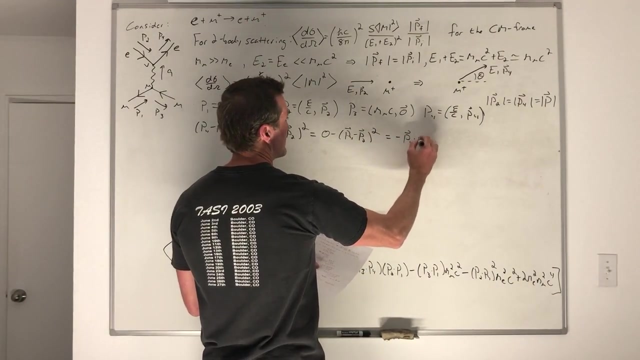 minus this squared, which is 1.. Okay, And now we're just going to clean this up. This is minus p4, dot it with p2.. Oh, sorry, Hold on, I'm going to do it this way. I'm going to do the squares of these first. 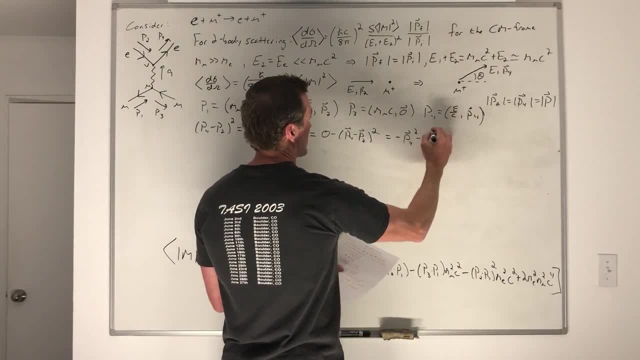 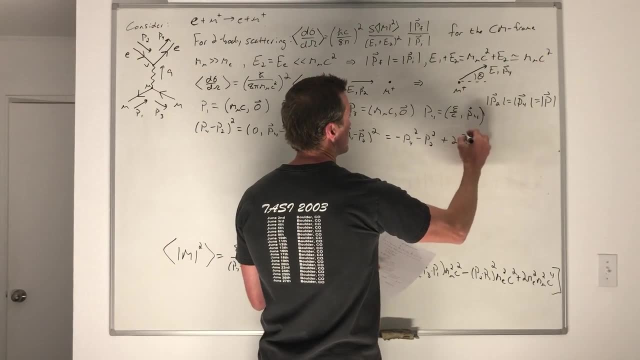 So p4 squared minus p2 squared, And of course I don't need vector signs over them anymore, because I'm taking the dot product Plus 2p2, dotted with p4.. Okay, That should be a manipulation that you're all very comfortable with. 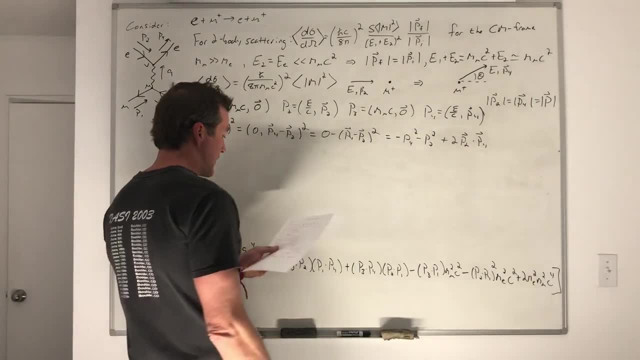 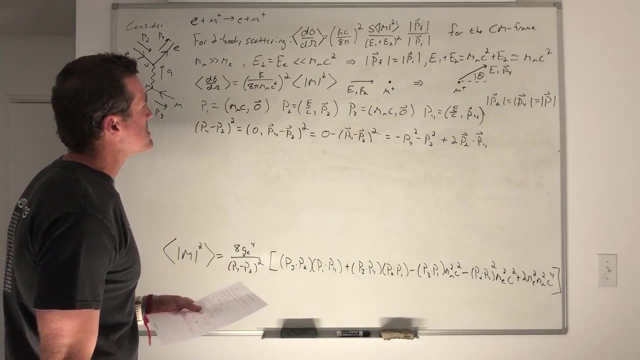 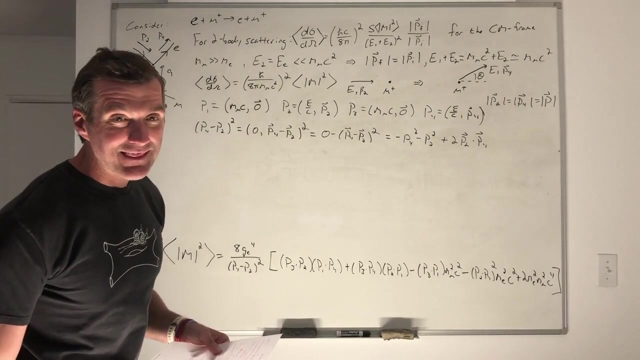 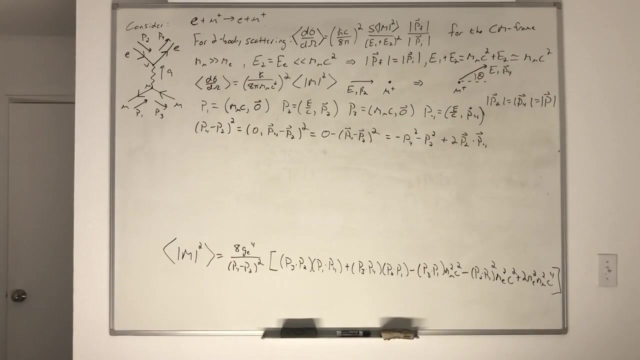 Okay. Oh, wait a minute, So let's head back there, Okay. So that's what I was going to do. I'm going to do this, I'm going to do this, Okay. So there we go. There it is. 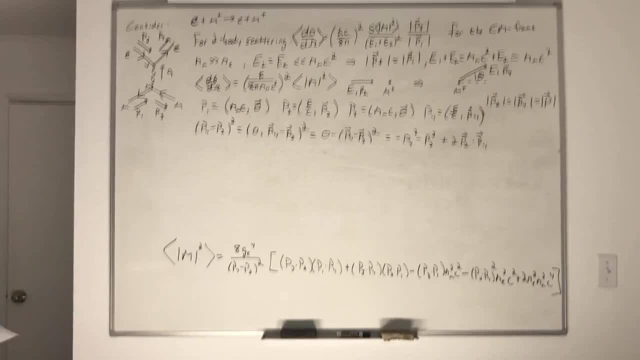 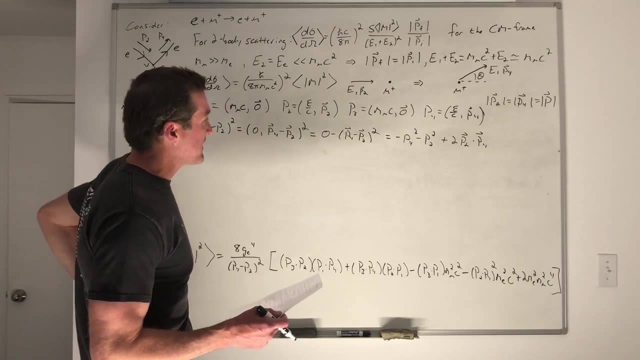 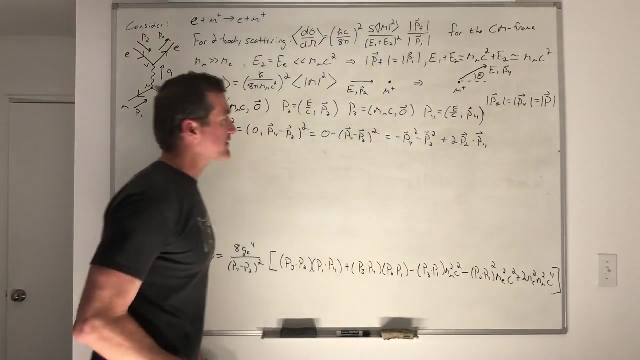 There we go. So there's my dot product. That's the one I'm going to do, And then I'm going to take out my segments here. Is it too much? No, exactly, Okay, so P4 or P. well, actually, yeah, let me put vector signs over these, just to remember that they're three component vectors, not four component vectors. 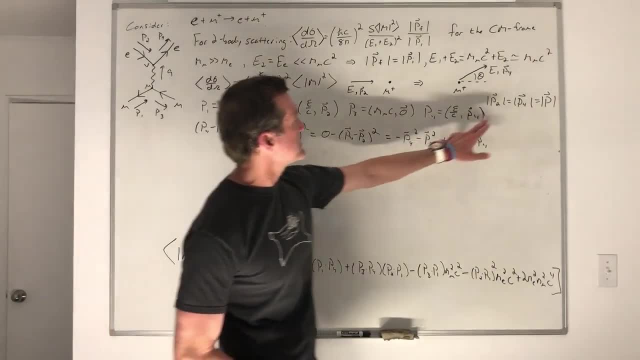 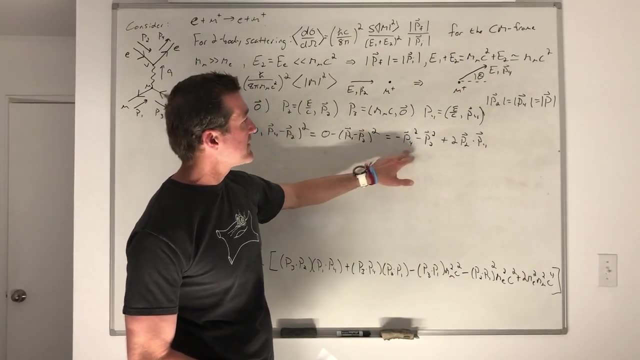 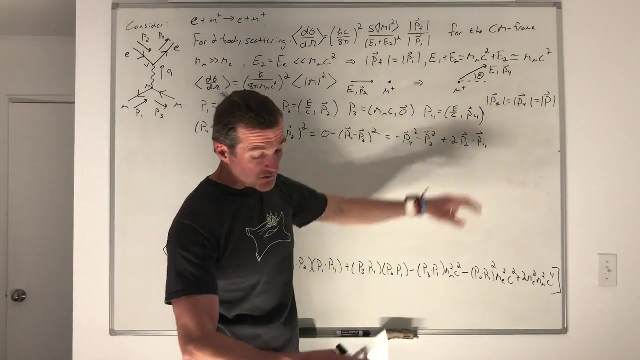 P4,. oh wait a minute. the magnitude of this is the same as the magnitude of this, So I could just call this P squared, and there's two factors of it. so, minus 2P squared, This of course is 2 times P squared, times cosine squared, or cosine of the angle between them. 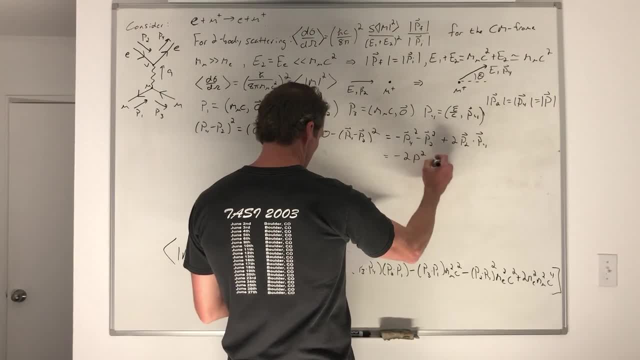 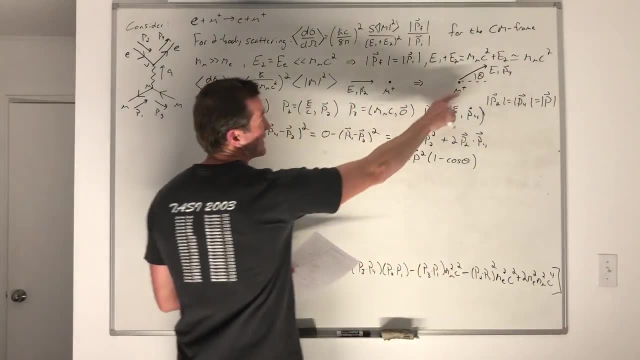 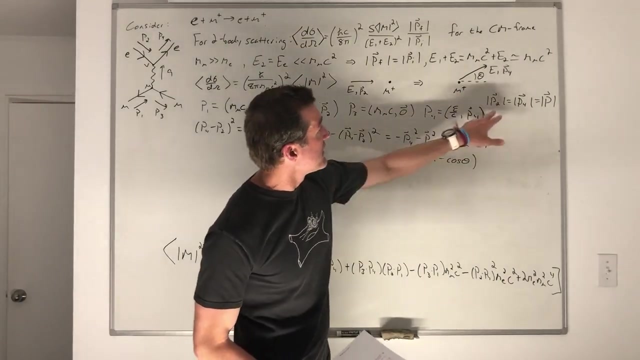 So this simplifies to minus P squared times 1, minus cosine theta, where that theta is the deflection angle. Okay, all I did was I said I'm going to call P2 magnitude P, P4 magnitude P and this is the deflection angle. 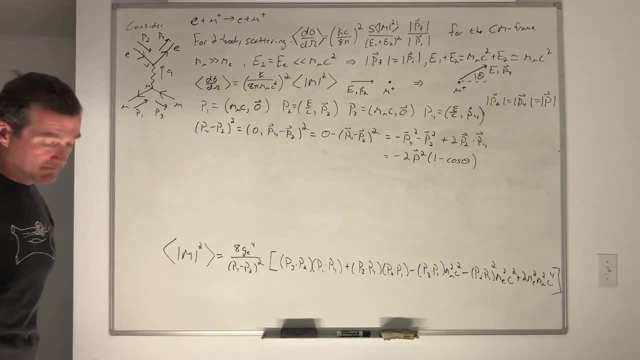 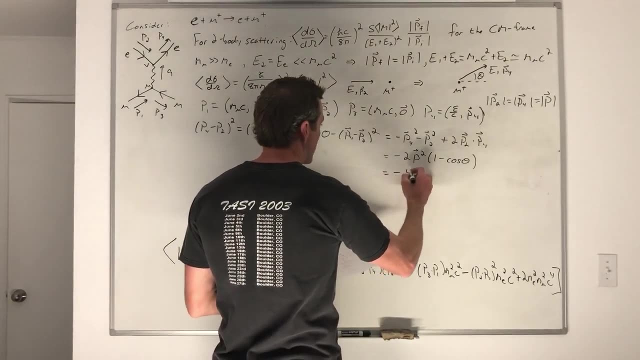 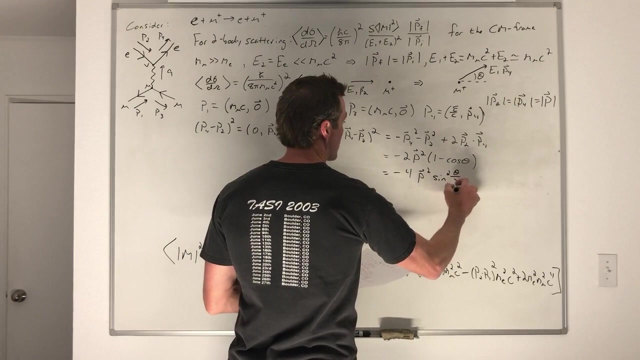 So this is the magnitudes times the cosine of the angle between them. That's it okay. And then, of course, we can use a trig identity to simplify that, and this becomes minus 4 times P, squared times the sine squared of theta over 2.. 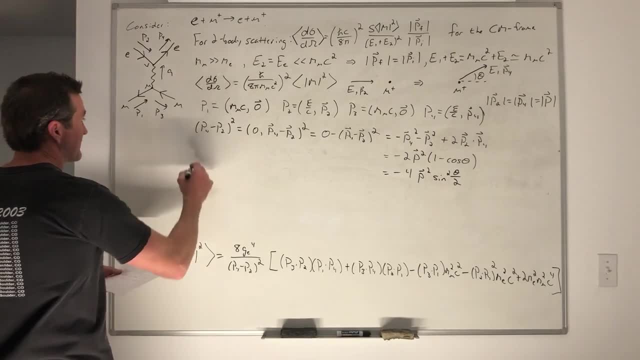 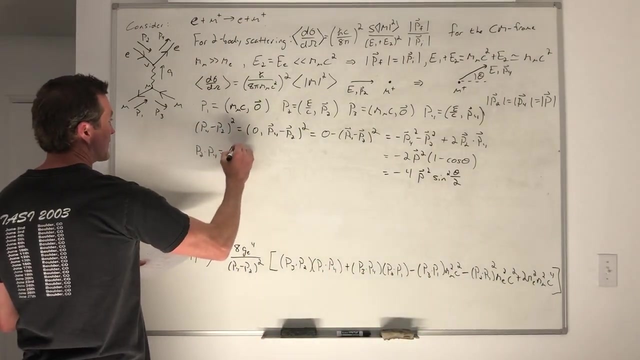 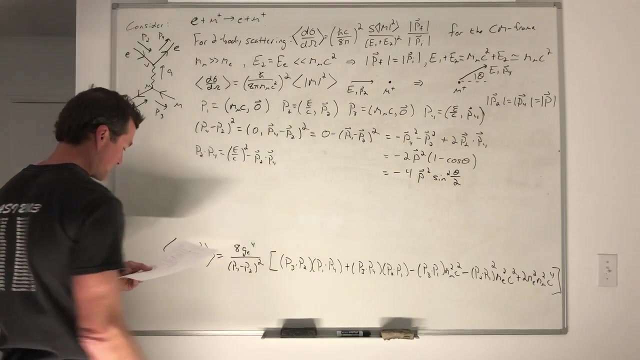 All right, and now let's bang out some other important stuff. okay, So I'm going to do P2 dot P4.. That appears here. P2 dot P4 is E over C squared minus P2 dot P4.. All right. 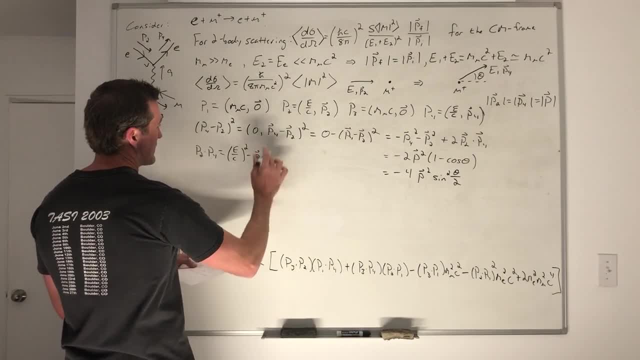 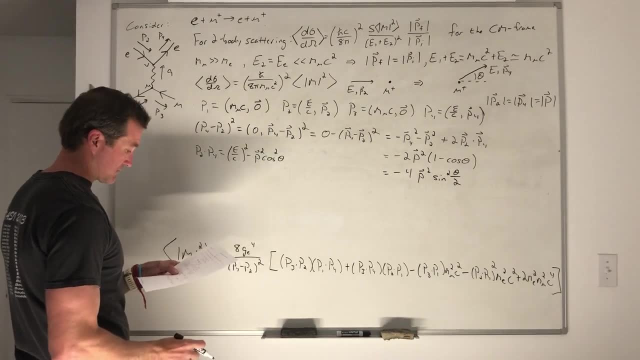 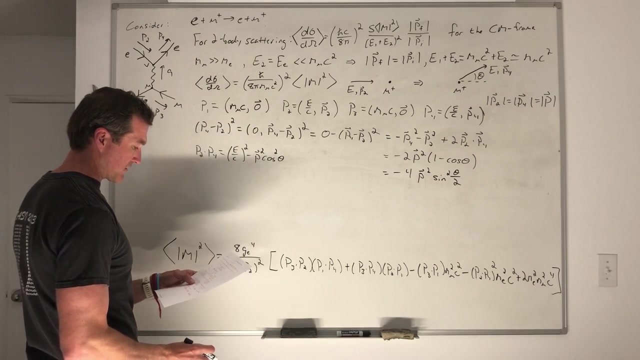 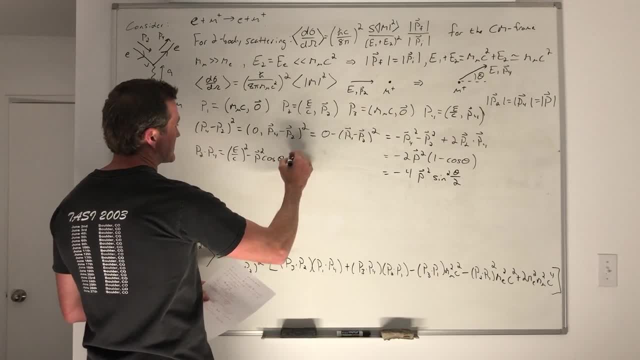 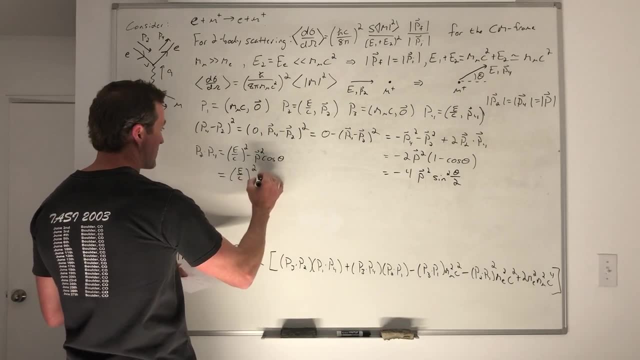 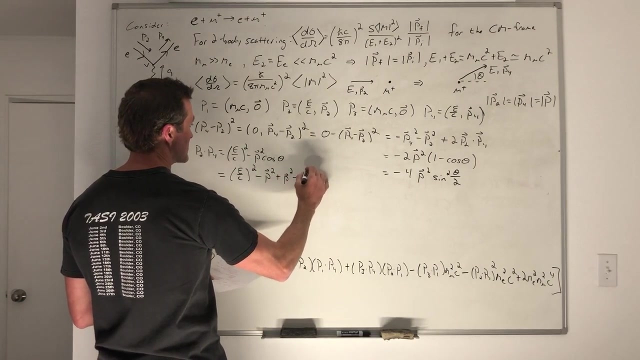 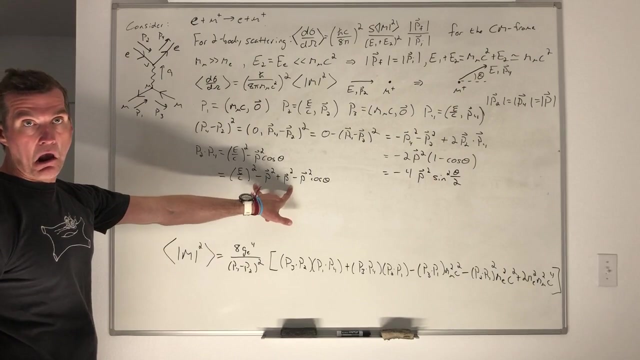 Okay, and then we can do something interesting with this, Because what we can say is: E over C squared minus P squared plus P squared minus P squared cosine theta. That's putting in just a demonic factor of zero. However, what is that equal to? 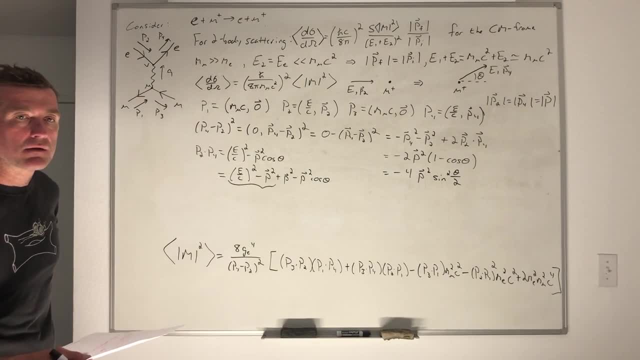 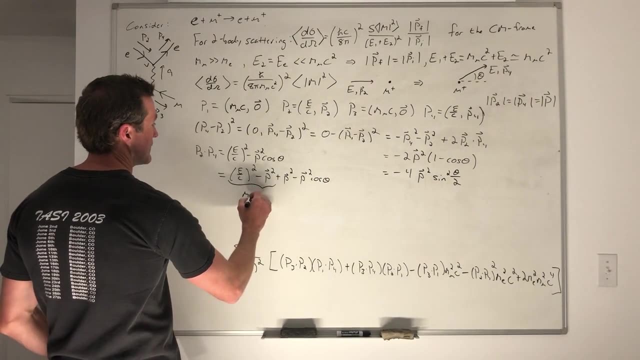 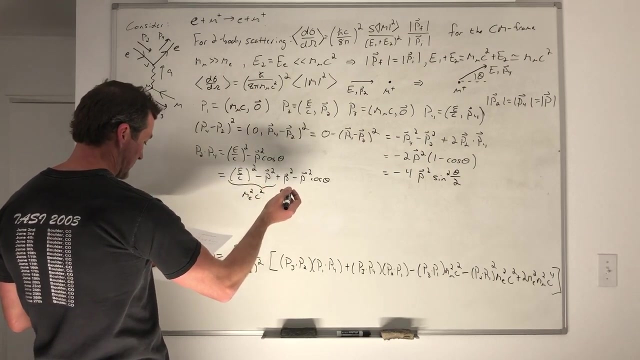 E over C squared, minus E over C squared, minus spatial momentum squared. Can anybody That's M? M2 C squared or M2 squared C to the fourth? Yeah, so this is actually M? E squared C squared. It's actually just M E squared C squared. 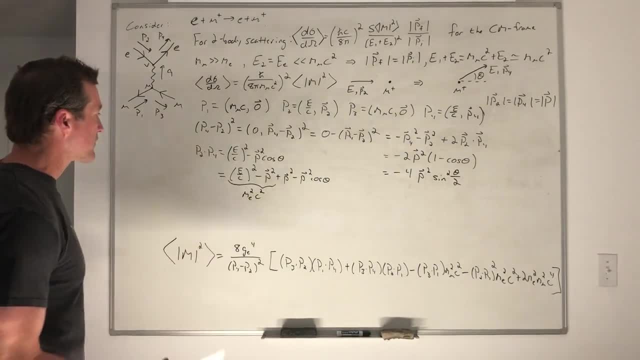 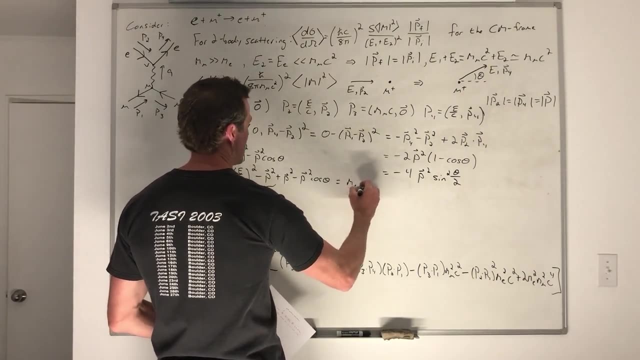 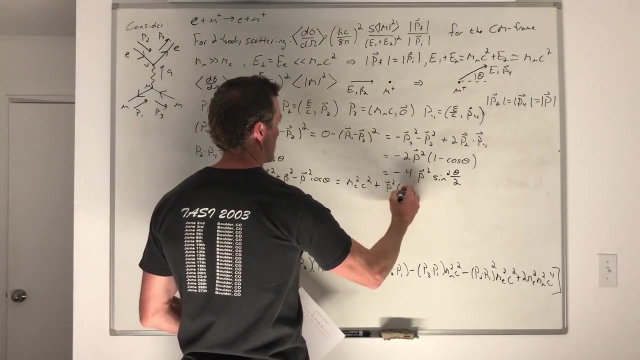 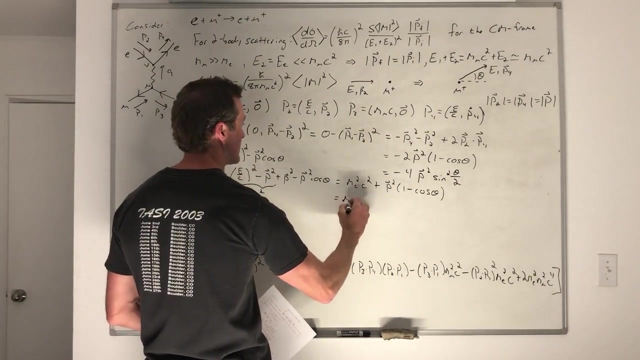 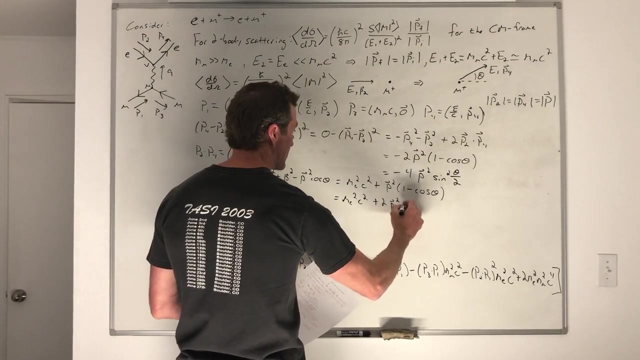 If we do E minus P squared, C squared, then it becomes M squared C to the fourth. okay, So this is going to simplify To M E squared, C squared. Ho ho, Look at that. There it is Okay. so in the end we get M E squared, C squared, plus 2P squared, sine squared, theta over 2 for that guy. 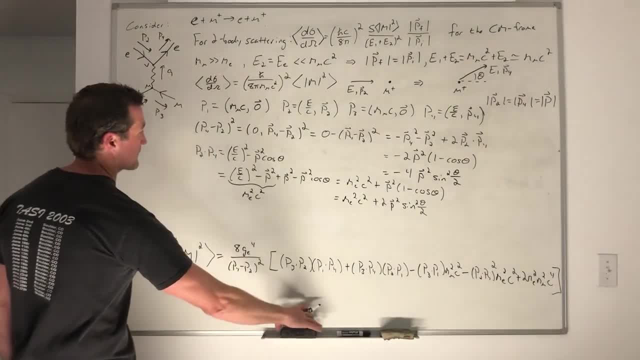 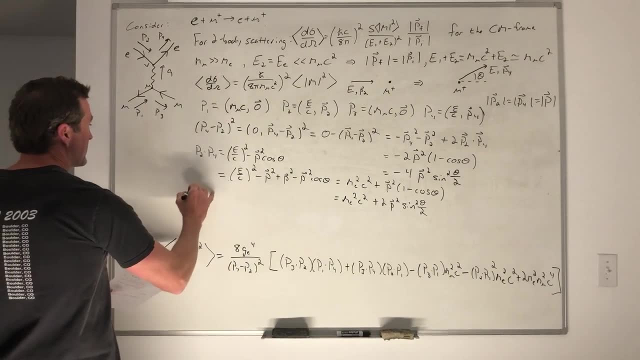 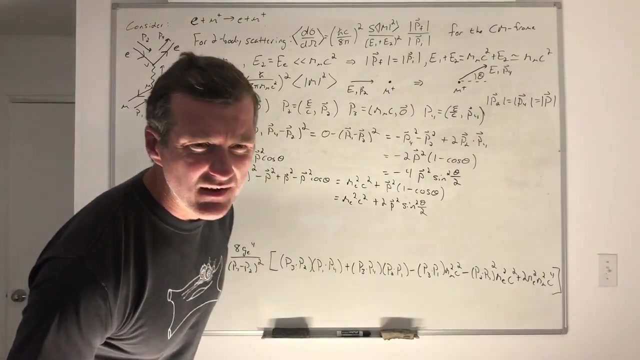 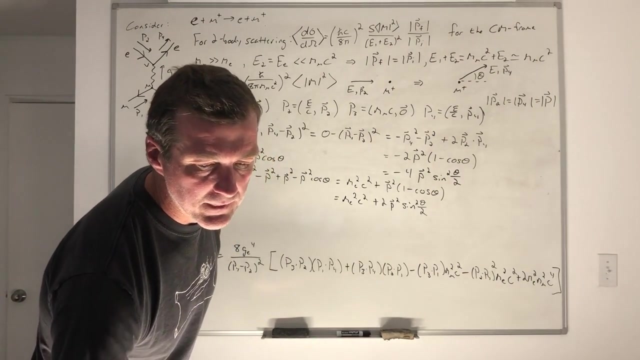 Okay, Okay. Now the other dot products we need are much easier: P1, dot, P3.. Let me get a victim, Eric, Are you there, Eric? I don't see Eric Man. Daniel, Is Daniel out? Oh, Daniel's out there. 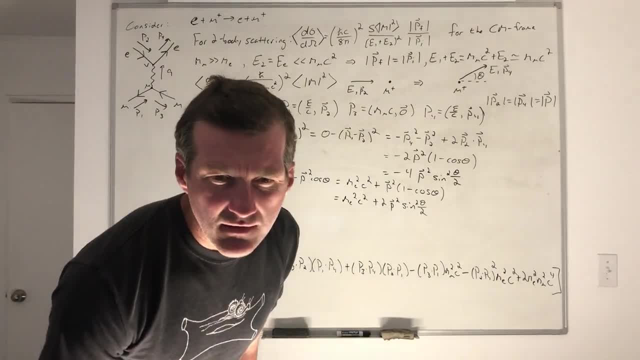 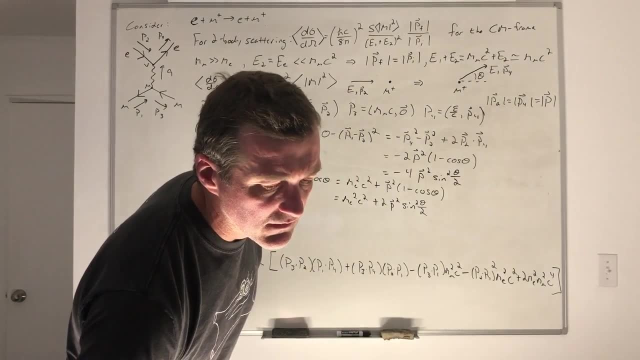 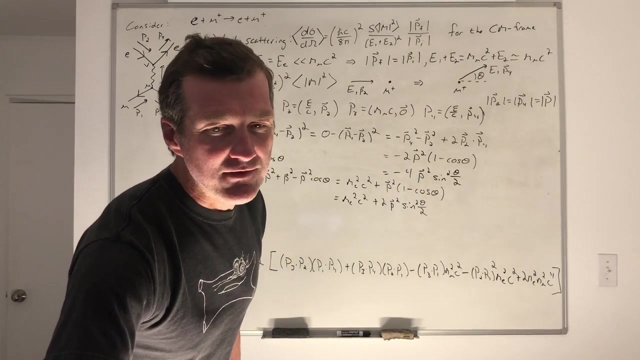 Wait, Eric is here. I think I just might not be working. Oh yeah, no, Eric is here. Eric is here. Say something, Eric. Oh, his microphone isn't working. He just chatted that out, Okay. 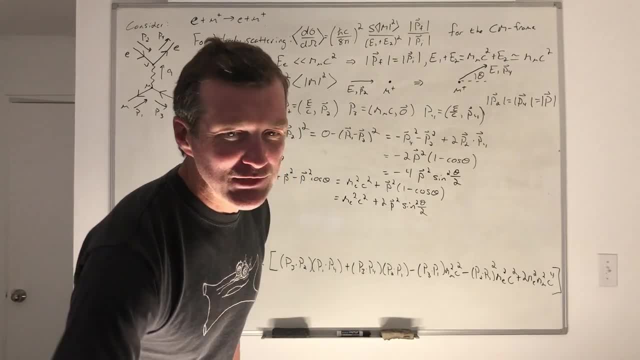 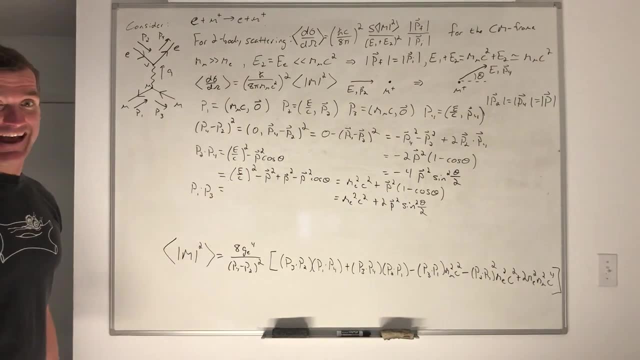 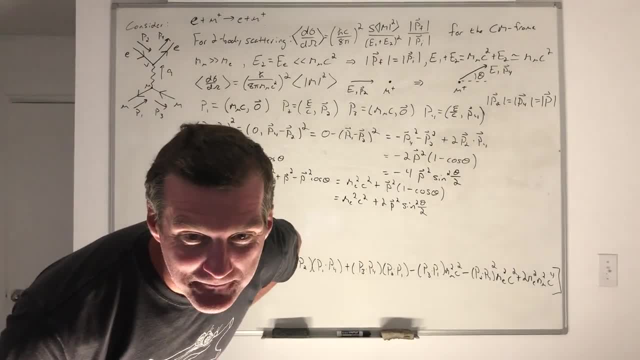 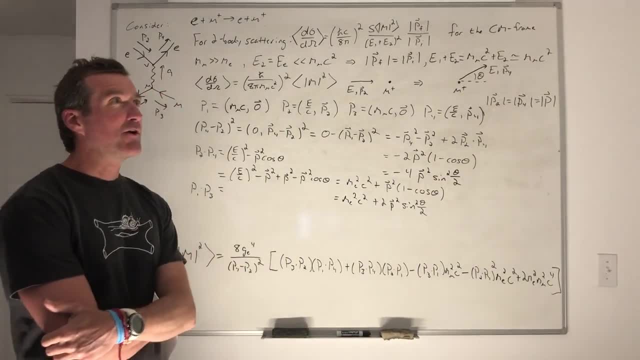 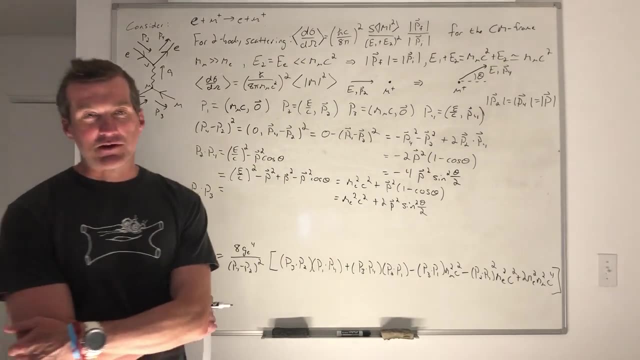 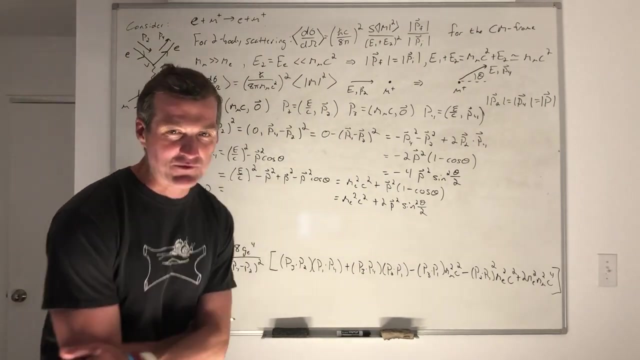 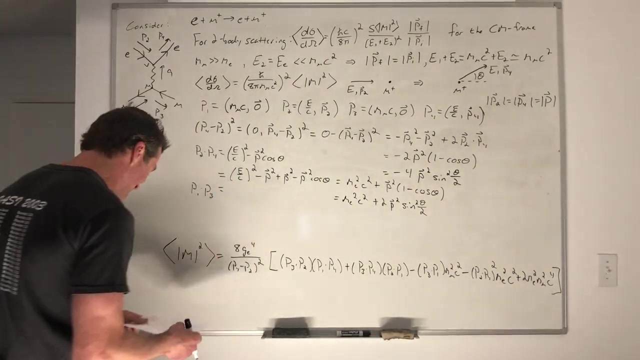 P1, dot, P3.. P1, dot, P3.. Oh, gimme a home Where the buffalo roam, Where the deer and the antelope play, Where seldom is heard A discouraging word. Okay, Alright, Ah, There we go, There we go. 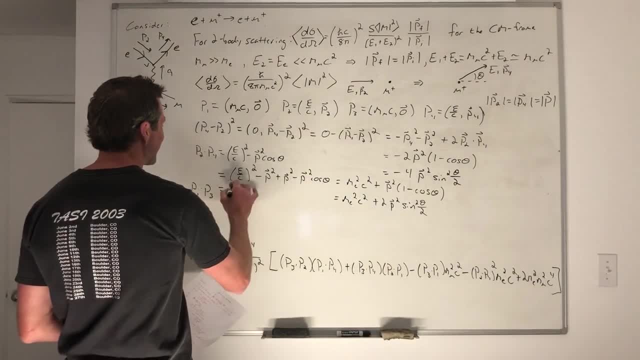 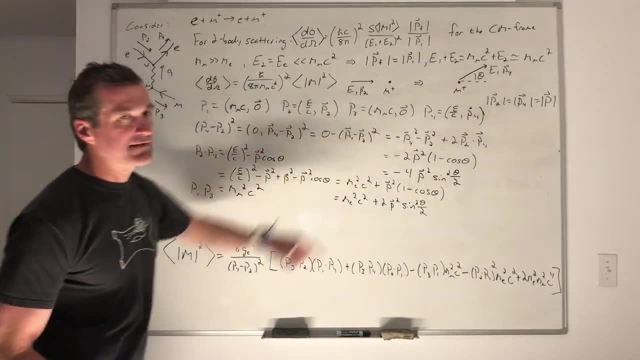 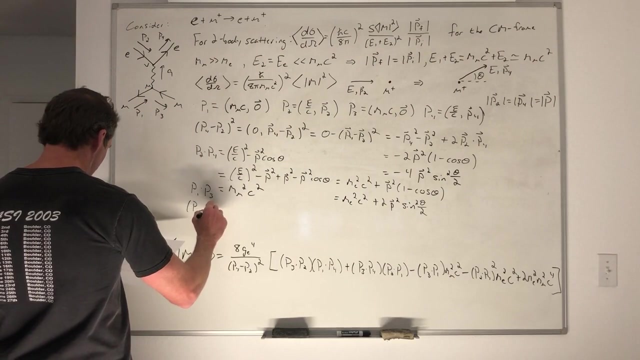 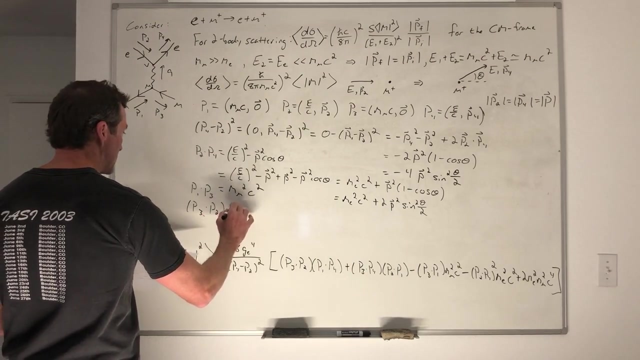 good, good. so this is just mu squared, c squared. all right, p1 dot p3. oh, look at that. p1 dot p3. that's pretty easy. i only asked him the easy one, okay. and then uh, p1 dotted with, or sorry, p3 dotted with p2. p1 dotted with p4. 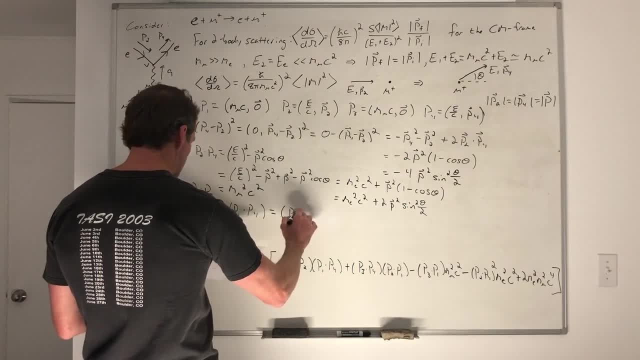 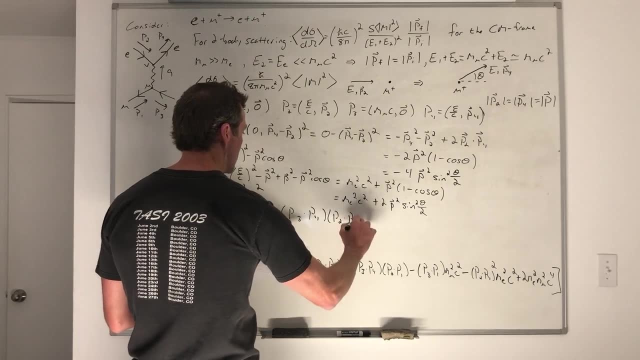 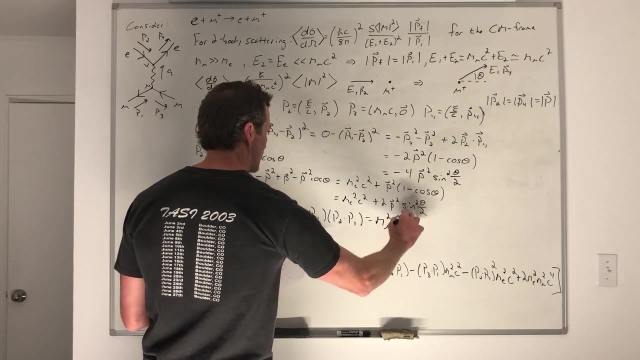 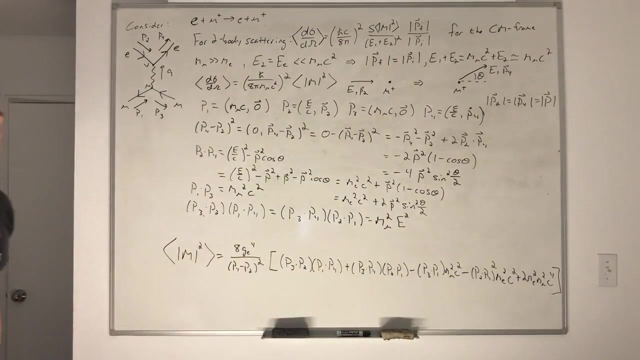 which happens to be the same as p3 dotted with p4 and p2 dotted with p1. this just comes out to be the mass of mu squared times the energy of the electron squared. okay, so this is all the momentum factors that we need, so now we're in a position to plug all of this in. 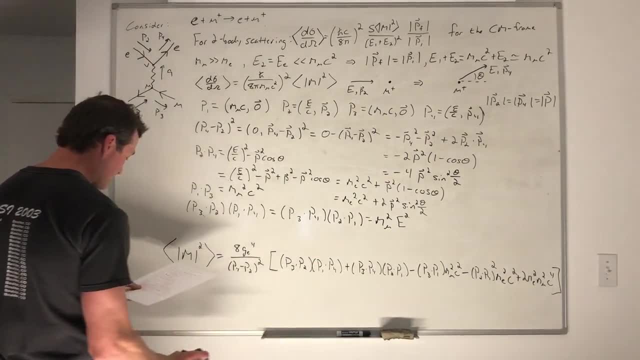 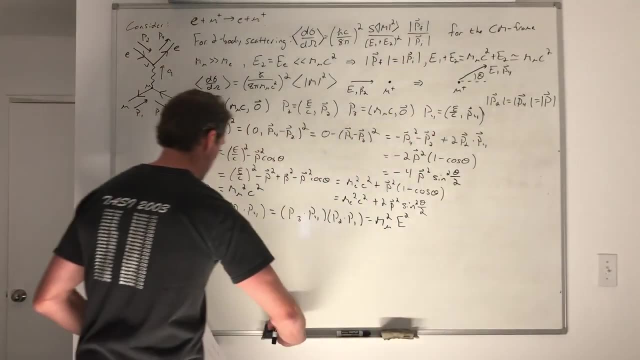 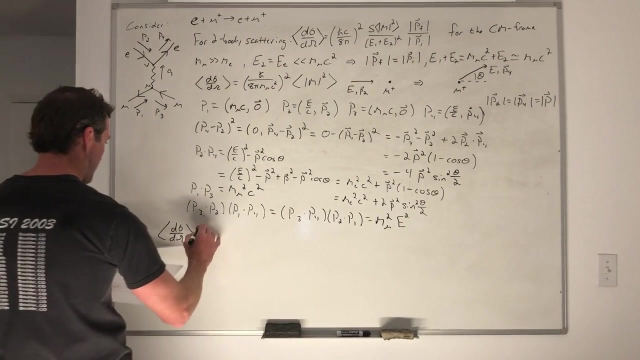 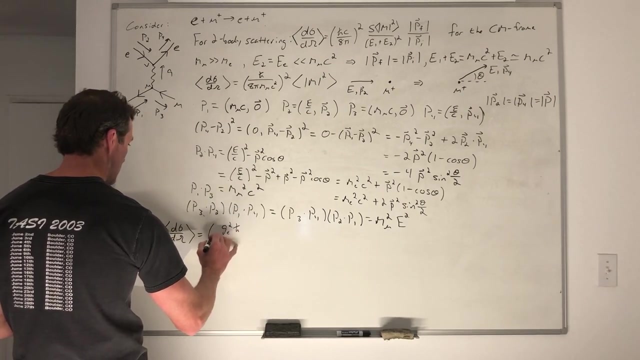 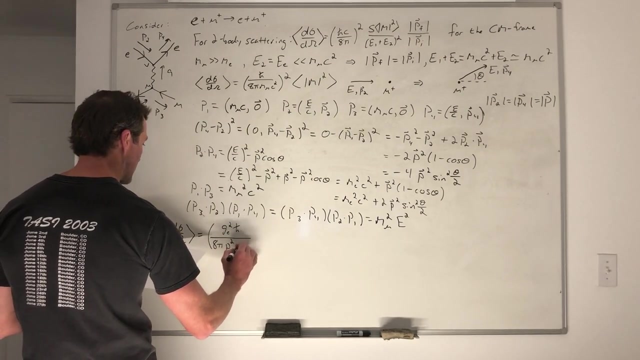 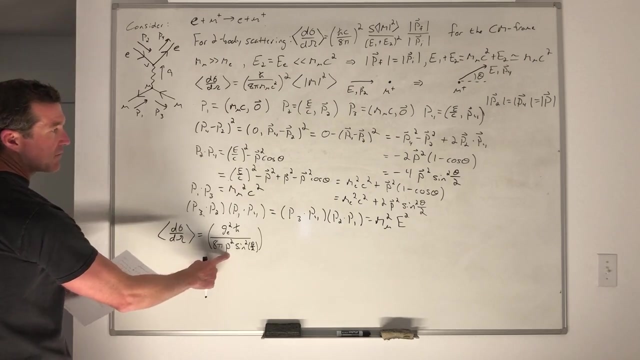 and there is a beautiful simplification that comes out of it, and i'm just going to erase this and write the n sub g e squared h bar over 8 pi times p squared times sine, squared theta over 2.. okay, this is just the magnitude of the only non-zero spatial momentum. 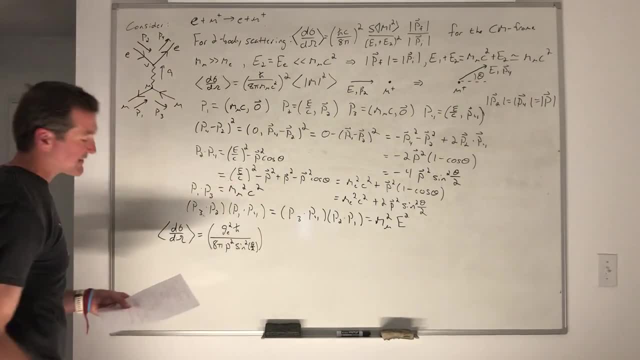 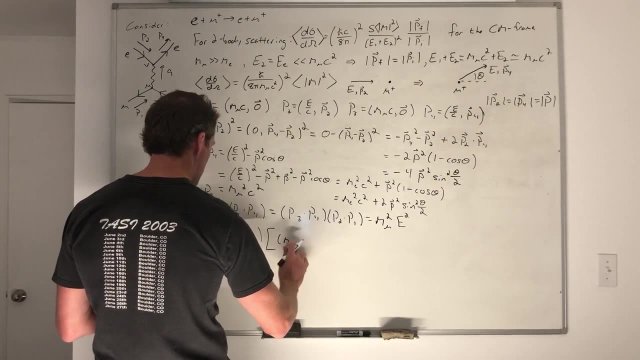 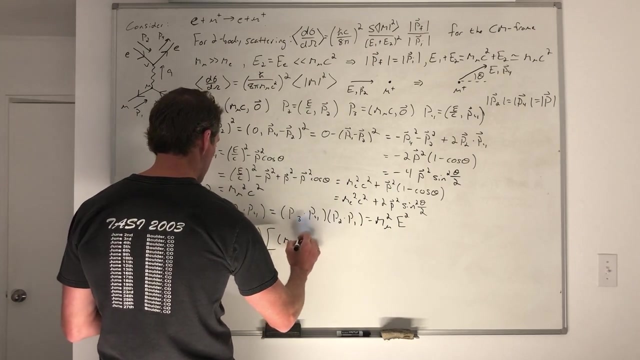 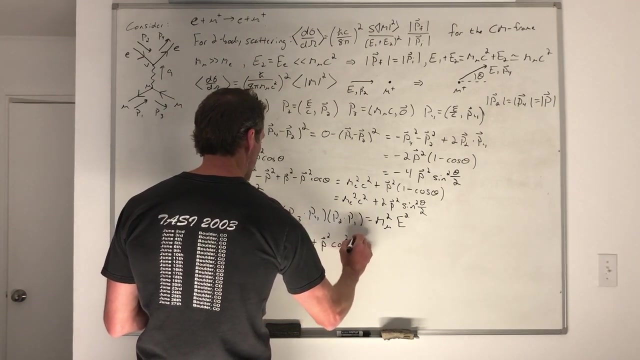 it can be the magnitude of the incoming or the outgoing, it doesn't matter, it's the same times. m mu sorry. m e c squared no hold on. no, no, no, no. m e c squared plus p squared, cosine squared, theta over 2.. has anybody ever seen that formula before? 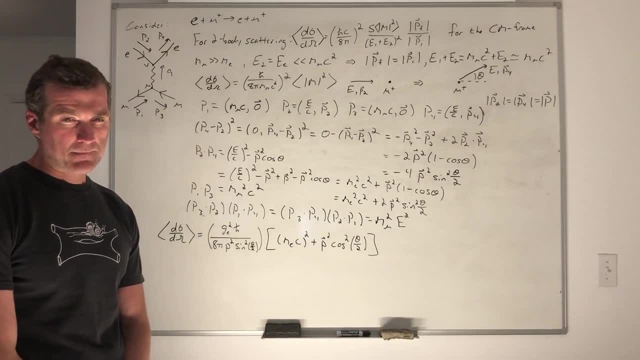 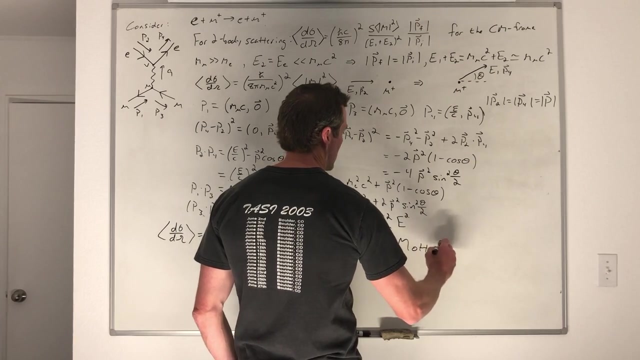 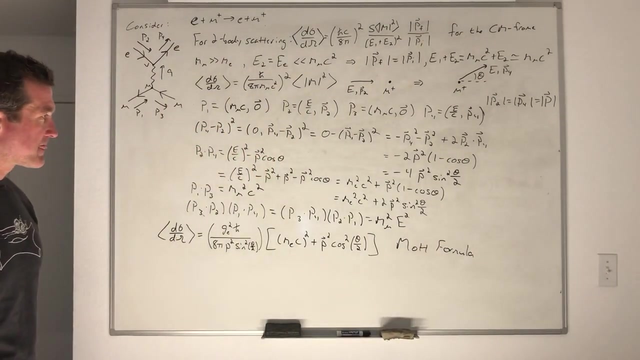 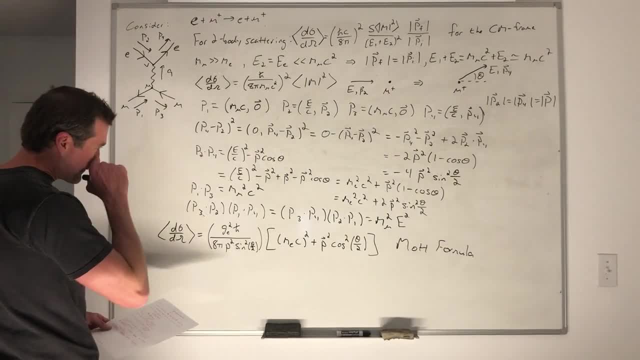 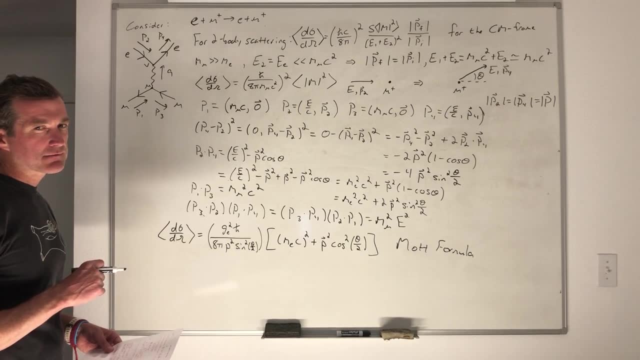 however, um, the mott formula might not be that familiar to you, because this is relativistic scattering. We really like non-relativistic scattering. So if I want to break this down to a non-relativistic scattering, all we do is we take the magnitude of the spatial momentum as being 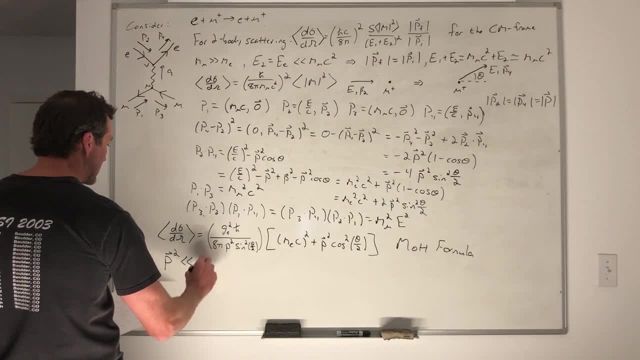 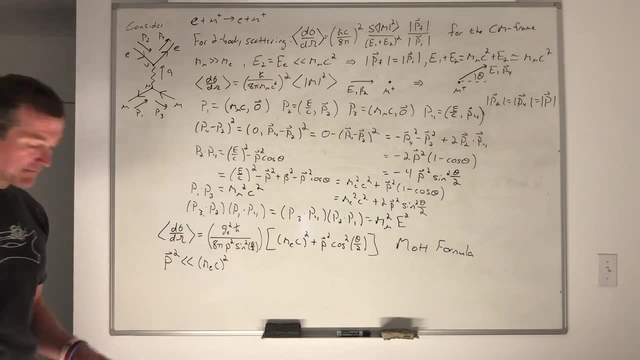 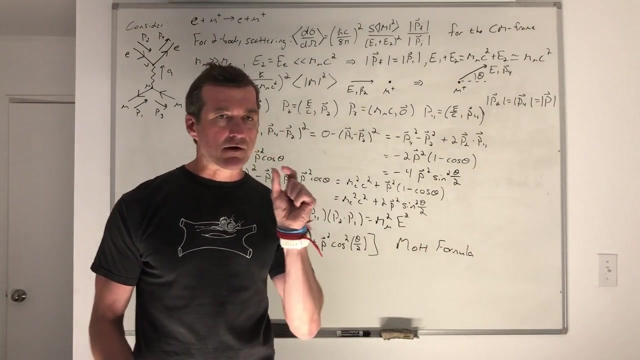 of the electron as being way, way less than essentially the magnitude of the energy. the rest energy, Okay, And that's one way to take the non-relativistic limit. in many cases, If you have massive particles, you take their momentum of motion. 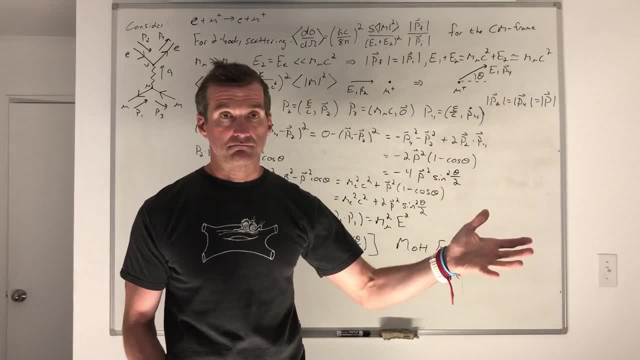 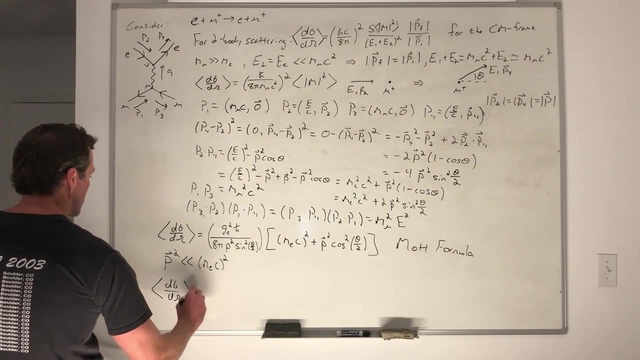 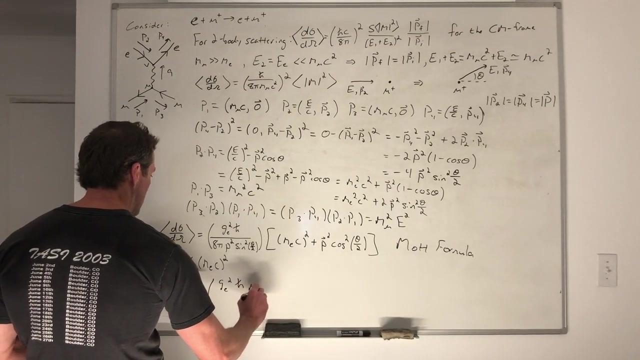 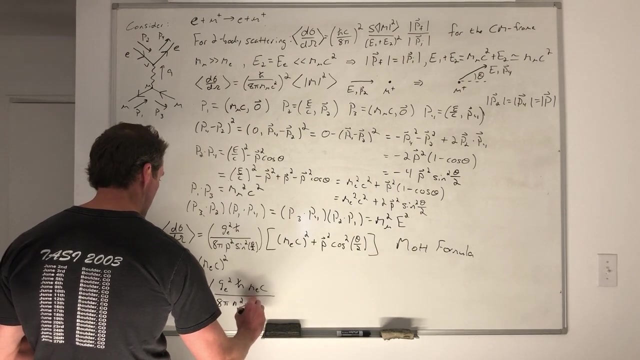 and you make it much, much smaller than the rest of mass energy. Okay, But if we do that, then this becomes d sigma, d omega is ge squared h, bar mec over 8. pi me squared v squared sine. Okay, So this is the non-relativistic momentum that we're going to be taking. 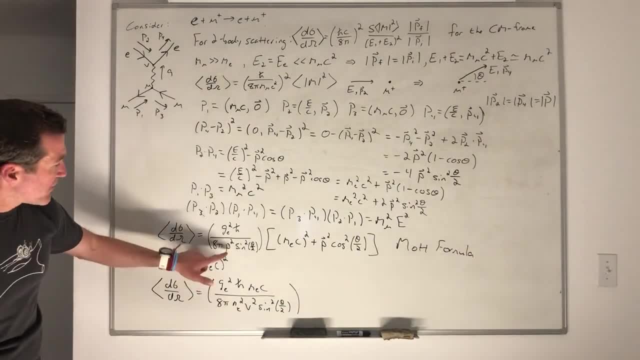 So we're going to be taking gamma to be 1 and we're going to be taking gamma to be 1.. Okay, Notice, I plugged in m squared, v squared instead of p squared, because this is the relativistic momentum, This is gamma mv. 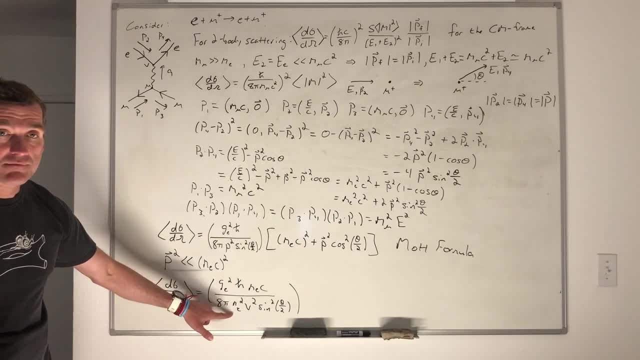 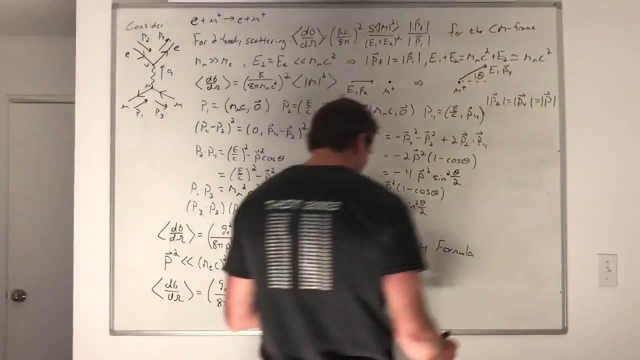 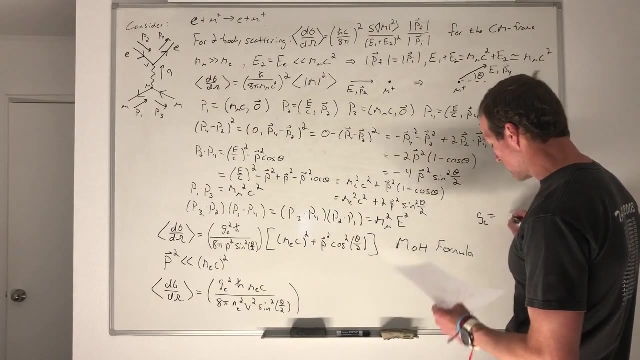 But if we're non-relativistic, we're basically taking gamma to be 1.. So this momentum becomes m squared, v squared or it becomes mv. Okay, Now, if we do a little substitution dance and we remember that ge the coupling is e times the square root. 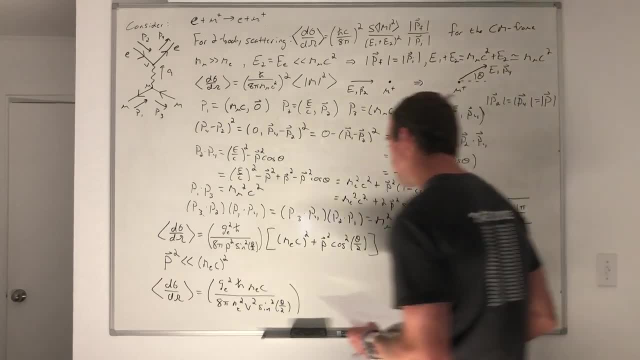 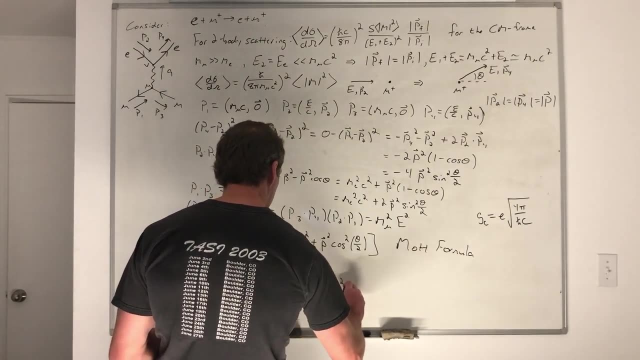 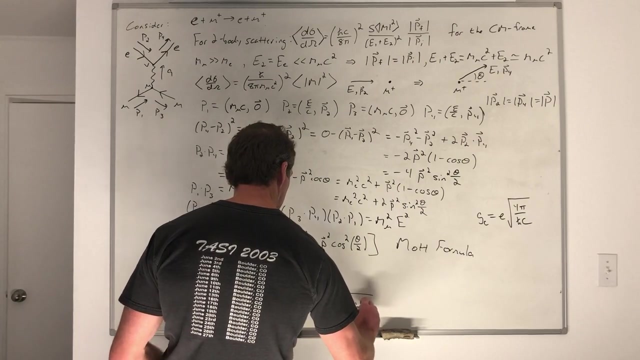 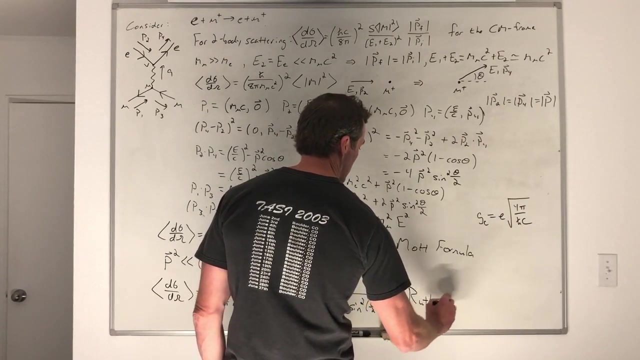 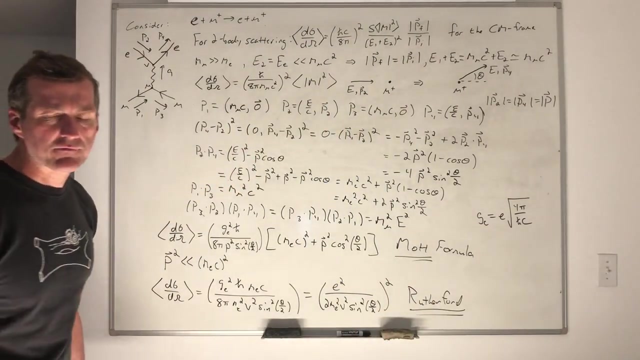 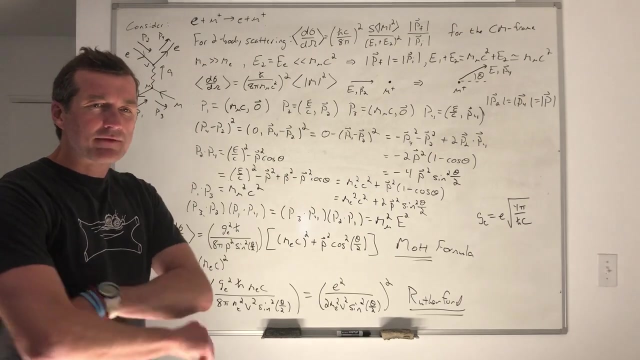 of 4 pi over h bar c, and we use that in here. this cleans up a little bit to something which is hopefully familiar. This is the Rutherford formula. How many of you have seen the Rutherford formula? Really, You've never seen the Rutherford formula. 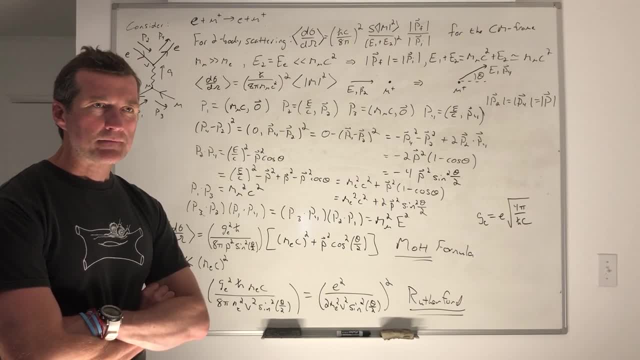 That's incredible. Was that in the modern? Did we do that in the modern? I'm not sure what class you should have seen it in, but you should have seen it. I think we saw it in advanced to something we did. You saw it in what class. 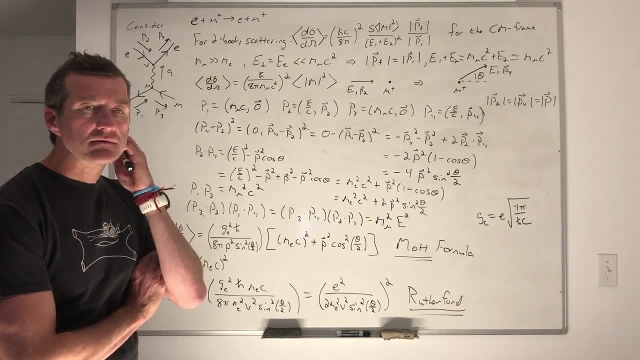 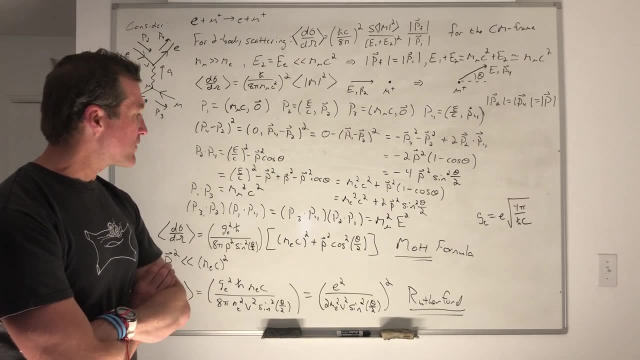 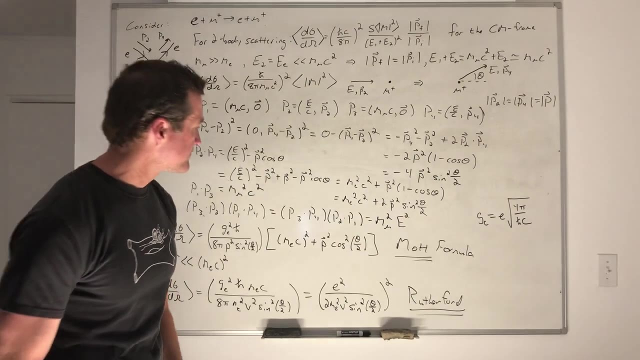 Advanced c and n. Okay, yeah, that makes sense, All right, But it wasn't in a different form though. Yeah well, there's different forms you can achieve by swapping out constants. So I don't want to, I don't want to try and change it up on you. 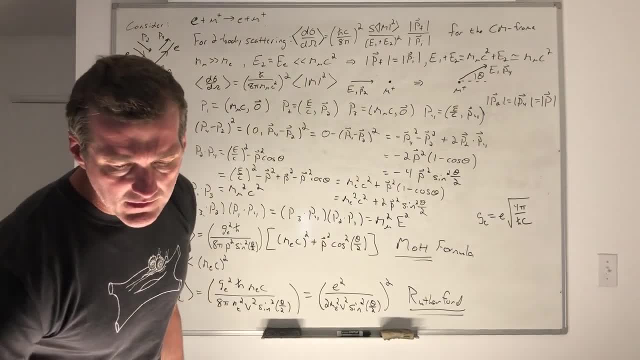 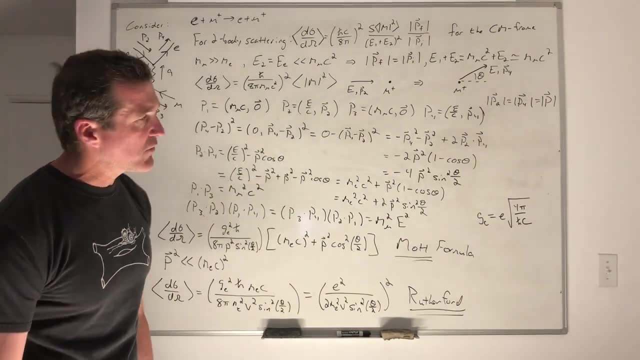 But there you go. So what we've done is we've used these rules, this you know. I'll walk through the process in detail again from the start, But we use basically the Feynman, the Feynman diagram approach to calculating m. 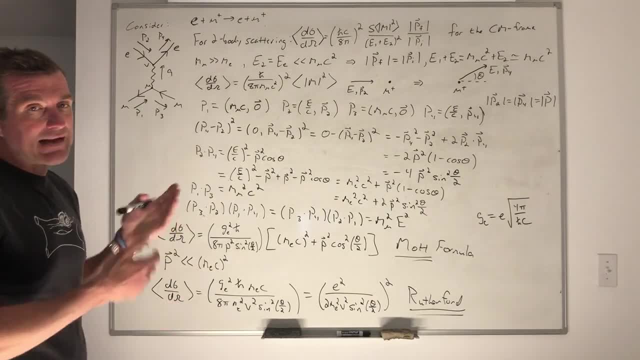 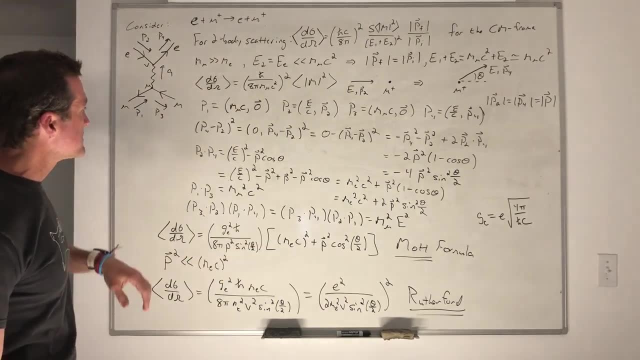 And then we use these tricks to sum over the spins so that we can average over the incoming spins by summing and then dividing by a factor and then summing over the outgoing spins And then using the trace identities of the gamma matrices, that got rid of all of the spin. 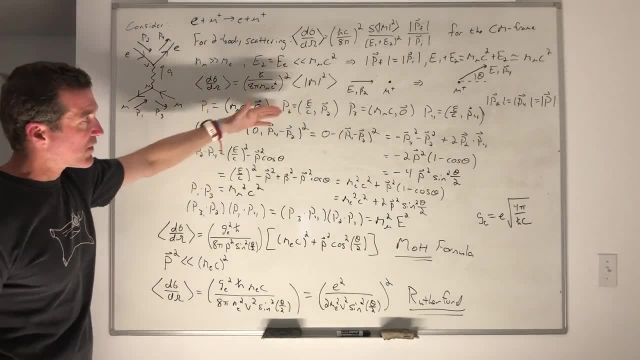 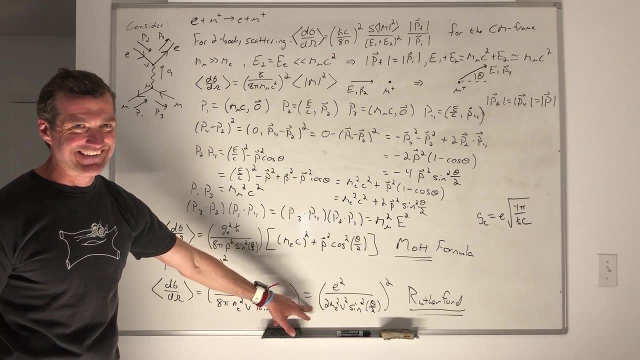 oil stuff, which left us just with momenta. And then we actually worked out the details of the momenta And lo and behold, there is our numerical answer. It's a number. God, that's so sweet. Okay, All right. 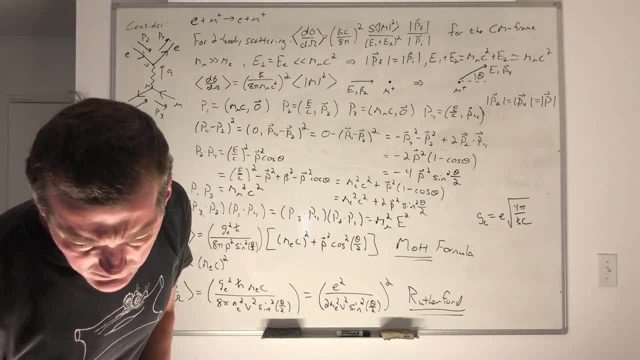 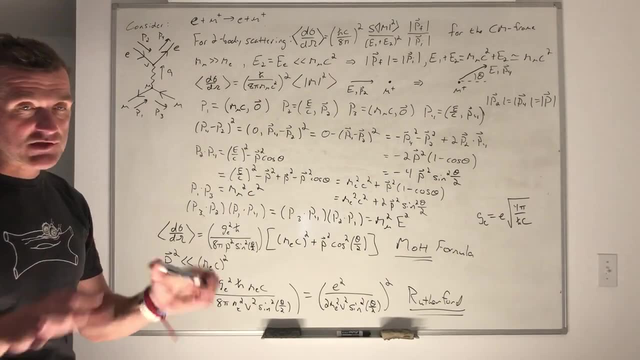 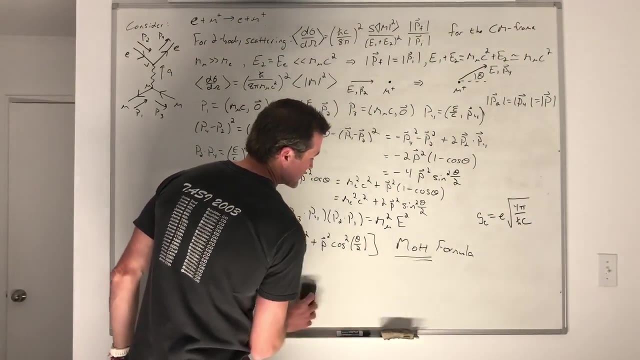 So I'm going to finish up with one more idea that I have to throw at you, And then this means that next time we can just start from scratch with QCD. But there's one aspect of the diagram which I haven't actually told you how to handle. 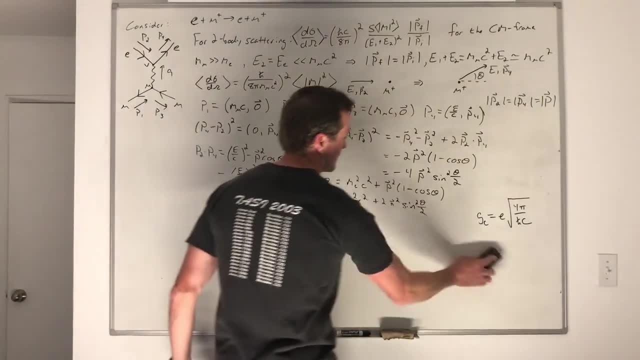 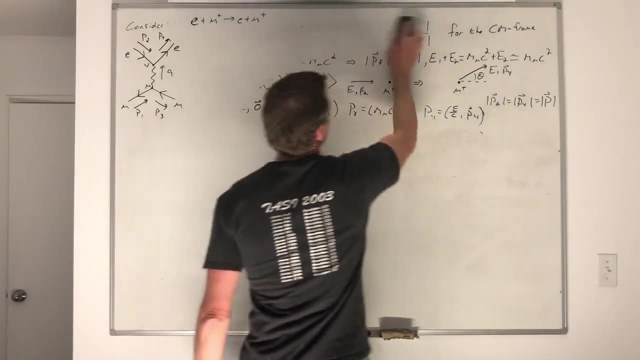 And I need to tell you how to handle that very quickly, And then we'll go. So if we can set up a little bit of time, we're going to have a little bit of time to think about what we're going to do next. 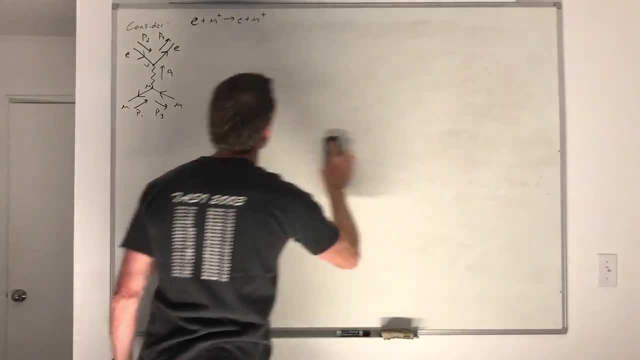 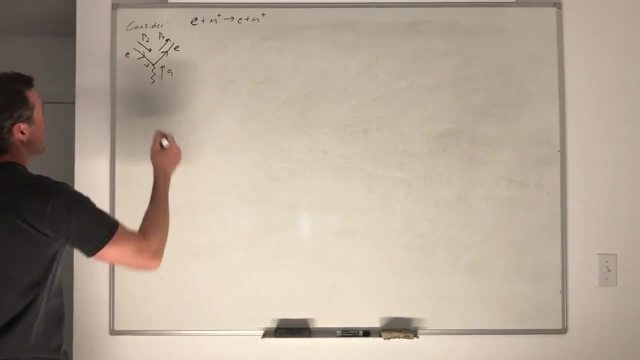 And then we're going to have a little bit of time to think about what we're going to do next. So, if we can set up a little bit of time, we consider this process, But we consider a higher order diagram, All right. 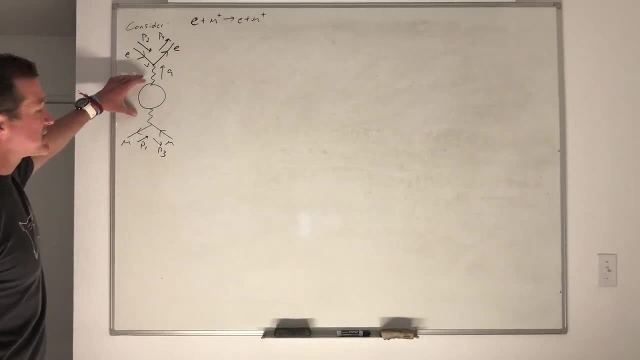 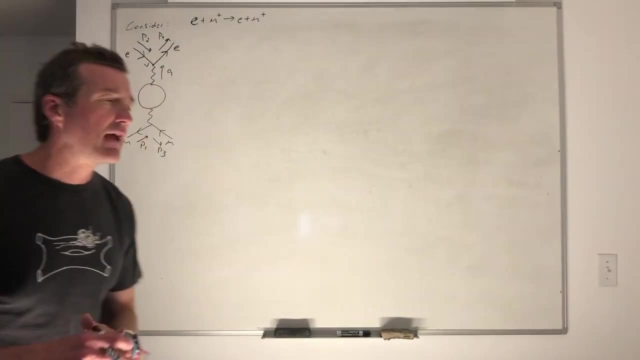 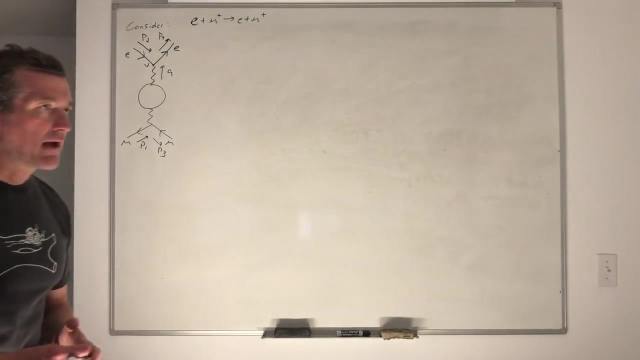 so far, everything I've told you has not really explained how you would handle an interior bubble or just more in complicated interior stuff. in fact, the feature of this diagram, which is different from the previous diagram, which i haven't really told you how to handle yet, is a loop. 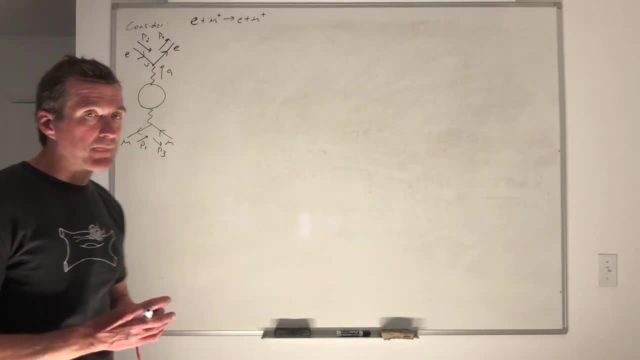 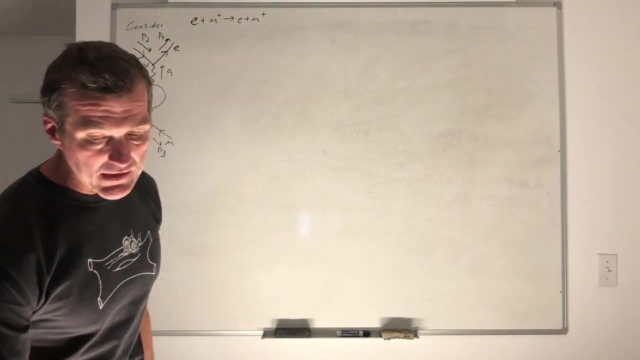 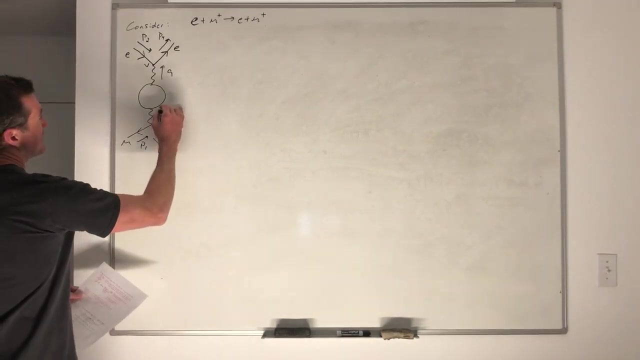 okay, the previous diagram had no loop. it was what's called a tree diagram. so this is an example of a loop diagram, and what i'm going to give you is basically what you apply to any loop that appears. so, first of all, i'm gonna be a little bit sneaky here, um, and trim things. 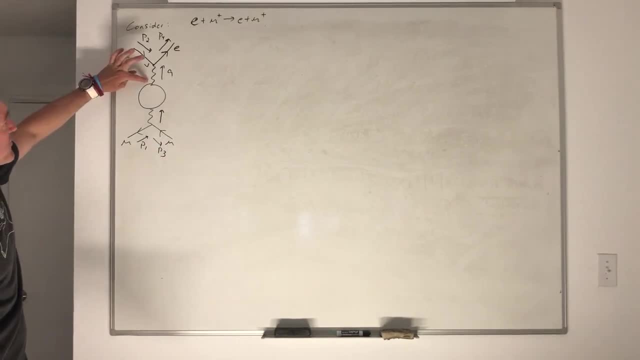 down. so, um, if the momentum traveling in this photon line is q, how much momentum do you think needs to be in this photon line? probably q? yeah, it's got to be q as well, because you know, if this q were different than that q, then momentum would not be conserved, so we might have 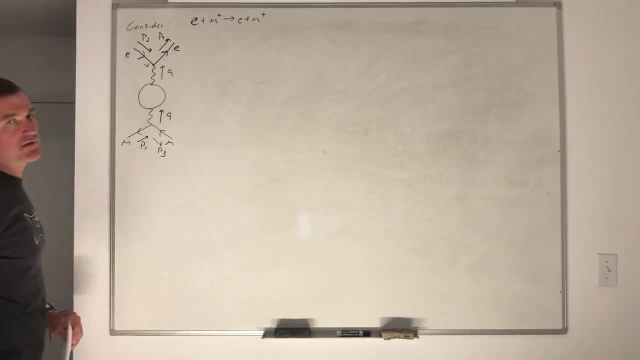 well, instead of labeling this q1 and q2, we might as well just label them both q. this kind of cuts down on the delta functions you have to engineer. and then, moreover, if i choose the particle here to have a momentum k, how much momentum does this particle have to have? 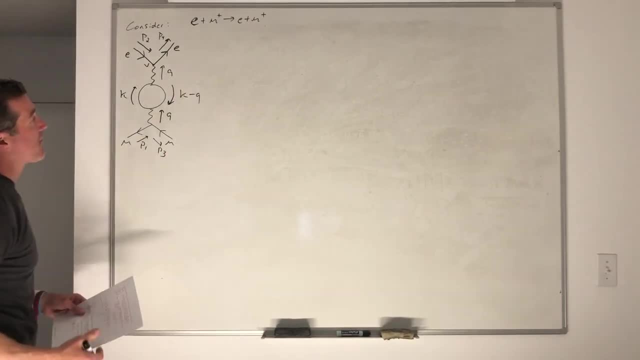 yeah, it has to have k minus q, so that i mean this is going down and this is going up, so the difference, so the sum of these, would be this, or it would be this minus this, but anyway the total is q. okay, the k's cancel. so i'm going to assume that this is maybe an electron and an. 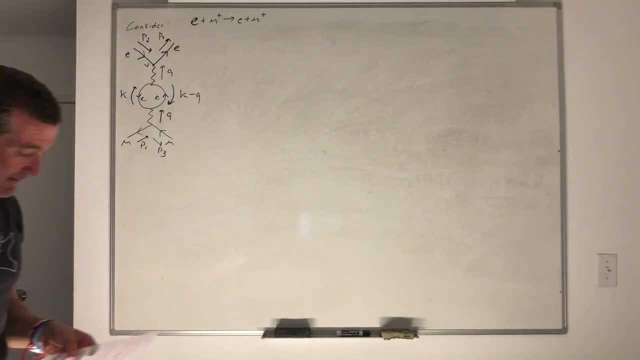 anti-electron doesn't really matter. you could use muons or whatever. okay, so, um, in doing this diagram, most of it should be familiar, right? you start with spinner sandwiches. so you do the outgoing electron, the vertex factor, the incoming electron. so you have a u bar 4, i, g, e, gamma, mu, u2. you do an incoming 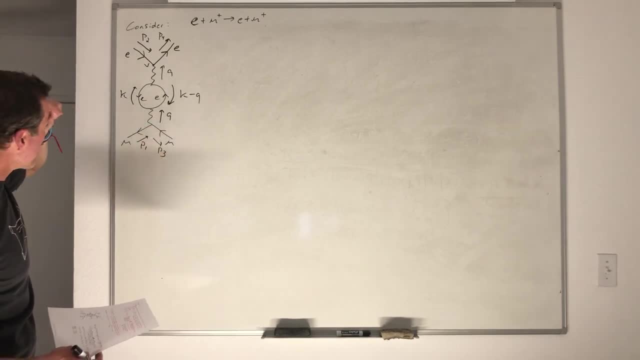 anti-particle, a vertex, an outgoing anti-particle. so you have a v v, bar 1, i, gamma, nu, v3. all of that is the same. you can put in propagators for the photons. but now you've got two more interaction vertices. okay, these are interaction vertices here, and then you've got more internal. 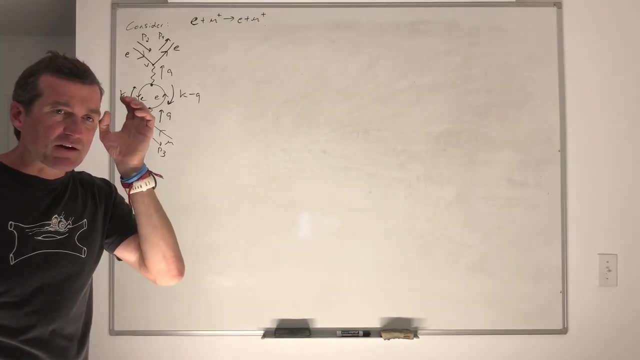 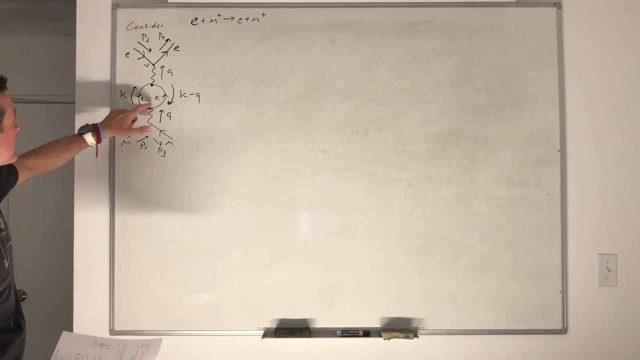 lines, and so you might wonder: you know, how do i make a spinner sandwich out of that? do i make this a u k bar and this a u k, you know? i mean it's, it's kind of weird, right, because i could call this like i could try and say that that gets a v. 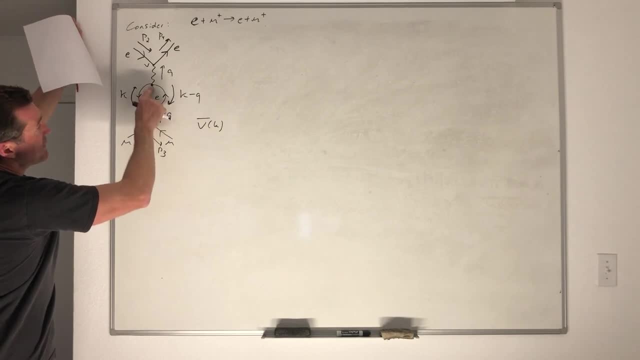 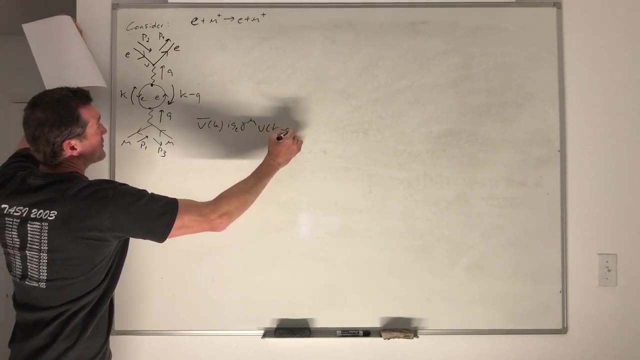 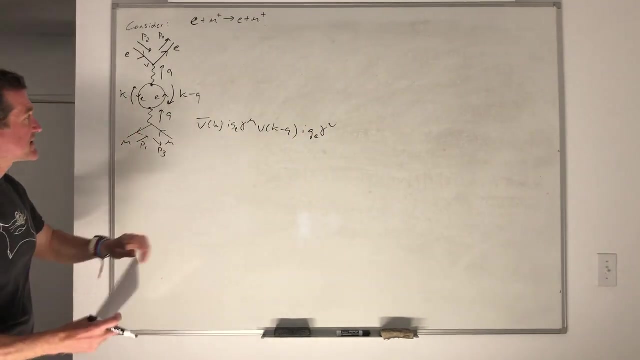 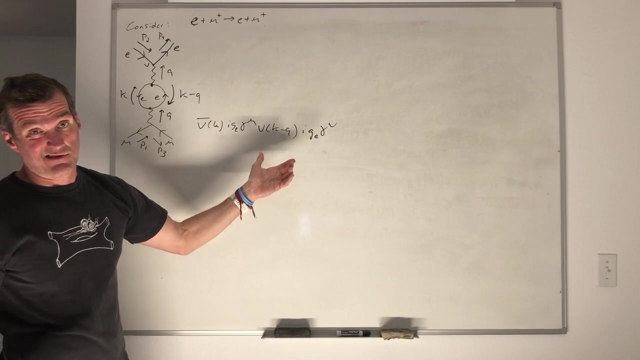 bar of k and then i go to a vertex and then i have v of k minus q, but then i have another vertex and this is screwed up because even though this gamma matrix is sandwiched in a spinner sandwich, this one is not okay. so that's kind of that's kind of crappy. so there's a rule for how we deal with these. 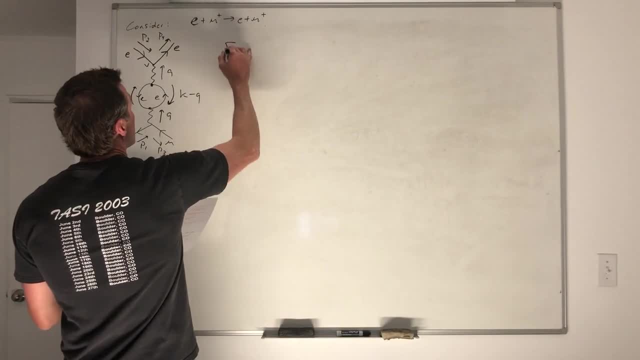 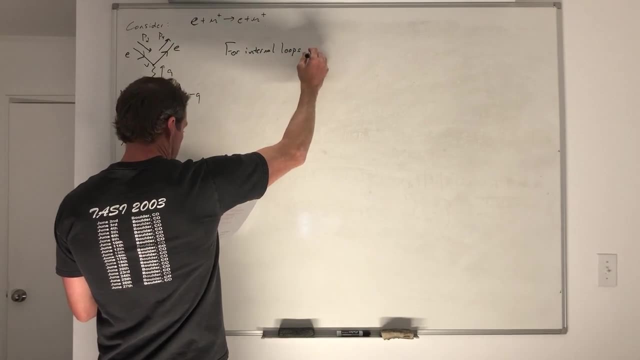 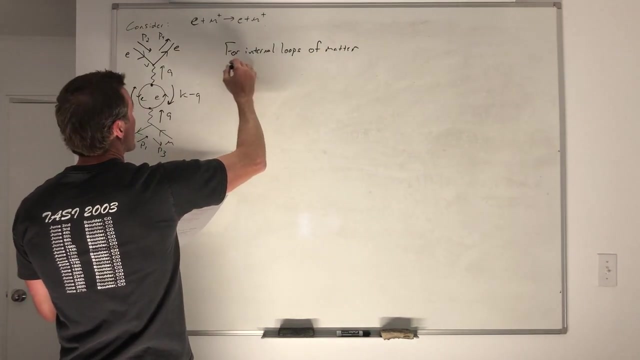 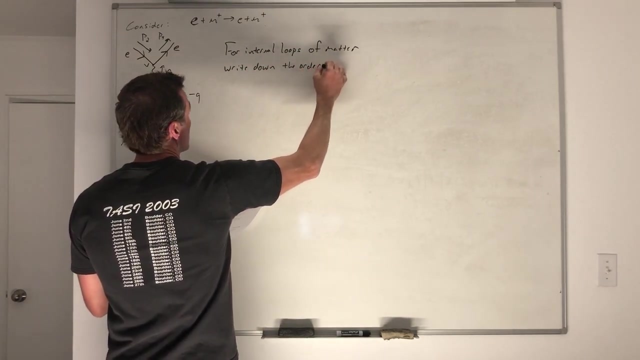 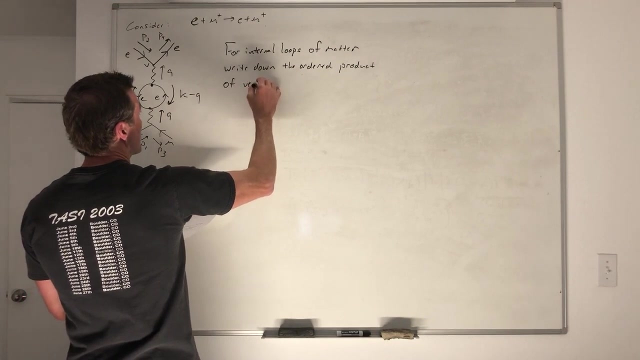 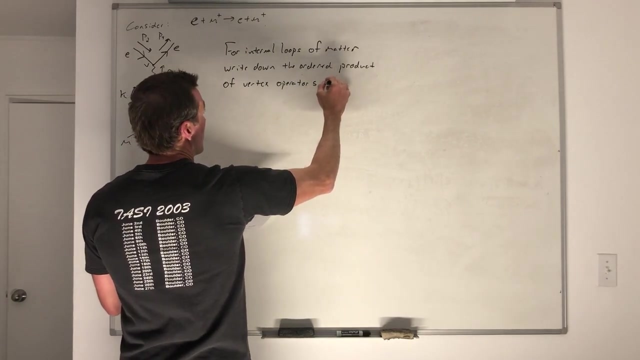 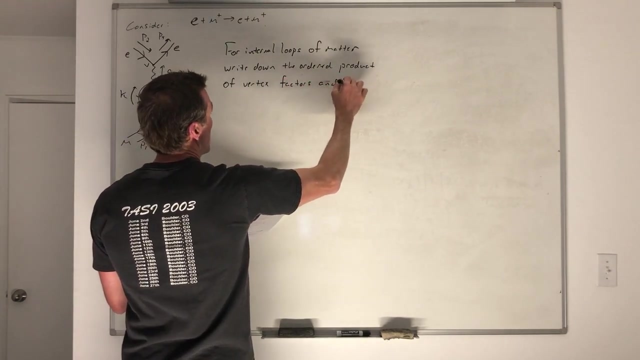 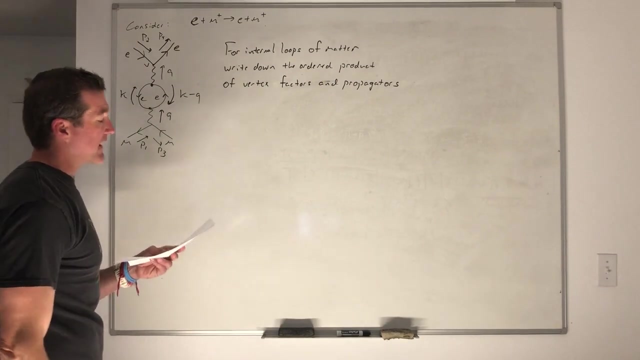 and the rule is the following: for internal loops of matter, write down the ordered product, so using a v turtle mixing. author of vertex operators. oh sorry, vertex factors and propagators, which i just did and i just erased. so that was stupid, okay, so let me. let me quickly write it down again, so maybe i can get over from our easily. 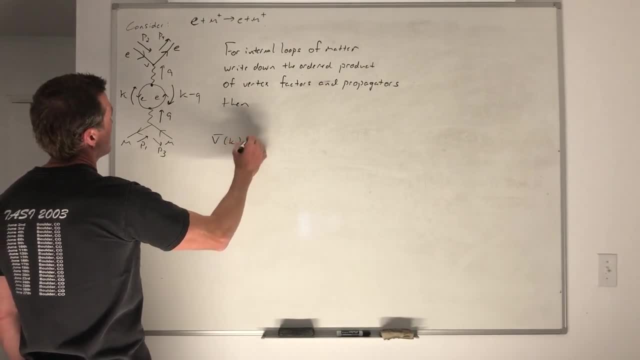 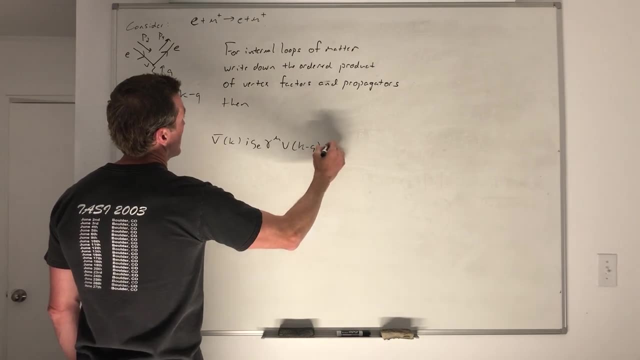 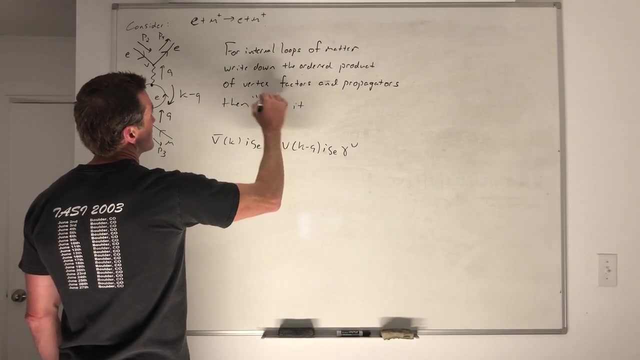 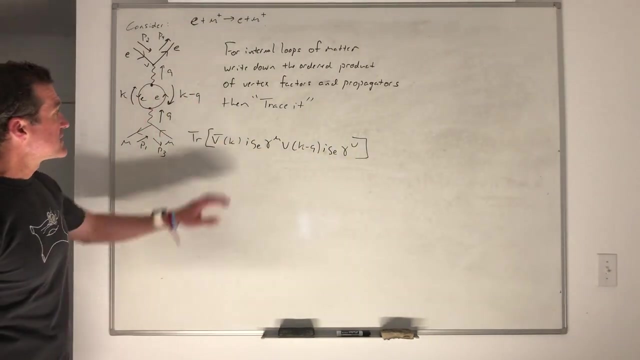 let's see. Maybe I've got a v bar k i g e gamma mu, v k minus q i g e gamma mu And then trace it. That's a trace over spin space. So what's nice is that if you're tracing it, 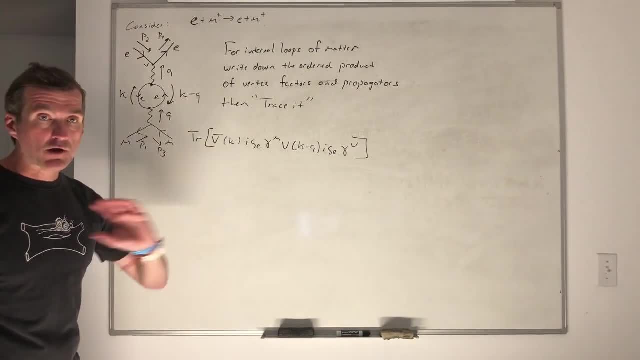 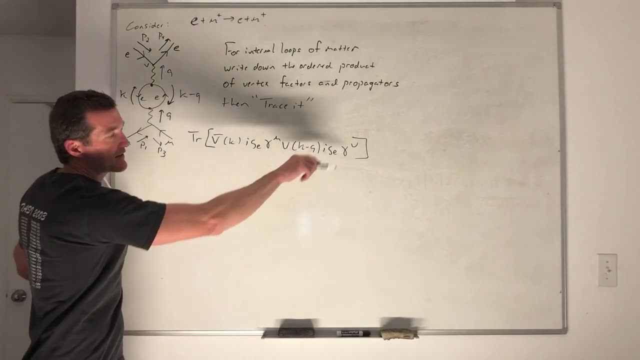 the spinorial part of it's going to disappear, because you're basically tracing over all of the spin matrices. They're going to become numbers. Also, if you think about it, the trace is invariant under a cyclic permutation. So I could have started with this vertex and then done the v bar and the i, g and this. 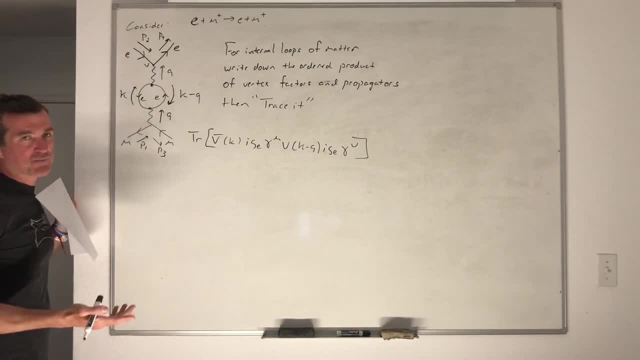 That's just saying, if this is an internal loop, there's no special place to start. You could start here and then do this propagator, this vertex operator, this propagator. Or you could start here: do this propagator, vertex operator. 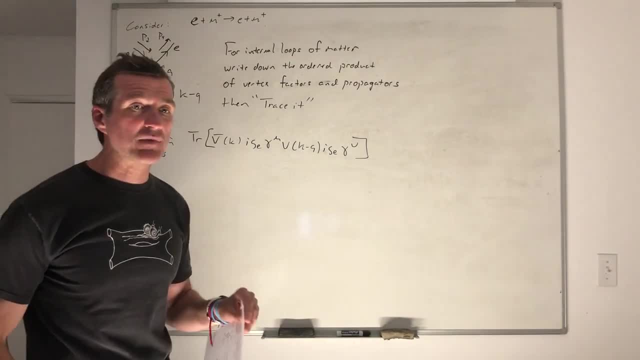 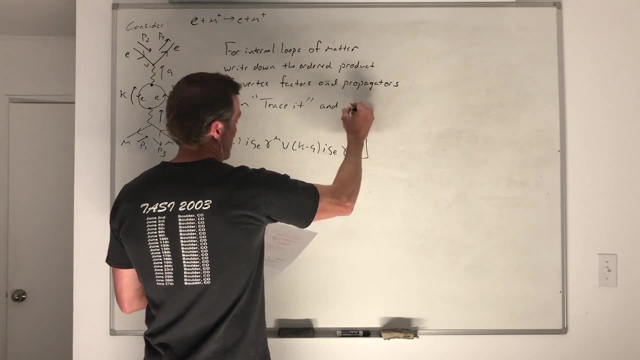 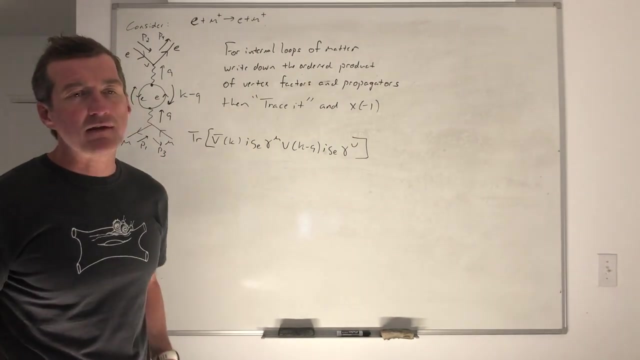 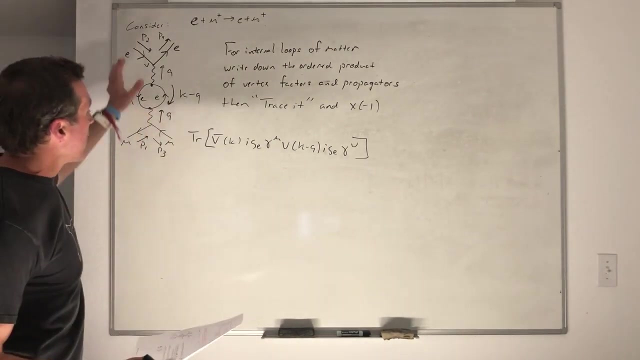 it doesn't matter with the trace, as long as it's a cyclic permutation. And then there's, of course, one of those weird final steps: You multiply the answer by minus 1.. So I'm not going to write out what this ends up being. 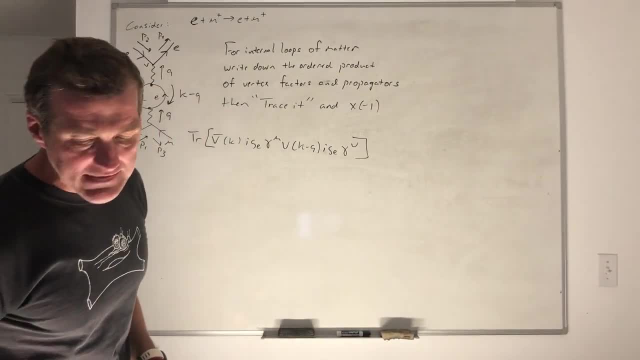 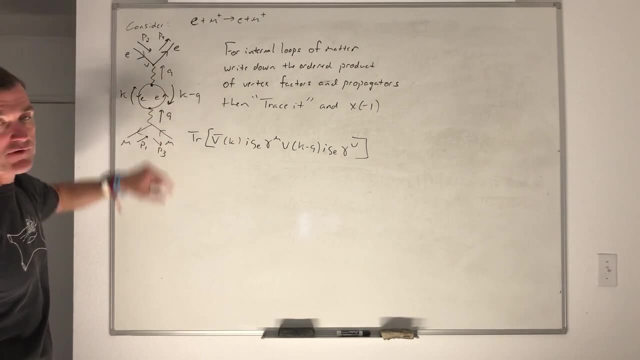 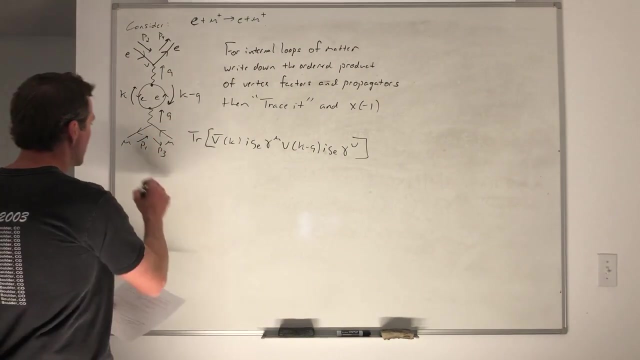 It's going to be in your notes. It looks quite similar, Similar to what we had before, except there's this extra factor that is the trace of summing over this internal momentum or this internal virtual particle loop. Okay, And then I'm just going to leave you with one interesting observation that follows from Furry's theorem. 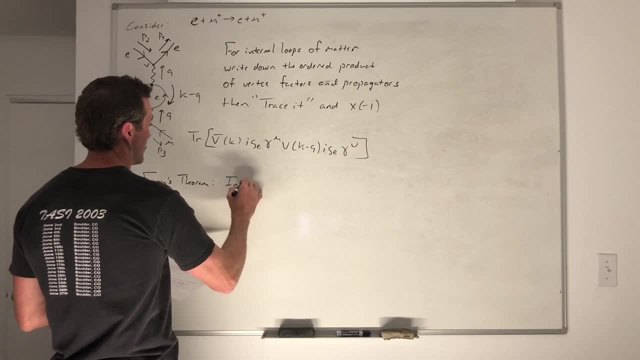 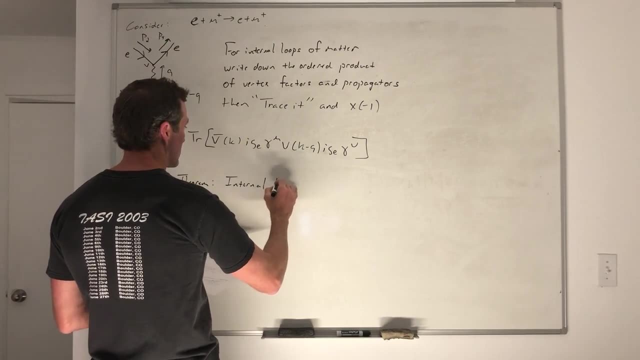 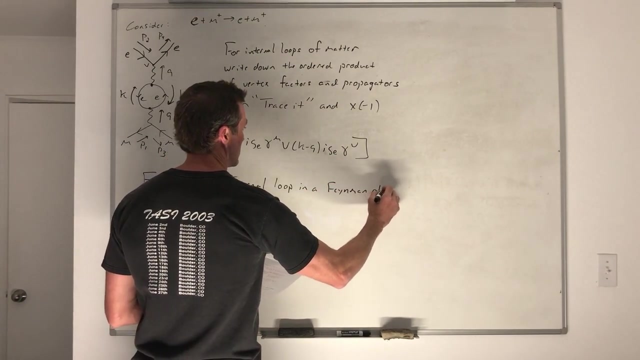 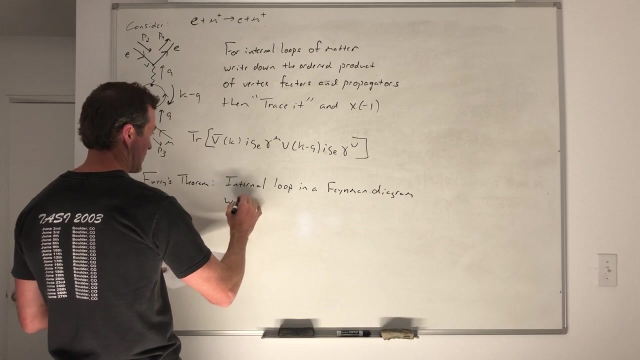 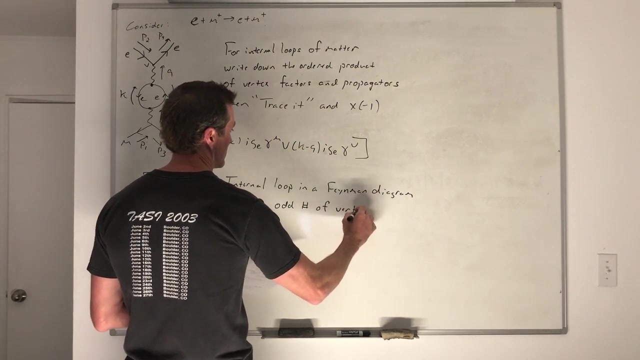 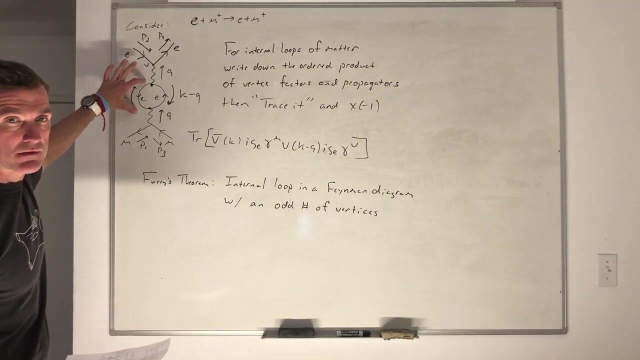 When you're doing Furry's theorem. or Furry's theorem says: if you have an internal loop with an odd number of vertices, Okay, how many vertices does this loop have? Two, okay. 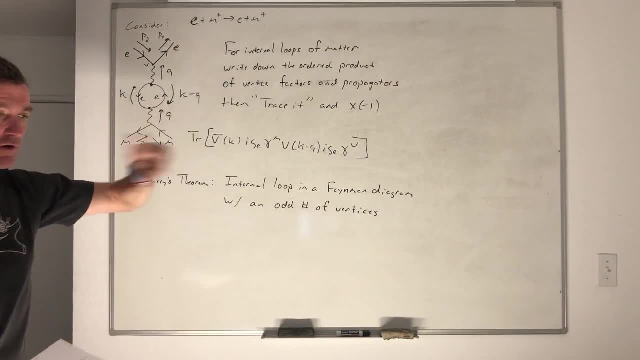 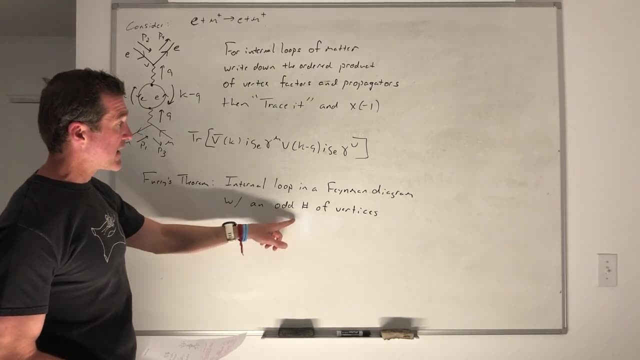 But you can imagine, you know, coming up with a process where there's an internal loop and there's three vertices on it. Well, here's Furry's theorem: If you have a diagram and you have an internal loop with an odd number of vertices. 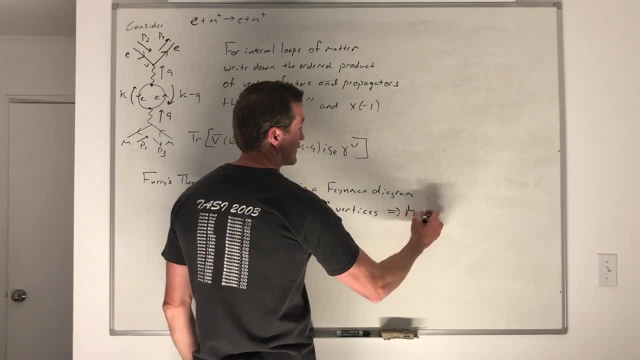 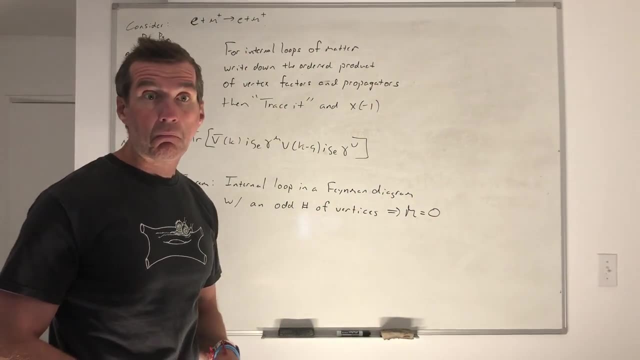 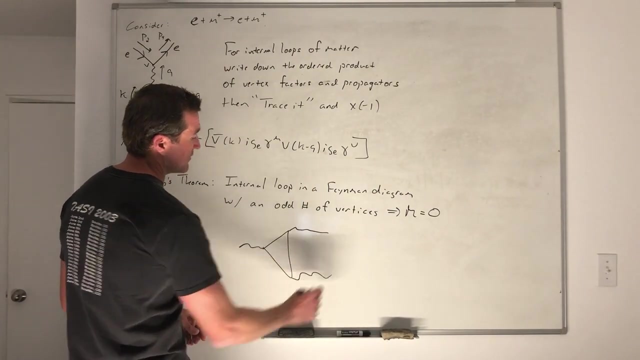 That implies that the amplitude associated with that diagram is zero. Pretty sweet. 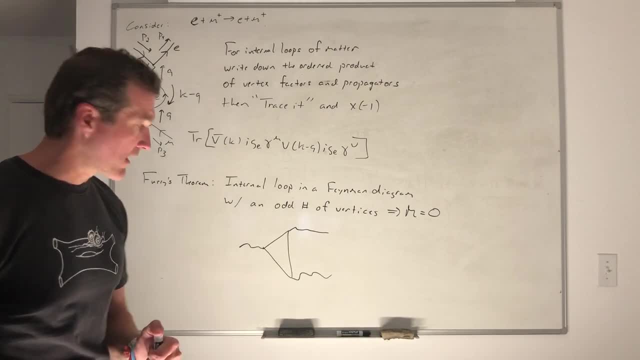 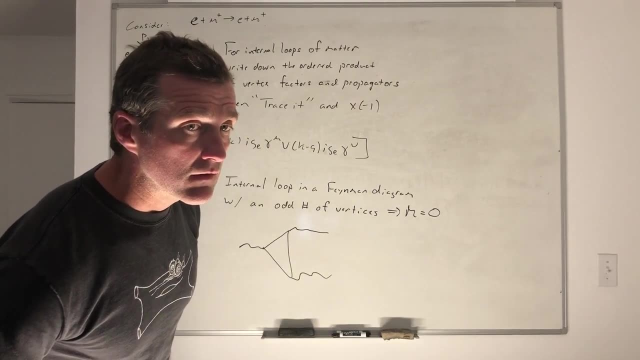 Just to give you an idea of what an internal loop might be in QED there's one Okay For the process that we're looking at here. would we ever have an internal loop that only has three vertices? 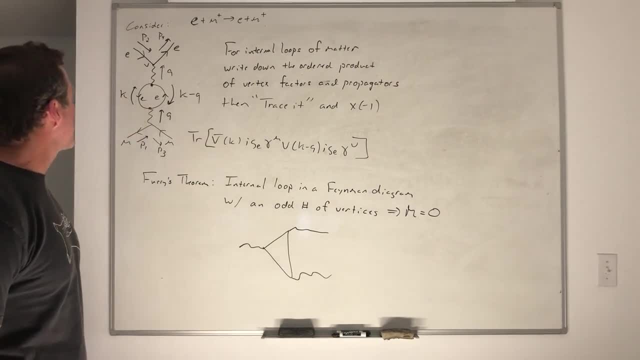 Well, I would have to think about that. It would just pop up somewhere else. I guess Could you just put another triangle on the end of that and condense it What you drew on the bottom there, just put another triangle next to it and then you have one photon going in, one photon going out. 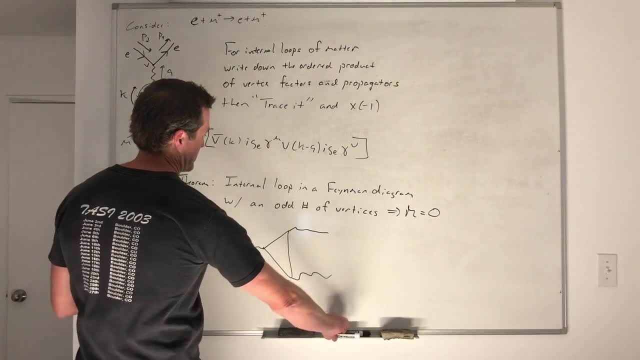 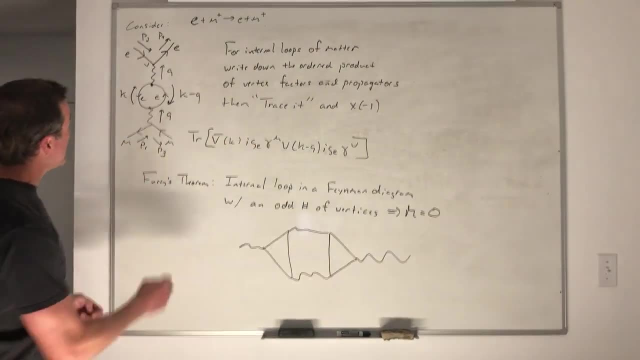 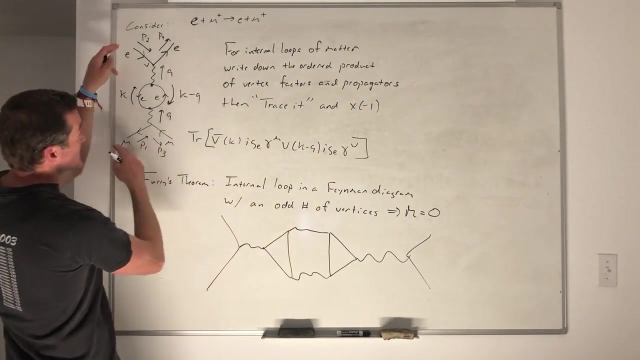 It's just a higher order. Yeah, yeah, there you go, Yeah, so if this was So, let's take this and just stand it up that way, so that it's this process, This diagram would give you zero. There you go. 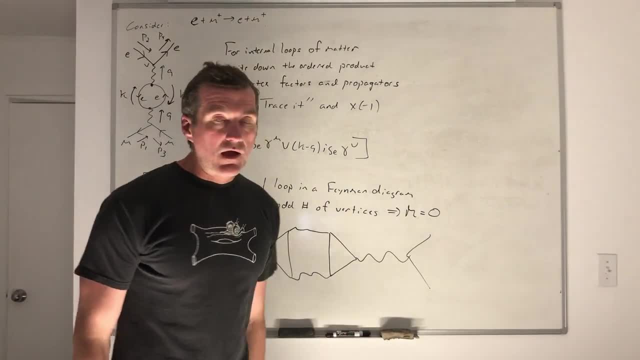 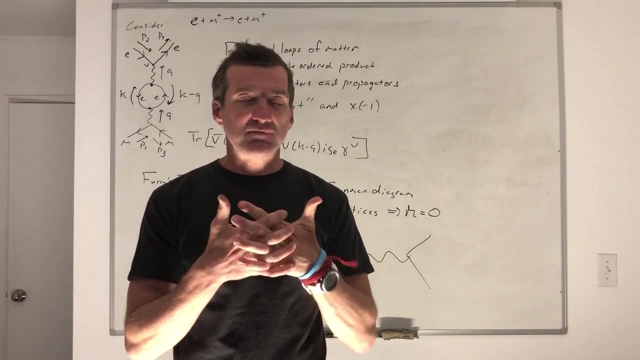 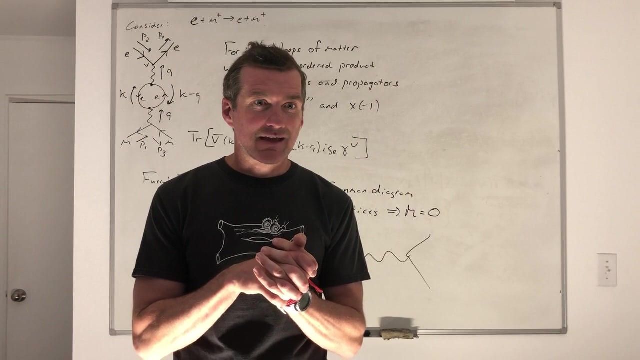 Yeah, All right. Thank you so much, everyone. Sorry for running 15 minutes over, But this means that next time we get to start straight away with QCD, which is fun, right after you take your homework quiz. I'll remind you I'll be on Zoom tomorrow from about 5 to 7.30 or 8.. 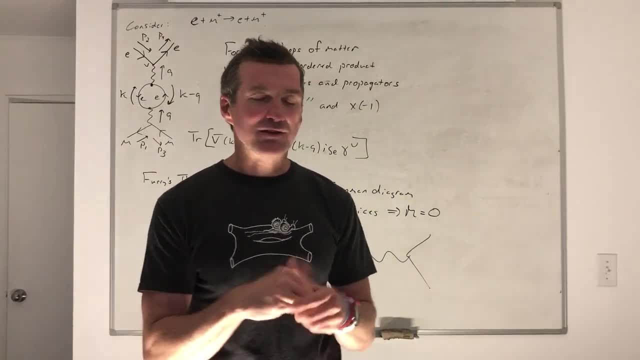 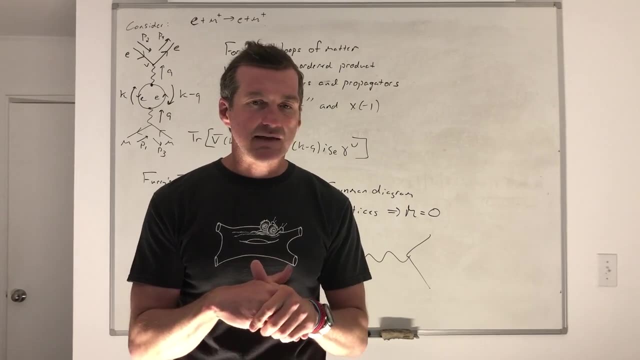 Last time I just stayed on until everybody left, which is about 7,. but anyway, If you have problems with the homework, feel free to contact me. You can also email me questions. I'll answer emails if I can. as long as I can, you know, type an answer to the question that you're asking. 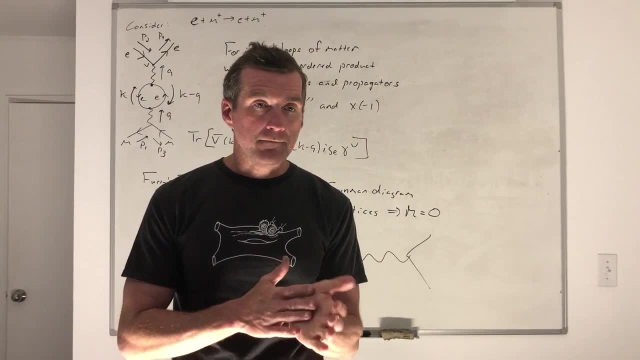 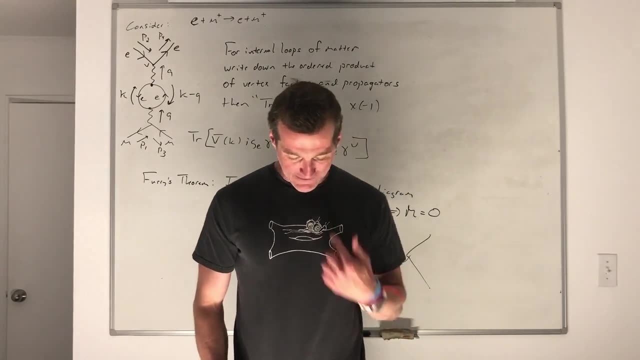 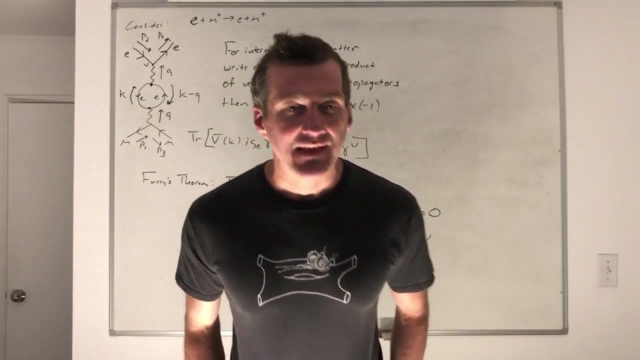 Are there any questions before we go? What's your T-shirt? Oh, I forgot that I was wearing this. Well, what does that look like? Looks like string theory, like a string theory diagram. Yes, So it is a string theory diagram. 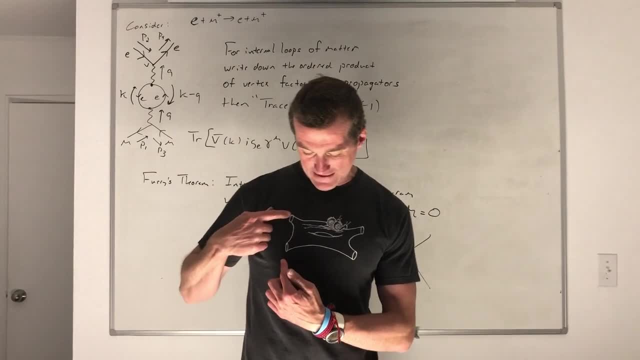 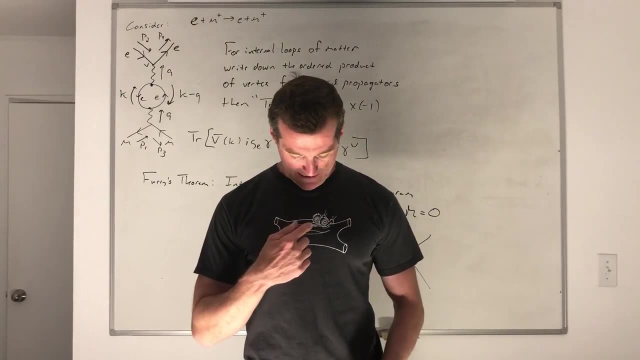 We're scattering. Oh, it's so awesome that I did this lecture. We're taking two closed strings, bringing them in, They're scattering, and then two closed strings go out, However, and it's a one-loop diagram. Oh my God. 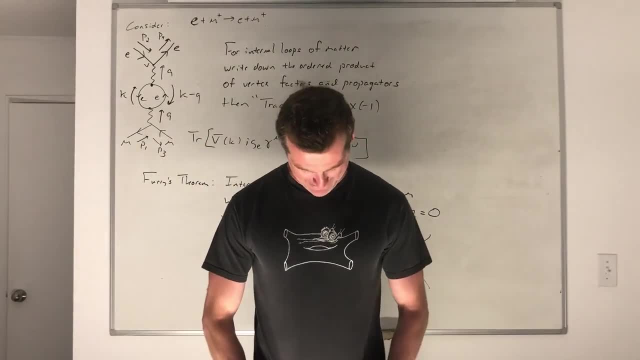 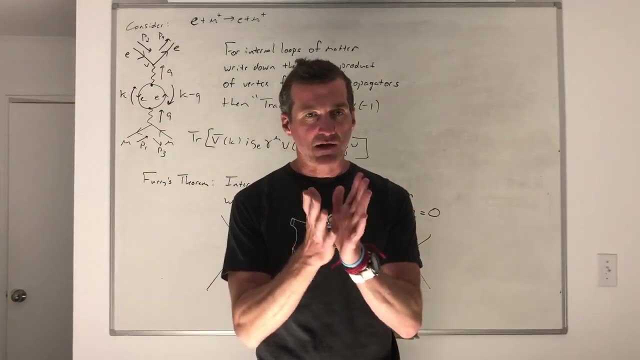 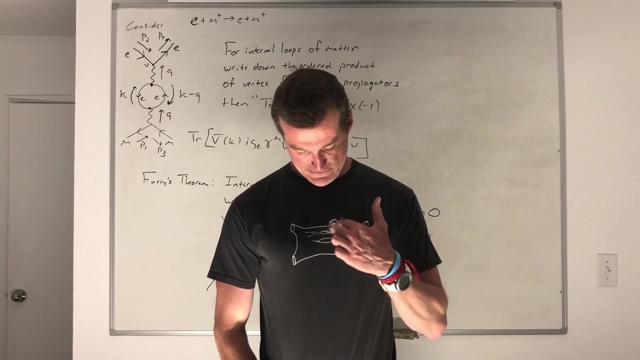 It's that fucking diagram. Holy cow, This is crazy. This is what a one-loop diagram looks like. A one-loop diagram that looks like that is in string theory, because all of these rigid lines and little intersections become smoothed out. Anyway, on it are two snails.